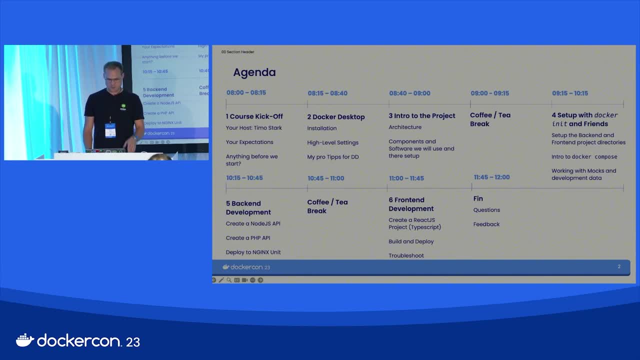 And then we'll start with the backend development and create a node. And then we'll start with the backend development and create a node. but it's not a programming course. today I'll give you some best practices I'm using in my projects. 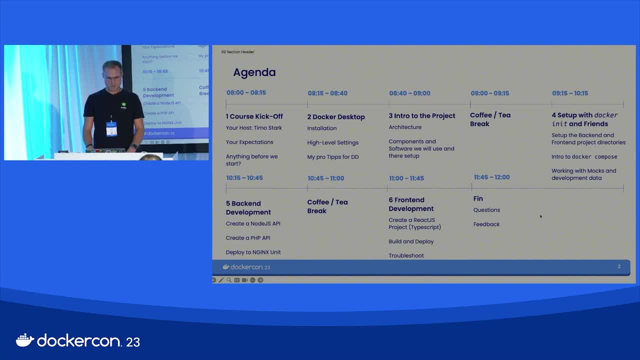 but that's basically what I wanna do. Then we have another break before we are doing the final things, do some front-end development using Reactjs and then we try to glue everything together: the APIs we have created and basically the front-end. 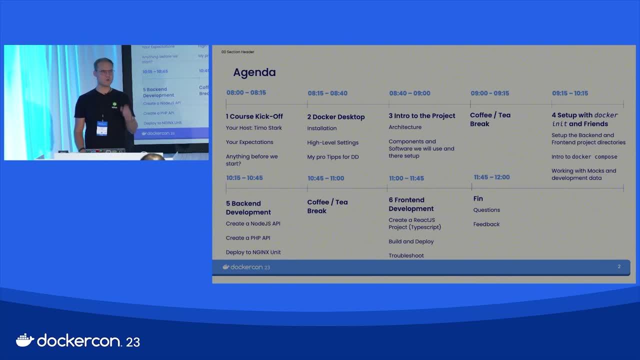 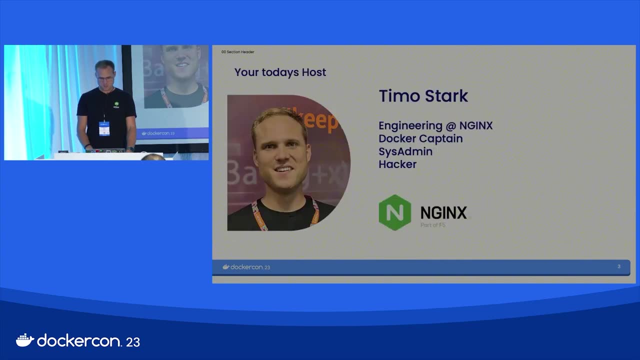 And at the end, yeah, we'd like to get your feedback and if there are open questions, we can answer them. So that's actually the plan for today And before I get your question, and what do you expect from today, would like to introduce myself. 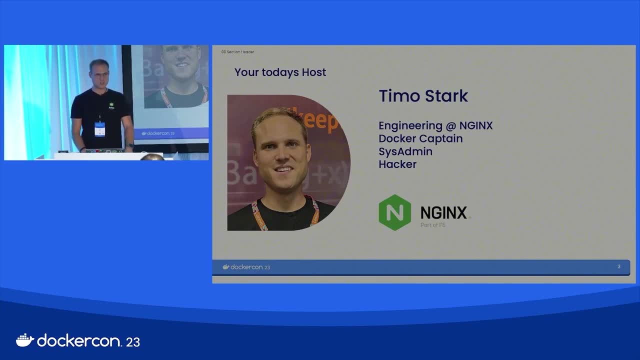 My name is Timo Stark, I'm from Nginx, working at the engineering team for Nginx, and I'm here as a Docker captain to deliver this workshop, but have more than 12 years of experience with web development. That's what I do half of my life. That sounds crazy, but I'm 32 years old now and I started web development when I was 12, so that was basically always my good love in development was something for the web, and I basically started with Docker back in 2017.. 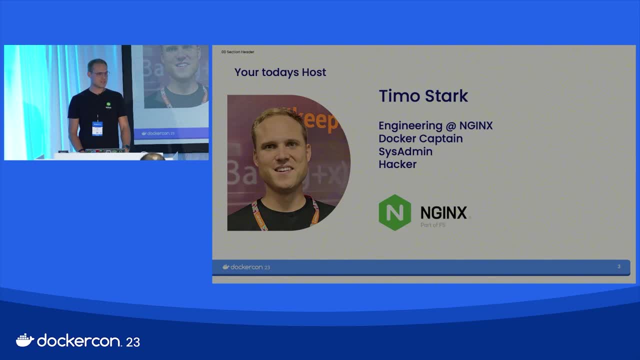 That was my first DockerCon in Austin and since then I'm using Docker heavily, especially for my day-to-day dev jobs. When I'm not engineering at Nginx or doing Docker captain stuff, I'm doing Docker, doing some sysadmin site work, Linux server administration. 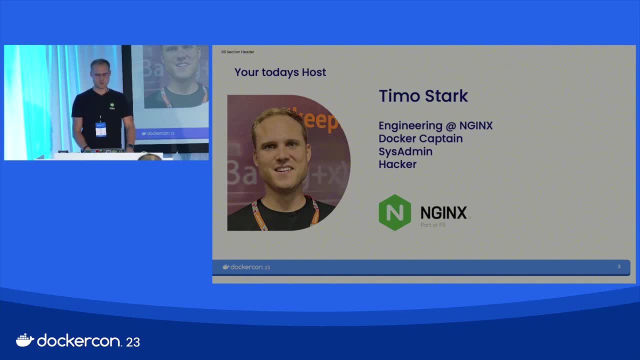 or just hacking around on bug bounty programs and do some security stuff at the site as well. Right, so that is personally basically what I'm doing, And now I would like you to get if you have any expectations, like: do you have anything to share? 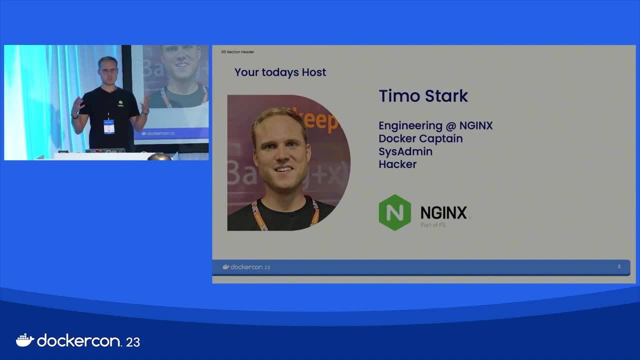 why you are here. basically, Do you have any questions, specific questions why you're here? If not, that's totally fine, But if you have something in mind, that would be good to know. Okay, so I am speaking tomorrow at a similar event like Docker desktop. 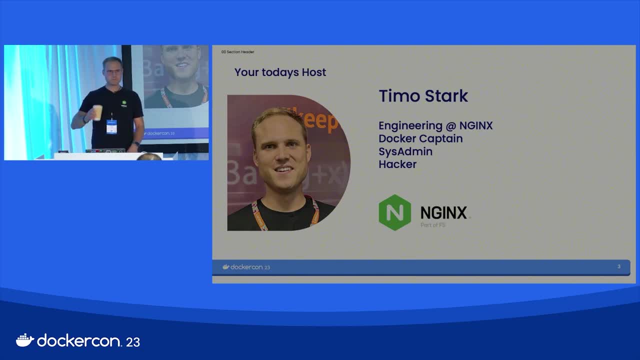 and webpagging and stuff. So I have this day-to-day inspiration how you're setting it up. Thank you, Let's see, like what is my. Okay, Oh, amazing, Perfect. Yes, I have some issues. I mean, I have a directory with Docker. 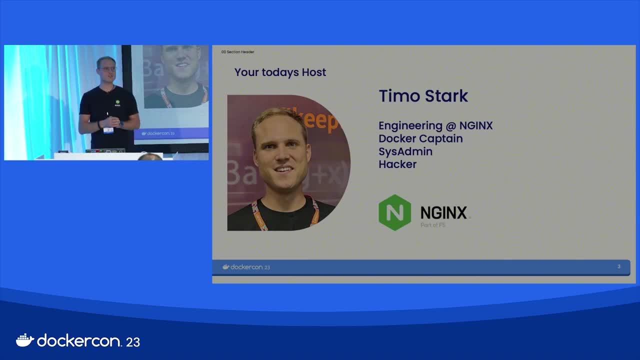 so I'm hoping to get some insight into that. Okay, Connecting Active Directory using Docker? Okay, Okay, good point. So just make it clear, you have a Docker container and you spin this up and then you can from this Docker container. 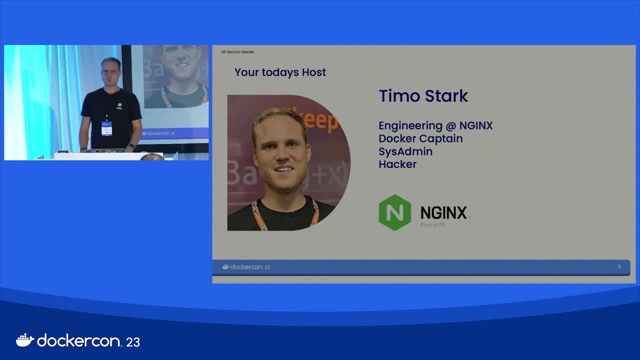 you cannot do an LDock connection. Okay, good, Good point. We'll try to cover this a little bit so we can talk about Docker networking in general. Okay, Okay, I'll just throw this out there. I work for a company that has a very large 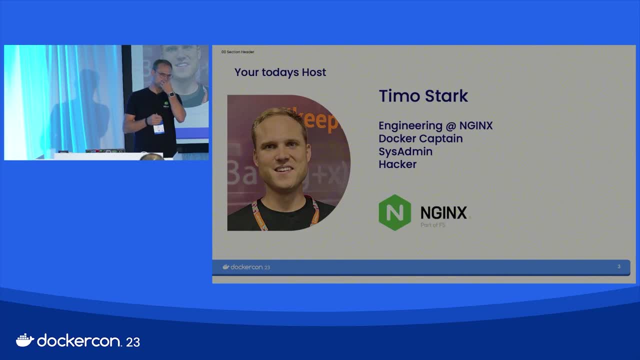 monolith monorepo spot and just how that's impacting that. All right, So I have one application with a couple of services in it and, Yeah, So you know we could split it into multiple containers perhaps. 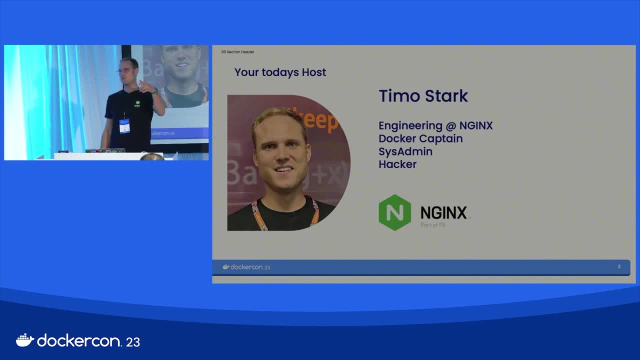 Oh, okay, Perfect. So the question here is what fits in a single container and what can be orchestrated in multiple containers. Okay, Perfect, Thank you. Yes, I'm moving a NET 6 application into a web app. I want to put an API on it. 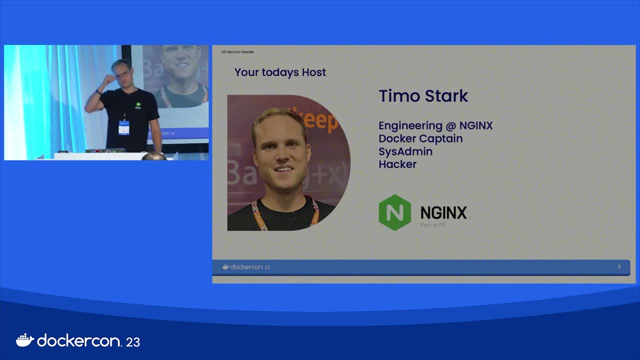 and then join it with an existing static. Okay, Perfect, So it's most questions about packaging and basically how to use Docker containers and Docker files to pack your and ship your applications. So that's definitely something we'll cover. Perfect, All right. 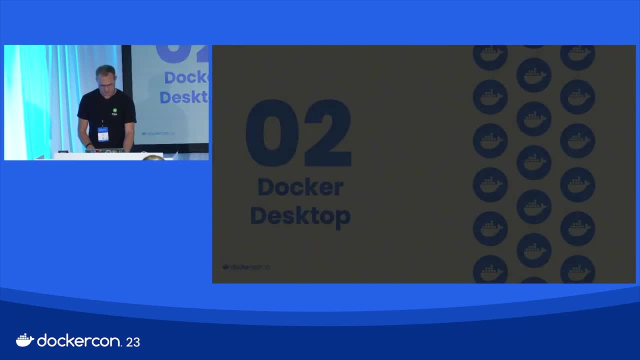 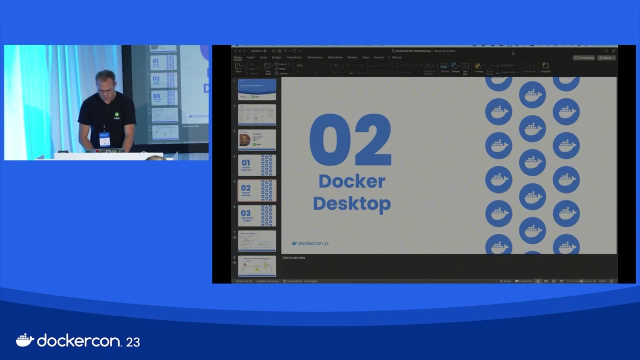 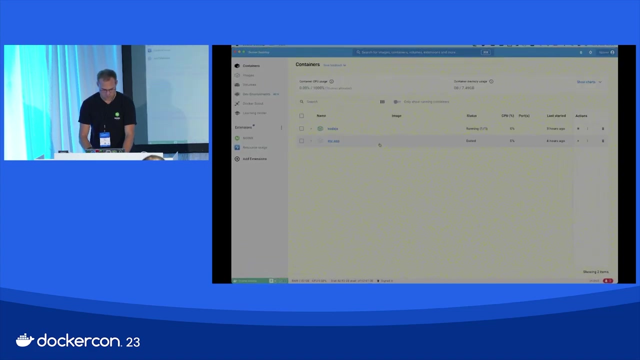 Great. So next step is Docker Desktop. Let me just bring this thing up, And Yeah, there is a neat trick. As Docker Desktop is fully web-based, I mean, we have this little thing right. that is the. 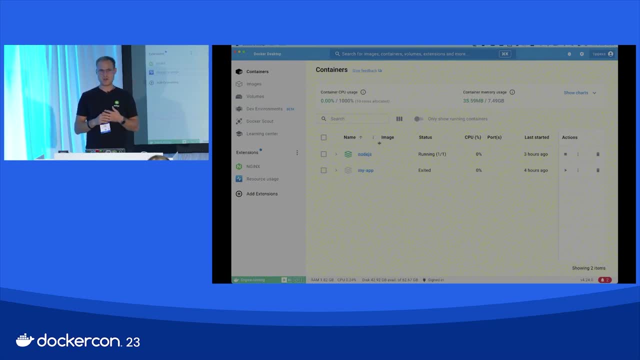 the, the, the, the wrapper application you can install. If you haven't already Docker Desktop installed yet, you can go to the Docker website and install it from from the website. Is there anybody that needs to install Docker Desktop right now? 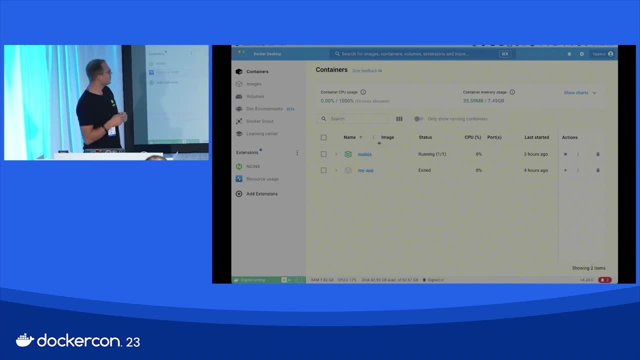 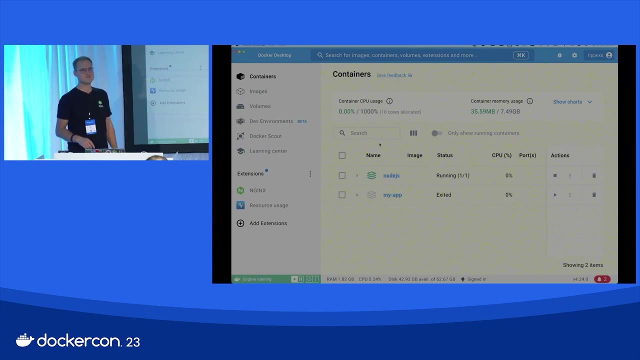 Okay. Yes, I'm getting a slide that I've been playing. It's hard for me to get it on. Maybe it's an adapter. Yeah, it is, We have. It's a bit light, It's like Right. 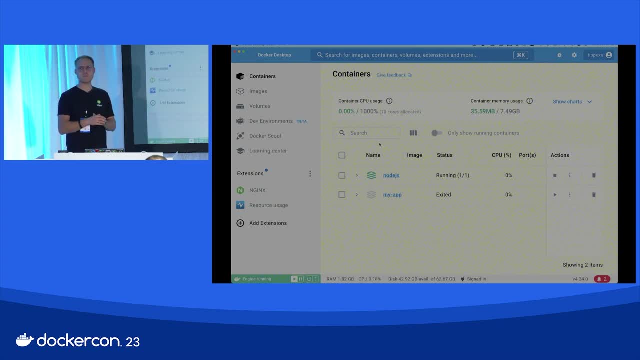 Yeah, this one is better, but I've already, I've already tried to fix that, but it's a. Can you see that? okay, Is that? Yeah? Otherwise, we have more seats here, If that, If that works better, then 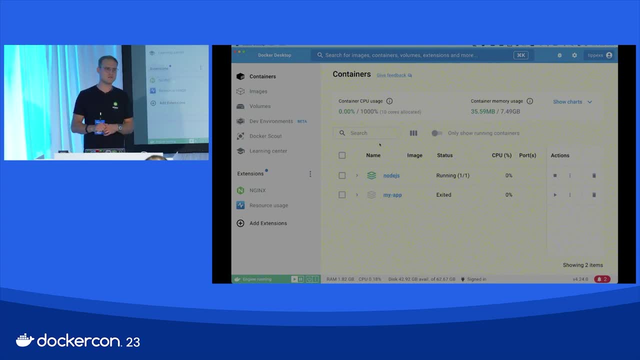 Sorry for that. Yeah, Can we get to the live presentation at the same time? I think so. The link was sent by email. I didn't. I didn't receive any link. Okay, Just do it. I don't know. 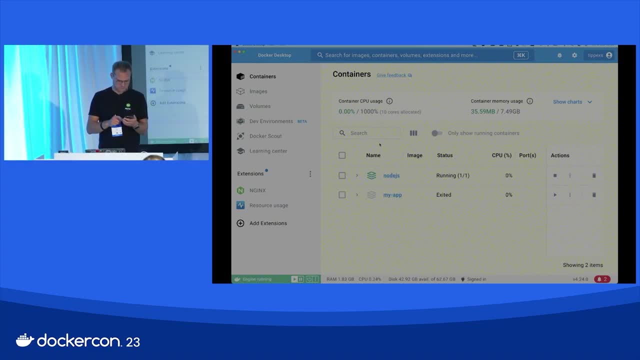 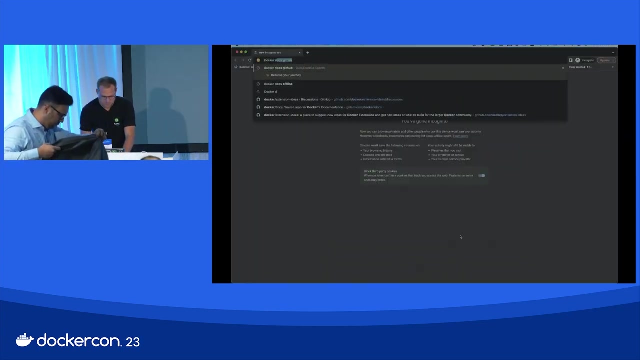 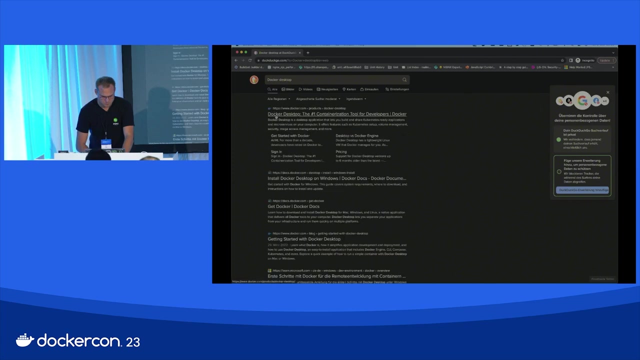 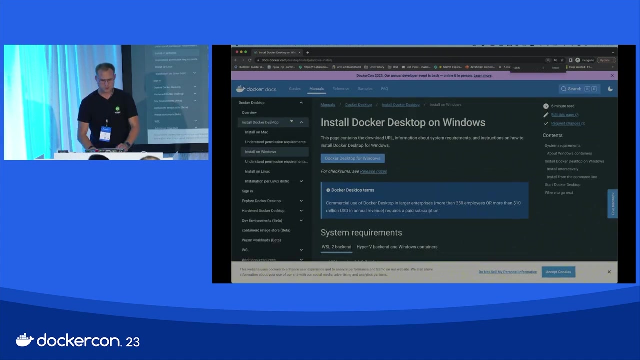 Awesome, All right. So let me spin up a new thing here real quick. Okay, All right, If you go to like, there We have docs- All the Docker people have docs- about installing Docker Desktop on Windows and Mac and Linux. 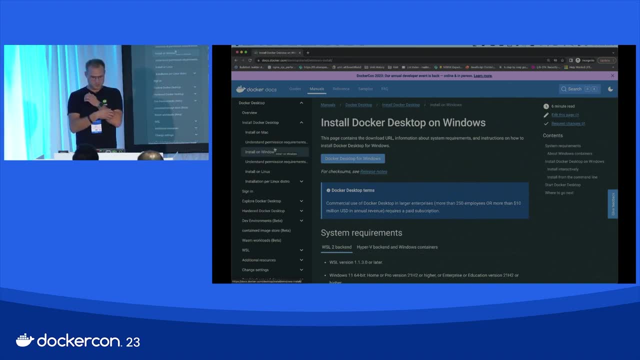 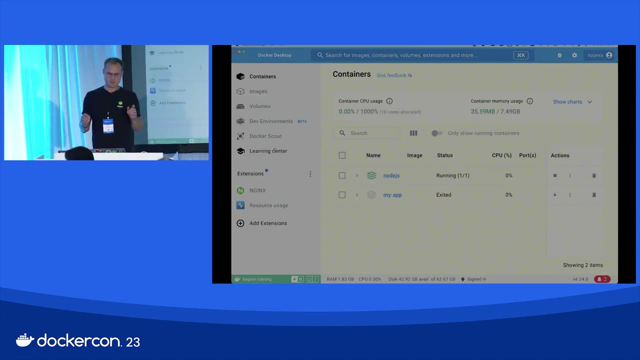 basically like in Ubuntu. And the interesting story about Docker Desktop in general is: I haven't touched- Not kidding, I haven't touched Docker Desktop since the early time of 2003.. 23,, right, So that was. 2023 was the first. 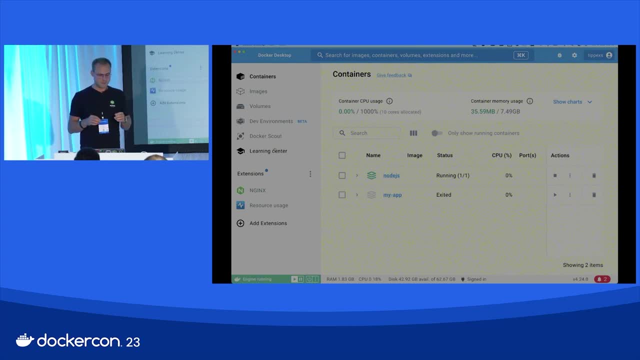 Actually the first year I have touched Docker Desktop at all, Because I've created the Nginx Docker Desktop extension. that was the main reason why I have touched Docker Desktop for the really first time And like I loved it after two hours of using it. 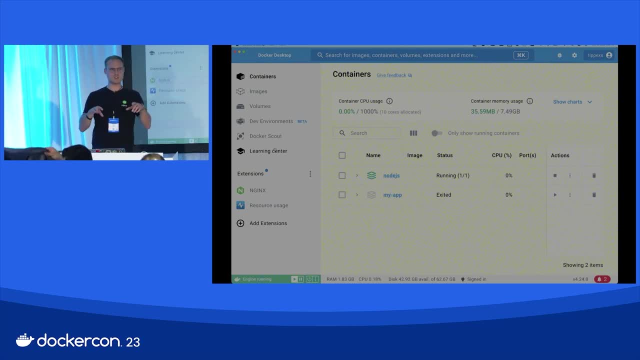 I was always the CLI person working with the Docker CLI while doing development. no matter what I did, And And And After using Docker Desktop for just two hours. it was so, so, so much easier than just doing all this typing. 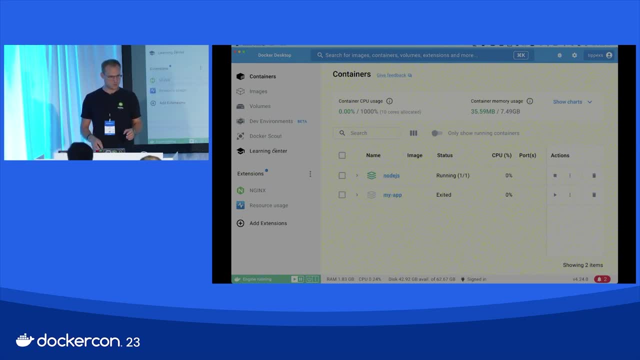 Because you can get a lot of insights, and that's why I would like to show you a couple of tweaks, a couple of things: how to navigate in Docker Desktop. It's not really a session about Docker Desktop, but I just would like to give you a little. 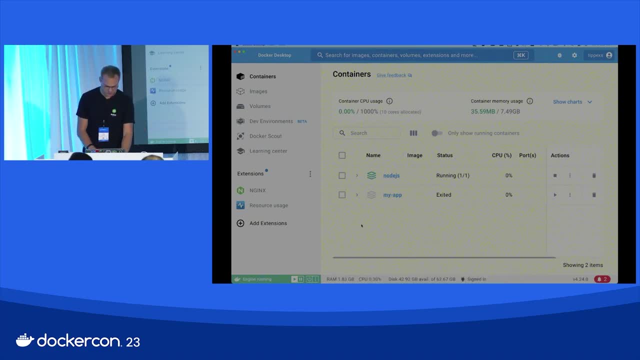 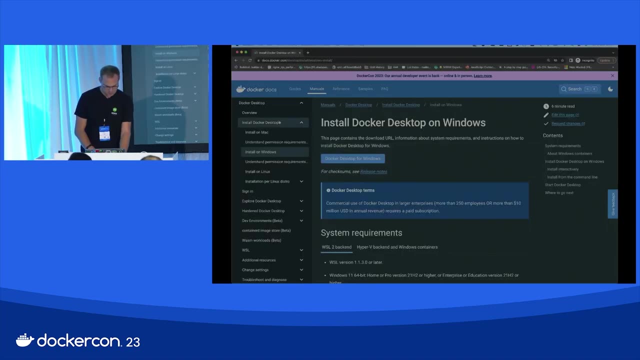 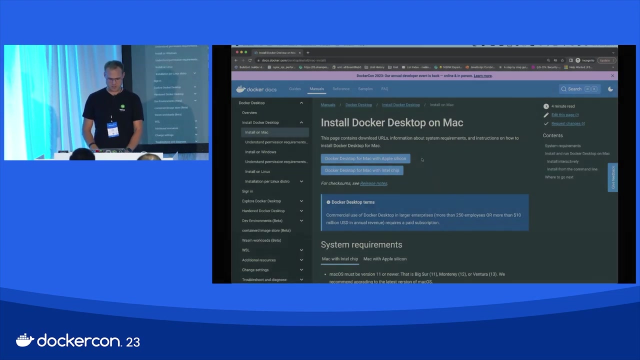 walkthrough through Docker Desktop what you can actually do with it. All right, So, as I said, you can download it from the website And ping here: install for Mac. Make sure you're using the right chipset, like Intel or the M2 chip. 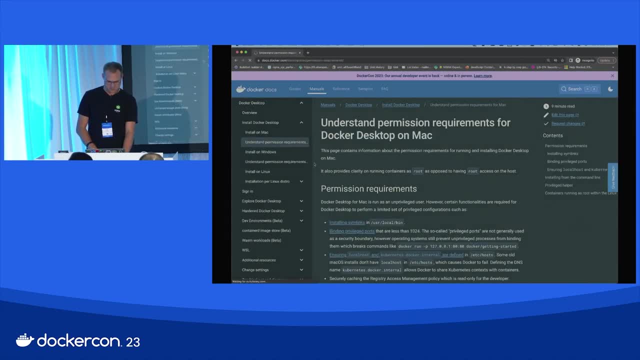 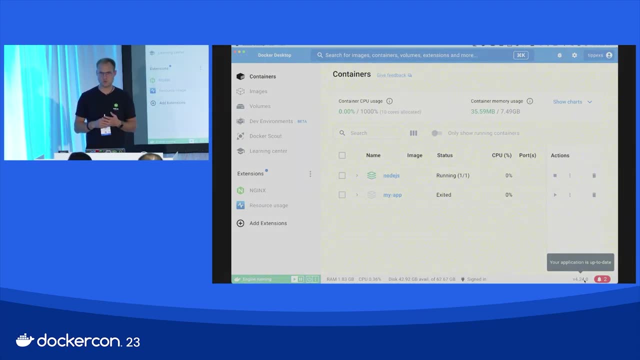 Then, Or Windows, Then you can install it, Launch it. So I'm using the latest stable version, which is 2.24.. So then, what you can do first is you can sign into your Docker Hub account, Right. 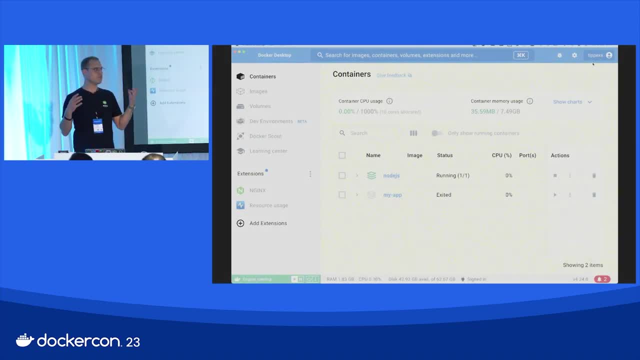 So if you sign in, If you sign in to your Docker Hub account, this helps if you have some private images, for example, in the Docker registry. If you already signed in to your Docker Hub account, you can pull them from your container. 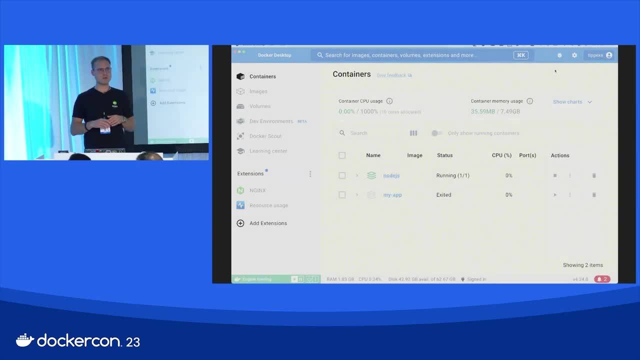 registry on Docker Hub without typing in the password manually into the CLI. So then, here on the navigation, you have the containers, and these are basically the containers that are currently up and running. And the neat thing with- Basically- Basically- this overview is that we can pause a container, we can restart a container, we 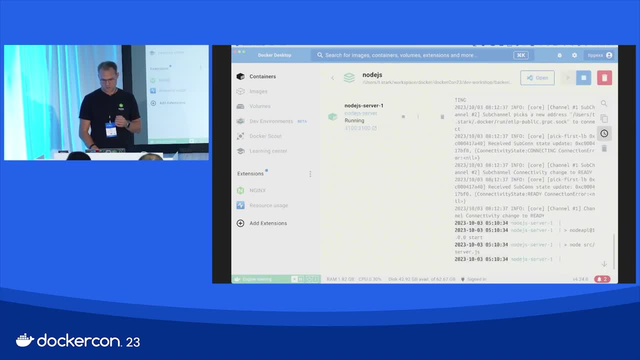 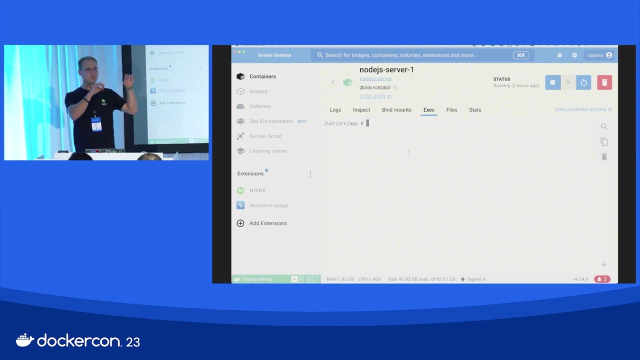 can delete it. but if you click on the container you have basically the output. You can copy stuff to the clipboard. Then you can directly execute in the container. So basically what you normally would do with Docker: exec something. and the neat thing. 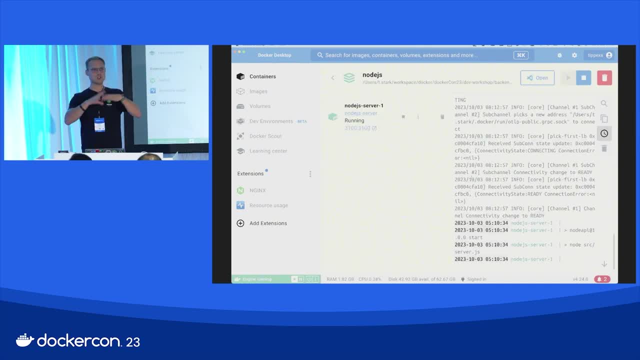 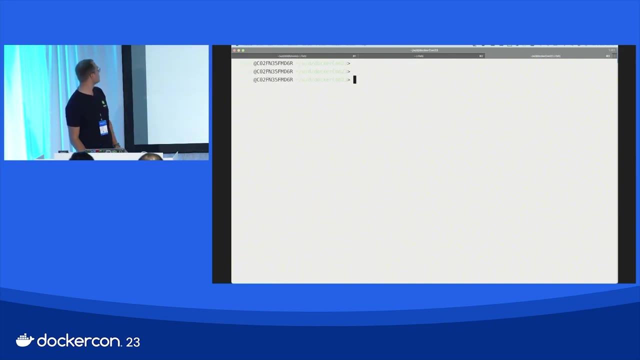 about. this is Quick question. If you have launched a container from somewhere and you would like to exec Or execute something in the container, what you always can do is Let me make this a little bit bigger. Can you see that okay? 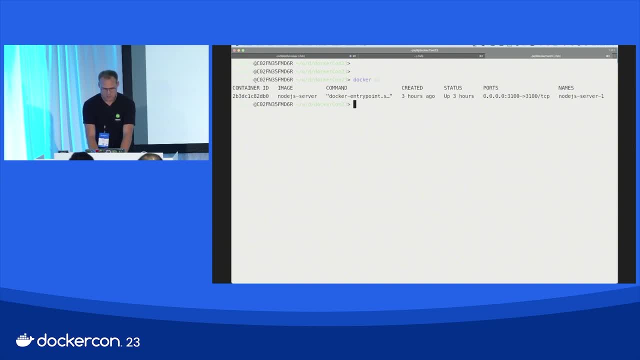 Yeah, So We can type docker ps. And now just imagine we would like to jump in the container and do something. So we can do docker exec et. And then you can use the name or the ID, but you don't have to specify the full ID and 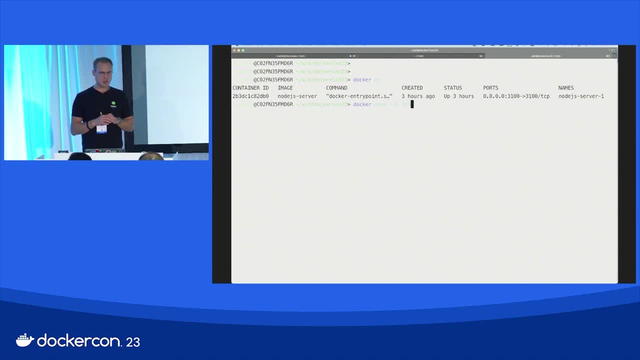 that's a neat trick I'm always happy to share. As long as the ID is unique, you don't have to type the whole ID If we have here just one container. I think To me I'm always using just three, the first three parts of the ID. 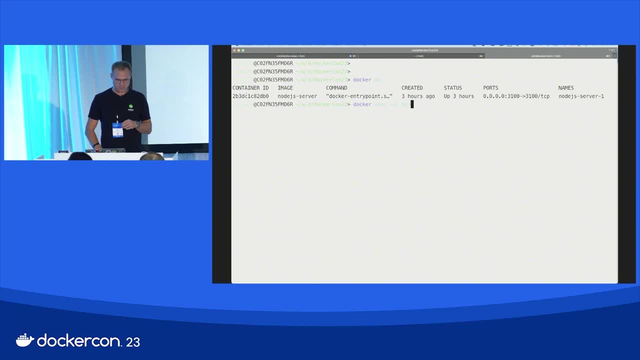 That's totally enough. I would never type 2b3dc whatever. That's not necessary, So it's a waste of time. Don't do this. So, docker exec space, dash it. 2b3 is all we need. So then, if you would like to jump in the container, we usually use bash. 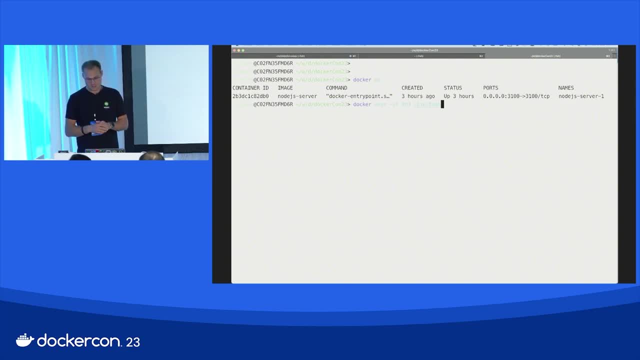 Because it's a Debian-based image, it's a Ubuntu, it's something like this. Then enter in. this time we see this little error saying: hey, that's not working. Okay, In this case, I know because this Nodejs thing is Alpine and we don't have bash in. 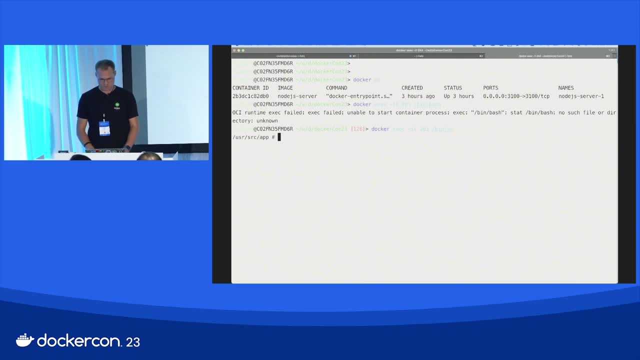 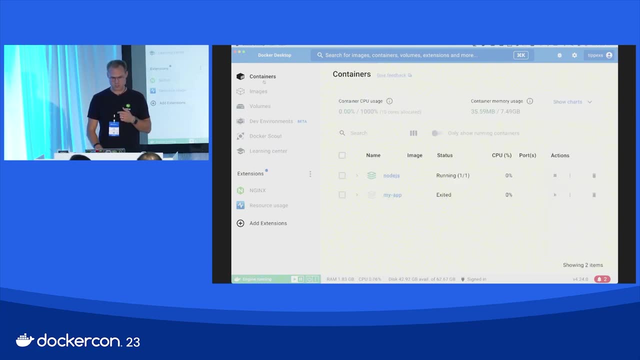 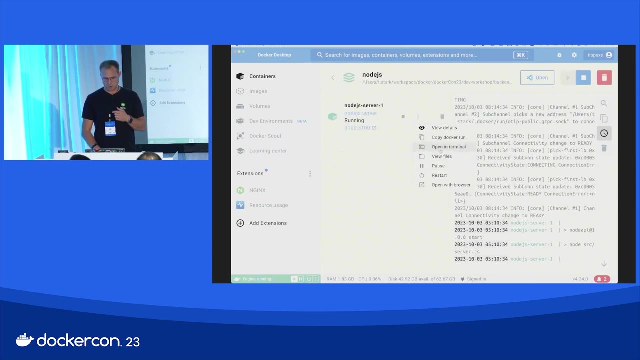 Alpine per default. So we have sh in Alpine. Oh, that works Perfect Good. So in docker desktop- and that's why I love this thing- if you click on your containers, then if you click on your Nodejs container, you can jump here, open the terminal. see. 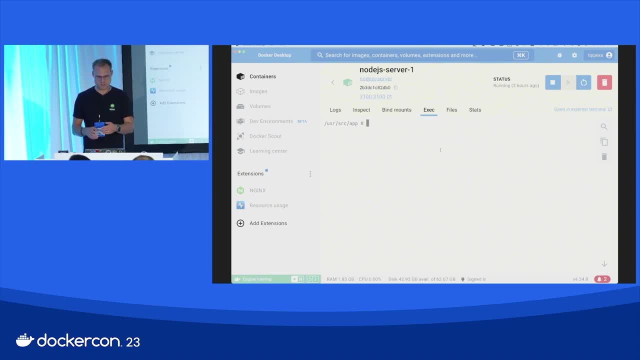 It just works. It knows it's Alpine, It knows that sh is in this case the way to go, So it's not erroring And you can do this in your like in your web UI. you have a second monitor, you just. 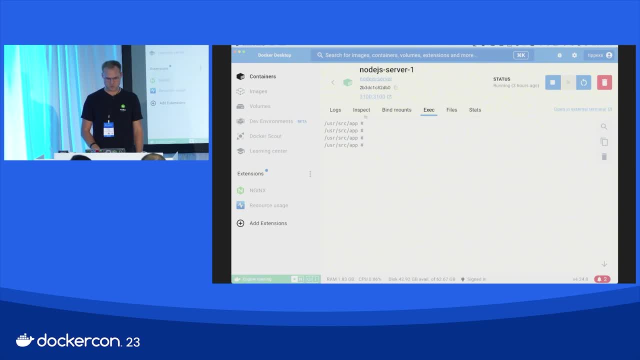 pull it over And you can navigate through your containers really really easy and can see the log output. You can see this, the inspect. Let me tell you one second about what does inspect mean, And if you're already familiar with things I'm saying, just let me know, then we can. 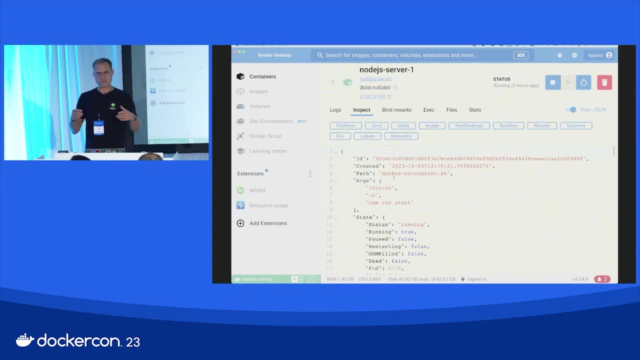 jump over it. Docker inspect is basically printing all the metadata of the container, Right? So why is that? Why is that, for example, important? It works. It will basically show you what ports are exposed If you have files mounted to the container. this is something that will be shown in the 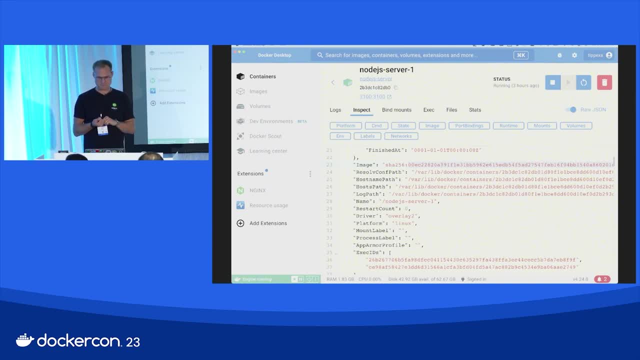 inspect mode And one thing I am most interested in when I do the inspect. we have this image, SHA-256 hash, That print. so this hash shows: okay, what is the exact version? What is the exact version of the image I'm currently using? 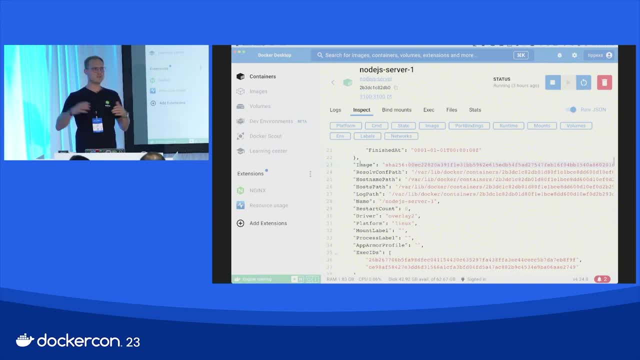 Because if you start developing with Docker a lot and you type 100 times Docker build- not always, but sometimes- you will see that a version you're pulling from a registry and you have on your development environment, like on your staging environment, for example. 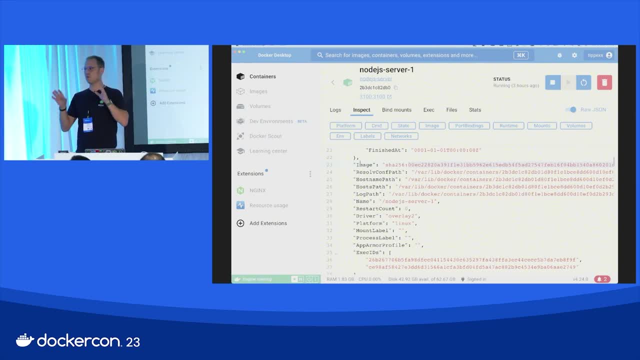 should be identical But for whatever reason you have a different behavior locally versus what's on staging, And then you can try half a day to find what are the differences, And sometimes this happens Because you have the Docker tech latest- and I will come to this during the session- absolutely. 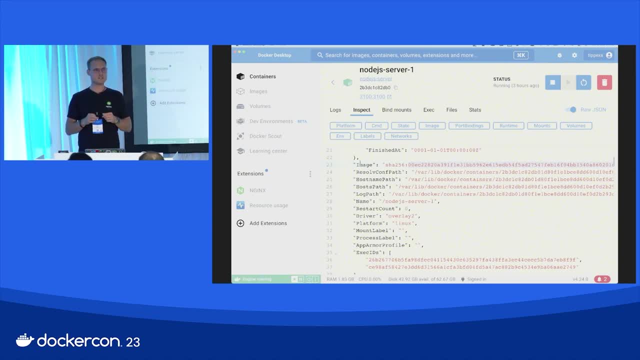 because this is for good and for bad. if you always use latest as a tech to push new images to a registry And if you have this kind of issue that the staging environment is doing something completely different from what you have locally, then it's sometimes important to check this image. 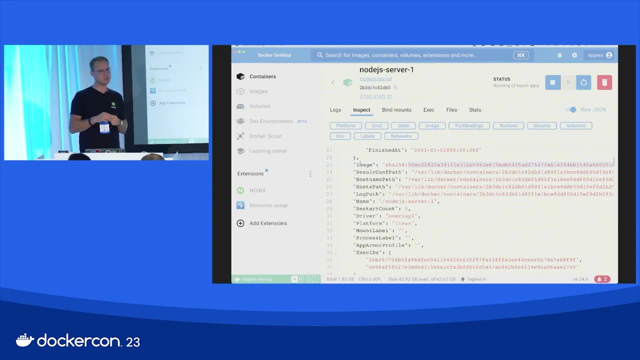 hash. You can check the hash online and you can check the hash on your local machine and if the image is totally identical, then the hash should match. If the hash is not matching, then you have local, a different image than on the staging. 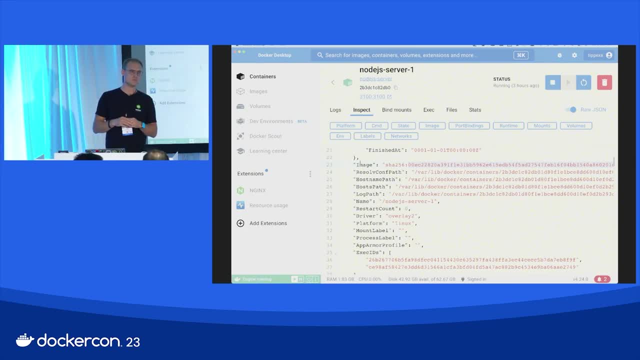 environment Right. How does that happen? That could happen, for example, if you push an image with a tech latest to a registry and then you have a tech latest on your machine and then you pull, for example, an image from: 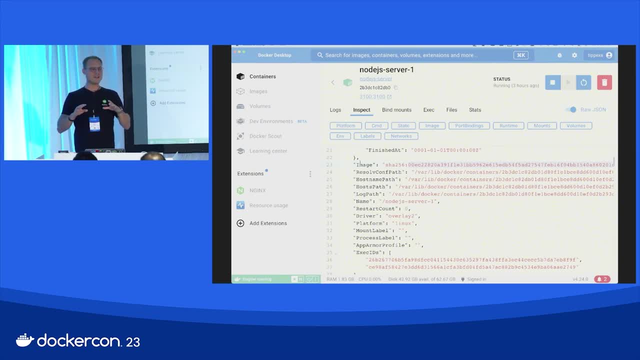 a registry And in 99% of the time it's the same thing, Right. In 99% of the cases it will override the latest image, But there are some smaller cases where this is simply not happening. So it will say already the newest version, or somebody else pushed something too latest. 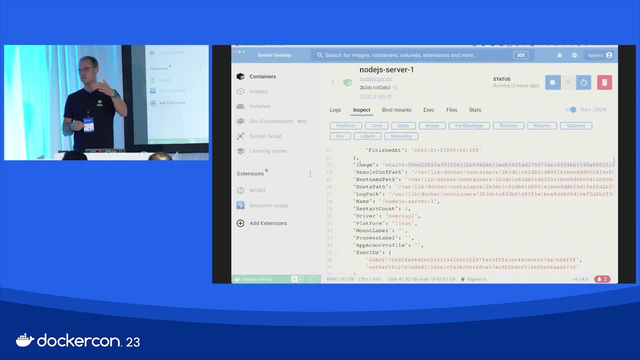 in the meantime, from another computer You pushed and somebody else pushed and you're not checking that the update was overridden. So you have not the latest image. That sometimes I mean. I came across this problem a couple of times and that is just. 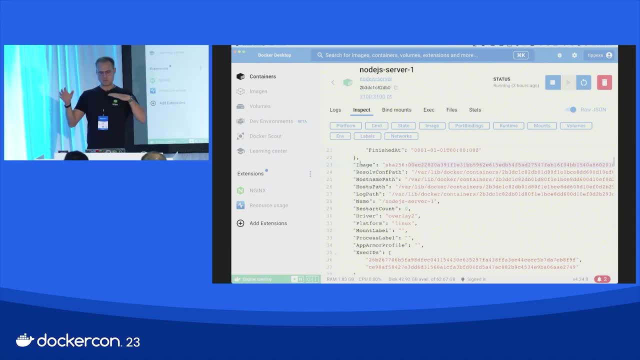 crazy. But to me, if I do some comparison between local and staging, because I want to inspect some stuff in the image, I'm always checking if the hash matches. If the hash matches, fine, Then I can inspect and can look in the container and do stuff. 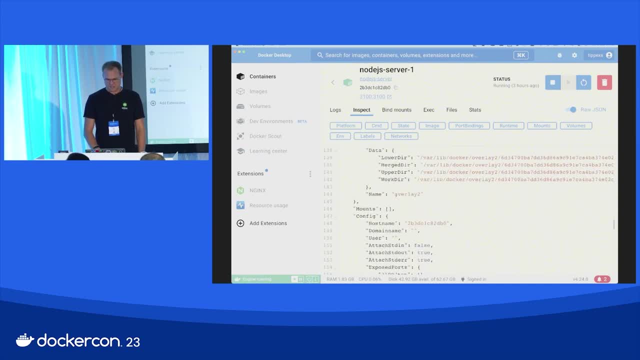 Good, So that's basically what's in the inspect thing. You will not use that really really often, But from time to time it's useful to do the inspect mode. And yeah, Another nice thing here is you can click basically on your anchor links to jump in. 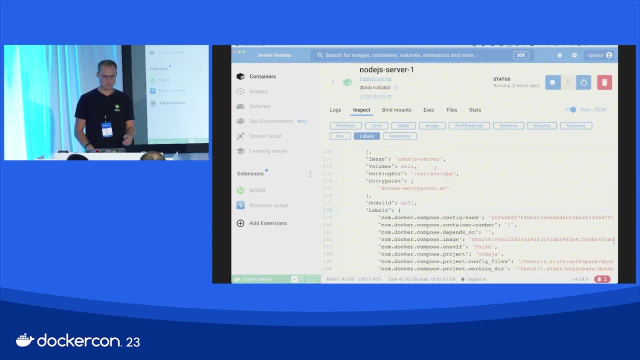 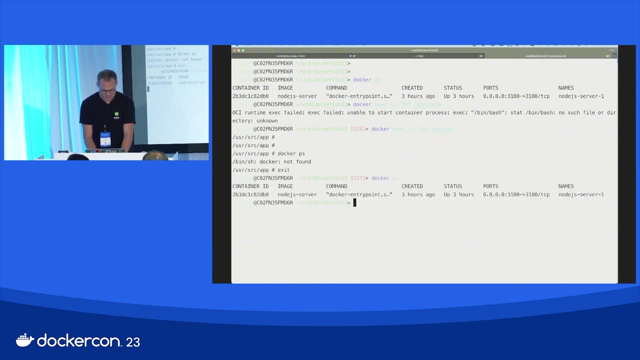 this JSON output. If you do this on the CLI, you can do the same thing by Docker inspect. Docker PS, oops, not in the container. As I said, Docker PS will print the running containers. And then let me clear that. 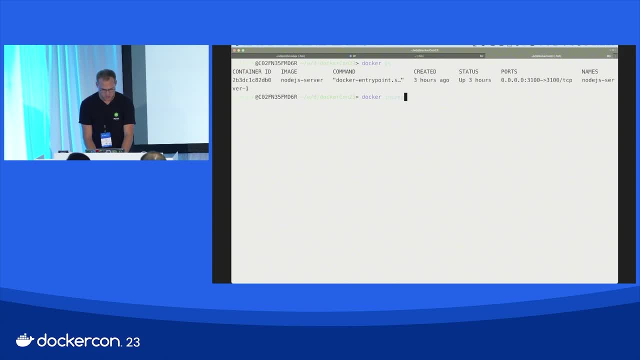 If we do Docker PS, we have an ID and then we can do Docker inspect and we get the same output. And then we can of course use JQ or grab or something to get to the point easily where we get this information. 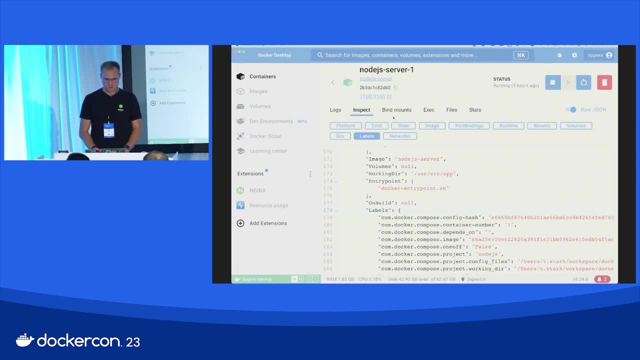 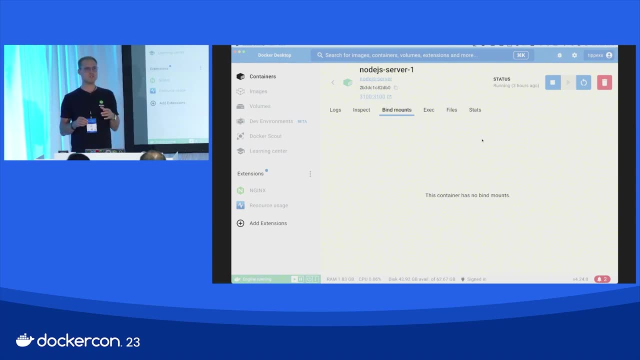 But it's just easier if you have a bunch of containers using Docker Desktop for that, All right. Bind mounts is something I will tell you in this workshop as well. What is a bind mount? It's basically mounting your local file system in a container. 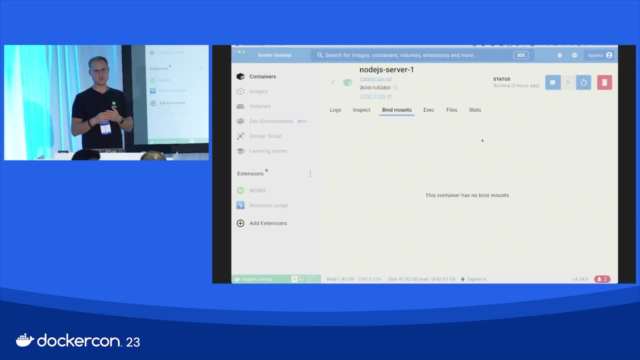 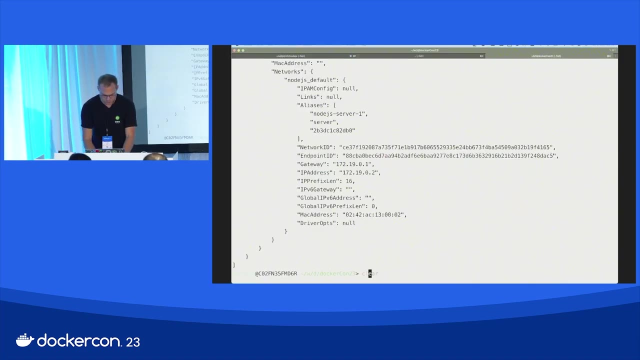 And before Docker watch, little spoiler alert, because that's something we will see as well. Before Docker watch. Okay, So I've always used bind mounts for development. So what does a bind mount do? actually, A bind mount is you have a directory on your computer. 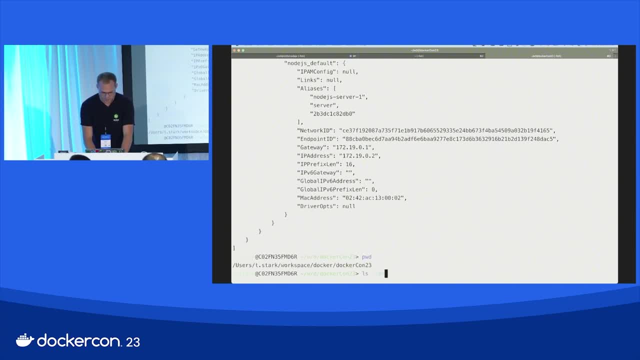 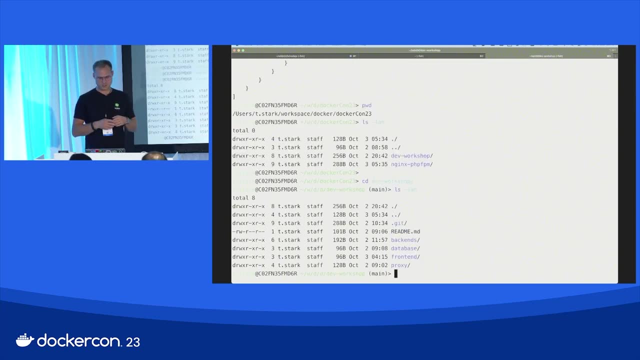 So at the moment we are here in Workspace Docker, DockerCon 23.. And then we have a dev workshop and in the dev workshop we have a bunch of directories like backends and database and frontend and proxy and all these kind of things. 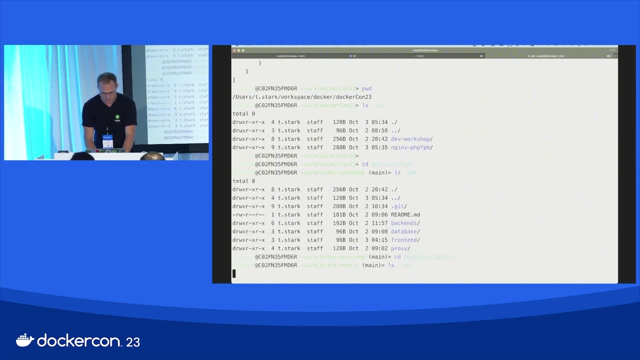 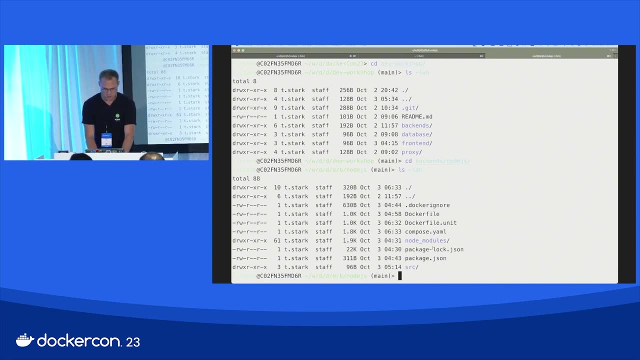 And if I want to do some backend Nodejs development, for example, What you can see here is we do have the Docker file and another one and compose and node modules and package JSON and things like that. So the bind mount is actually when I now do Docker run and I put V as you can see. that's. 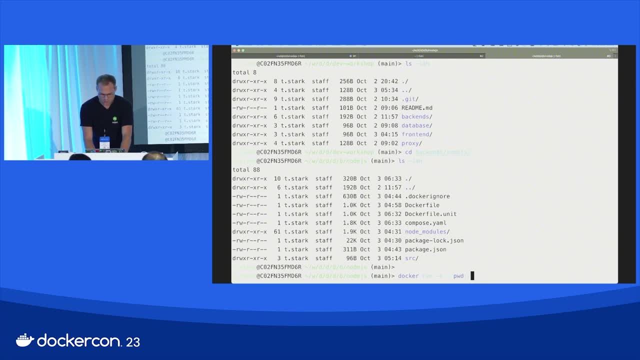 something different, but that works as well. So we use the current work directory and we mount it to, let's say, I don't know. let's put user source for what it's worth, Okay. And then we use node as an image. 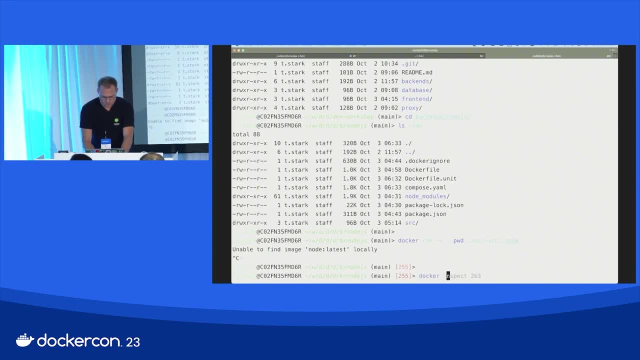 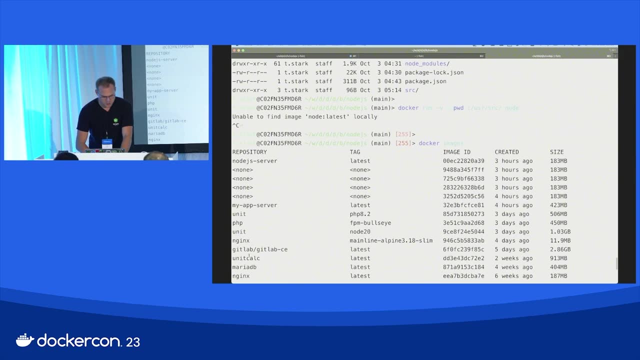 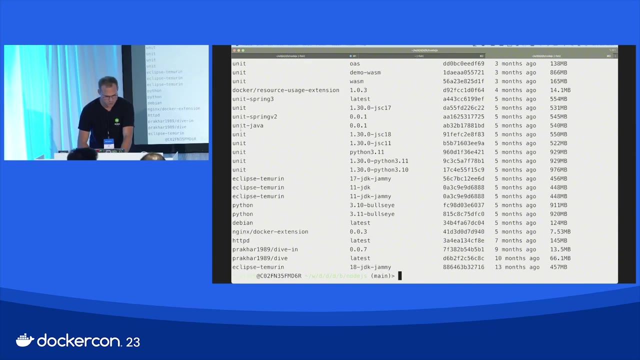 I don't want to download it because I think the network is not So. this is also something I can show you. This is now. you can see that it's node. where it's node, I can try to find it here, and there should be somewhere a Nodejs image. 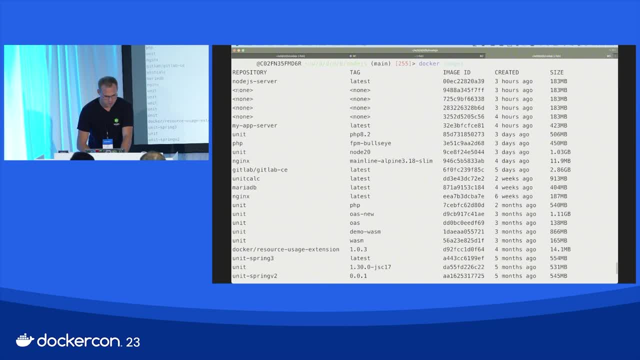 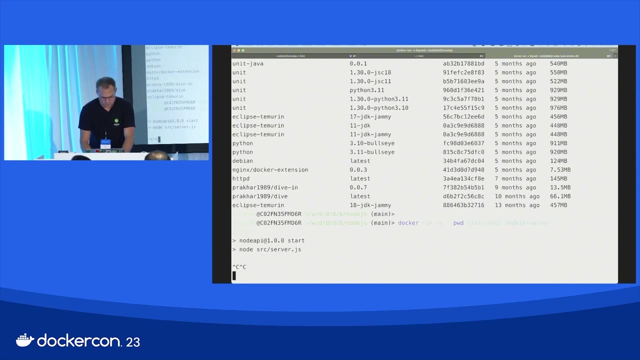 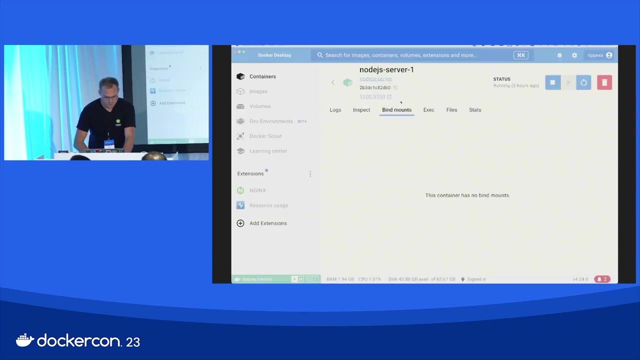 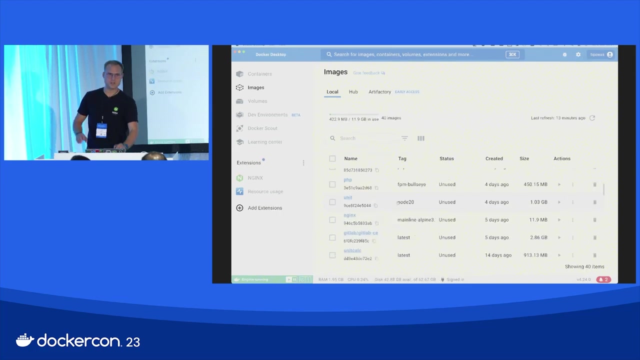 Already downloaded it. Okay, Cool Nodejs server. That's fine, Let's use that one. So Nodejs server: Yep, All right, That's great. So now another thing: You can use Docker images on your CLI- Okay. 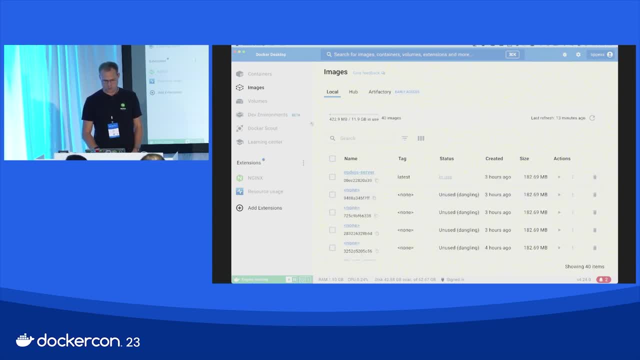 To detect where your images are, or you can basically use here the image tag to see what are the images that are currently on the system. Is it 100% clear what the image is? The Docker image? Yeah, That's fine, Okay. 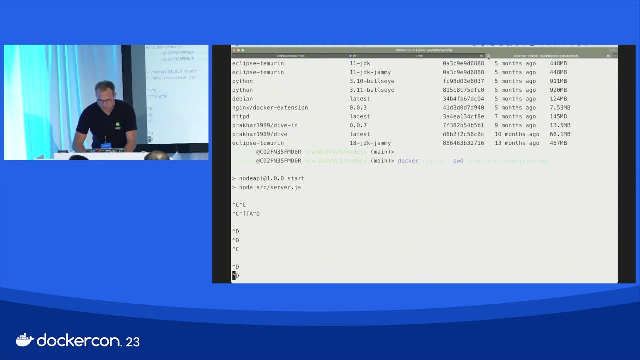 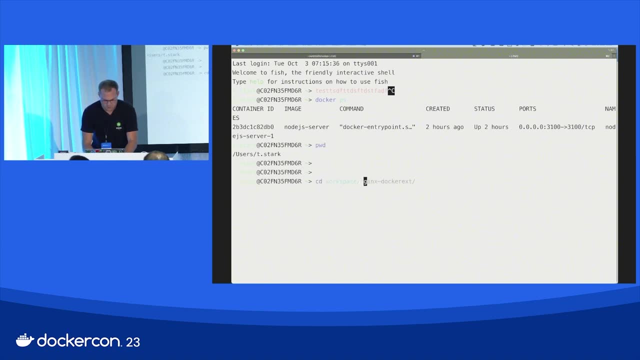 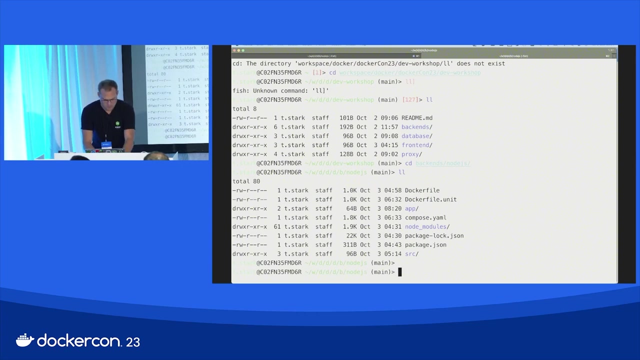 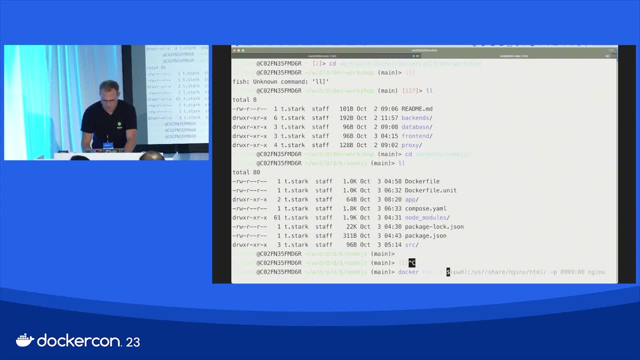 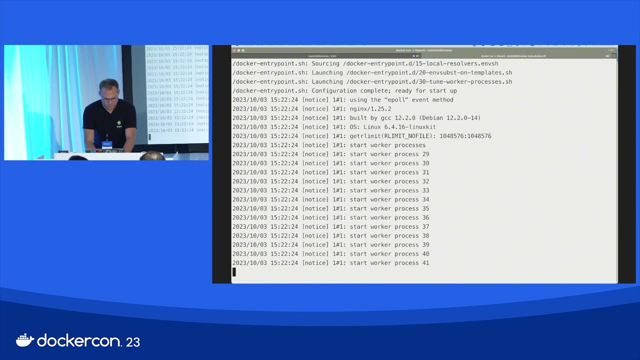 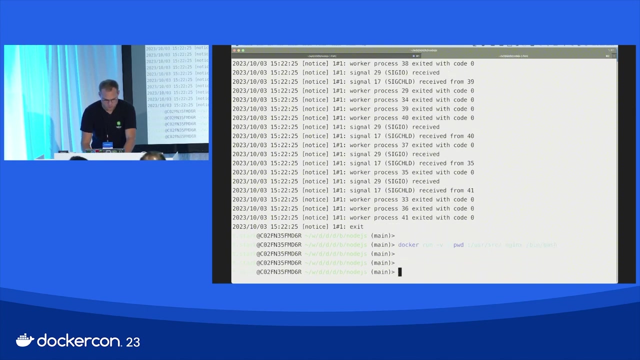 We can do this Docker runv. Let's use nginx container. That's also fine, User, Because it's not. we are not doing actually anything with it right now. We are basically just trying. Okay, Then we override the entry point. 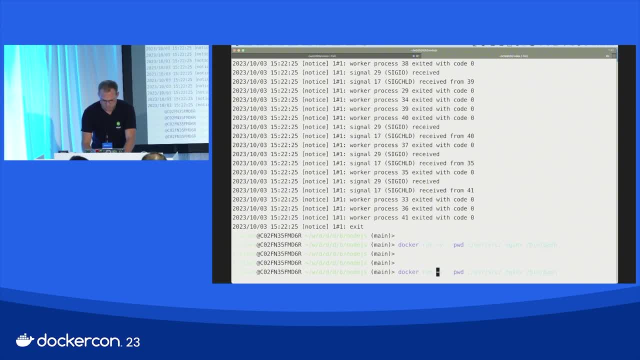 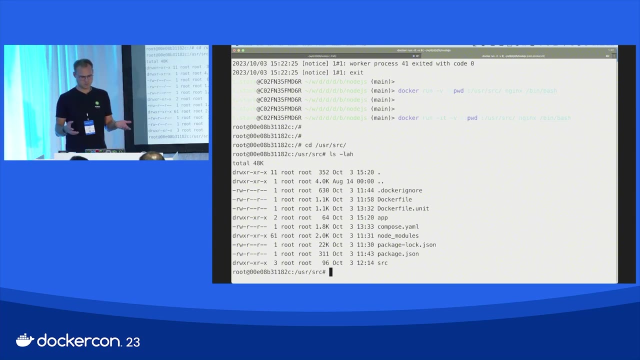 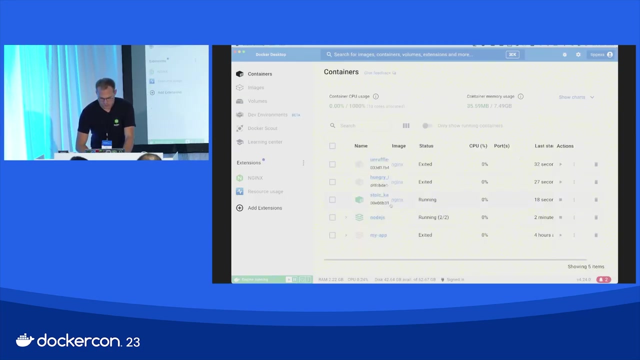 All right, So now we should see the user. Okay, So we see all the data in here, like node modules, package, JSON source. So when we do now, when we look in the in our Docker desktop and click on our image, 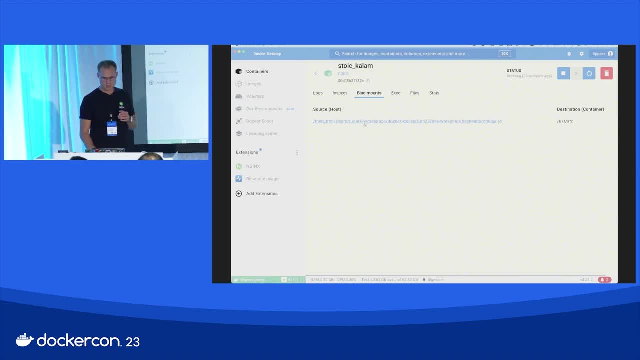 here in bind mounts we can see, okay, we have mounted this directory to use a source in the container. It's like literally like a mountain hard drive on a server, Okay, And we have some problems with it And this is something I will tell you later when we look for the new Docker compose watch. 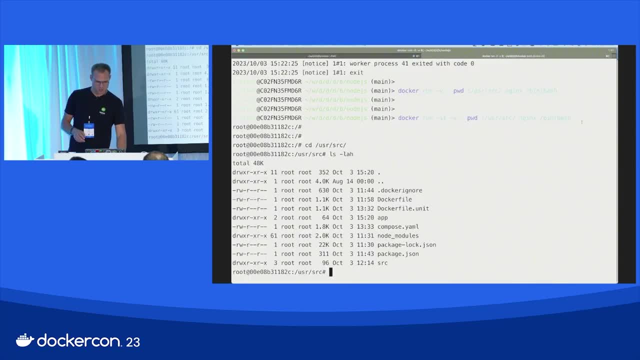 features, Because now anything we do inside of the container with the files we have just mounted in it will also represent it to the host automatically. There's not a copy, It's like literally a mount of your files in the container. Sometimes you need this, but it can also be very dangerous. 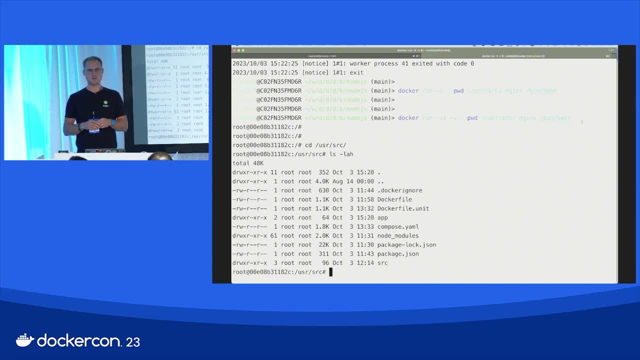 And I I shot myself in the foot a million times with this, Not kidding. So especially when you do something in a hurry and you would like to test something and you mount something too quick in the container and in the container you delete something. 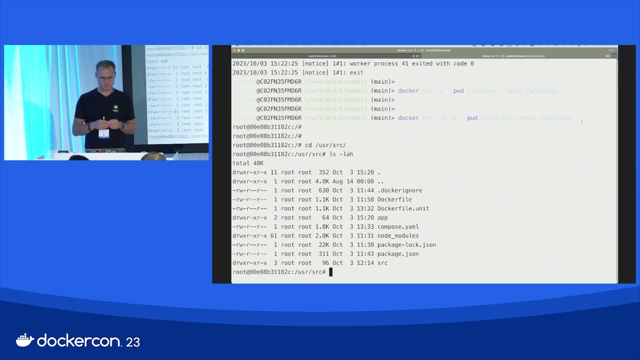 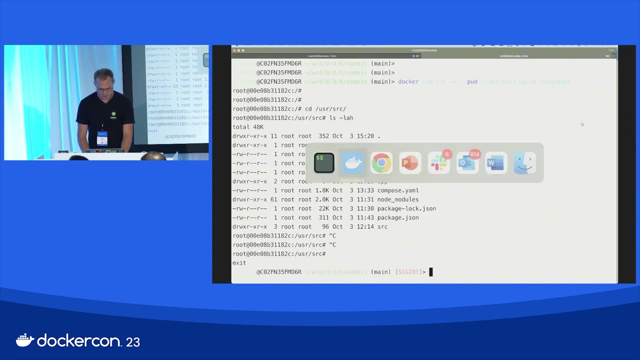 and you go: oh no, it's gone. Oops, Not good. So all right, Perfect. So this is a bind mount. This is this is what we, what we can inspect here as well. XSEC is what I've done a million times right now. 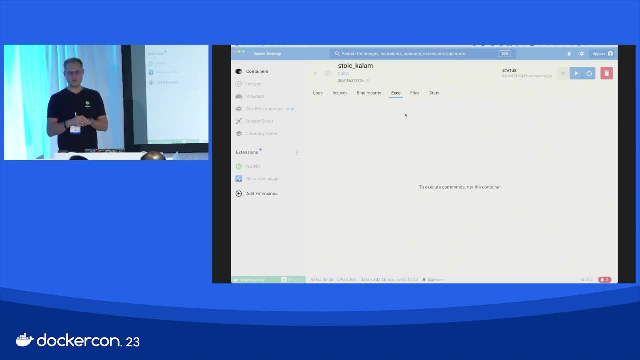 Just doing this Docker XSEC thing. Why is that useful, Especially when it comes to development of web applications or applications in general. There is a a process, or I have a process, of developing Docker images or container images. You can- I mean you- start from a base image, as always from some base image. 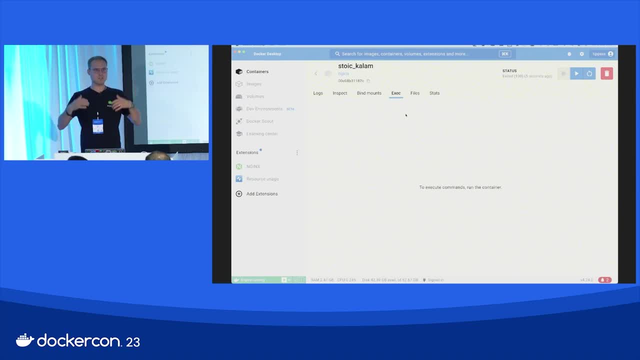 So, and then you have to do some things in your Docker file, Like Update, if you have a Debian-based image, and then you install things, Perfect, And then you do X Y, Z to make it work. Okay, Absolutely perfect. 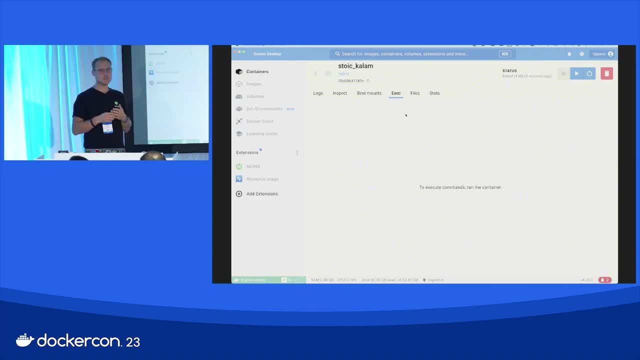 But how do you come to this point to know what I have to do? basically, in the Docker file- And I saw a couple of attempts from other people- They're writing a Docker file. Then they say: Docker build Failed. Okay, Change the Docker file. 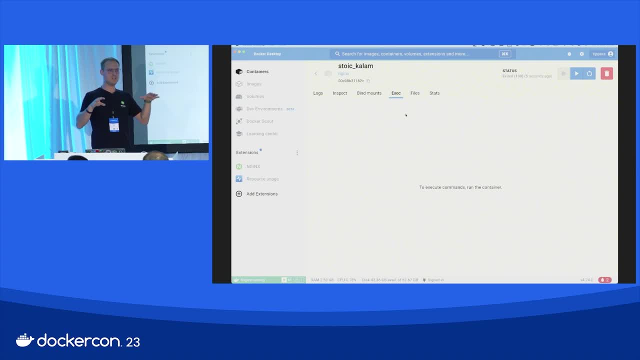 Try Docker build again, It fails again. This works Technically this works, but it is inefficient as hell. I mean you try Docker build a million times and if you install like 400 megabyte of dependencies because you build a container, that that is for your builds, your software, it's not your. 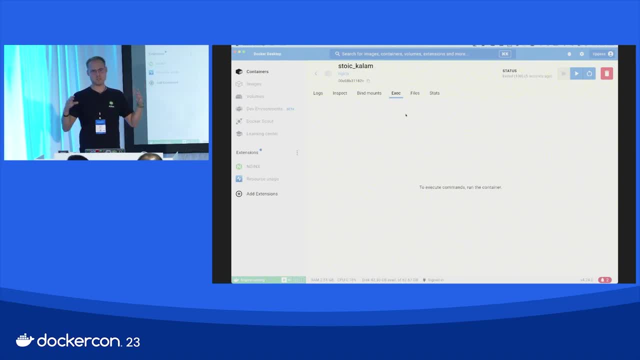 production container, but you need all the build dependencies in this container. This can be huge very, very soon. So what I do when I run, when I develop Docker container images, I look for the base image I'm going to use. Either it's Nodejs or Alpine or Ubuntu or UNIT or whatever image you want to use, or 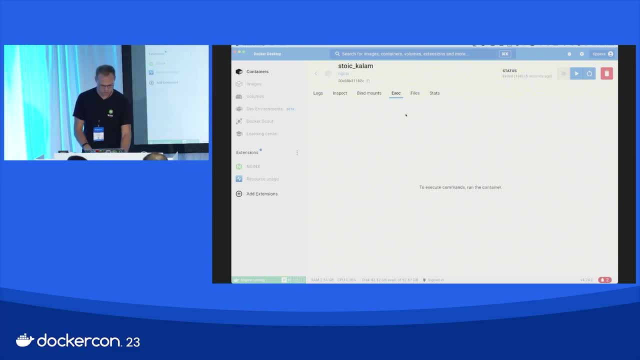 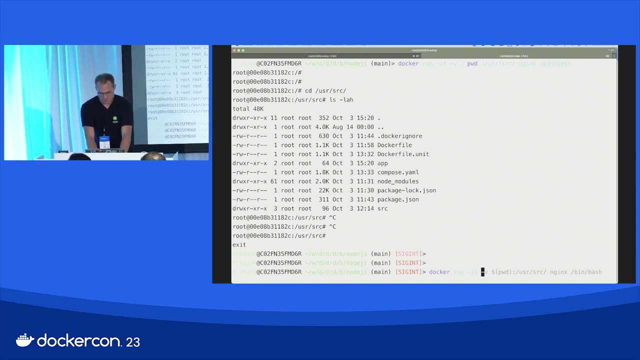 your own base images. Then you start this image in a way, for example, Docker run dash IT for interactive TTY. So it means I can actually type something in. Then you can use a bind mount if you would like to test something with your data. 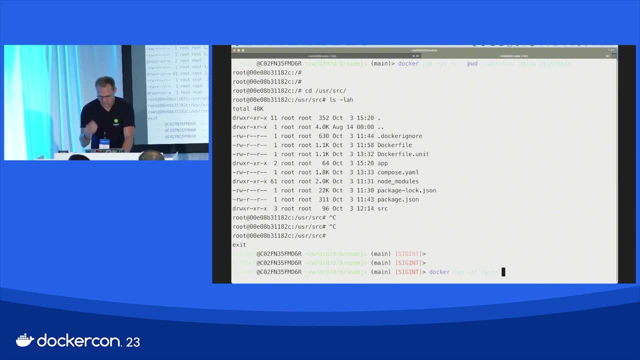 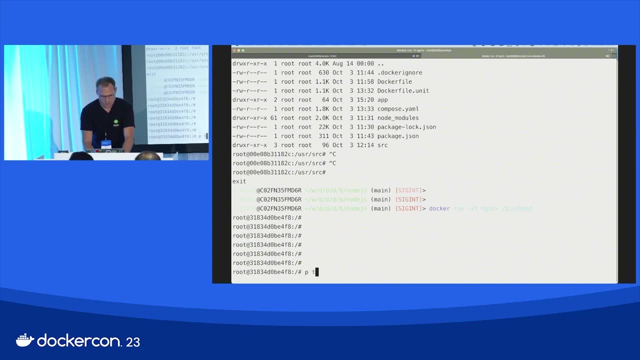 And then you type the image- In this case, let's use Nginx as a base image for what's worse- And then, at the end, bin bash. So now you see we are here. Good, And now, when I type update, I will update my repository catalog. 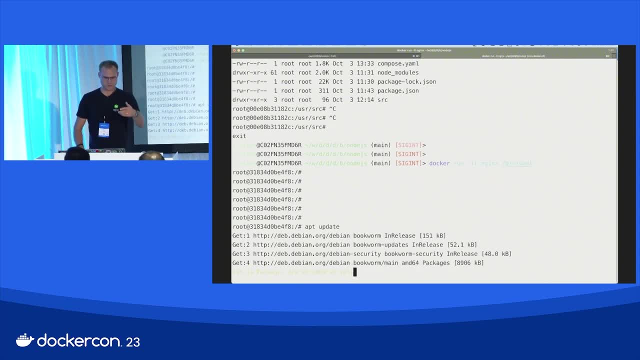 Good, So let's give it a while while I'm talking. So what happened is I have this now on one screen, I have my text editor IDE on the other screen, And what I'm basically doing is I'm bind, mounting or create a copy. 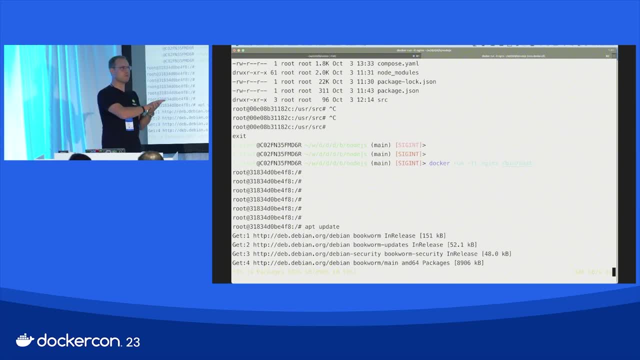 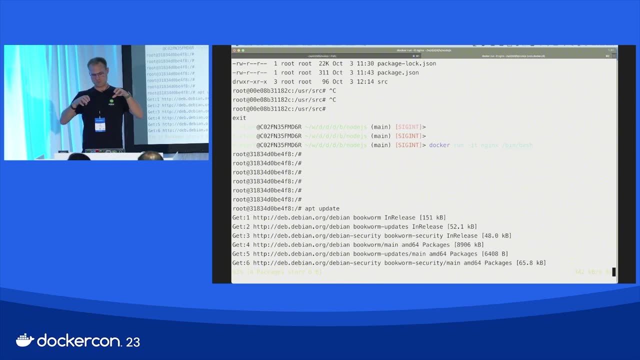 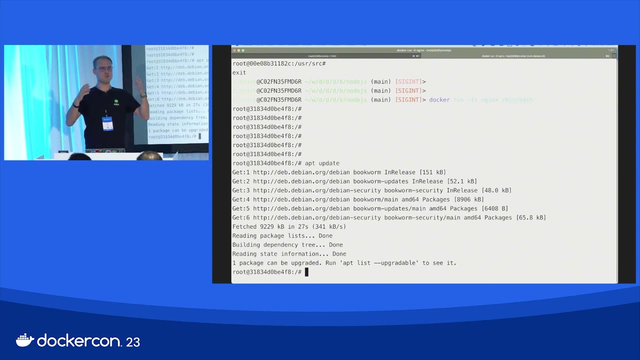 Any of my data in a zip archive or something, And then I'm bind mounting the data in this interactive container And what I'm actually doing next is like a live development of this Docker image. So I know what I want to do, Like, for example, if I need JQ to parse some JSON data. 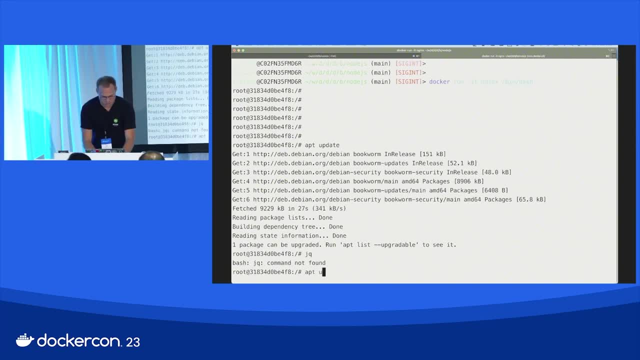 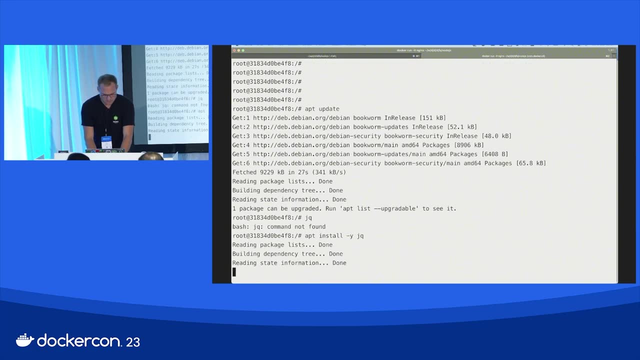 And I'm pretty sure JQ is not part of the default Nginx image. It's not, So I have to install it. So I do update, Perfect, And then I'm doing this and install JQ. And there's another thing. 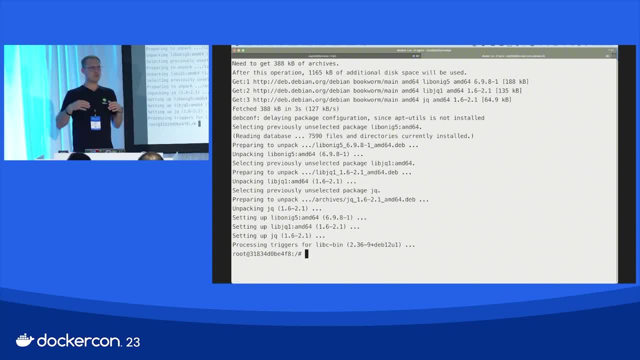 This little dash Y, If I do this live development process of a Docker image, make sure any time you're typing something in your active shell that you do not need to type something extra than the command you're trying to execute. Otherwise your build state will just fail. 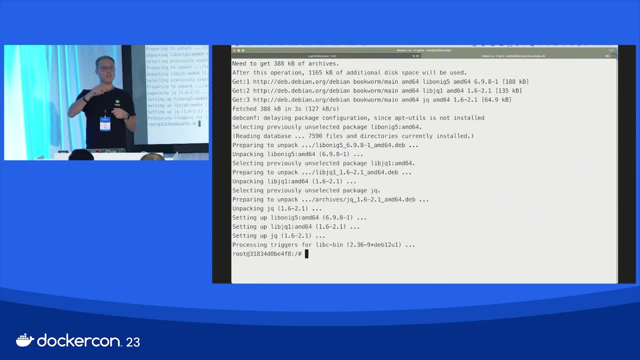 Right. So if you just type apt, install JQ, it will wait for this little OK click that you're fine by to install the library and that it consumes I don't know like five megabyte or something of your disk space, And then the build step will fail. 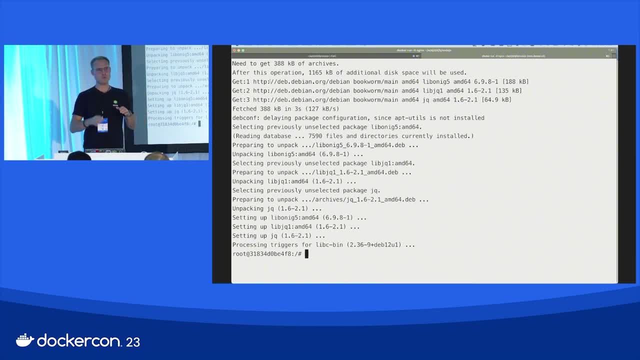 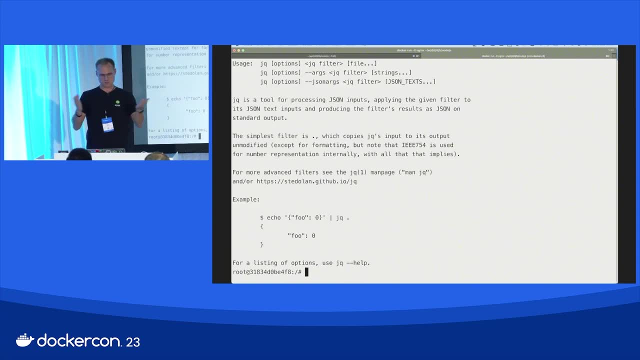 So make sure you type dash Y so it will just run smoothly without asking for anything else. Good, So now it's JQ. I can use it, actually Perfect, And I've installed it in the container. So what I do next is I can do some tests in my container and then I jump in my IDE and 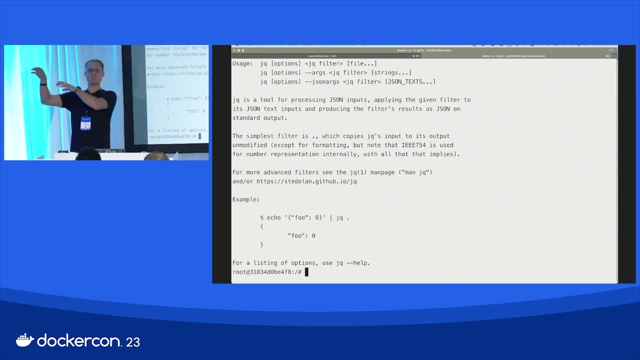 type in my Docker file: Run, Update, End, End Up, Install, Dash Y, JQ. So then I go back into my interactive container and do all the stuff I have to do, And each step I'm doing live in my container. I'm like copying over into my Docker image. 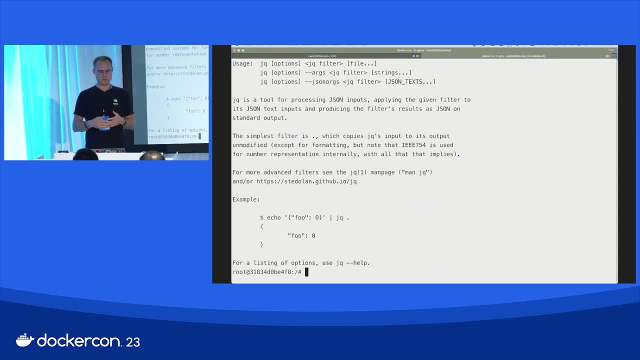 in this Docker file basically. So this helps me because I can interactively do the development of my Docker image in this interactive terminal and can test things out and can try them and it's like navigating in a normal shell And as soon as I have a solution in my container image that works fine, I just copy what I have. 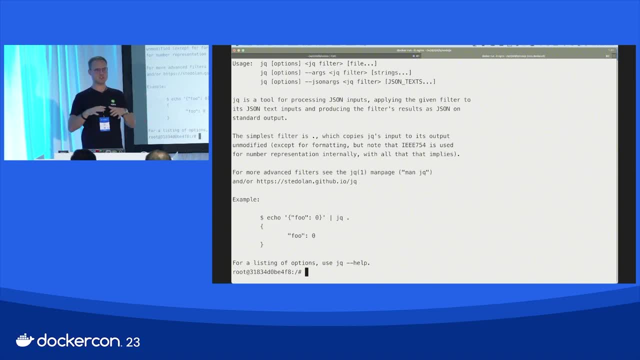 into the Docker file And at the very end I can just run Docker build. Sometimes it works on the first try. Sometimes I forgot to add some non-blocking things, like this dash Y, for example, But most of the time this is a lot more efficient than just doing the Docker file and build it. 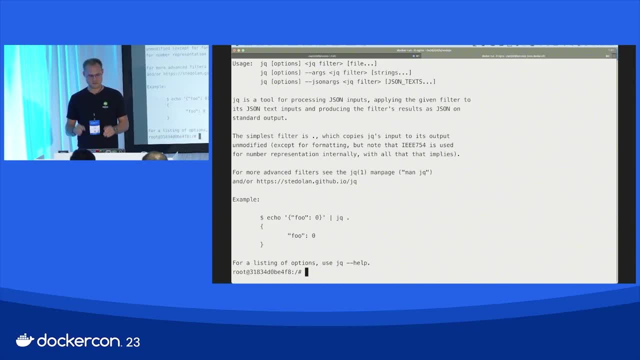 all the time. All right, This is my pro tip for building and creating, And most of this is like: how does that relate to XSEC? That is XSEC because, for example, if you would like to jump in a container that runs, 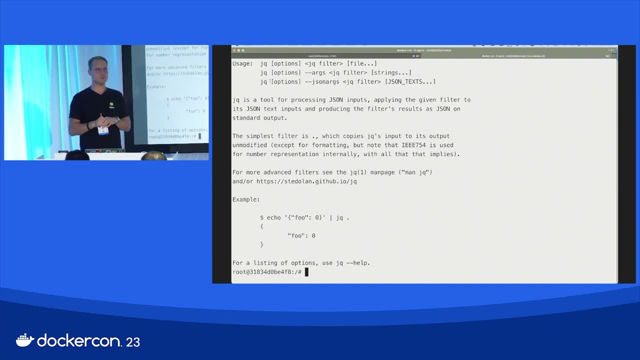 from multiple terminals, then you can use XSEC to directly jump into this one. So you can start it up, let it sit somewhere. And if you do not start it with Docker, run dash, IT, bin, bash, then you have to do the XSEC thing. 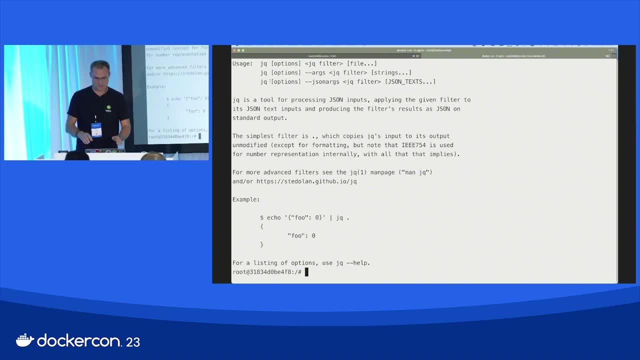 To jump directly in the container. So it's a reason why I'm saying it is because the Docker XSEC command for me is one of the most important things, Because if sometimes something is not working as expected from outside the container, I would like to go in the container to see what the heck is going on. 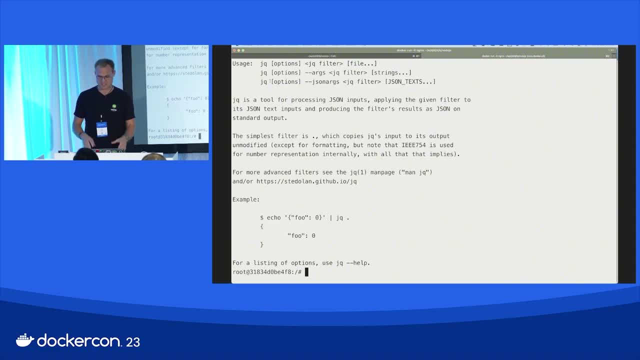 And that's when I use Docker XSEC. So it sounds always like a special thing Because we all know Docker run And Docker stop And whatever. But Docker XSEC to me is one of the most interesting things, just to see what's going on inside. 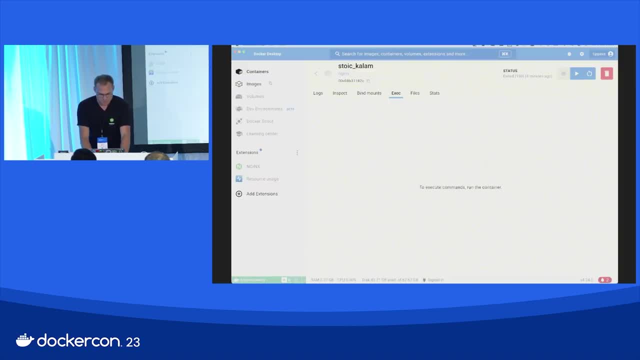 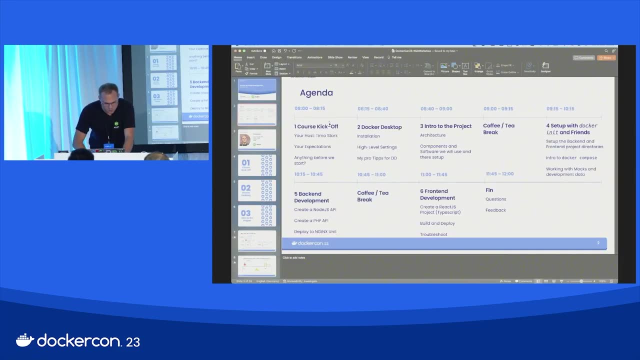 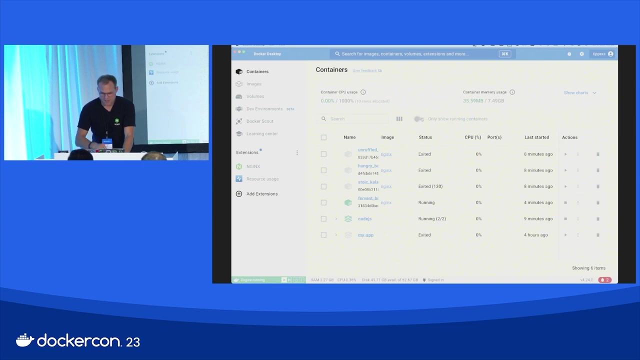 the container: Great. So this is what we can see here in the containers. Let me just see. if I'm not, yeah, we have 10 minutes for Docker desktop left, So that's Docker XSEC. And then it's like: yeah, you can just show my running containers. 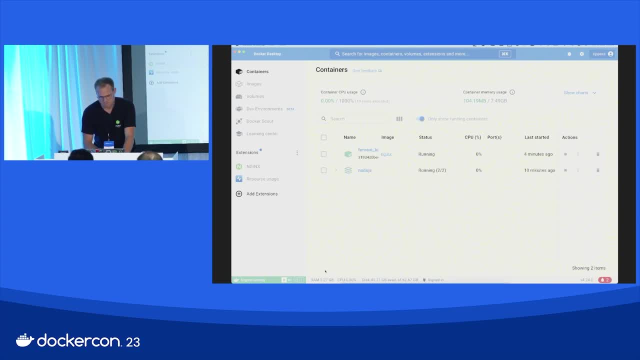 Because if they are stopped, fine, Just running containers. also, good Images is something we already saw. That's all the images you have on your system. And another thing that is like a pro tip when it comes to images: the image is mostly stored. 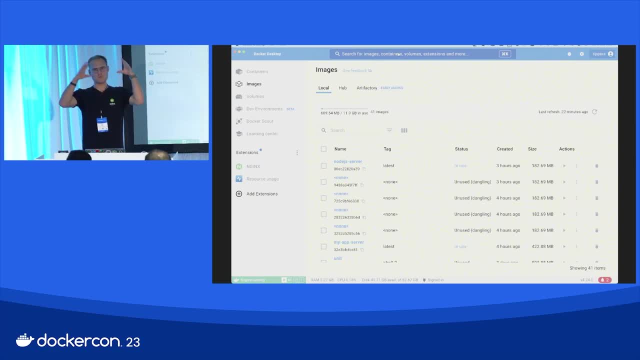 on Docker Hub So you can download them by Docker pool image name. It's not already present, Then it will download it. If you type Docker run And the image is not present, You know this pulling from Docker Hub thing, Perfect. 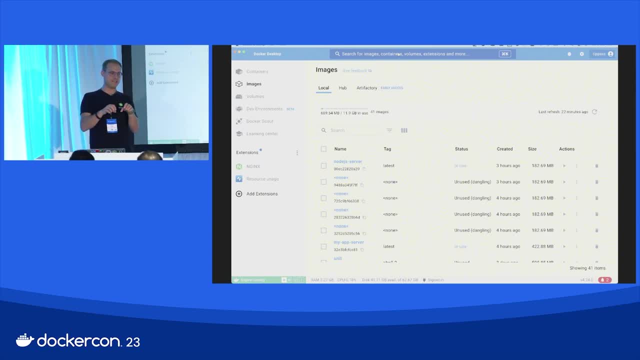 But can I see with show of hands, how many times have you at least typed this Docker run command three times because of this image name at the very end is like somehow wrong. and it was not able to find the image on Docker Hub. Like I want to run GitLab. 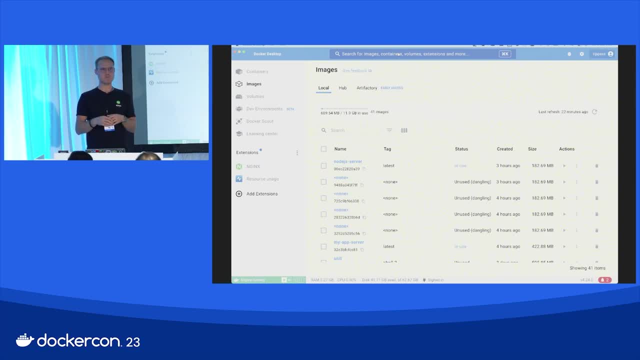 GitLab Enter. Okay, It wasn't fine. GitLab dash CE. GitLab CE. Then it has special text: No latest. So then there's a Docker CLI command And then there's a Docker XSEC, So there's a command that is Docker search. 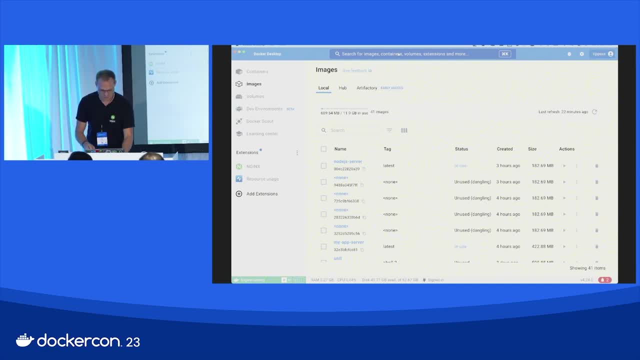 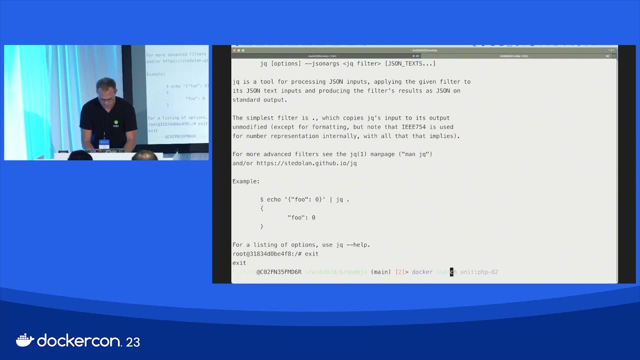 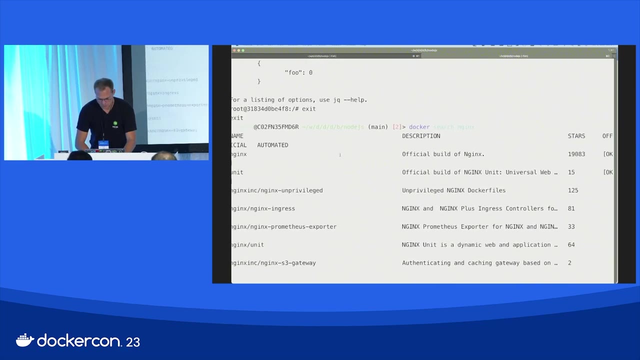 You can search from the CLI, the Docker Hub, and say Docker search and then type an image name Docker. Let's go out of this thing. Then we type Docker search, Docker search, NGINX, And it will show: okay, what are the NGINX containers? 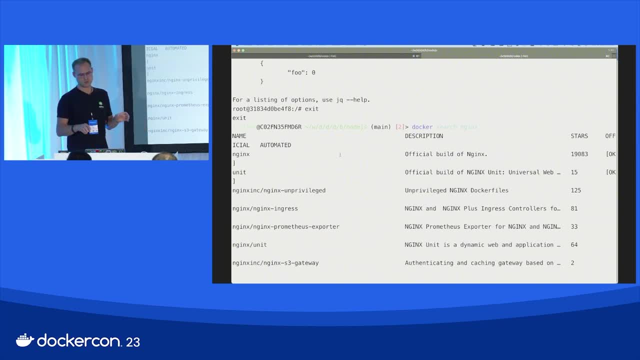 So, but one thing that I always miss when I do Docker search: it's not showing all the text. It's literally showing the image name. That's fine, But this is in some cases, for example, when I look for our unit container we will use 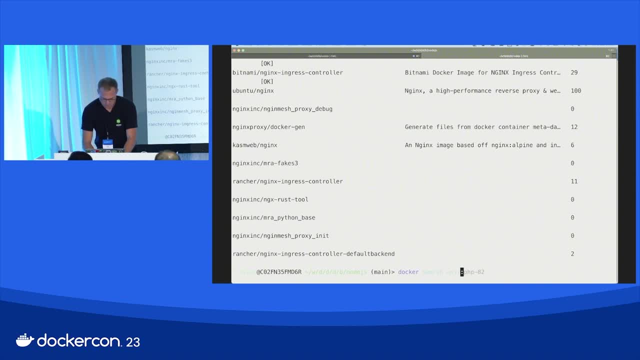 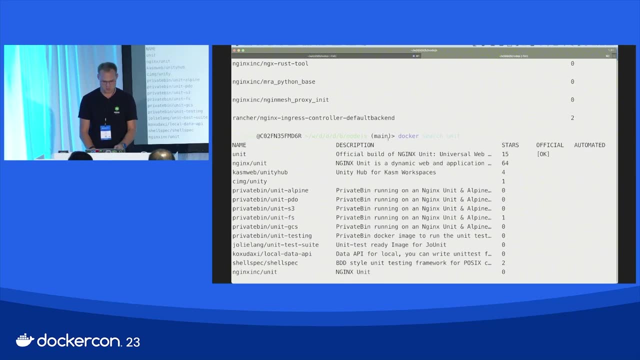 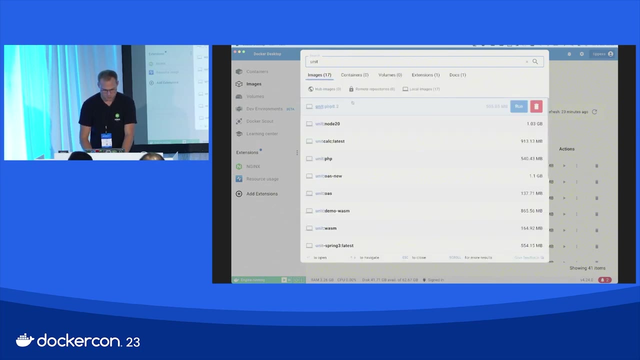 later can't type unit, it will show me that there is something that is called NGINX unit, but it's not saying okay, what are the text I can use. So I can go to Docker Hub, or I can use command K here and type unit. 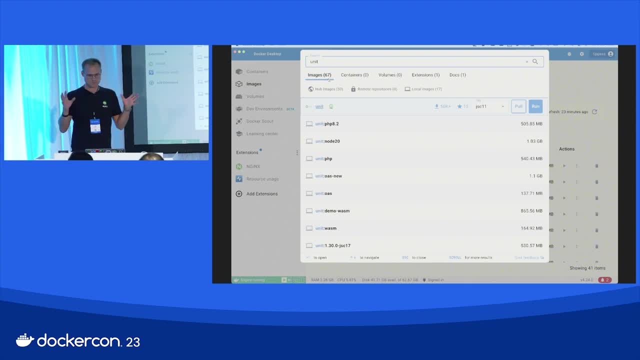 And then Docker desktop will Okay, So I can open this magic search, and I really like this because of a couple of reasons. First, it will show me here: This is the official image, Perfect, And here it has this little tech drop down. 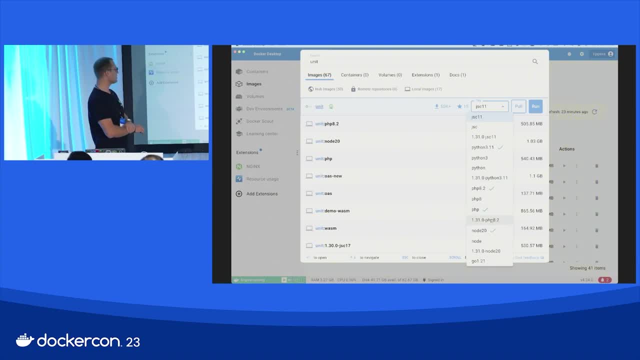 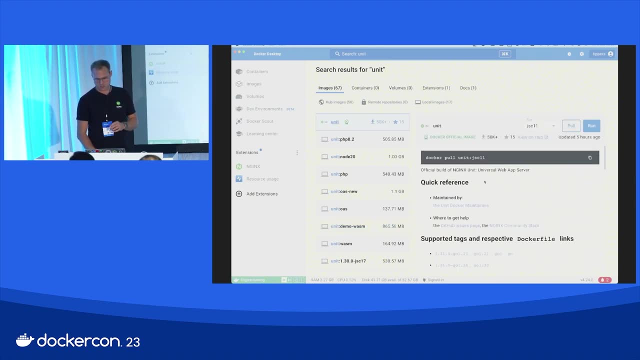 So I can see what are like the current text and kind of select one And then I can run it, I can pull it, I can see here The documentation about an image, And this is especially when we come to develop a container image or, if you want, for example. 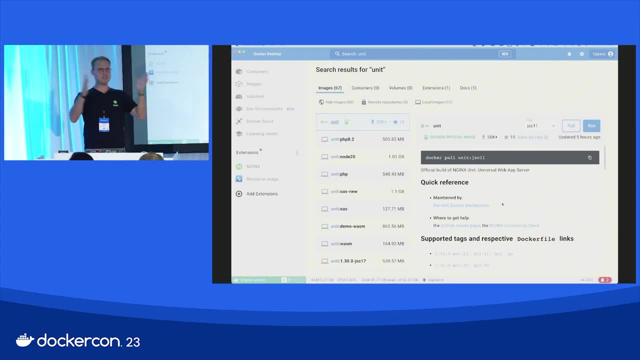 this little example we have that you would like to split your images or your services into different things and you would like to containerize your application with a compose file. the Docker desktop search for images on Hub and all the documentation is something I use, since I'm using Docker desktop. 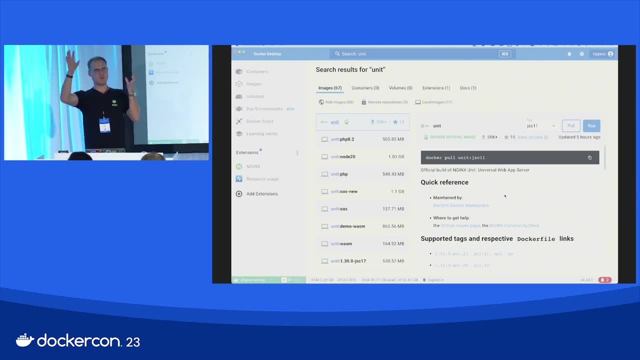 I'm using Docker desktop More often than going to Docker Hub on the website, Right, So type the image name, control K or use the search bar here. Then you can click on the image. Here is the tag. Then choose one and then you can see here the documentation. 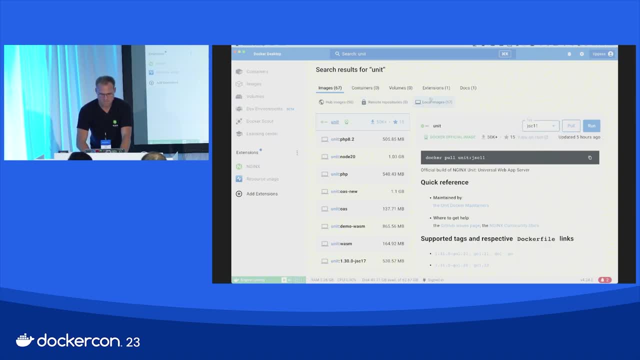 You can pull a given tag. You can run it, That is. that's just easier than go to the Docker Hub itself. Okay, There is a search bar here Right on top. You can click in the search bar or you can use the command K key or, I think, on Windows. 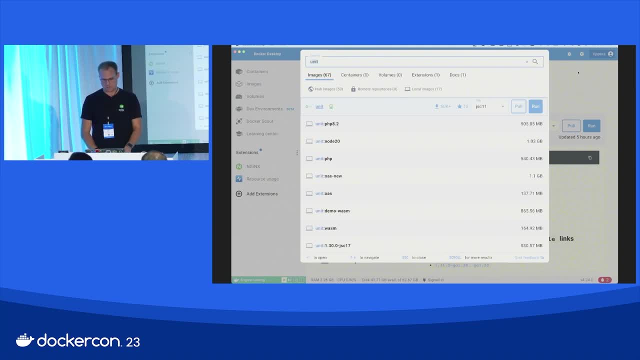 it's control key, control K to jump in the search bar Right. So let's make an example. We would like to use MariaDB as a database. We can search it, You can click on it And it will pull up the documentation. 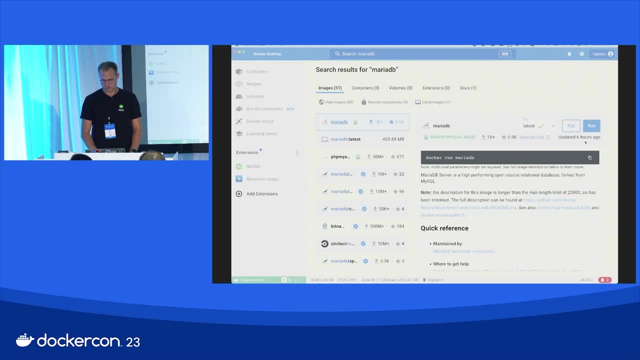 Okay, Cool, And then you can copy the. you can search for 11.1.. It will automatically change here the command. and if you, I mean you can click Docker pull. but if you would like to issue this on a development machine, that's not your local machine, just. 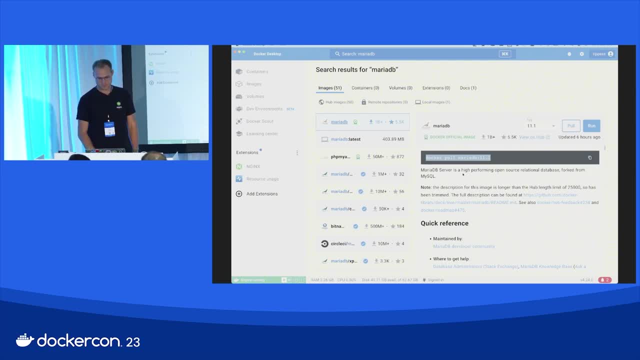 copy that here and dump it in the terminal and it will work. So to me this is a lot more efficient than just going to Docker Hub and do this like in a web browser. Okay, So I would like to leave my Docker desktop for searching images and doing like to find. 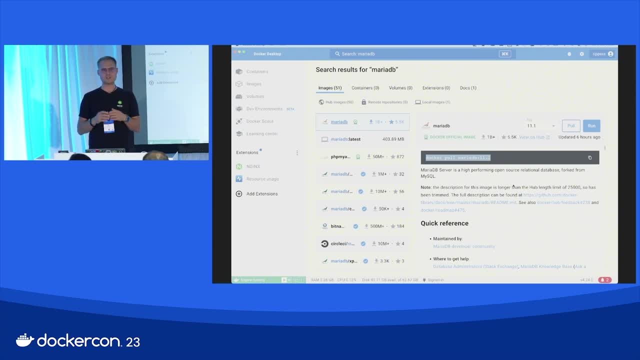 the images I would like to use for my Docker Compose file. Is Docker Compose clear to anybody- what that is, for what it can be used, or is it for any? is there anybody here that says Docker Compose is new? Never heard about it. 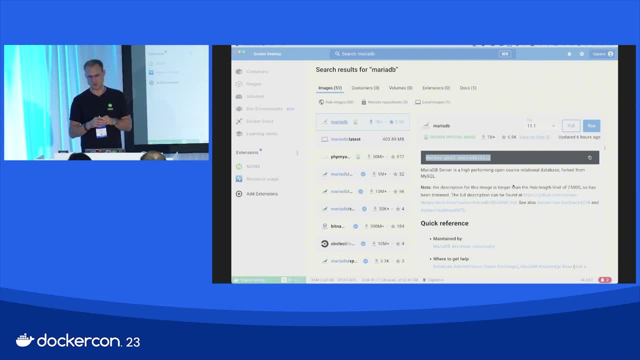 Okay, So one sentence about Docker Compose, then, and then we move on to the next thing. Docker Compose is basically a description, Okay, Of a stack of different containers and how they interact with each other. So, for example, if you run a container, we're using Docker run- you have always the problem. 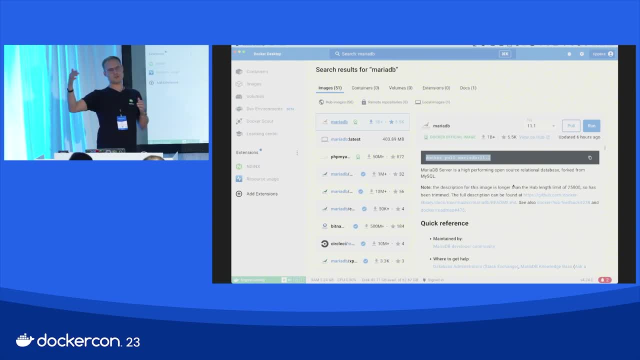 how do you document basically for another person on another machine, what ports you want to expose, What environment variables do you want to set? What bind modes do you need, What kind of maybe extra entry point at the end? this bash bin, bash at the end is the entry. 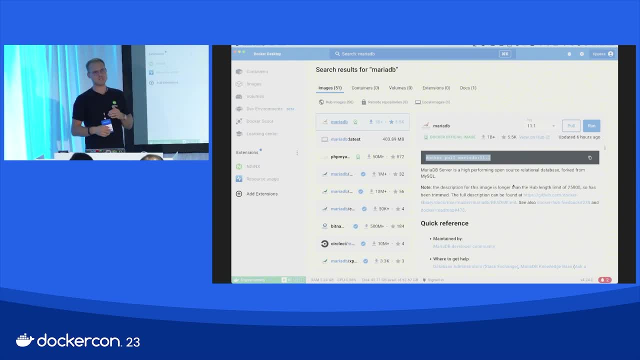 point. Okay, So you would like to document this. even for a single container, I always advise using using Docker desktop, and you will use Docker desktop here, of course. we will use this and I can show you how that works, because it will. it will describe the 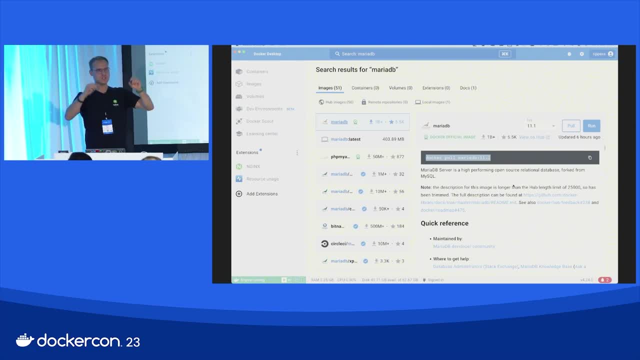 whole stack. It will describe how the container image is. What are the environment variables, What are the ports you want, you would like to expose. So it's, it's a, and if you do this for multiple containers, you can use Compose to start up. 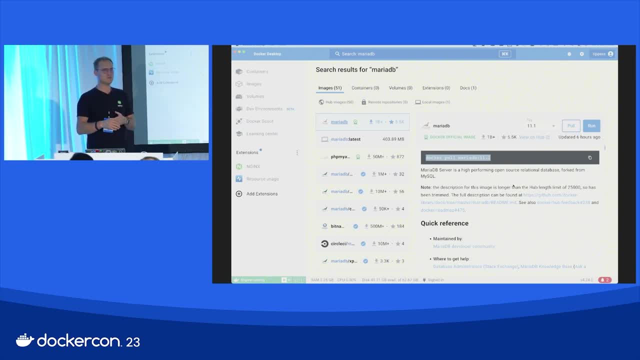 multiple containers. Good example, You wonder. and that's what we do here today. So you're definitely in the right course. We will use a database together with PHP, for example. right? So you would like to spin up the database and then you would like to administrate your. 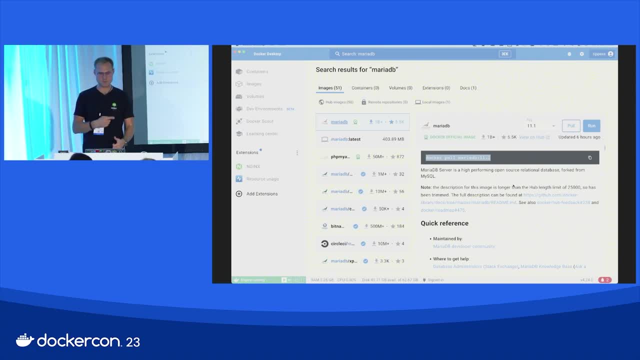 database with PHP Madman. So what you can do, you can spin up Maria DB, you can spin up a database and you can spin up PHP, my admin, to administrate the database just by simply use a Docker compose file. This is something we will do. 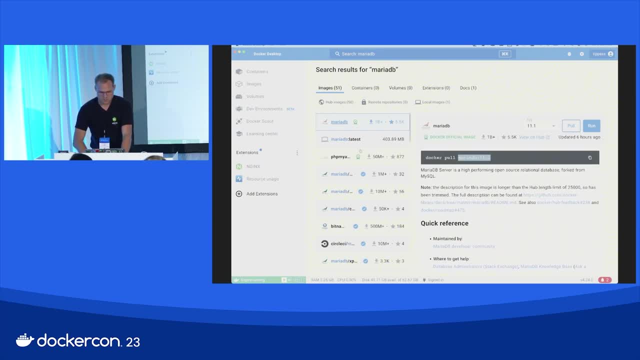 Great. So that's what I'm saying. to get image names and stuff is is important. So Docker hub is good and Docker desktop gives you a very neat interface to search images on Docker hub. Yes, Yes, Yes, Yes, Yes, Yes. 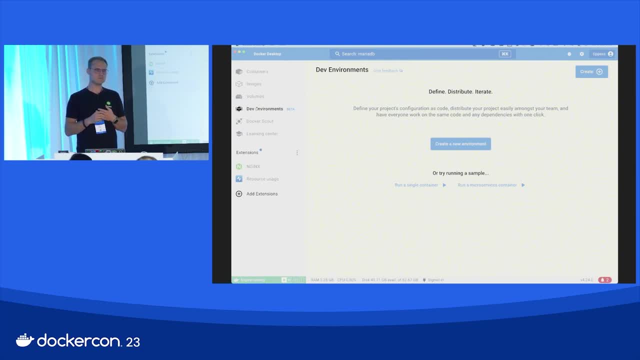 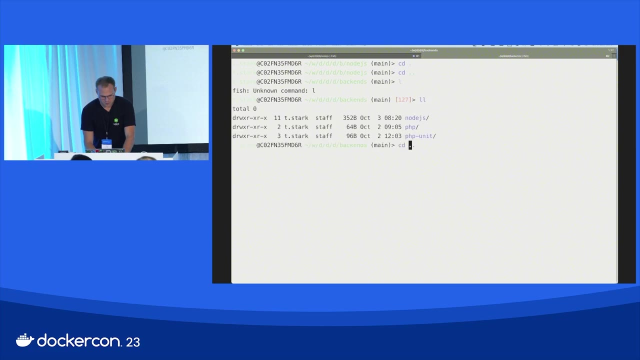 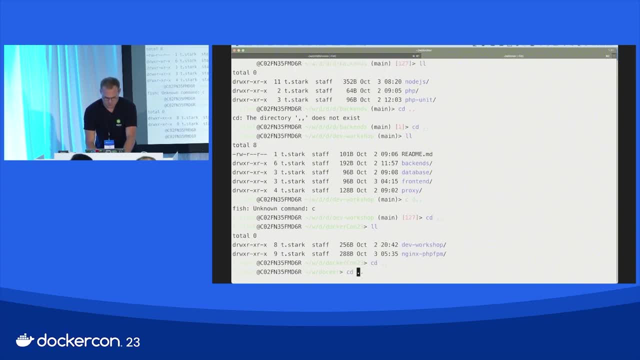 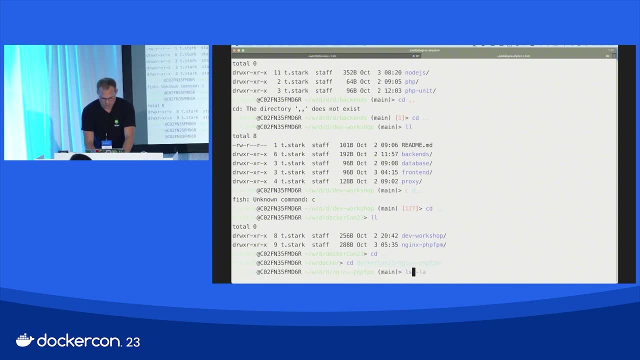 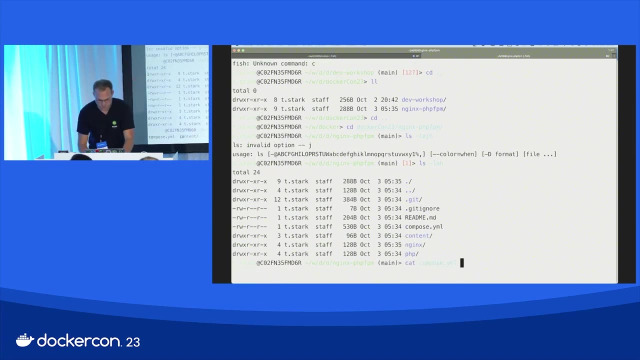 Can't tell you. This is something for later, but it doesn't really matter. Let's do this right now. Yes, I hope it's okay if we do some jumps here. So let's use nvm. I think that will do a little print. yes, 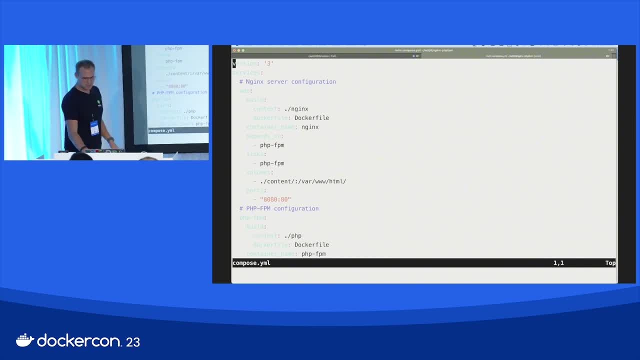 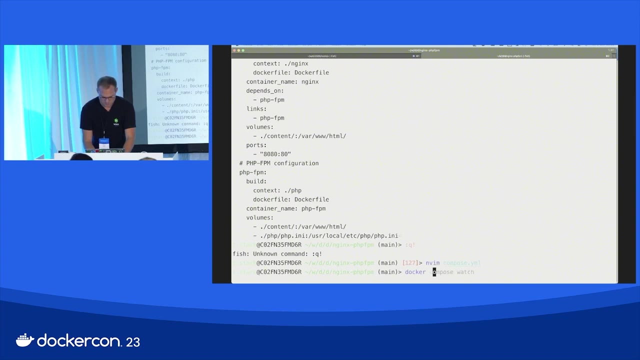 So this is a Docker compose file. that's how it looks like. So we define services with names. that's web, that's nginx, that's a PHP FPM. we need that later. So let's spin up this thing just by run Docker up, Docker compose up. 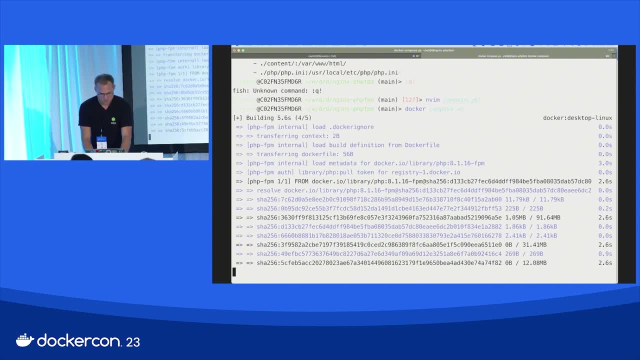 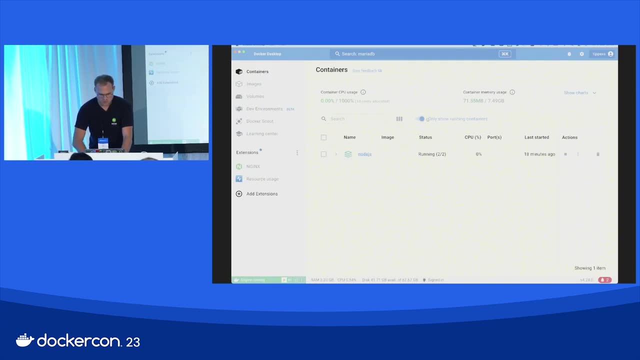 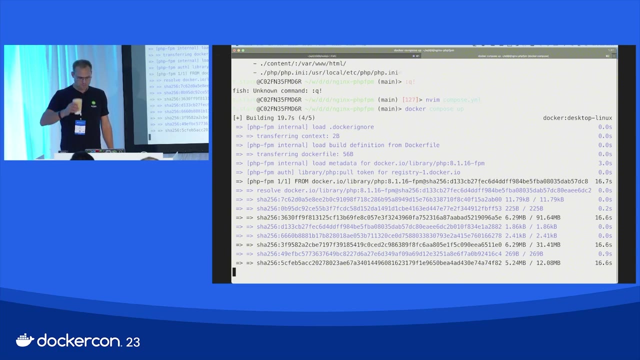 So right now it will pull it down, it will download the images from Docker hub and let's see. So now here in containers. it's still downloading. And this is another nice thing, because if you use the Docker CLI like you can use Docker. 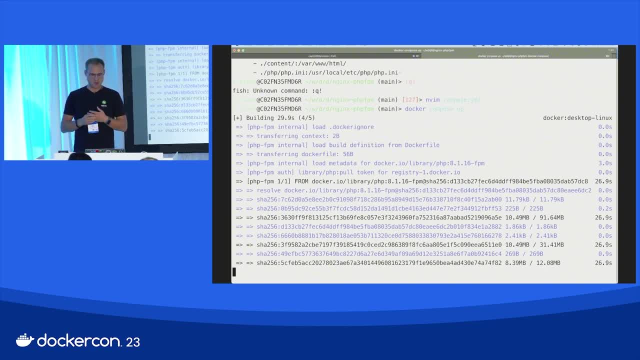 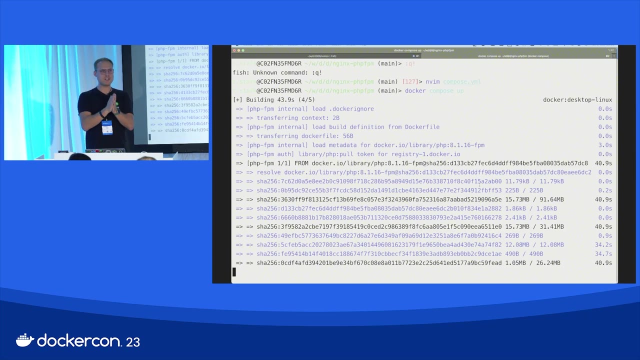 compose to print what are the containers. this is always advised. if you are using compose files and the compose in your process, you can type Docker PS to show all the containers, The only indication you have with Docker PS that these containers are like to print. 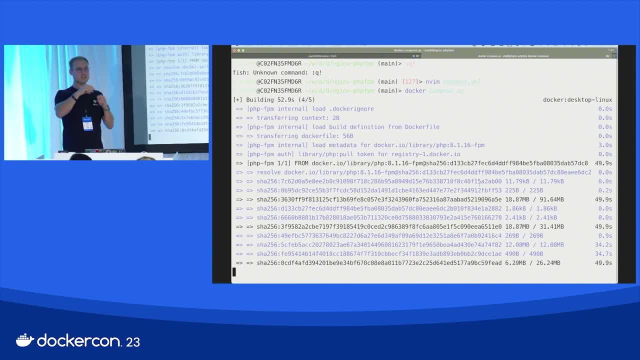 together in one compose file is the name at the end. If you change the name it is really hard to see in the Docker PS output what containers are in this compose file. There is another argument in Docker compose LS to print all the compose projects and the 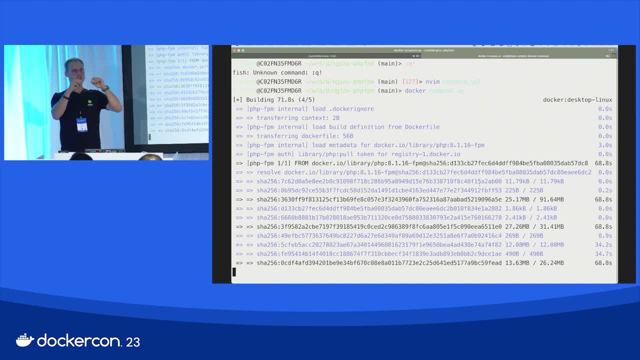 containers that are running inside of this project, Because if you have like two, three, four different projects currently running on your machine and you just type Docker PS, it is really huge output And it will become a little bit difficult to understand what container belongs to what. 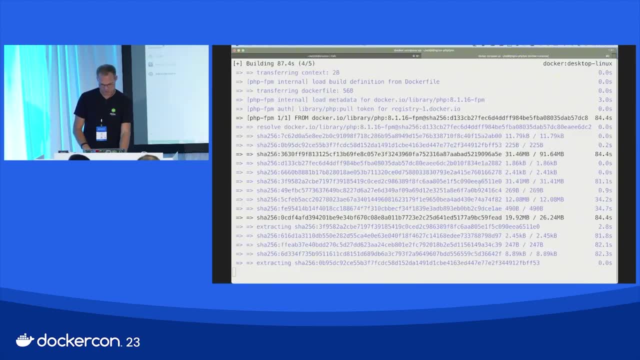 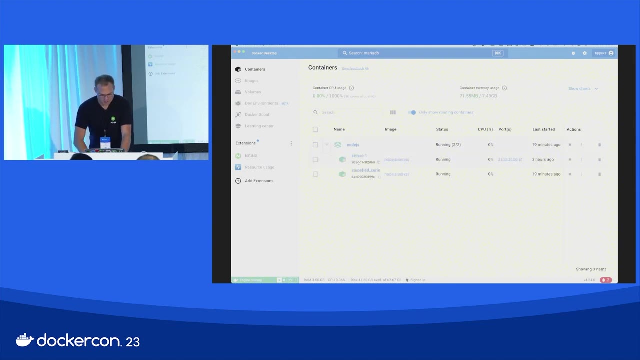 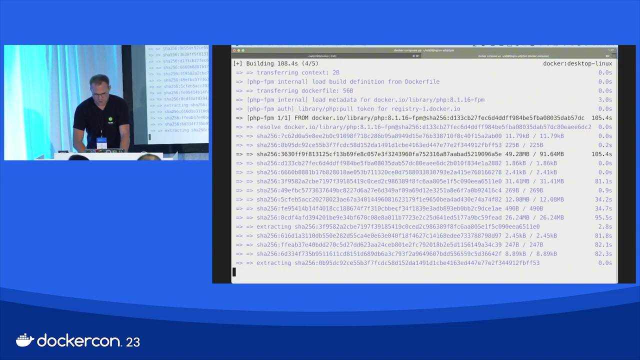 compose project. So it's still downloading. Yeah, but we'll be finished in a minute, And good point. We need this later anyway, So it's a good thing that we are downloading it right now And here in the container overview. as soon as this is up and running, we're going to. 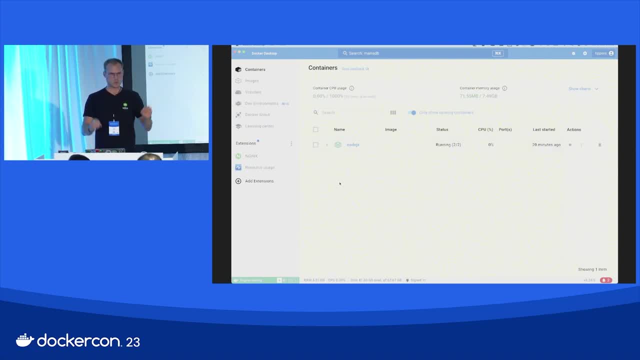 see. we will see there is this stack icon, And then we will see this is the compose project, And then we see all the containers that are inside of this compose thing. So it's again another nice overview of what's going on on my machine currently. 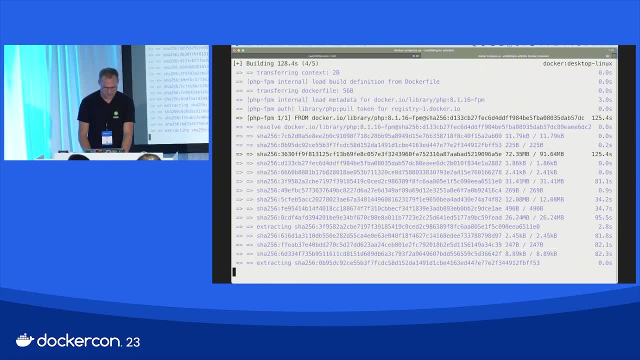 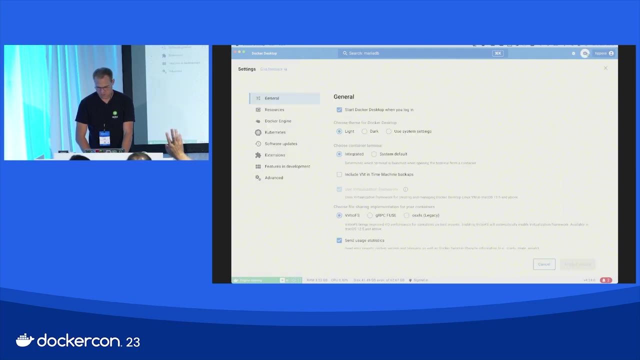 All right, So I let that download And while this is downloading, we can do then the overview of the container Of the project. Okay, So that was part of my pro tips for using Docker Desktop. In the settings pane, there is basically not really much special to say. 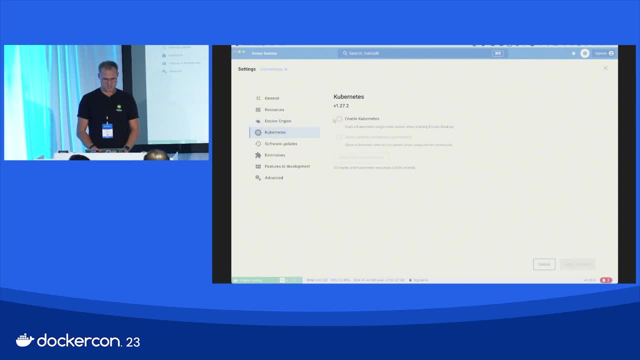 In the: yeah, Kubernetes is interesting, but I know there are plenty of yes, Yes, You can. So, yeah, In the settings there is a Kubernetes thing, but I know that we have plenty of sessions here about Kubernetes itself, so we'll not cover this. But this option is really handy because it starts a single node cluster- Kubernetes cluster- on your machine when starting Docker Desktop. So that means if you're using Kubernetes in your day-to-day business as a developer, sometimes you would like to check out if your Helm chart. 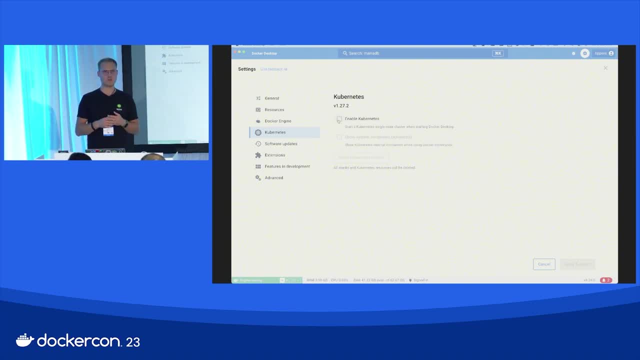 Helm is a packaging program or packaging project. So if you're using Kubernetes in your day-to-day business as a developer, sometimes you would like to check out if your Helm chart is working or how your container works or your manifest you're creating for Kubernetes. 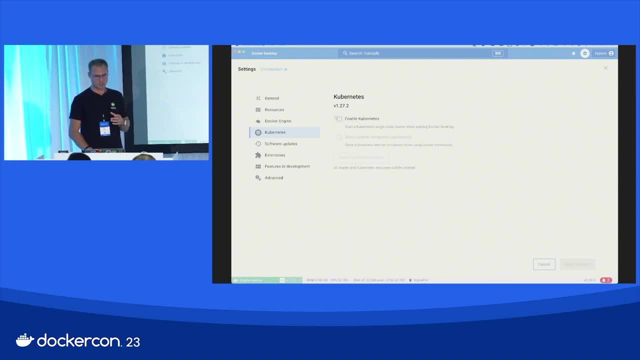 You can use something different, of course, but for quick and dirty testing. this Kubernetes thing is really great. I used that a couple of times as well. That's great. I mean, I'm doing Kubernetes from time to time, Building Helm charts. 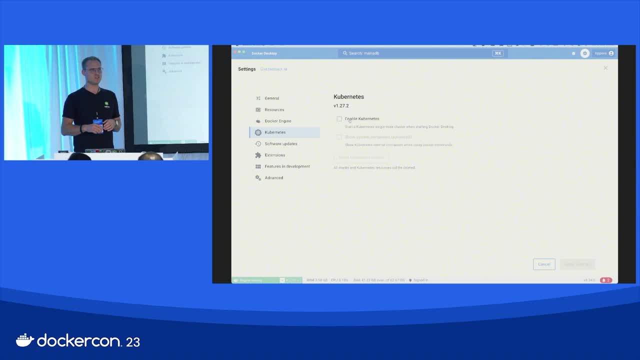 That's great. I'm using it, Adding SVER and all these built-in layers, And we do have a bunch of different Прminsų-type tables and stuff For this testing. this is absolutely great Because you don't mess up with this whole kubectl thing and Minikube and another VM. that's. 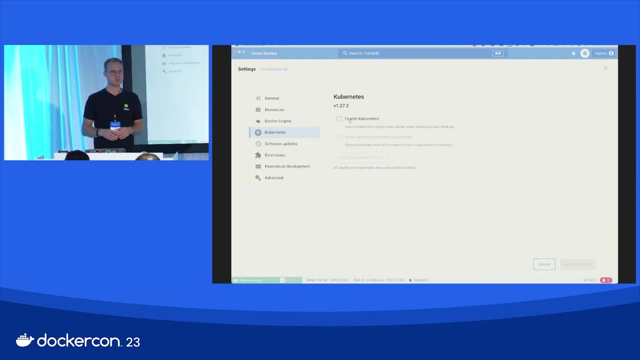 simply click enable Kubernetes and you have all the Kubernetes tools you need, and it just works. It's super simple And I disable it most of the time when I'm not needed to save resources, especially when I'm travelling or on the plane, I will not forget about the composting. 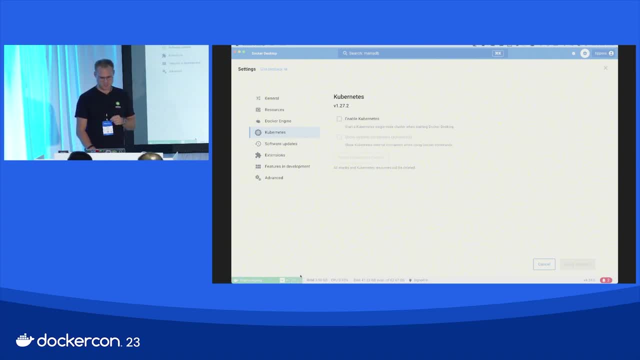 But there is a since the latest 2.2.7 upgrade. of course there's been some changes on the Motion which has shown some wear and tear to the compensation, but I'm not going to answer any further. two versions of docker desktop. they have improved the, the consumption of cpu and ram dramatically. 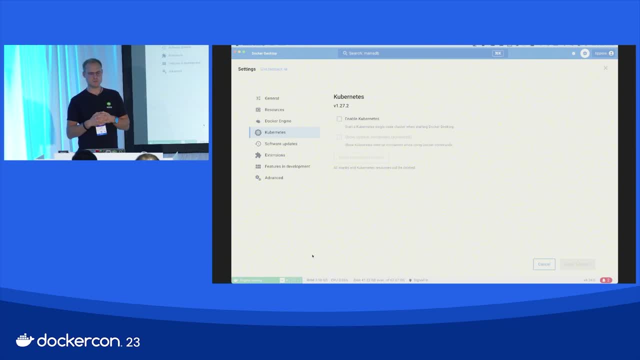 so it's dropped by 50, not just because they say it online, but because i have used docker desktop on flights a lot and prior the latest two versions, it was always like reducing your battery life by i don't know 60 or something right, um, and with the newer version they have some some memory saving. 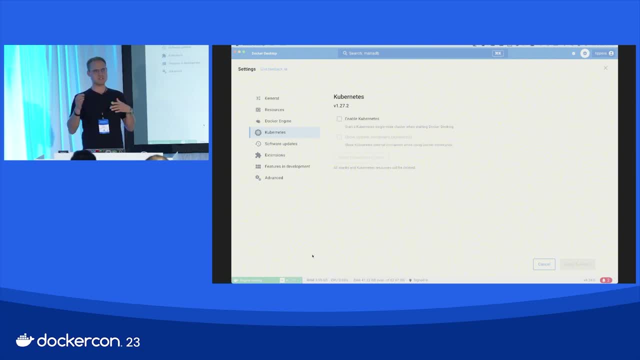 mode. so that means any time the docker desktop is detecting some idling stuff can turn it off. so it really saves your memory. and then in new, since the latest version, i really like this: if you want to stop or pause or do anything with your, with your engine, i can't. i don't know if you see that it's. 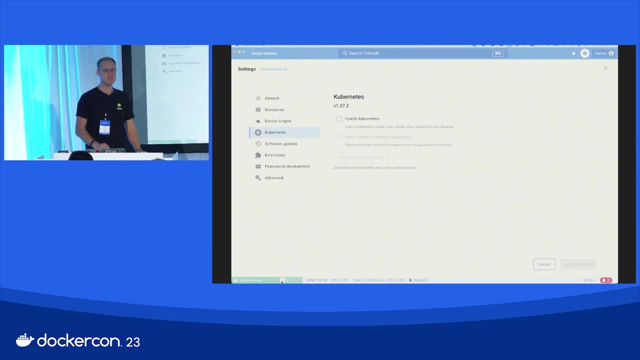 it's right here on the very bottom left in your docker desktop pane. you have now quick buttons for the docker engine. you can stop them, you can pause them, you can restart them. before that you always had to go here in the settings or right mouse click to the docker thing and then go here and say pause, restart quit. 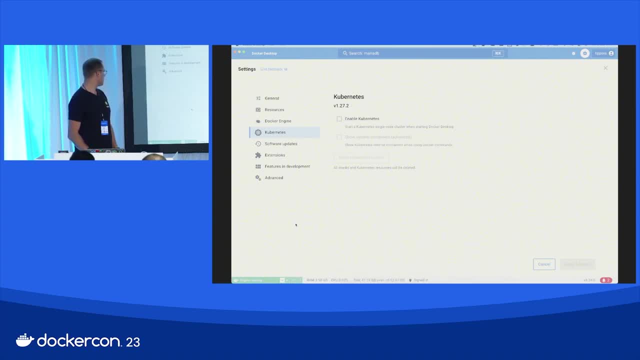 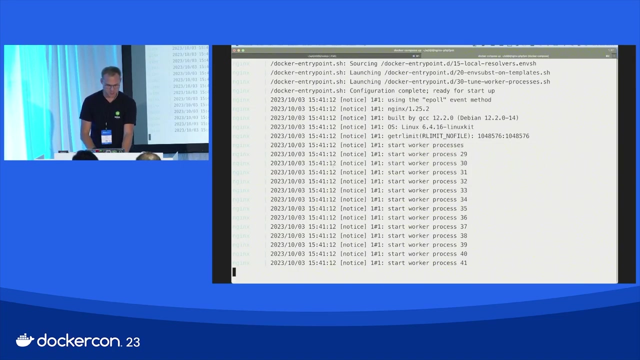 here and that's now here. it's like one one right click less and you don't need this actually very often. sometimes you would like to pause it. um, and the composting: now you can see this. it's things. yeah, it's downloaded. we see it's nginx and docker and the php fpm in. 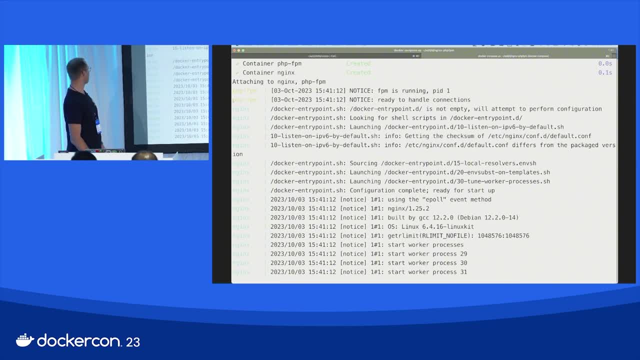 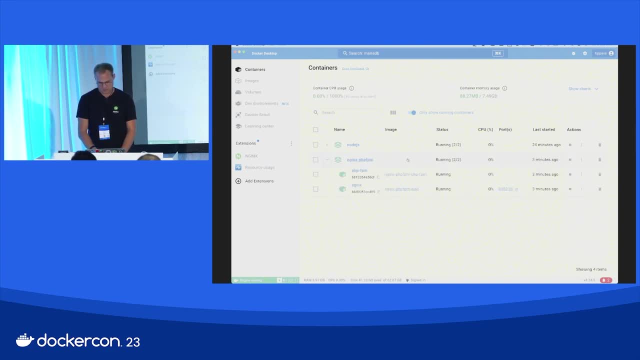 what color is that here? like, like, i don't know, yellow, brown, that's blue. um, so if we go here, we see this: we have the, the nginx, php, fpm project, and it says now php, fpm and nginx. so you can, you can see this stack and it shows you that we have two containers. 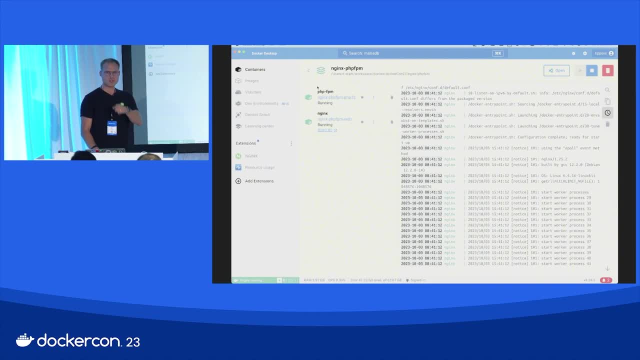 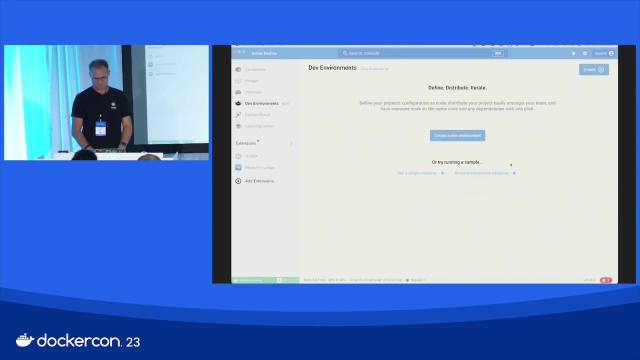 running in this stack and your question um about running compose files from um docker desktop is something you can use. this development environment. there is dev environment. it's currently in a better mode, but you can create this and this is basically creating a docker compose for you so you can give it a name. 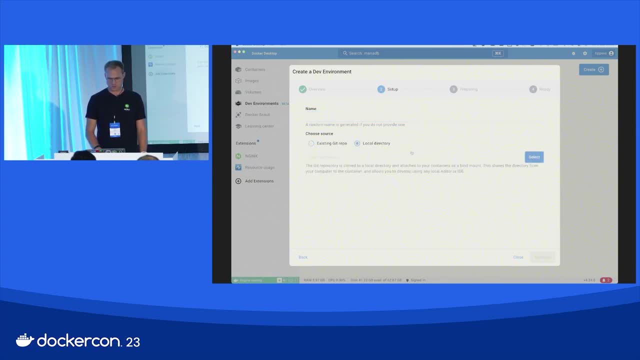 you can use an existing git repository or a local directory. select one, then it will basically prepare all the images for you and then you can use the dev environment to spin up this docker compose. the dev environment to me is kind of a ui for creating docker compose stacks. actually, haven't really used it a lot. reason for that is i'm 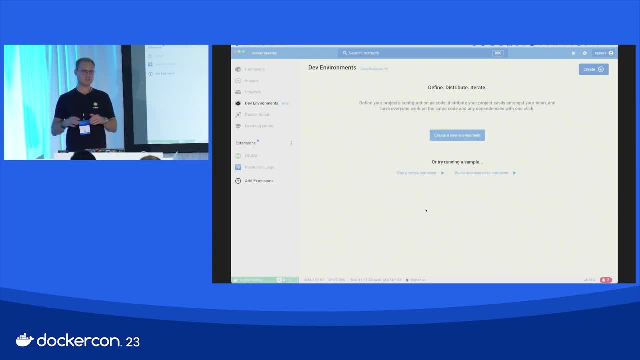 maybe i should try that, because i'm i have like lots and lots and lots of docker compose files already ready, um, so you have github repositories as templates, so to me it's not really interesting to basically create them from scratch again, um, but i think- and this is something we can try if we have some time, i think um. 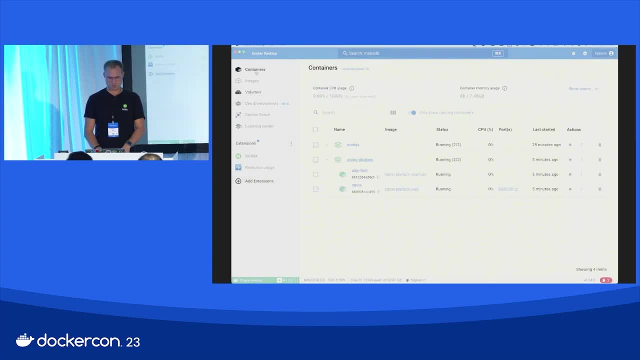 if we can load a docker compose file here in docker desktop and see if that works. yeah, i think that that should work. then let me see when we do dev environment, create new, and then let's- i love screwing things up- um, add presentations. docker con 23. uh, local directory select icap. 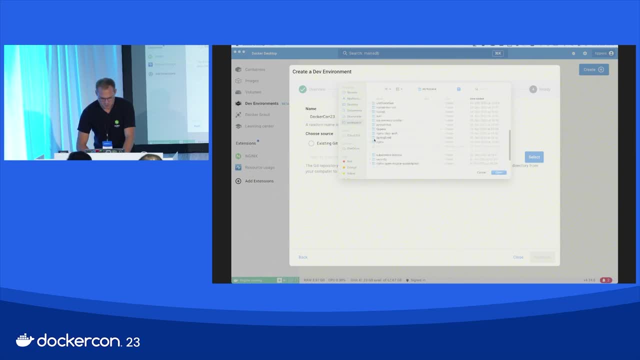 where is docker holy cow? docker, docker con um is here. yeah, there's the compose one. okay, open, continue. well, let's see there's a compose file in it. that's what we just started like 10 minutes ago. let's see what this thing is doing. yep. 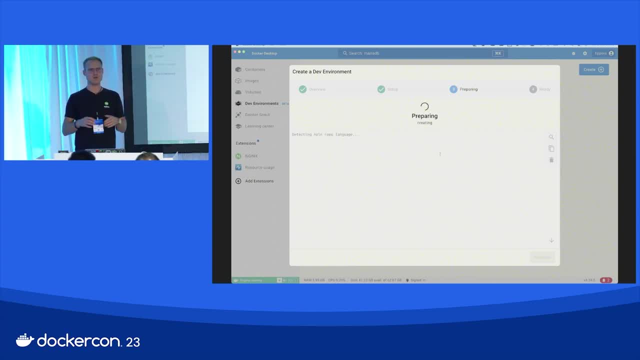 all right. the question was: what is the difference between a docker file and a docker compose file? sorry, a docker file is defining a single container image. it's like you're building construction plan for a docker image. a docker compose file is more of a construction plan or con instructions for. 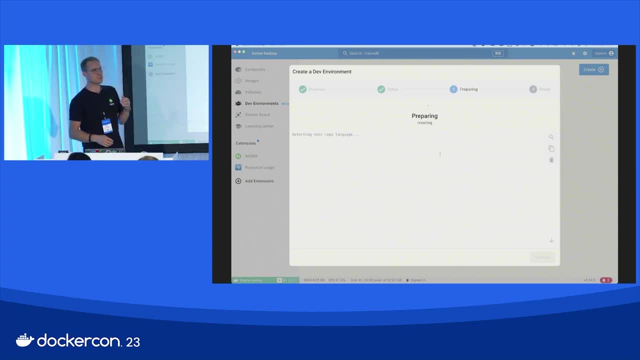 your whole service. for example, if you need a web application, for example, if you need a web application that has a database, php, my admin, an nginx web server- and this is something what we will do today- a nodejs backend, another nginx container for something different, then you have like five or 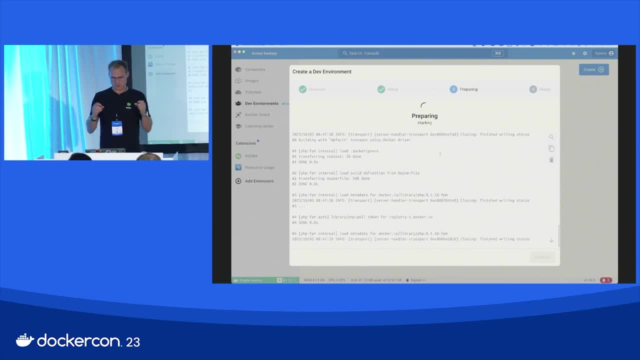 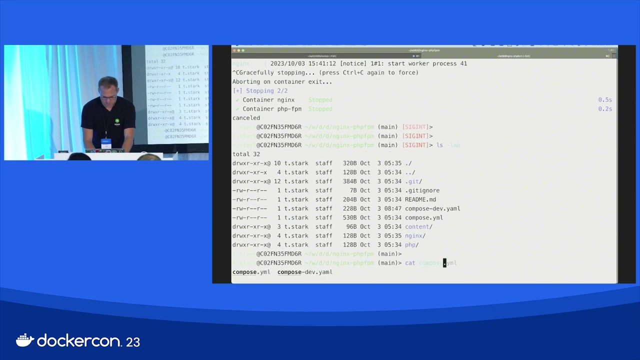 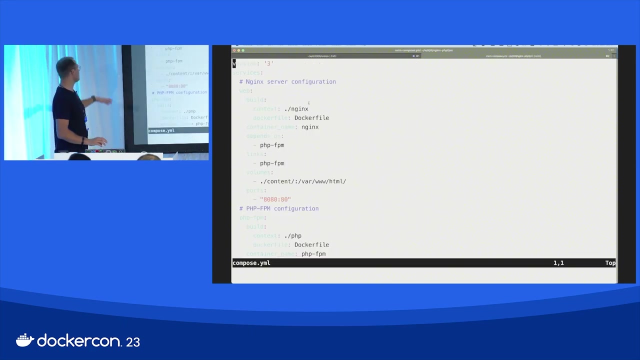 six different docker containers. and then this is a compose file. this is what we have in a in a compose file. so card compose, yaml or use nvim. see, this is not the. this yaml syntax is not what we have in a docker file, right? so what you see here is we define services. web is a service. 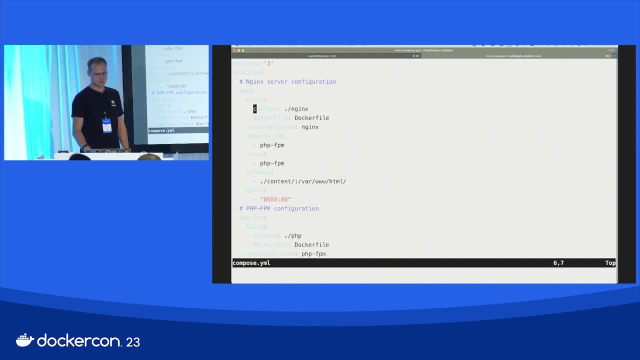 and this can here. you see, this is built and build tells docker compose. go in this nginx directory, use this docker file. in this case you don't have to define docker file as a separate line because the Dockerfile is the default. If we say, go in the nginx thing and build the container. 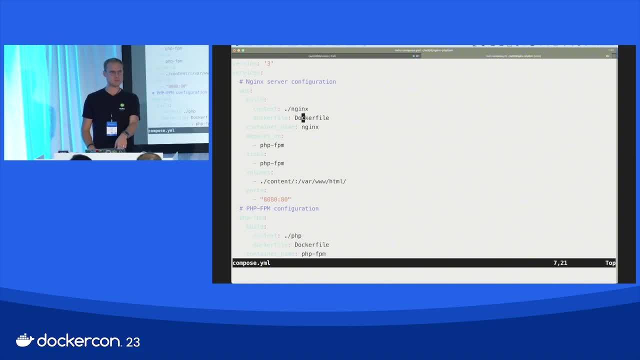 it will automatically look for Dockerfile. The reason why I'm defining this here is because then I can tell you if you have a Dockerfile for production that is Dockerfiledef, Dockerfilesomethingdifferent, for whatever reason, you can use the Dockerfile tag here. 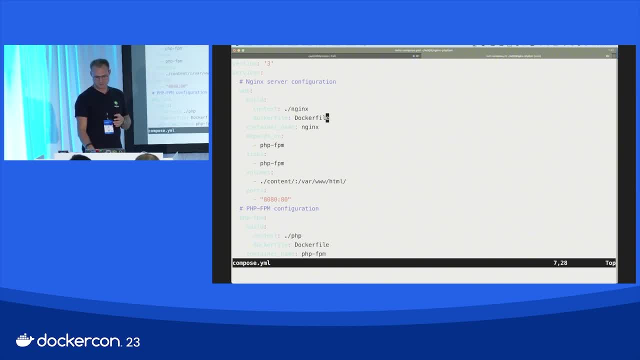 or the configuration to define, okay, what Dockerfile you want to build. See, this is the reference between what is a Dockerfile and what is Dockercompose. Dockercompose defines your services and the way you deploy your services, even on production environments, to be honest. 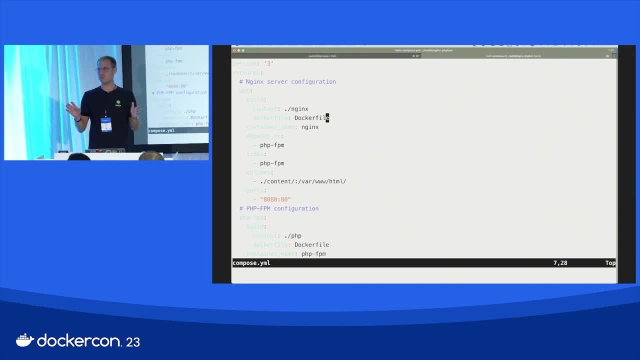 It's not a development thing alone. You can fairly use Dockercompose on production environments as well. Yes, Yes, Sorry. So this is the question is it's? this is like a service file for Kubernetes That's not aligned to Kubernetes at all. 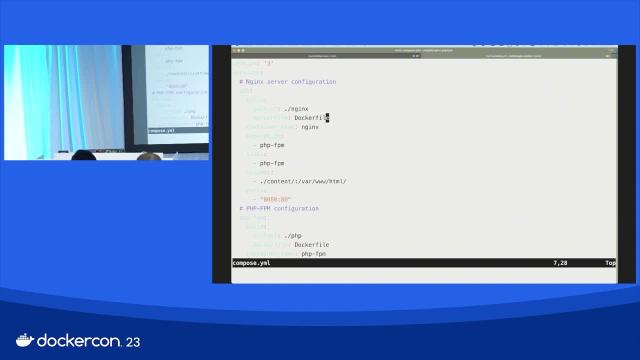 A service definition. a service YAML for Kubernetes has the same syntax, because it's YAML as well, but it has a different. it looks different. It looks different. So this is not a service file for Kubernetes, This is a definition for Dockercompose. 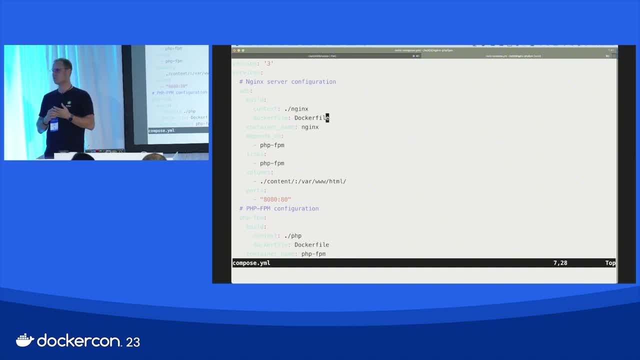 A service definition for Kubernetes looks a little bit different. No, You cannot use a Dockercompose file to just deploy a Kubernetes service. Yeah, you can. I mean, if you have a Dockercompose file you can create service files out of. 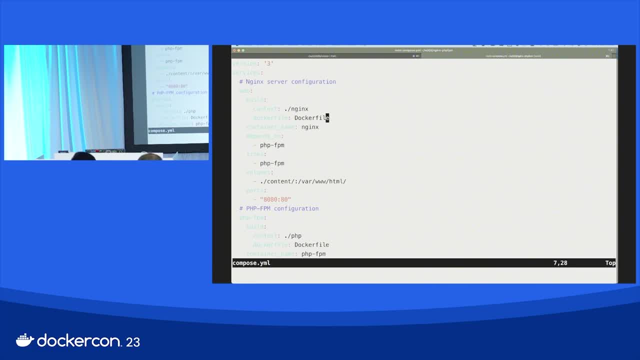 out of a Compose file, But not like automatically. You have to combine, like, write them, but it's, it's, it works. What link? What do you mean? Oh, links, Okay, good, good point. 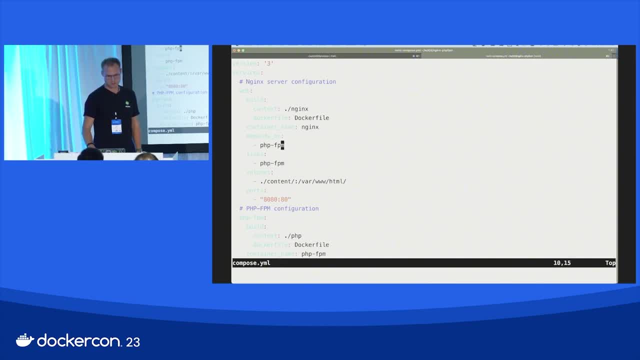 Links. Okay, The question was: what does this link mean here? A link here means that depends on, and link means that this NGINX image here depends on the PHP FBM one. That means I can like. I have to start up the PHP FBM first. 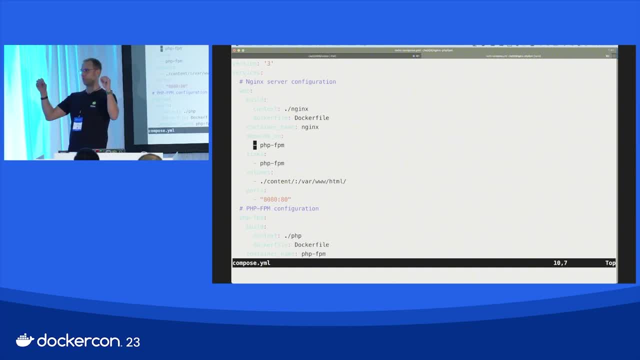 and then I can start. NGINX And links is like a net, that that we connect them on the network level so they can work with each other And can connect to each other, And this could maybe something for the Active Directory thing. 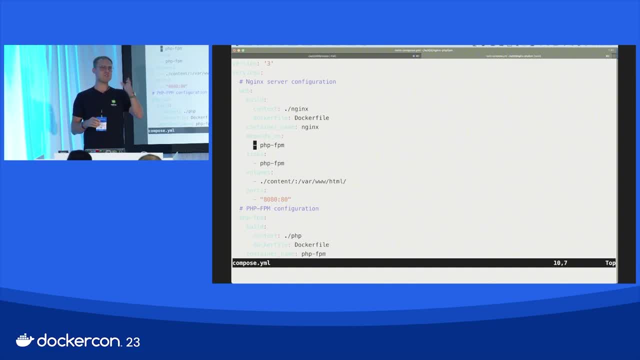 But this is. yeah, I guess you have the Active Directory outside of a container, right? So so we will have a look on this problem in the break. Yeah, How is the links different from specifying a network between Network, tells the Kubernetes. 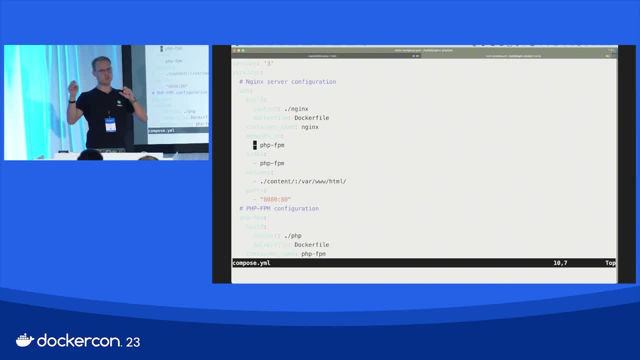 oh, Kubernetes Network tells the Docker Compose what network to use, And with link we can. we can, for example, exit or use the, the name of the of the FPM inside of the container to simply navigate to that. 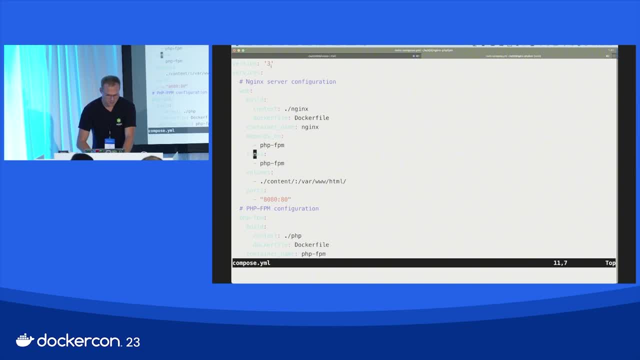 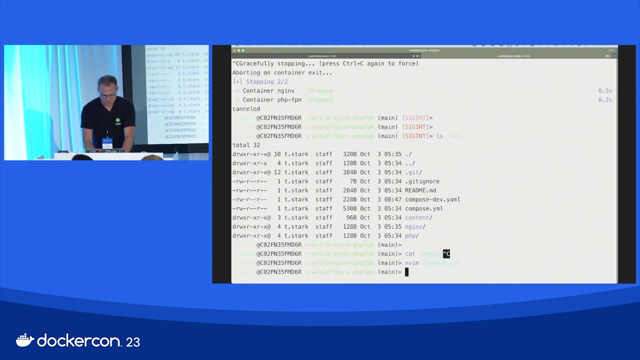 And that's what we see in the. let me show you this Here. we see we have the name of this one, of this FPM thing. There is a container named PHP, FPM. See this, this one. And now, when we look, 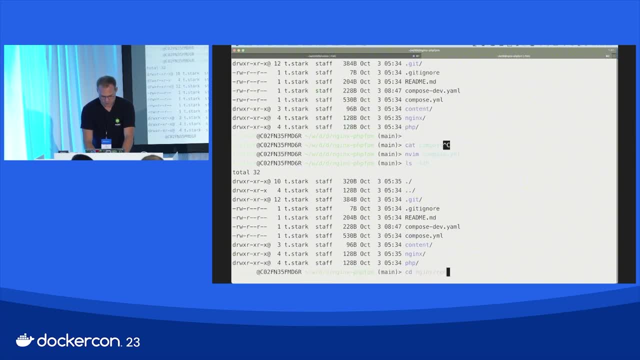 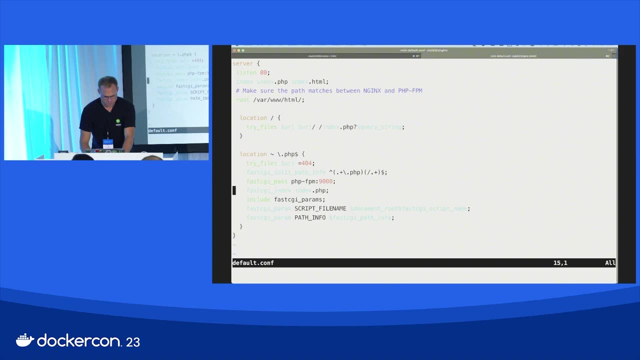 in the document: hey, in the Nginx config See. Then we say it's PHP, FPM, port 9000.. We don't have to expose port 9000 to our host machine because it's not needed, because Docker creates a network. 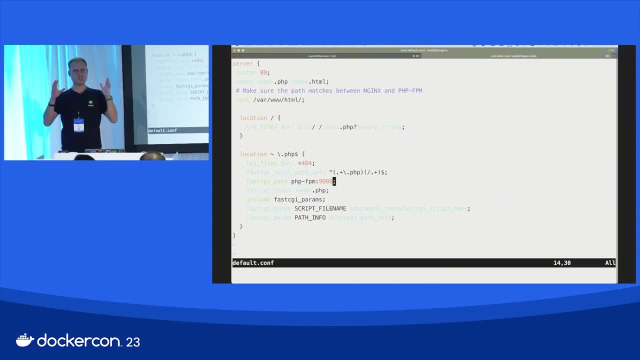 like a NAT network for this composed project, And what we do is Docker puts some host magic in each container that then resolves to an IP address. At the end it's behind an IP. FPM is like the PHP. FPM name is a link to a given IP address, of course. 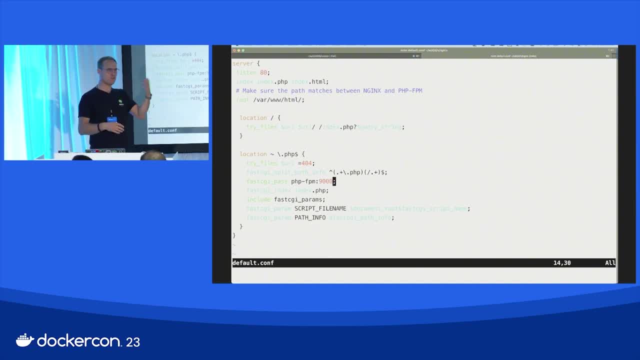 Because we're doing TCP of course, So in layer 4 and 3 on the network cannot really work with names, So we need an IP address to do an actual binding to the FPM port, which is 9000.. But Docker knows how to do it. 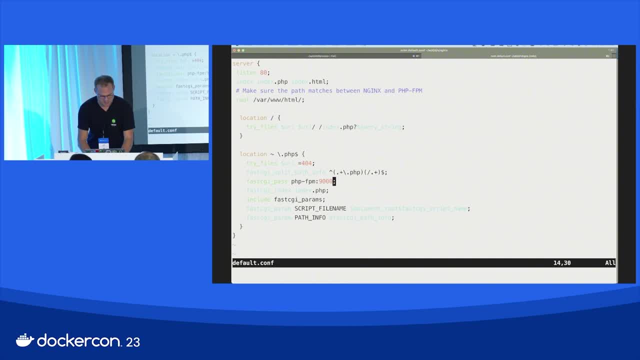 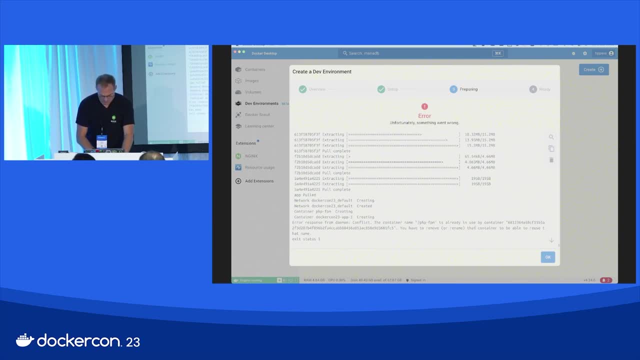 Docker knows what IP address is behind PHP FPM, And this is something we can find out using Docker Desktop as well. Absolutely amazing. It's saying error: It's already used by another container. I think it will work as soon as we delete. 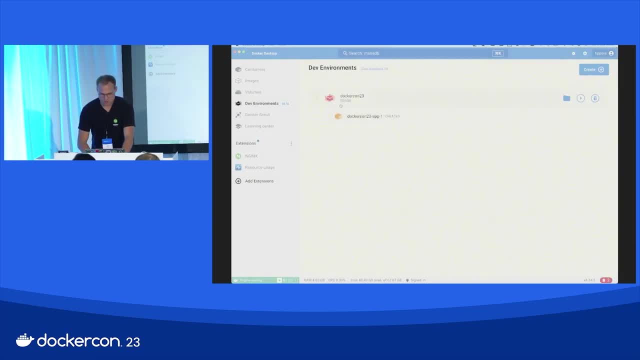 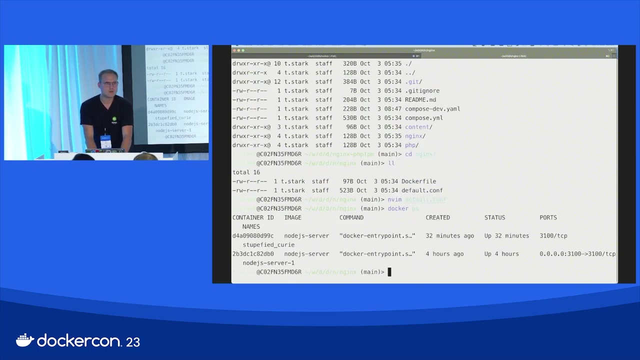 this. I'm pretty sure we can use Docker compose files in the dev environment as a getting started point. I will test this in the break. So What did you say it uses for 9000? That's the FPM settings, basically. 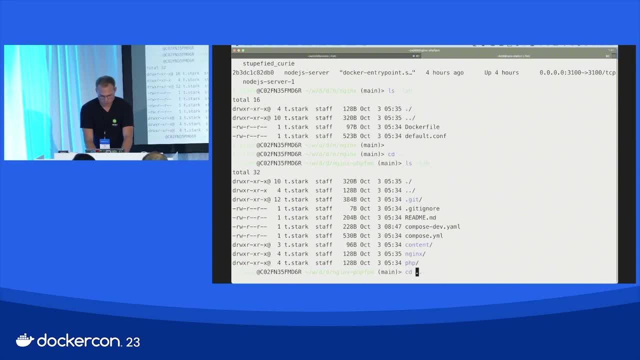 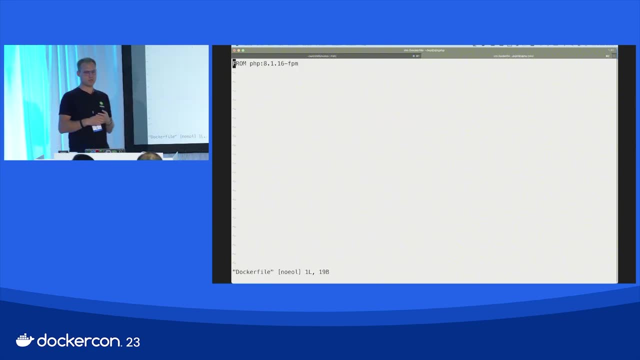 Inside of the. that's default. That's default. See, we're just saying PHP. Well, that's old PHP, 816, FPM And per default it's using port 9000 as the entry point for the FPM. 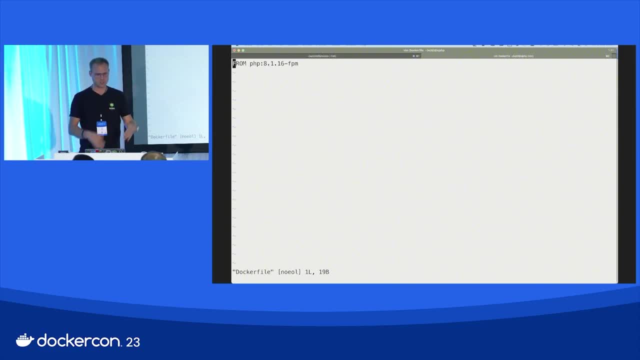 That's something we can look up in the documentation using, for example, Docker Desktop check, PHP 816 FPM. And then we can see this: And the error we just got in the Docker development environment was saying: hey, you're trying to create a container. 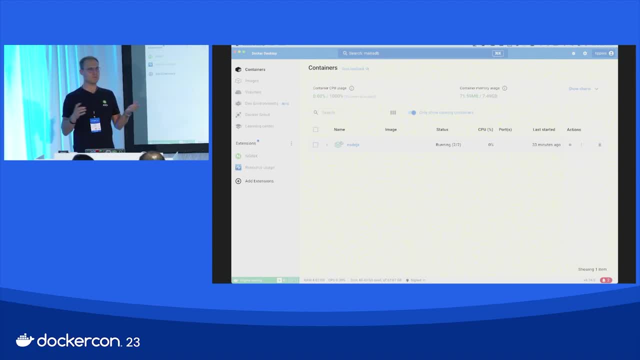 that is named PHP FPM and you cannot do it because there's already a name And the names, as you can now imagine, because of this IP address thing, they are unique. That's why Docker is always creating these funny names. 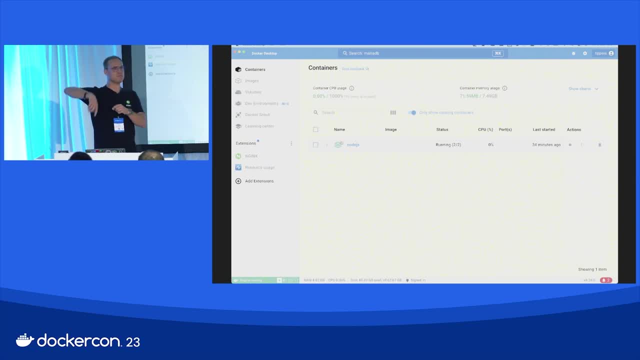 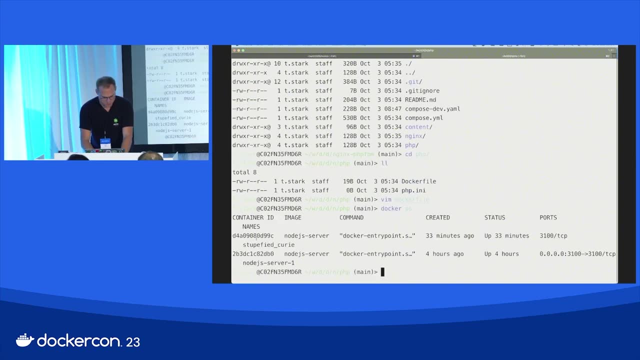 If you don't define a name and you type Docker, run something, you will have this funny name, this funny container name. Have you ever seen this? Yeah, Stupified query. Interesting Things like that. that's pretty amazing. So that's why. 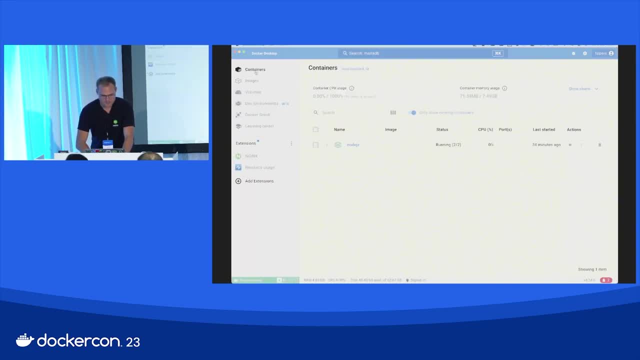 And now the Docker PS thing or the Docker compose thing is telling me that the PHP FPM already exists. So it's here, So we can delete it. delete forever, Don't need it anymore, Go away, Start. Oh, it works. 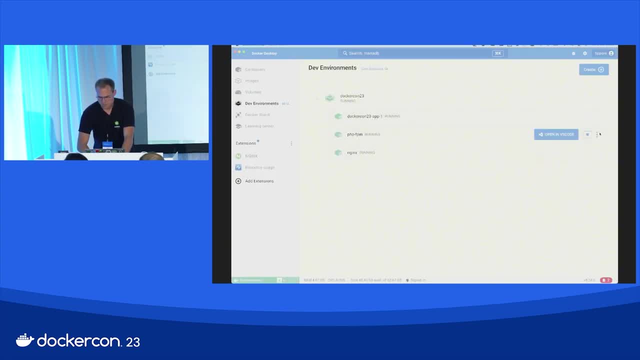 Yep, Let me see PHP FPM Next sec. Yep, Okay, so it works. So what we just did here was there was the question: can we just host the Docker compose file in Docker desktop? What I've done is I've used the dev environment. 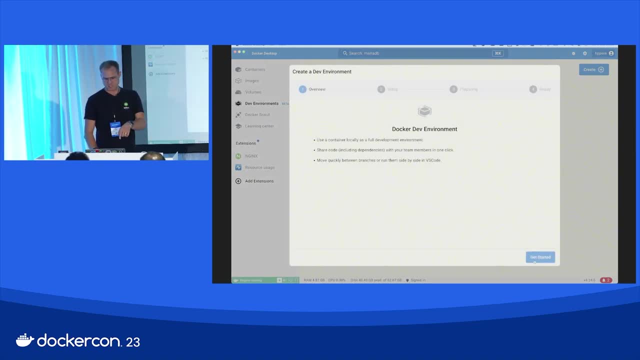 and then I created a new one, And then I pointed this next step to a local repository where the doc, to this PHP FPM thing, where the Docker compose file was already in it, And then I just said launch, pulled down all the images. 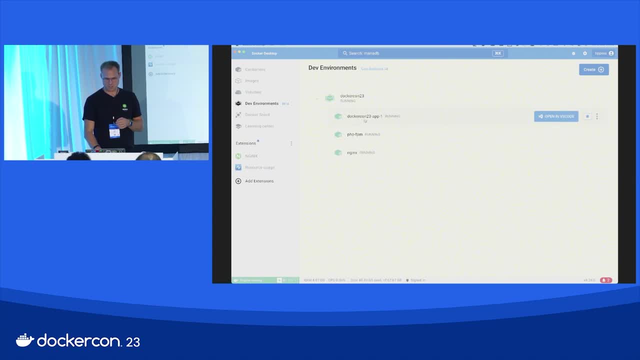 and now it's created this thing. I have no idea what this is, but this is something I will find out in the break, but in generally it works. So that means we can use the dev environment to basically host our Docker compose file. 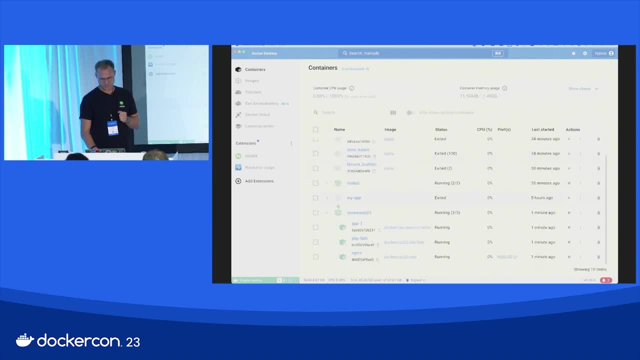 So we can see what's going on in the Docker compose files, in Docker desktop, And then we can see here again: this is the stack here: Docker con 23.. It's saying running three out of three And then if we click on it we see we have the PHP FPM. 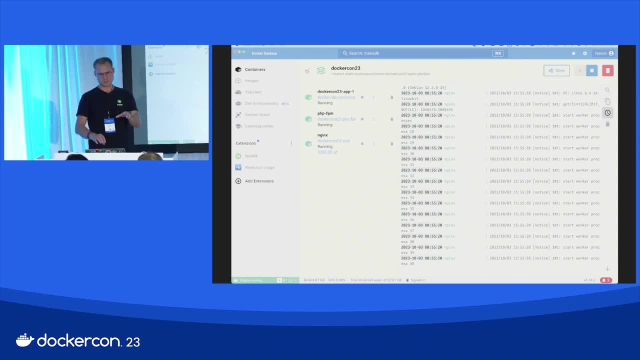 and we have the NGINX one. So that's why I'm saying this: this Docker desktop gives you a nice overview about what's going on in your compose projects, And compose, to me, is one of the most important things when it comes to development and web development. 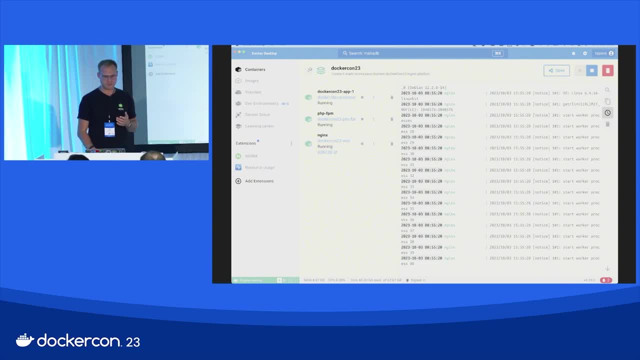 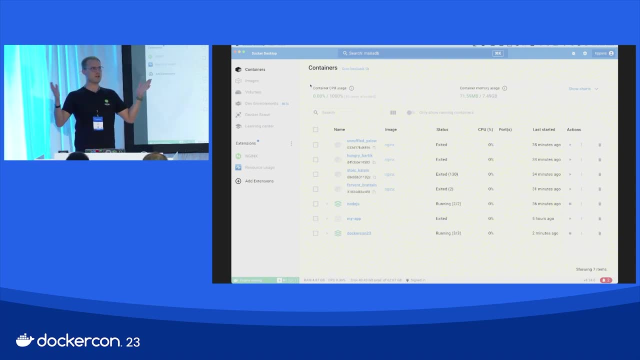 and Docker, because it will just define the stack you need to launch an application, And this is something that's very interesting for you, actually, when it comes to break your applications into smaller pieces and you would like to refactor huge applications into smaller pieces. 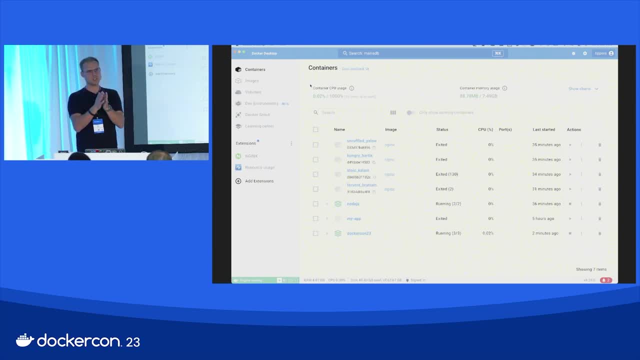 Docker compose is very important because it describes what's basically needed to launch and spin up the application for development, right? So we will see this during the course, All right, so then Docker extensions. Yeah, I said pretty neat, pretty interesting thing. 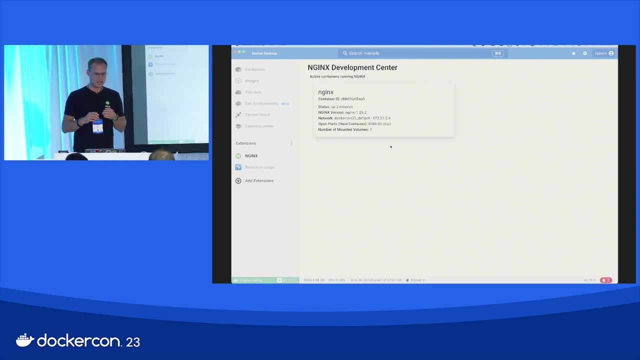 I have created this Docker desktop extension for NGINX a while ago And extension is a great thing to enhance the productivity from Docker desktop even further. There is a catalog here you can browse and you can install like there are many, many. 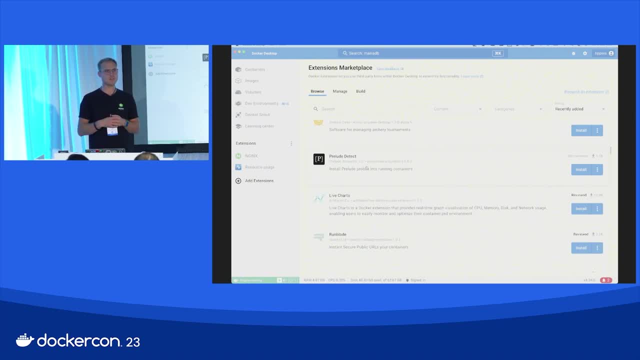 many extensions and they will be more every day. If you have an idea of creating Docker desktop extension: very simple, easy. It's a very simple process. For example, here we have the NGINX extension and what's the normal way of managing NGINX? 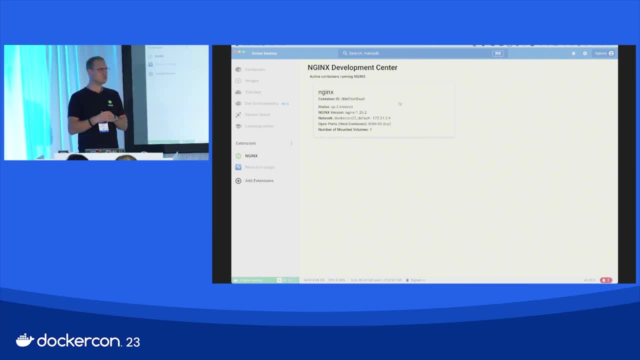 on your dev machine. when you're doing Docker compose, You're using Docker exec or you binded the config in your NGINX container. then you change the configuration. So you have to reload NGINX. you go Docker exec, NGINX is reload- annoying inefficient. 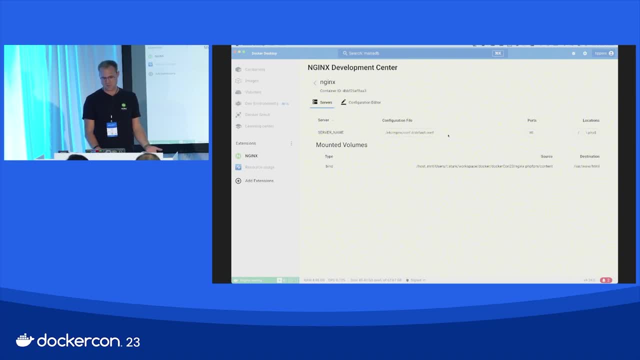 With the extension we can see: okay, this is the extension. that's the container ID. It exposes port 80. It is this file for find here that we can use and change it. We can do some changes to the file. 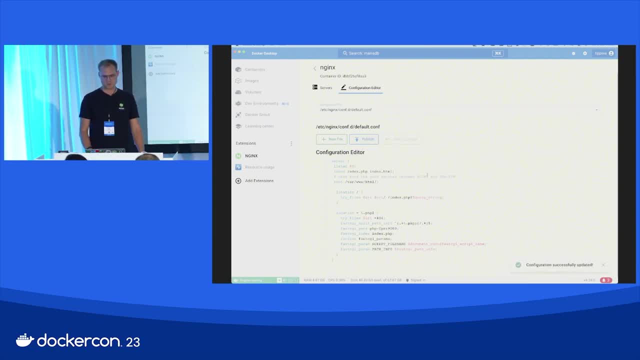 and then at the end we say publish and it will upload the configuration and automatically restart NGINX in the background. So it's just efficiency. yes, I wrote this. yes, Perfect, Oh, literally cool. That's good, that's great. 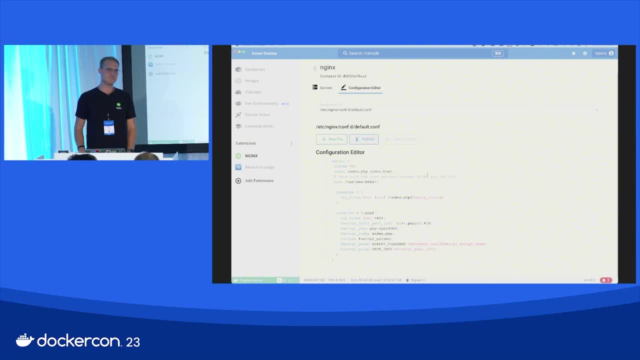 So tell me if you have any problems with it. then It's really nice, because the desktop pop-up it said you should be using this, otherwise I wouldn't know about it. Okay, How did that alert happen for an extension? Yeah, that's because we were. 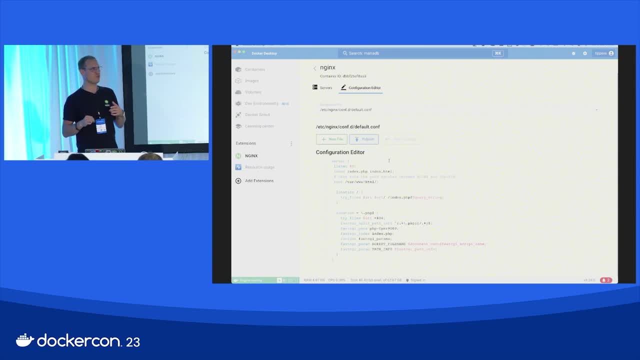 like Docker, was thinking about recommendations, about extensions for given processes or given, like, specific user groups. If you're in web developer, it is very, very likely that you will need some proxy server somewhere in your Docker desktop environment just because to deal with stupid course headers, and we will see this today. 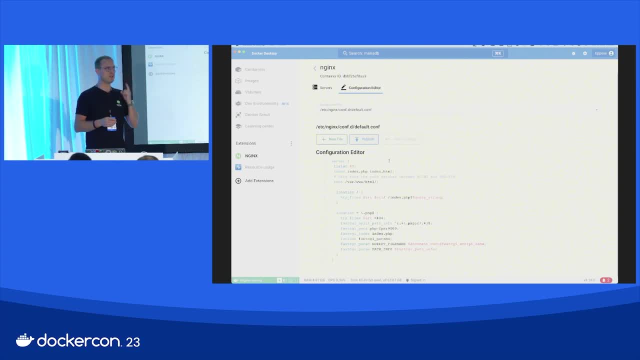 because this is the most common pain point when you do even web development locally. You have a front end that is localhost 3000.. You have an API that is localhost port 8080.. You try to combine them and the first thing you see 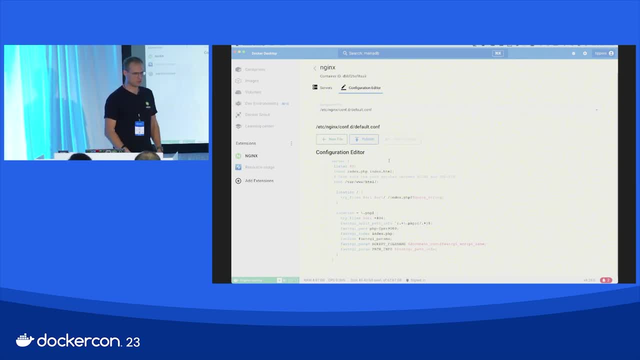 in your browser is: hey, there's no course header, It is localhost. I don't care, We need course. It's localhost, I don't care, so we need course. So, and to do this, Docker desktop and the extension. 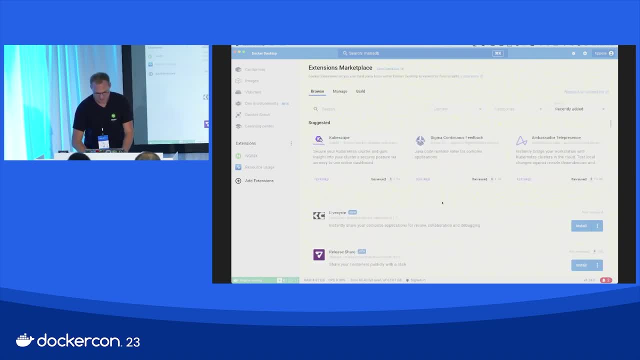 is really helpful And because it has how many downloads. It's like Jesus, let me see: Oh, 21,000.. That's good. So that's why Docker sees: hey, 21,000 downloads, So looks like people need it. 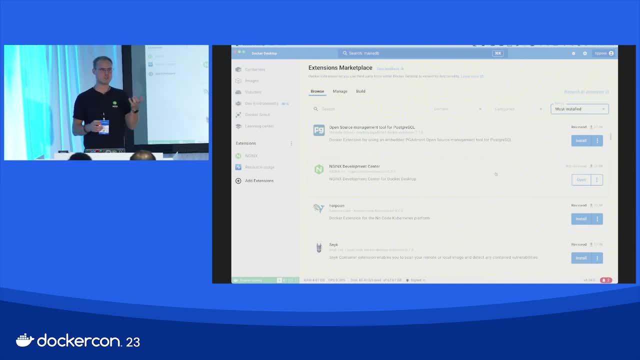 People find it useful. So that's why you see this recommendation And we will use the Docker desktop extension from Nginx through this course. So good. So this is extensions. Another reason why I really love Docker desktop because with the extensions you can do resource monitoring. 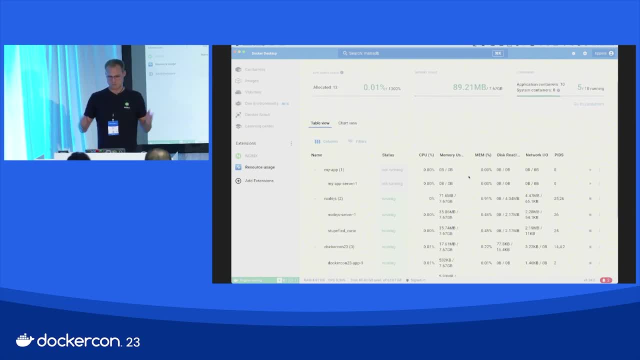 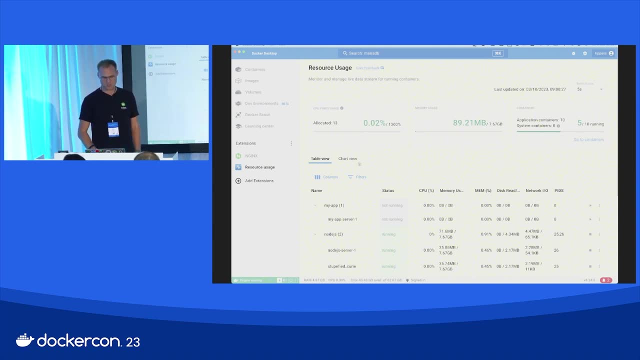 and see why your machine is freaking out, because you're running Jenkins and GitLab and another Java process and that's eating up all your memory, for example. So that's what you can easily see here in this resource consumption thing. Let me check the timeline. 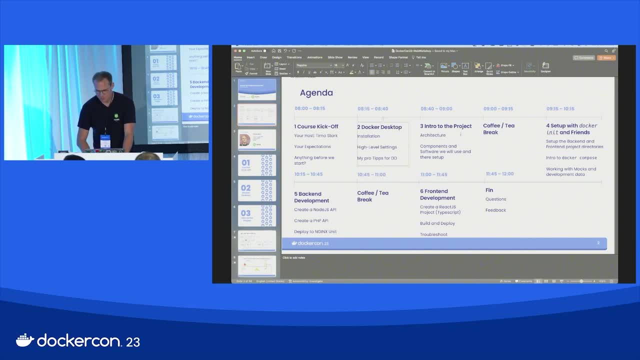 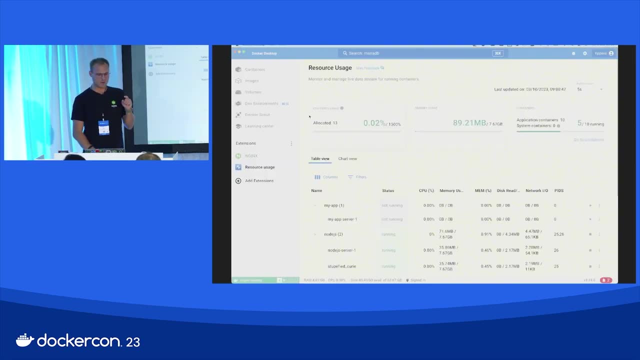 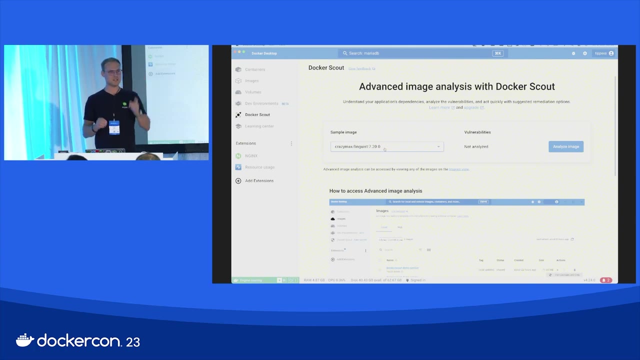 Holy cow, We have a tea break actually right now. That's bad. OK, We do this And then I will jump, I will shift gears a little bit, then We will do the Docker scout and vulnerability scanning. That's a word. 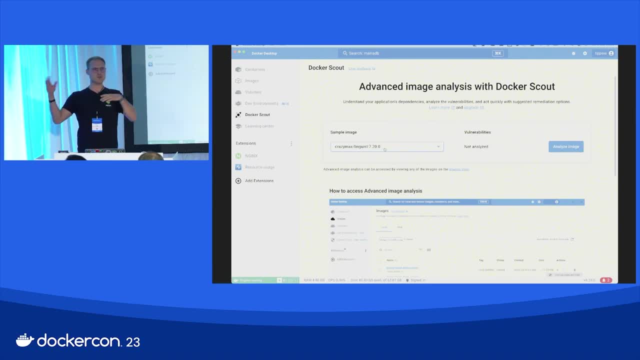 Then when we introduce the vulnerability scan in the process later, It's part of Docker desktop, It's part of the CLI, But we will do that later. then after the break. So that means after the break. I have to give you a very, very quick introduction. 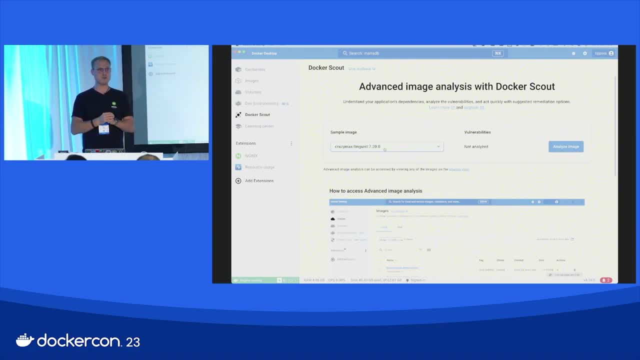 to the project we are going to build, because I have talked too much about Docker desktop and how to get started. OK, But I hope that is interesting for you because that's the most important thing, because you can waste a ton of time using Compose. 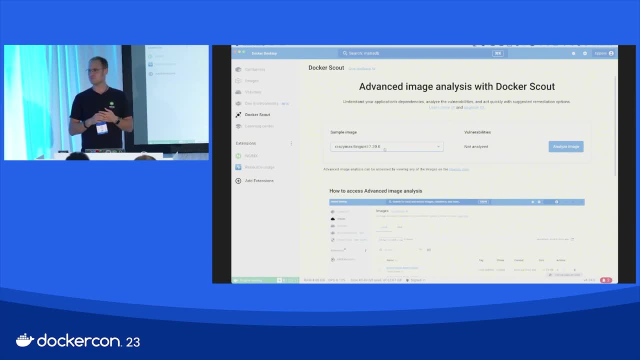 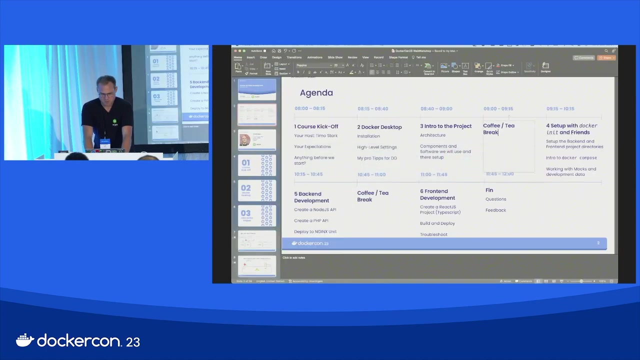 and the whole thing just not efficiently enough. Oh cool, Yes, Yep. What images do we need? That's an excellent idea. You can pull down Nodejs, OK, OK, OK, OK, OK, OK, OK. 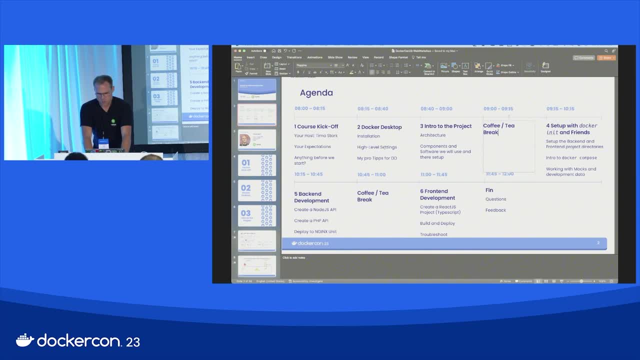 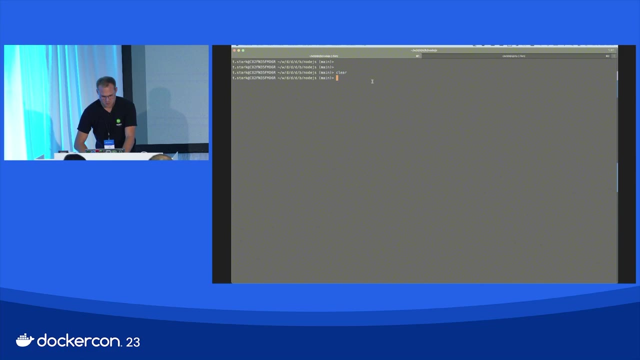 Nodejs is something we need. Version doesn't really matter, 20 should be fine. Nodejs, Nginx, of course, The PHP FPM. There is a Git repository for the PHP FPM And let me show you this: GitHub, the Git repository. 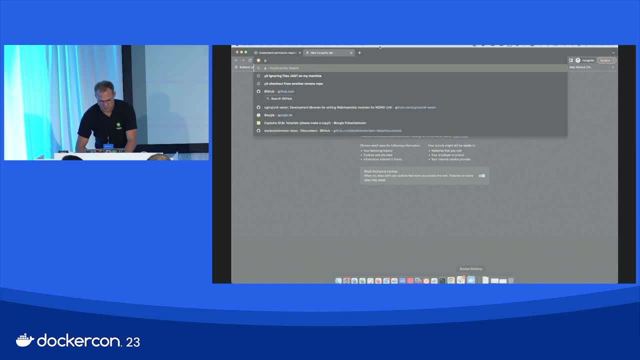 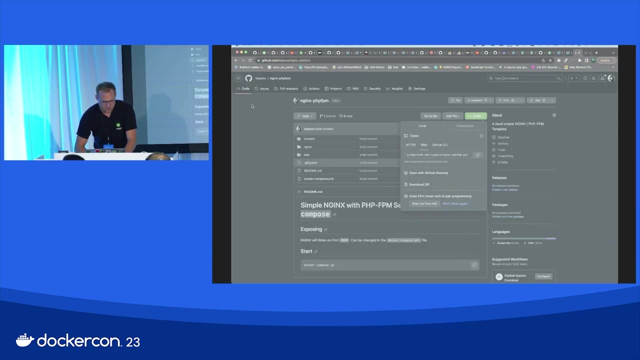 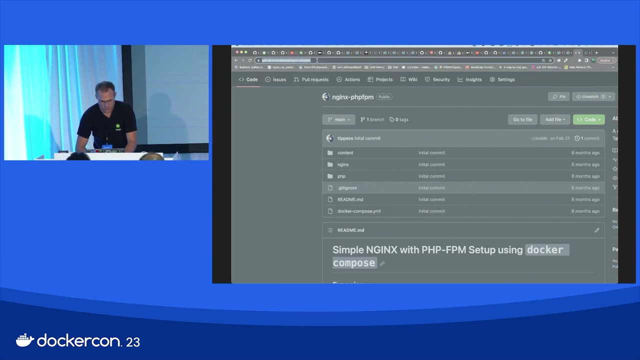 Because then you can pull this Nginx FPM example, because I have something that is a lot simpler than FPM. That's why, Yeah, it's on my GitHub repository, It's this And this will pull down at least the. it's an older FPM image. 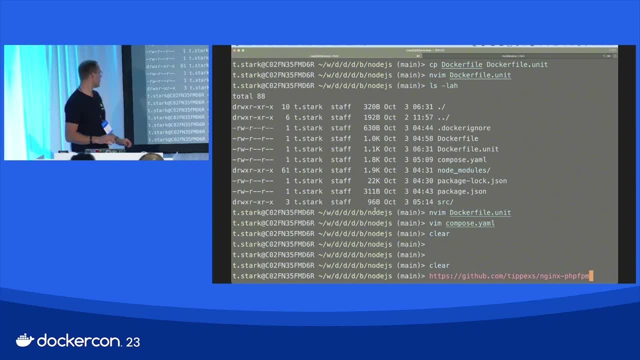 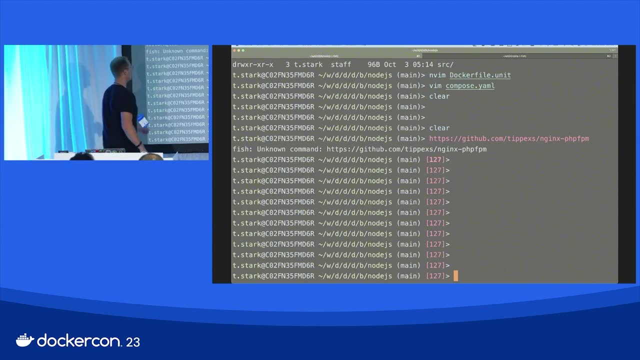 but it doesn't really matter. Can you see that? OK? No, because it's on the very bottom of the page. It's this one. It's GitHub, my interesting username, and then nginxfm- OK, And then nginx-phpfpm. 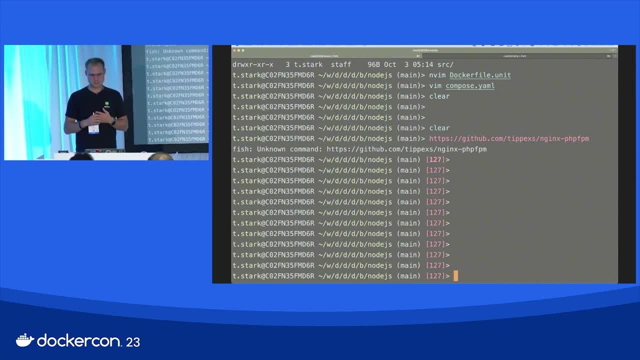 If you pull this image, like this repository, and then if you do docker-compose up, for example, it will automatically pull down at least the nginx and at least the FPM image. So we have something we can play around with If you really want to, and that's something. 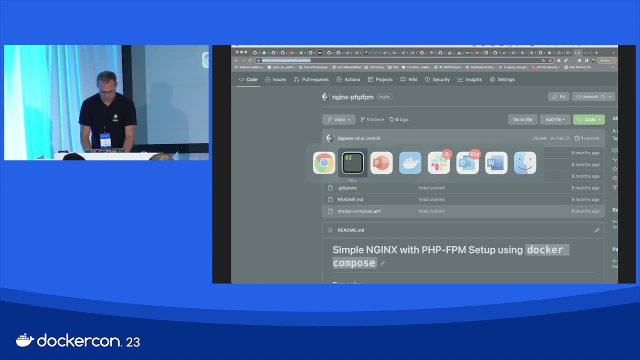 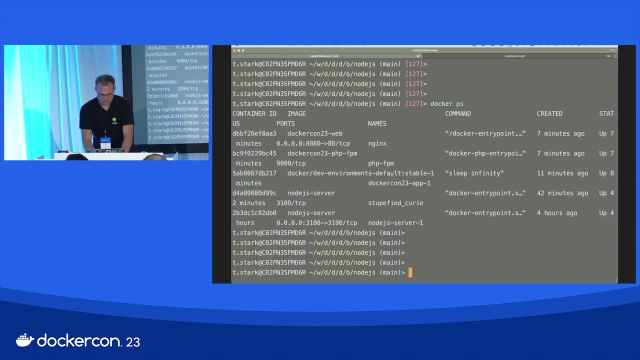 I'm doing here. actually, It would be good to have like MariaDB and phpMyAdmin So I can show you how to set up a database and using phpMyAdmin to do this. So that would be MariaDB and phpMyAdmin. 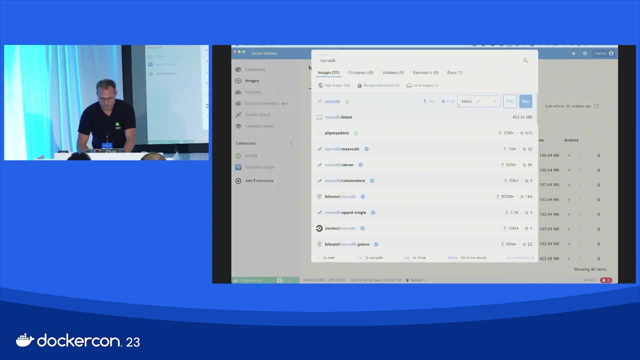 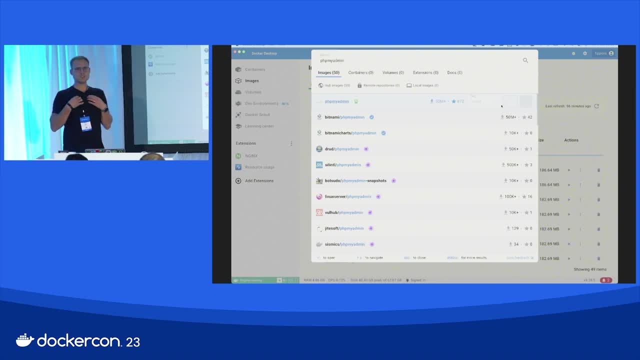 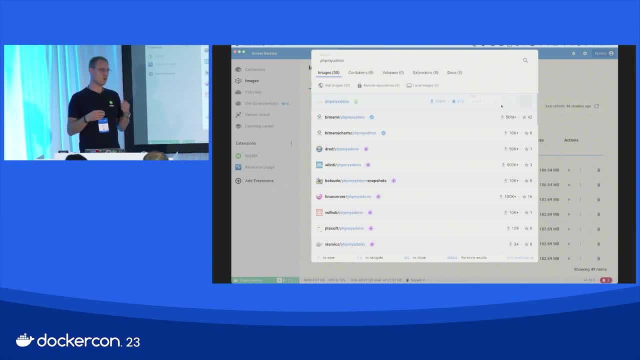 You just pull down the container And to me it doesn't really matter, even if I work for NGINX, if there's an Apache web server in it or not, I don't care. I need php. I don't care about the web server it's using. 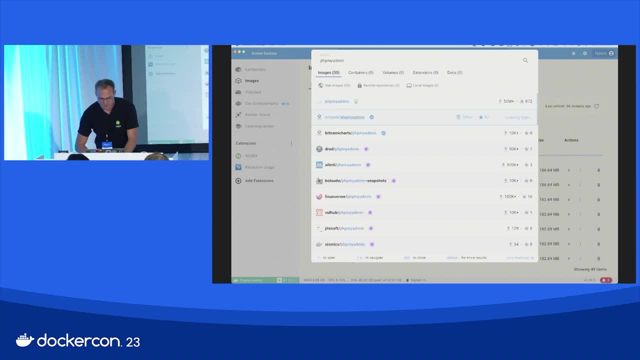 So to me it's just pulling down, use it and that's it. But if not, I will share everything we are doing. here is something I will push to a GitHub repository. It's not there yet, because if we have some other things you would like to do and then 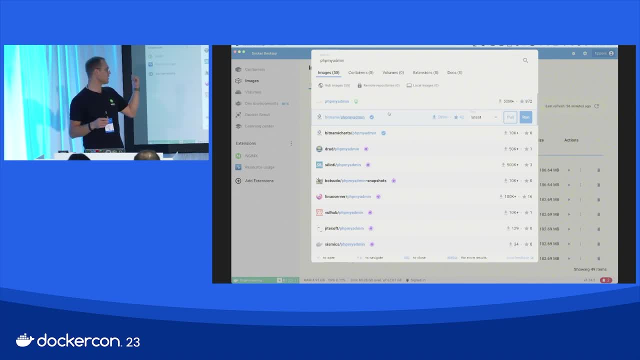 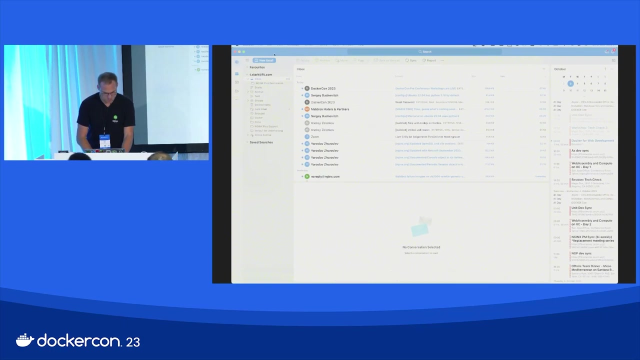 I can put everything in and just push it after the thing, and then you will get the link. So if you want to do this at home, no worries, Then we do the break. I'm working on a course guide. Just started with it yesterday. 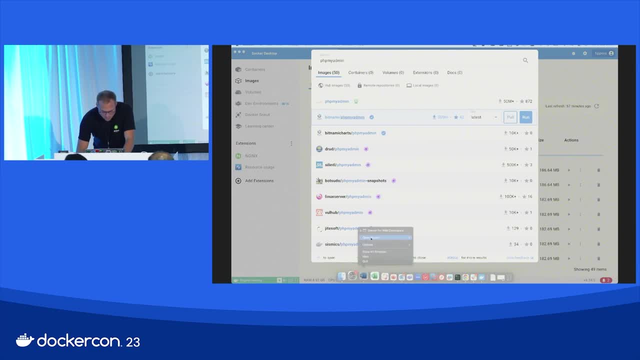 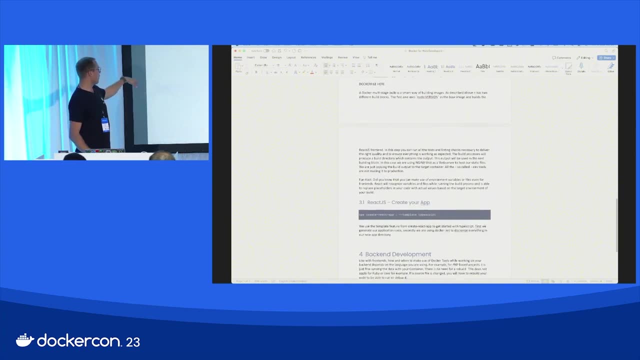 Where is it Here? So we'll work on this And this will have all the things we are basically doing in it as well. It's just not done yet, Just started on yesterday, But if you think that's helpful, I will just. 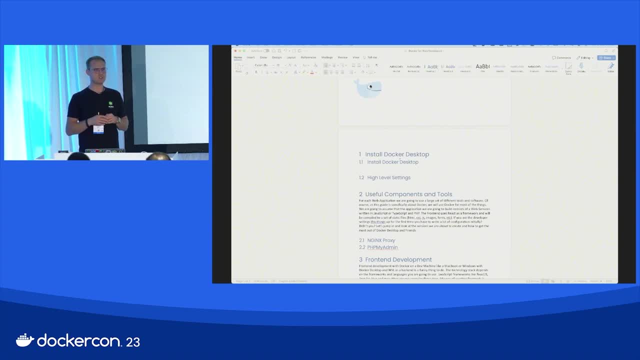 Just put everything we do in a PDF and just drop it after the conference. Then you will see it in the GitHub repository and then you can just pull it down and it has all the stuff in it. Okay, Perfect, All right, Now we do the break. 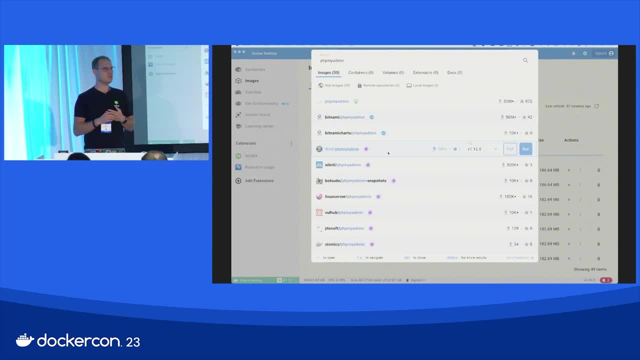 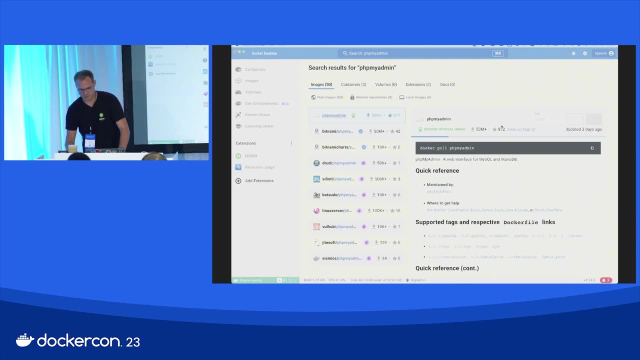 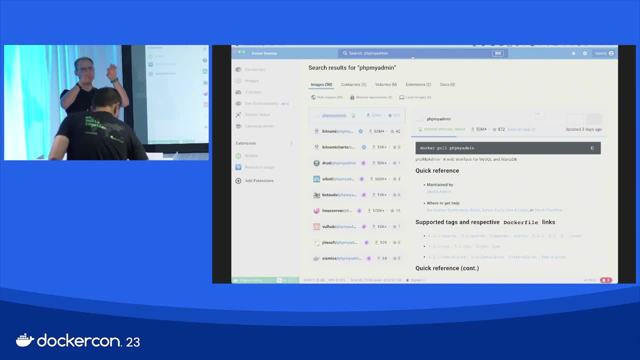 rm. but how much is it? $ proud? great, OK, OK, OK, Eh, all right, You can use it a bit more. when you can use the official one like official is, then the official PHP is a tag of PHP, So you type you. that's sometimes a little bit weird. 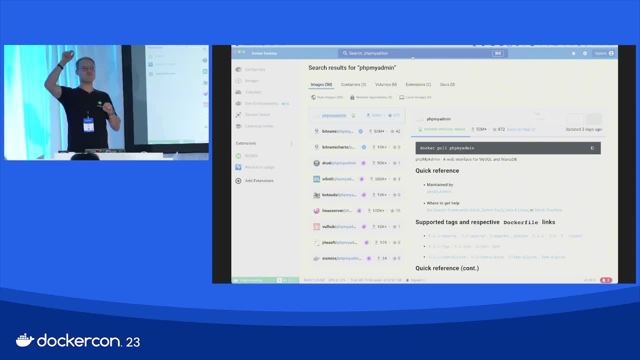 If you search for PHP-FPM, you will not find the PHP one because it's a tag. You have to search for PHP Uh-huh, And then you can find the FPM as a specific tag in this fpm. Is there something else? you need more. 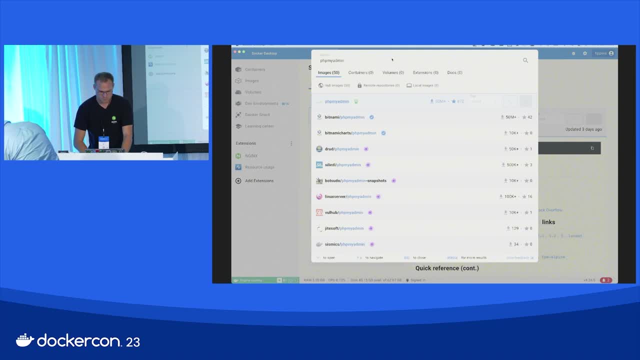 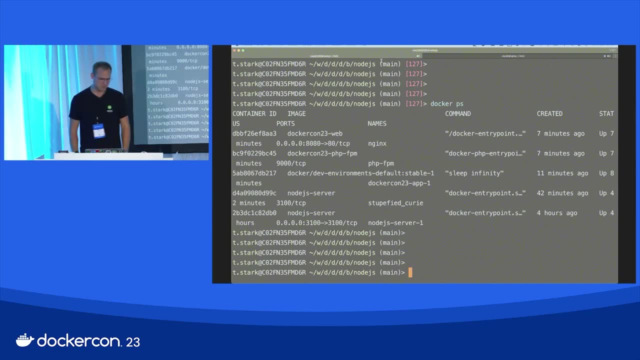 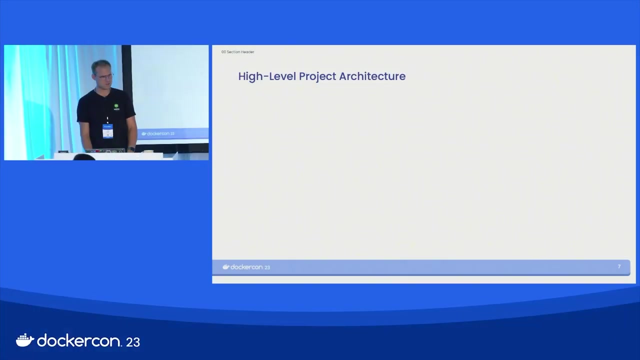 in this PHP image, but I said if we have trouble I'm downloading it, I will make. let me make some notes at this on the side. next time we do this workshop I will let you know before what images we are going to use. good, so high-level project. architecture of a common web development project. 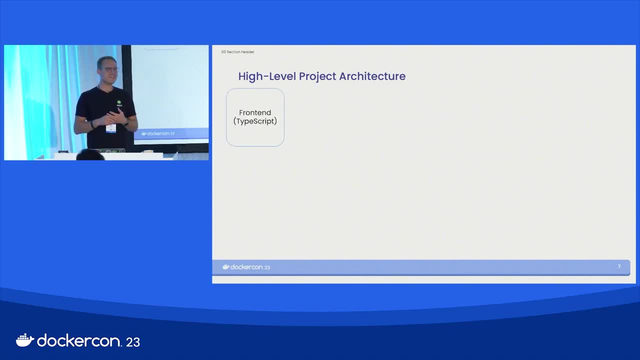 we have some content. it can be integrated in the backend language, like PHP or Ruby rails something, but in many cases, like today, it is something like react or view or angular or it, kind of a front-end framework that then you're that you're using, so you have a it's decoupled from your API. this is where 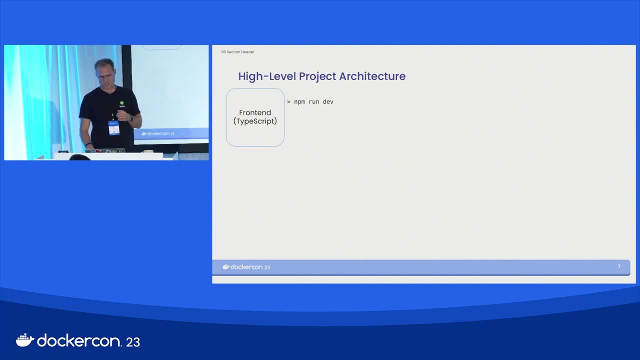 the course problematic comes into play. them right, so we can start this and we'll do this. we can do this npm run death thing. we can do npm build to build all this kind of things. npm is the node package manager. we will use this. so now we have sorry. 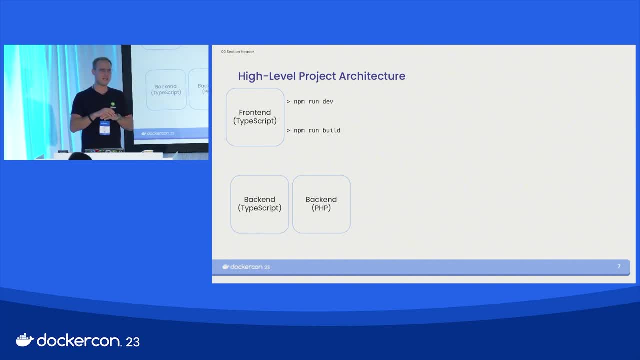 we have the back end, and the back end can be in like all the different languages you can think of. it doesn't really matter what language you're. you're using can be Ruby or PHP or TypeScript, which is like JavaScript- it's not JavaScript, it's, but it's come, it's, it's well, it's well. 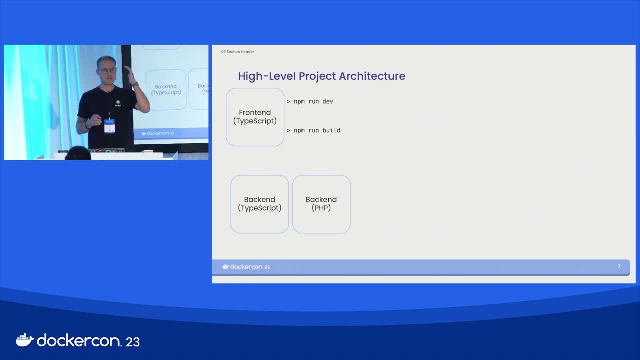 fitted into this, this JavaScript ecosystem. it can be a rust API like word, Kotlin, Java API, whatever, it doesn't really matter, I love it. I love typescript. if I'm, all my projects are using typescript. when I, when I do anything, even in the front end side, I'm always using typescript. 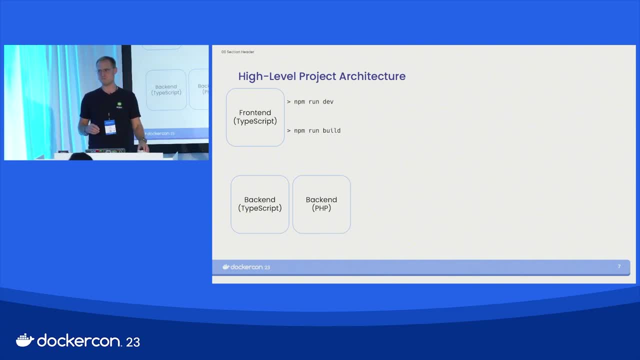 that's like, even if it's if it, if it hurts sometimes because of all the interfaces and types, I mean it's not like JavaScript. you cannot say, hey, either I have a class or an in. like JavaScript doesn't matter if it's an integer or a. 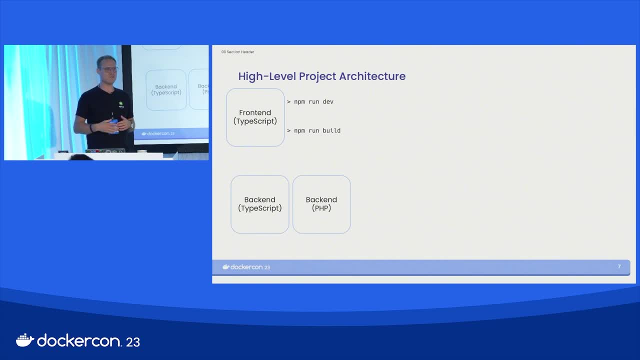 string or an array or an object. it doesn't really matter. if you have a property in the class that's called something. you can put really literally something in it. JavaScript don't care about it, it's, it's fine. and in TypeScript you have to to basically describe: hey, I have an interface, I have a class, an interface and I have 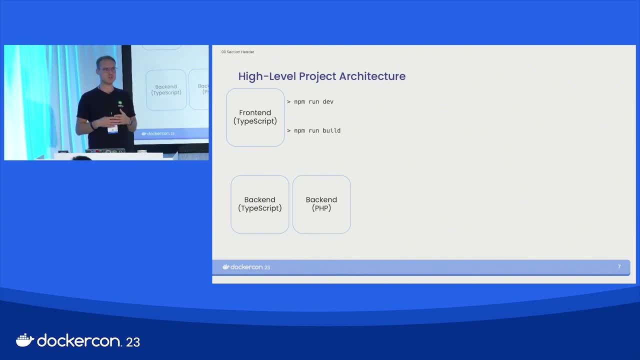 like a couple of fields, and if this field is an integer or a number and you try to put an object in it, it will scream and cry and say, hey, this does not work, This will not work. Define it right. So yeah, But I love this TypeScript feeling And we will. 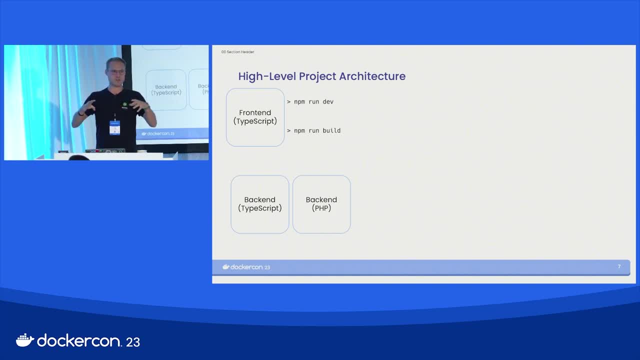 see some. I have some stuff not really prepared, but I have some thoughts about how I'm always creating TypeScript projects for Reactjs, for example, and how the directory structure look like and how to interact with different services And if you're all interested in. 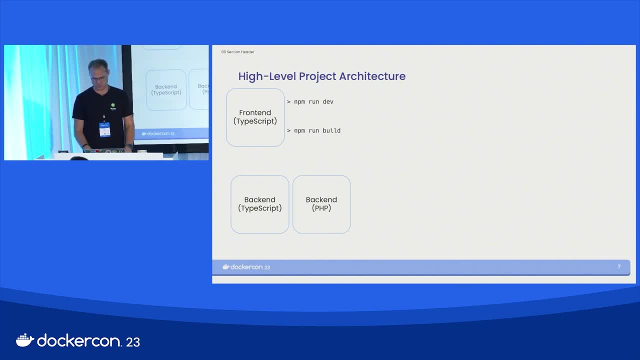 seeing this. I'm more than happy to share that. So, all prepared, we can see that. Good, The backend can be TypeScript or PHP. In this case, we're doing a Nodejs backend and a PHP backend. So, and then this is what you have on your laptop most of the time. You have something. 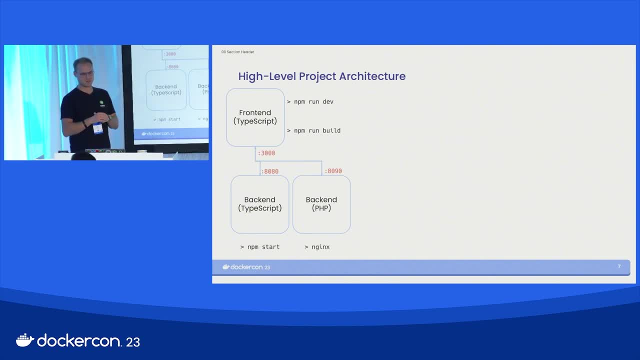 that listens on port 3000, and then you have something that listens on port 8080, and something that listens on port 8090.. But just the backend and just PHP and just TypeScript isn't good enough, right? We have a bunch of other stuff. We have a database somewhere. It can be MariaDB. 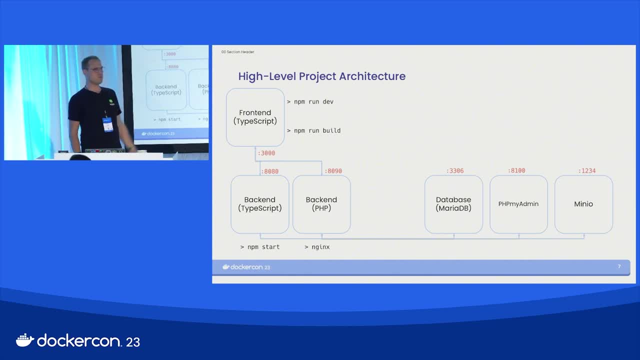 or it can be Postgres. Sometimes you have one service that uses Postgres and you have another one that uses MariaDB, And then you have another one that uses Postgres and you have another one that uses MariaDB. Awesome, Great, Excellent. So we have Postgres and 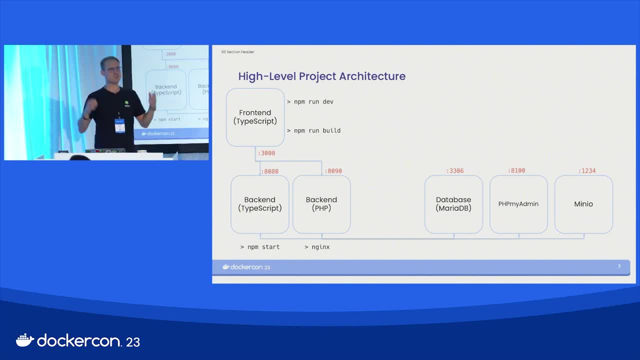 MariaDB on your system, And then we need something to administrate the databases, even on our development machine, PHP, my admin pgadmin, Or you use some tools like the MySQL workbench or something. There are some slight differences like what you want to use to administrate. 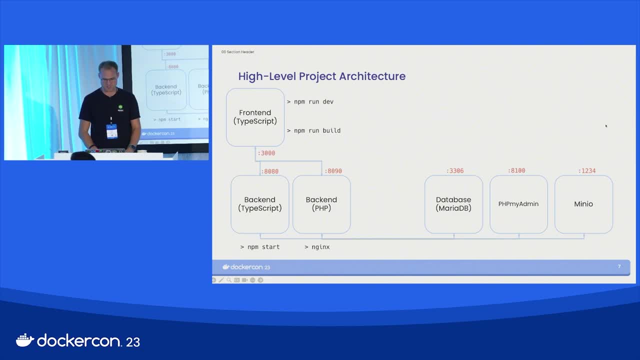 your database when it comes to setting up all these things here, and Minio is, for example, a nice little object store that is compatible with AWS S3,, for example. So if you have an API or if you have services, 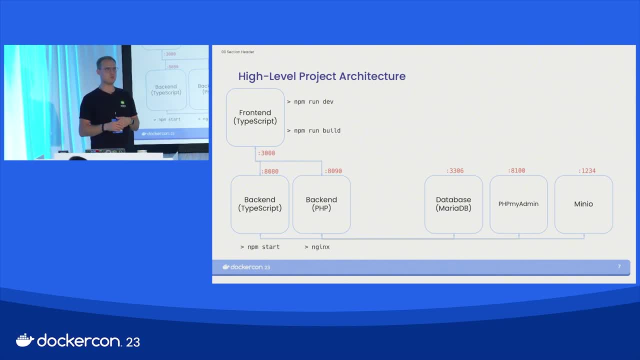 that normally would dump data to AWS S3 and you would like to do this on your system without dealing with AWS S3 while development. then you can use Minio. That's basically what I'm doing all the time. So From MongoDB there is something that is called. 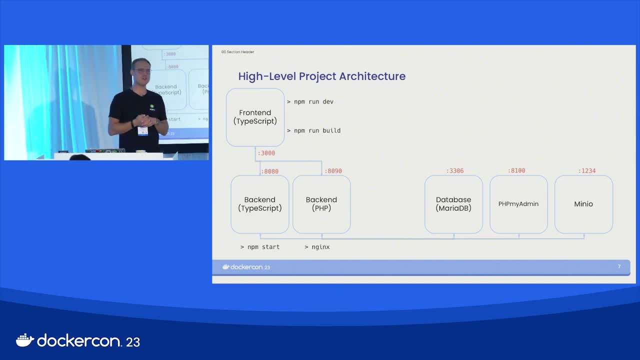 That's not advertising, by the way. That's just what I do. There's something like NoSQL Editor. NoSQL Editor is like a little green leaf. I use that. It's no advertising. Use whatever you want, But that's what I'm using. 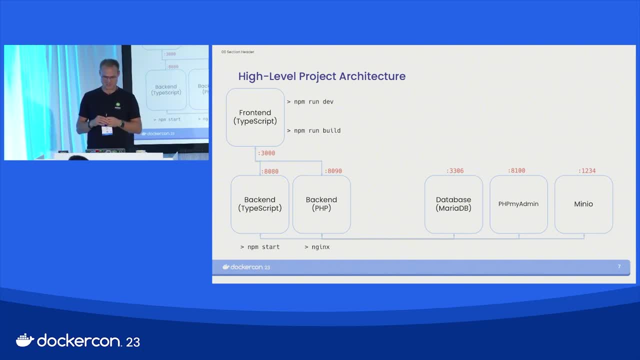 I love it, So it's called NoSQL Editor. Actually, I found a CVE by them, so I got a premium license for free. I was still using that one. So look for CVEs and then you'll get a lifetime license for free. 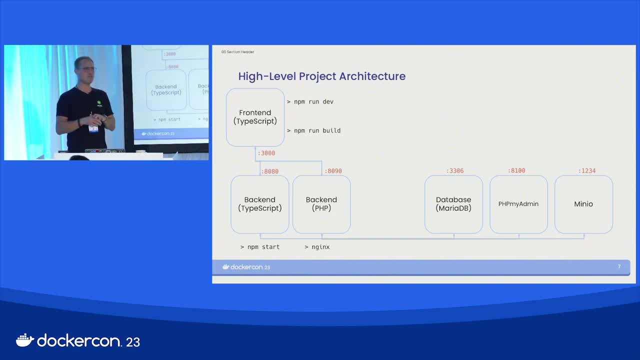 All right, Good. Yeah, MongoDB is another good example. I'm using MongoDB in some of my Java projects and, as you can see, the reason why I put this on the slide- and this is one of the view slides I have- 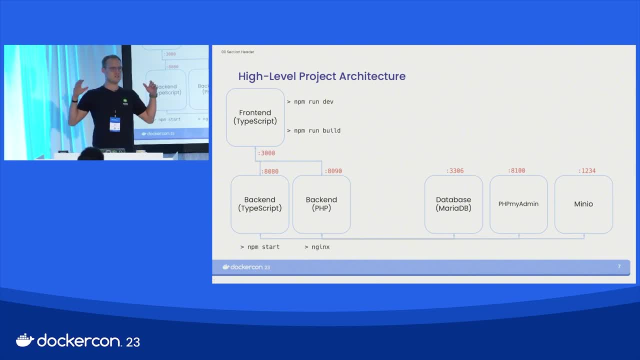 like not many more, is because the stack can be very complex very soon, even for small projects, Because what is a small project? Is it two or three different services, And you will likely have two or three different services today: Mongo, MariaDB, Postgres, Minio. 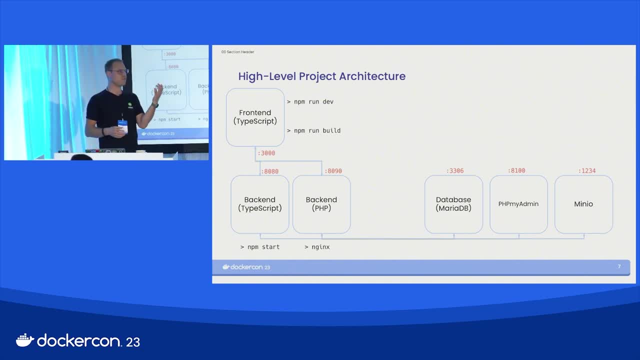 maybe Redis for caching some things. So that means you have at least five things- call it things or containers or whatever that's needed before you even start writing a single line of code, right? So this is why we are here, because I would like to teach you. 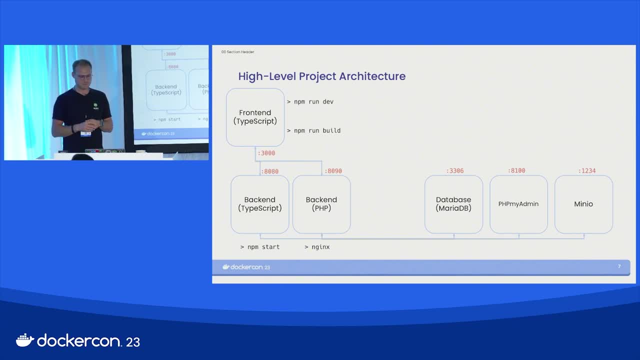 or show you how I manage this stuff efficiently. All right, So then this is my favorite thing: always Love it. You do development locally and you use it in your Nodejs or in your React applications. You use an API that is a localhost port 8080,. 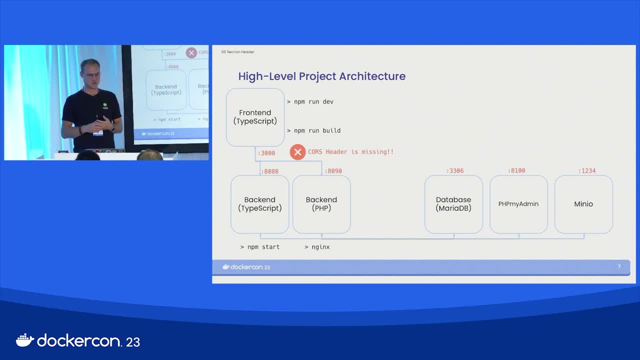 and the first thing the browser is doing is saying: hey, this is not working because there is no course heading. I don't care, It's localhost, I don't care, So So Right, Good, Okay, So what is course? 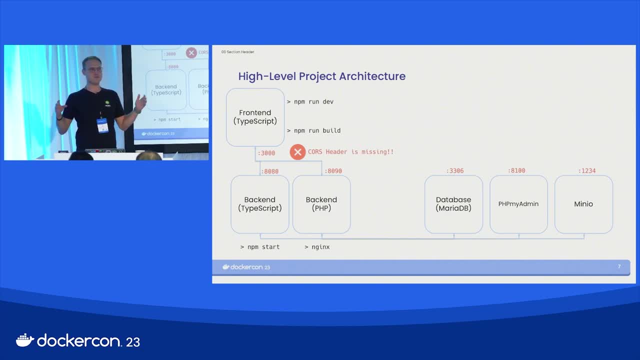 Is it fine if we talk two minutes about this? everybody's darling. Okay, good, What is course? Cross-origin resource sharing is the long version of what course does. what does it mean? And it's like the browser checks if an API or a resource 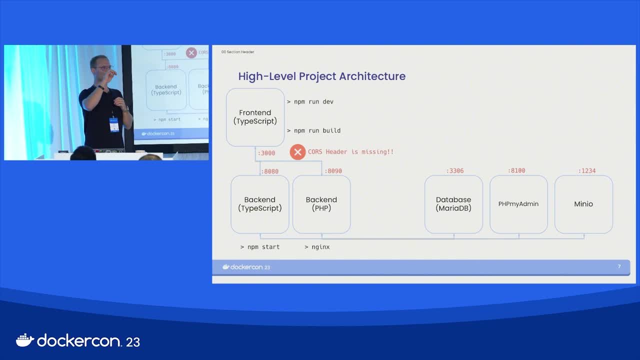 that is not your origin. What is the origin Origin in this case? if our front-end front-end runs on localhost port 3000, this is our origin. like our home, This is where we live currently with our application Good. 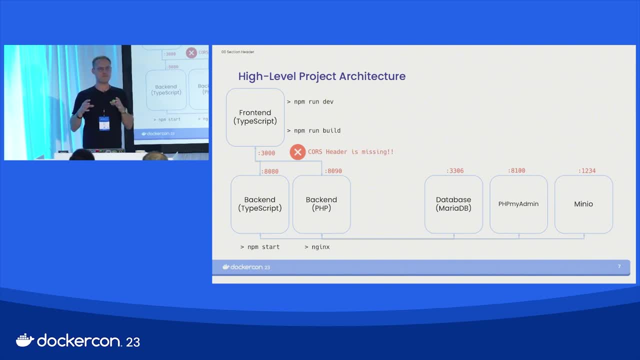 If we try to call consume data from another origin, localhost port 8080 is another origin. That's important. It's another origin because the port is different. It's another origin, So the browser requests a resource that is hosted on localhost port 8000. 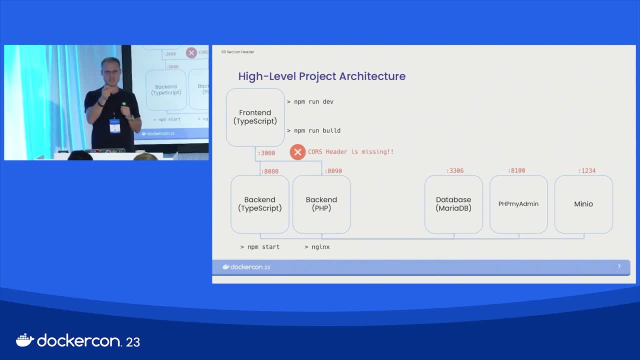 or 8080. And what the browser will do in this case. because you do the call from JavaScript or TypeScript from your React project, you're not using the browser to navigate in a new tab to localhost port 8080. And this is a common mistake. 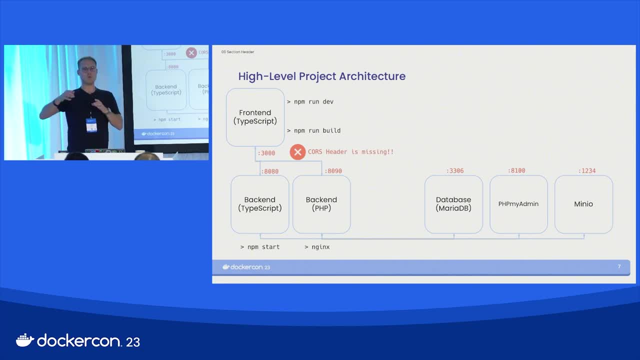 If you do a browser tab, a new browser tab, and do localhost port 8080, it will work. It will show you the JSON output. Why not? I mean you're navigating to this endpoint, That's totally fair. But if you do the same thing from inside of your React app, 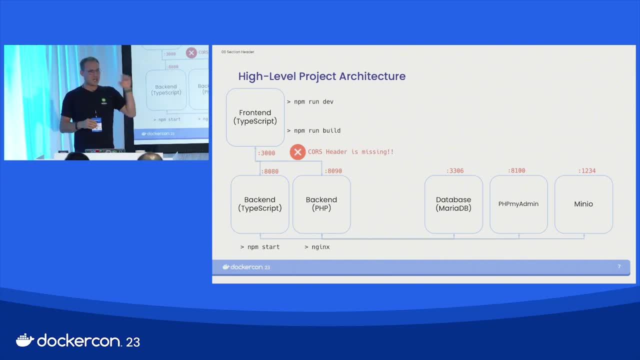 and we will do this here. it will tell you I cannot get the data from localhost port 8080 because this cross-domain allow origin headers thing is missing, And that is because it's the browser tries to prevent resources, in this case our frontend, to get information. 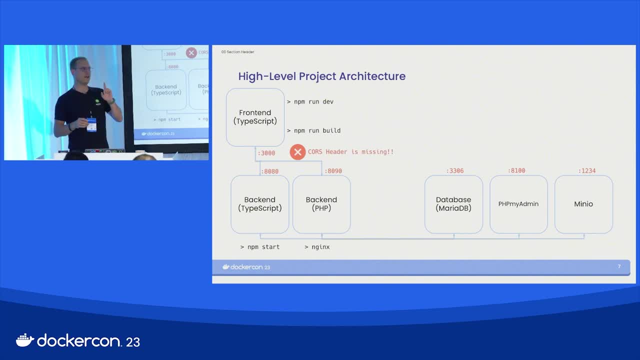 they are not authorized to get. And this is the thing. And I remember I was working almost 10 years for a German car manufacturer and remember I explained that in a meeting because they added course headers everywhere, not kidding everywhere, because they literally did not understand how that works. 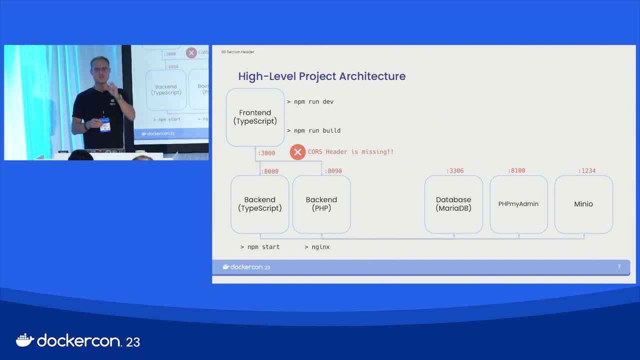 They added everywhere a course header. I was like: look, this will not work, because the point or the place where you have to add the course headers is on the backend API. You don't have to set a course header for your frontend. The frontend literally don't care about a course header. 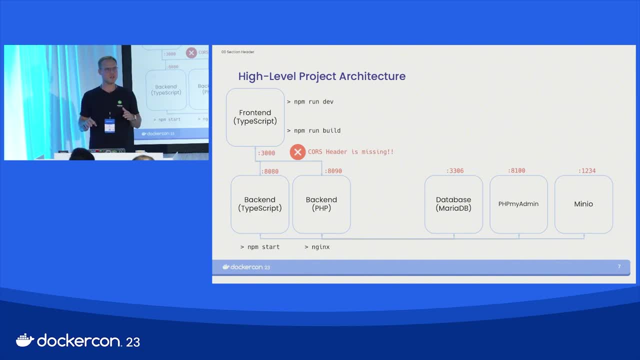 That's totally. that's not the right place to set, because the frontend calls your backend API and because of this cross-origin sharing, the browser says, hey, do you even have permission to get this resource from this other region? So let me tell or ask this origin localhost, port 8080,. 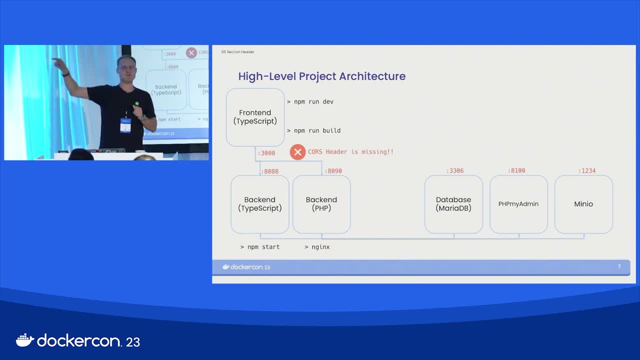 if you have permission to get those data. So it will ask your API: hey, do you want that this frontend is displaying your data? And if the API says, oh fine, do it send it. then you will see it. 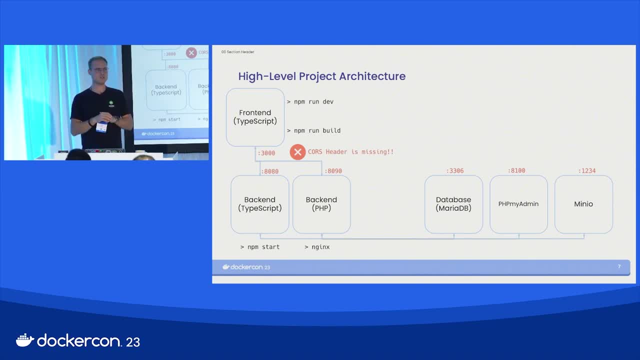 You will see the data. The frontend doesn't care, right. So this is where to put the course headers. It's on the API side, It's on your backend side, It's not on the frontend, So don't put them everywhere, right? 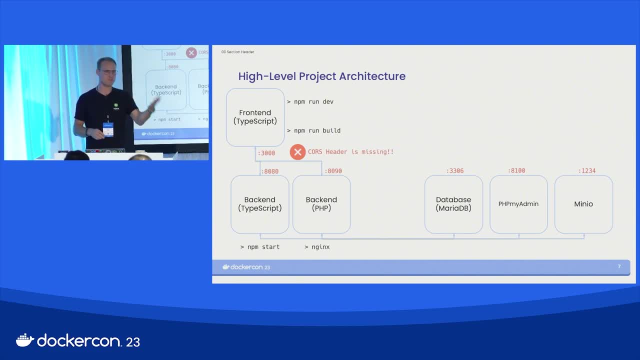 And we can do some course juggling later, like what does star mean? What is a? and I have a nice trick. I think it's one of my production services, So maybe I have to drop screen sharing for a little minute. And then, because I have a nice little trick, 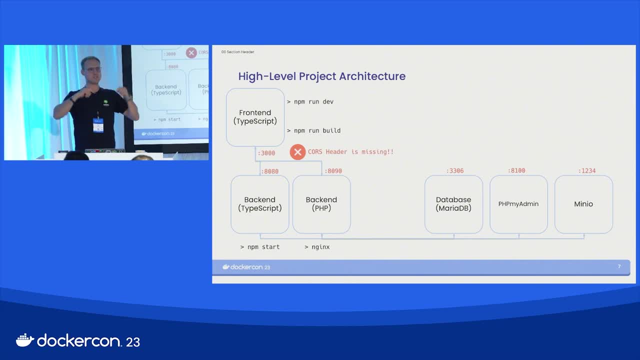 how to do this, like course, headers with different host names, because you cannot put in this cross allow origin header. you can put star in it or you can put a domain name in it, but you cannot put a list of domain names in it. 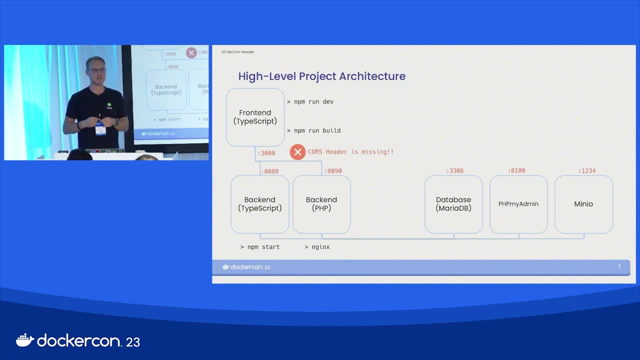 But I have NGINX configuration that gets the domain name dynamically and then puts always the right domain name in it. So, just so, I think I can share this one with you. Okay, so we have the course headers even locally. That's where the proxy comes into play. 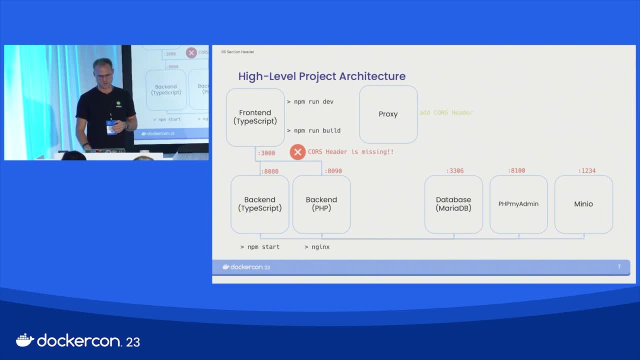 even on your local machine, because you don't want to have this course errors. Then you add the course headers, then you remove this, you wire things a little bit different. So then you have this, You have NPM, that your local front end. 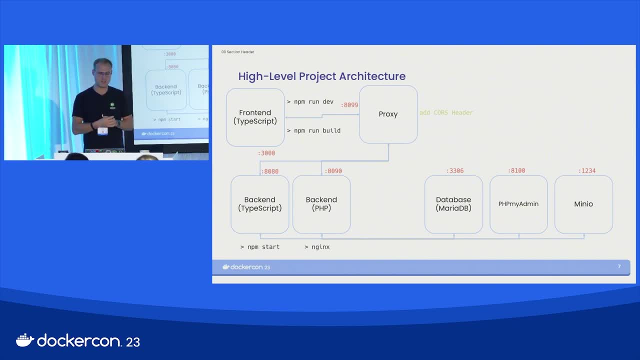 is talking to your proxy server, which is hopefully NGINX on your local machine, And then this will proxy to the different Docker containers on port 80,, 80,, 80,, 90, and add some course headers And you don't have to like. 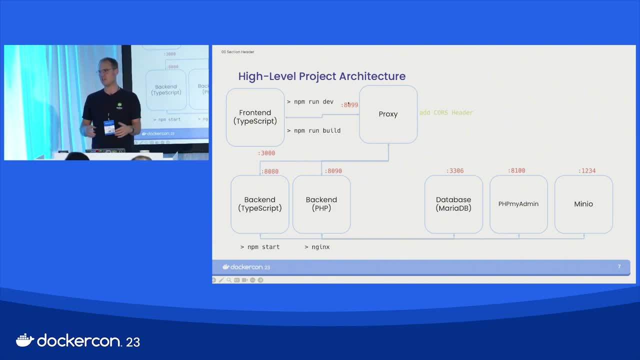 you can even have NGINX listen on port 80,, 91,, 80,, 92, and then proxy to your containers as well. And this is again where the Docker desktop extension comes in handy. because- let me show you this real quick- 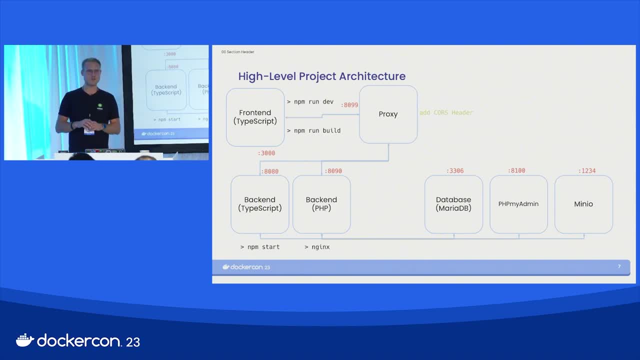 Is this proxy the same as a reverse? Yes, that's literally a reverse proxy, Getting you know like it accepts traffic on a given port, knows what to do with it and just sends it to the upstream. That's basically what it does. 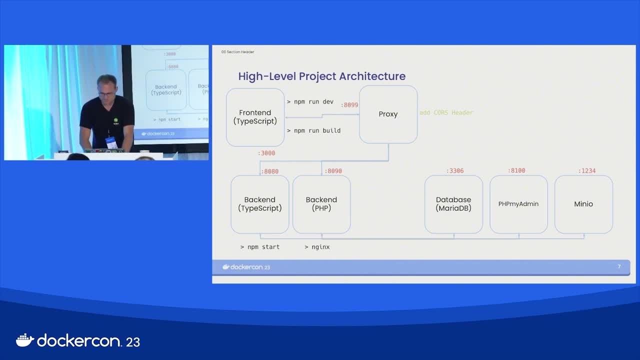 So the good thing is with the Docker desktop extension, let me see: Yeah, I have this. oh, where do I have it? I think it's here Because in the Docker desktop extension. I'll show you that in a minute. 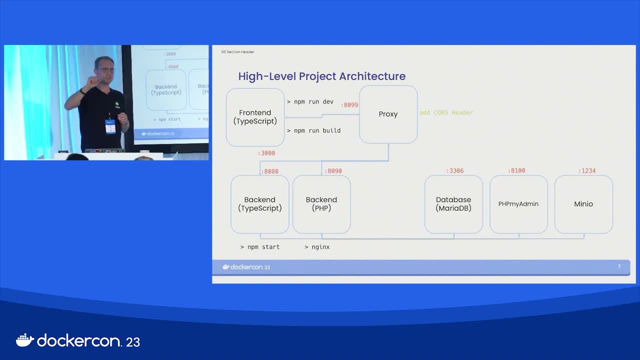 It knows what other containers, with which, with what ports, are in the same network, And then you can select them when you're creating a new configuration. basically, So you only have to have the cores other than the proxy, not to follow the backend server. 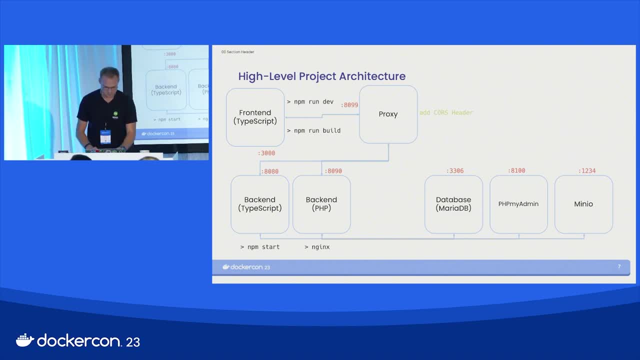 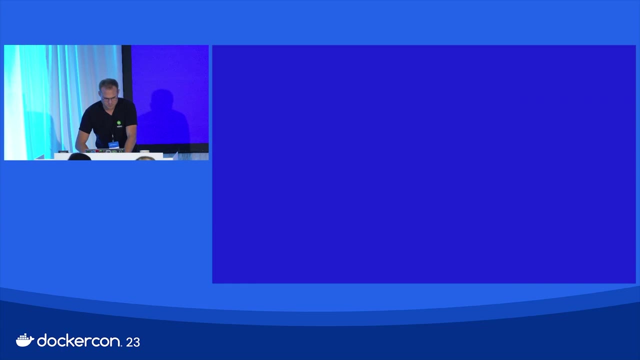 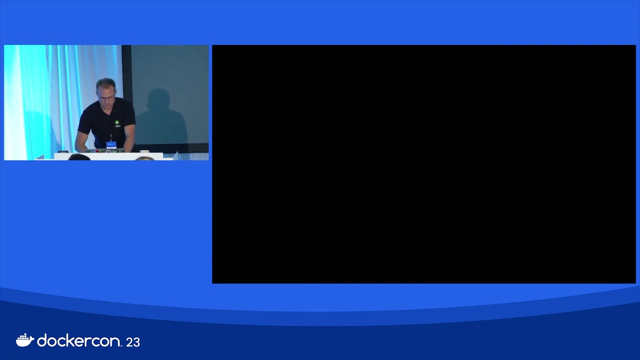 Just the proxy. Proxy is dealing with the cores, then, And we can do that in a minute. So, And this is Docker Compose Watch. That's for later, Good, So now the components we are trying to set up. this is something we already we already saw, basically. 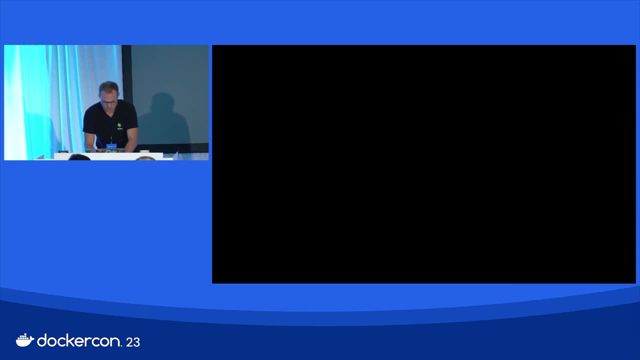 And now I will show you something. Yes, All right. So this is a real project I don't like to get like to create. No, that's not a real project, That's just a black screen. That's interesting. 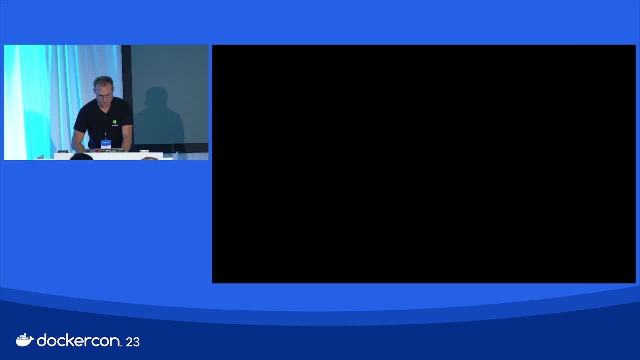 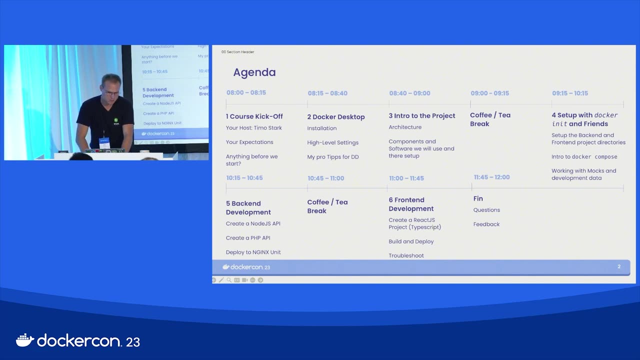 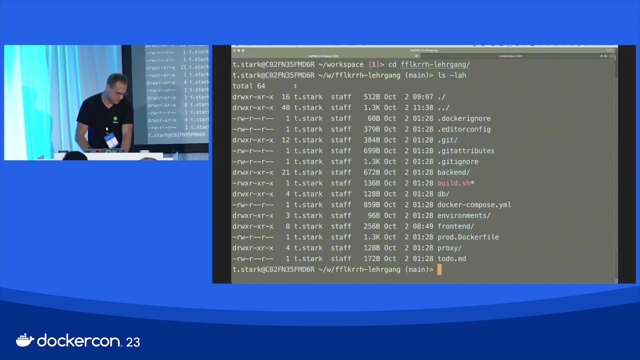 Let me do, let me try, If it okay. Now I'm presenting mode in PowerPoint again. Let's see: Yes, Okay, Now I hit and exit. Let's see Yes, Yes, Okay, Perfect, It was just too too fast. 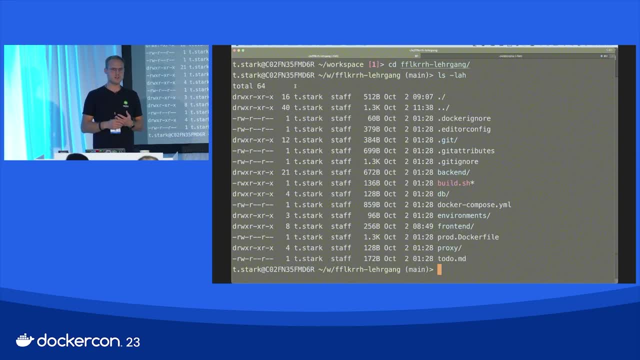 Okay, So this is a real project I'm working on, Like something that you can use to book courses for the fire departments in the city where I live. You can book courses And they did that manually And they asked me a couple of months ago. 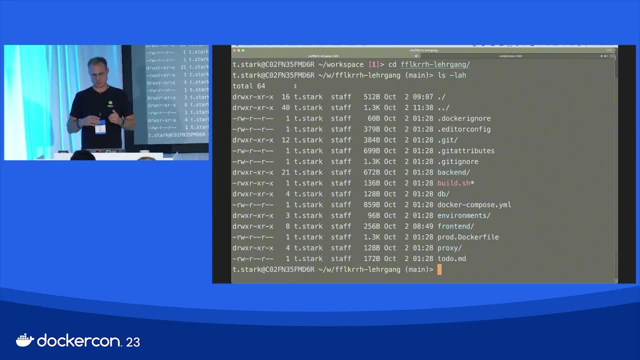 hey, can you create a website for this? Yes, of course I can, And this is the project. So real project. So it's not a demo thing, It's a real project. So we use this as a reference, because I don't see a reason. 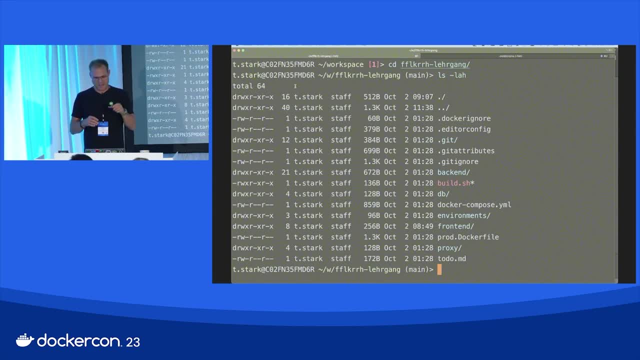 why to create a thing? Or I have created the same directory structure. Now we can move parts into this directory structure, Then we can push it on GitHub so you can download it, because this is a private project. It's not even public the source code. 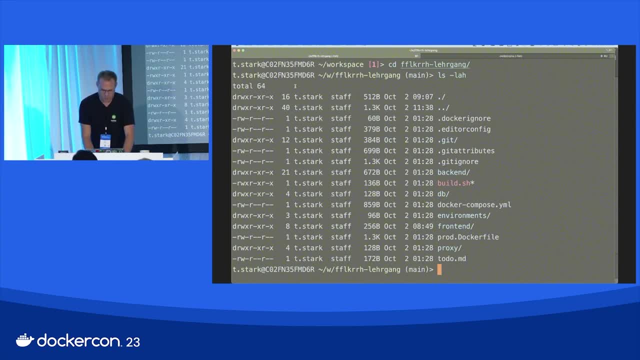 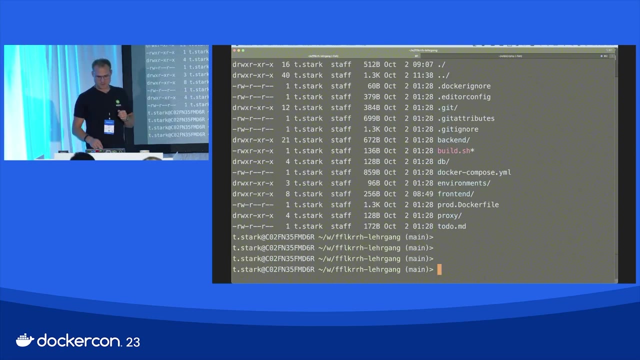 So it's like, yeah, closed source, So I will copy what we need. So, but you see this directory structure. We have a backend directory, We have a DB, We have frontend, We have proxy. I like this directory structure because of a given reason. 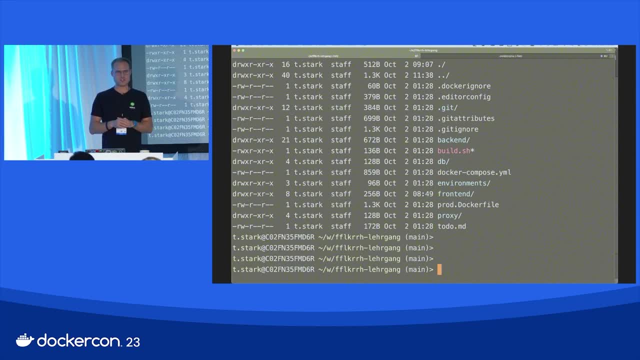 And this is where Docker Compose comes into play. Let's imagine you start a new project and you own the whole project, Like you do the frontend. In this case, I own the whole project. I do the frontend and the backend and the database. 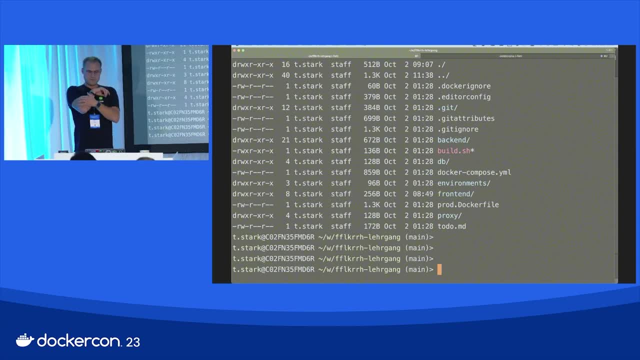 and the proxy and everything. But then I can push it to Git. OK, so we have a Git repository that has all the different things in it, like the backend or the frontend. Good, With this structure we can easily say today or tomorrow or next year, somebody is taking care. 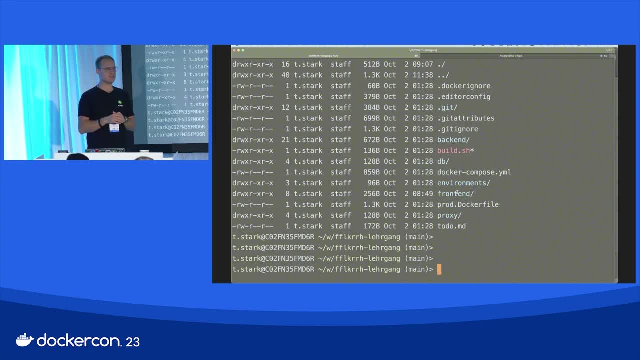 of the backend. I'm not doing it anymore because somebody else is writing the backend code for me, which is fine. What I can do is I can get this backend code and just move into a completely different GitHub repository and use something on Git that's called submodules. 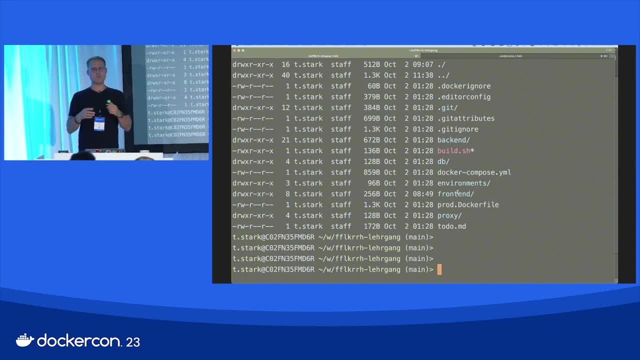 and just put it back in my GitHub repository. So what will happen is that I have one GitHub repository with all the frontend code And this has a reference to this GitHub repository. that's the backend And it's a submodule. I'm not even owning this stuff. 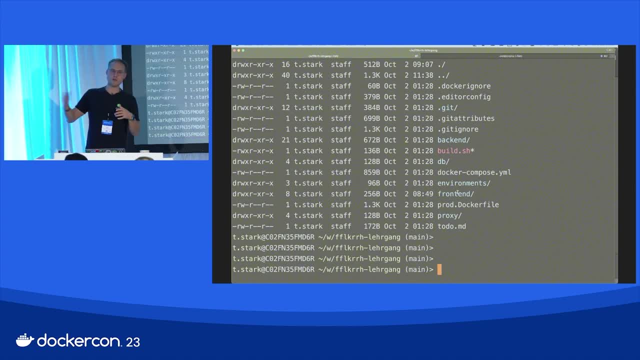 I don't own this thing anymore, But I can try Docker pull then, or clone and include all the submodules so it will get the latest version of the backend on my system without me even taking care of it. And this is where Docker Compose comes into very, very handy. 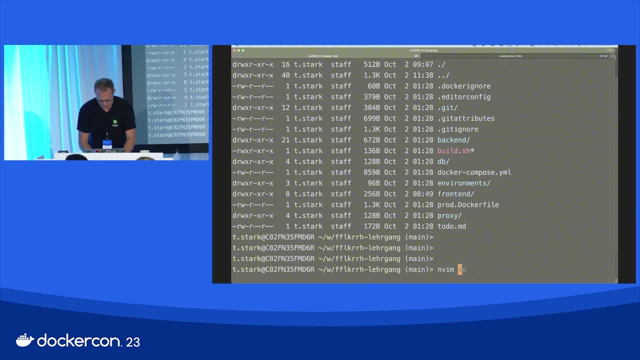 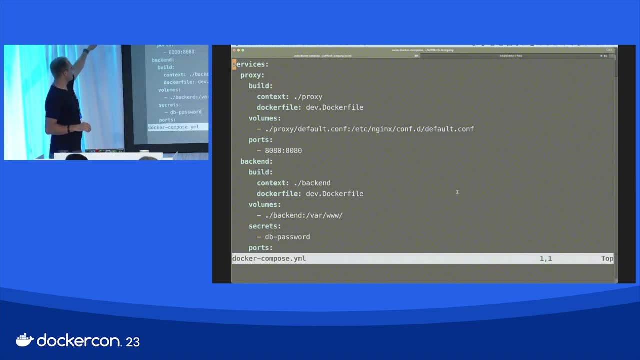 And this is what I would like to show you here. Good, So again, we have the services, We have the proxy, We have the backend. What you see here is in the proxy section we have this context that's saying: hey, 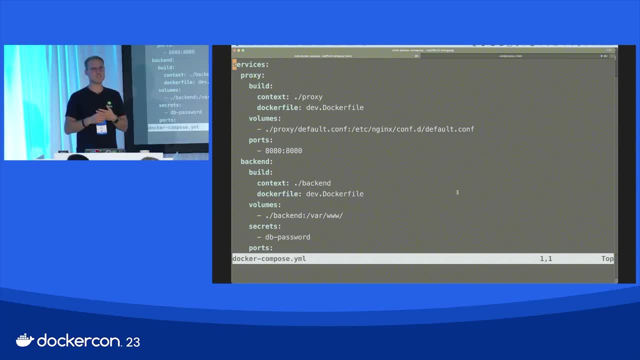 dot. slash context is proxy. Proxy is the directory name. where call this? however you want beaker or whatever. something meaningful, please, that others that are new to this project can understand. hey, what's going on? And this is the reason why I use Docker Compose file. 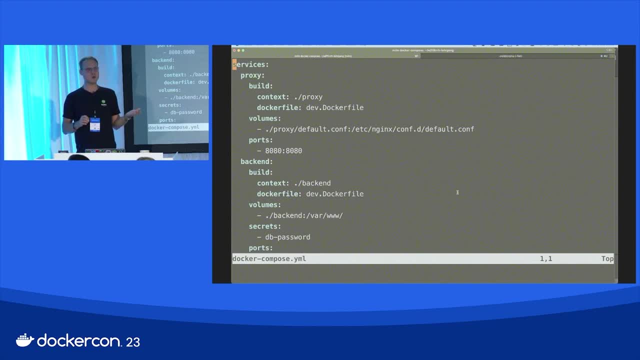 for most of my projects, because I would like to let others know how this project works, And it doesn't matter how complex it will be at the end If your Docker Compose file is structured well enough and you have these directories set up at the beginning. 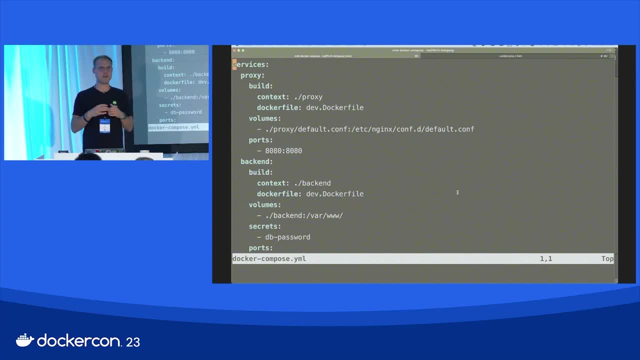 in a meaningful way. if you have multiple backends, I love to do backends plural And in backends I do Java backend, PHP backend, Node backend that people understand. hey, this is my backend, OK, fine. 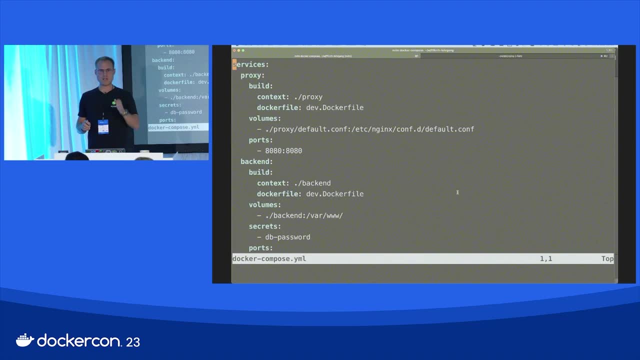 This is my frontend. In frontend, I do React. Reason why I'm doing this is because if you're new to your project and you don't know what React is, for whatever reason you have, it's unlikely, but maybe you don't know what React is. 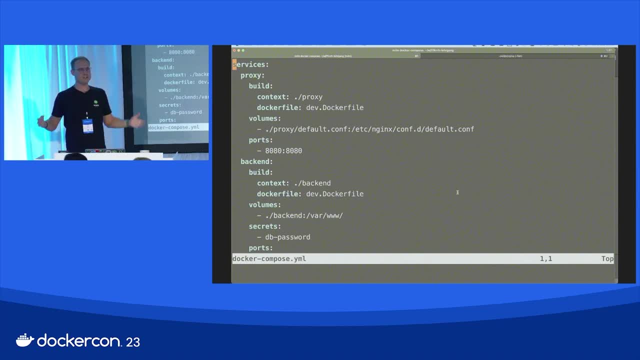 But you know what a frontend is most of the time, right. So you go to frontend and you see in this frontend directory you see something that's called React In this second you understand this React thing, whatever that is, is the frontend. 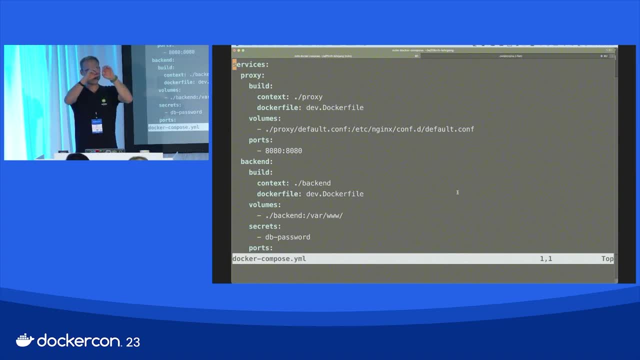 Perfect, So you can Google React frontend. You can link things logically together and understand what that is. If you are in backend, and in backend you have a service that is Nodejs API. If you just put, just imagine you have a directory. 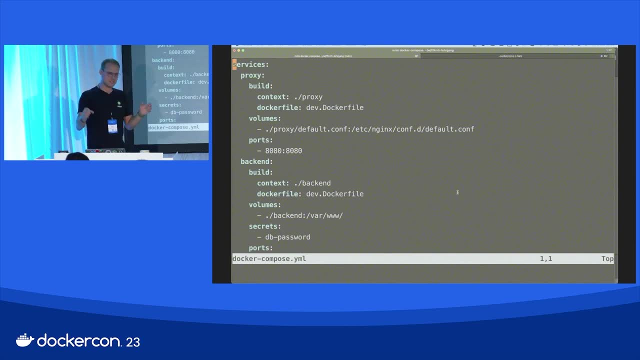 and that is frontend code somewhere. And then in the same directory you have your backend API And it's just a folder that's called Node. What does it say? Nothing. You have a very hard job finding out what is Node. What is this directory Node doing? 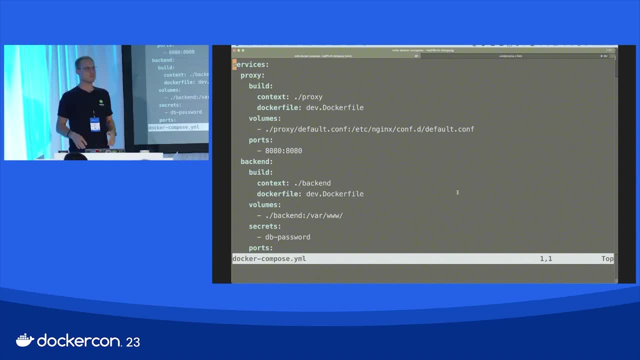 What is this? And I saw that like a million times- that just people dumping everything in a single directory And then, yeah, having trouble to linking things logically together and it's a mess. It's literally a mess. You're mixing up things and then you rename. 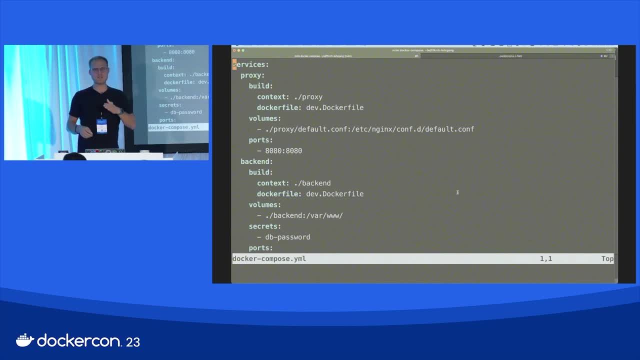 What I saw, like you have source src for the backend and then they had a source underscore frontend folder for the frontend. I mean that it becomes very messy at some point. Yeah, if you will, you can do that. 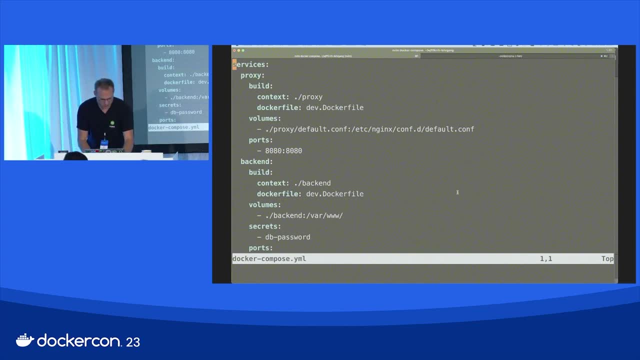 So- and this is what I have in the example- we are doing here as well- So the directory structure to me matters the most If we get started with development- and I have a good template- I should share that as well. 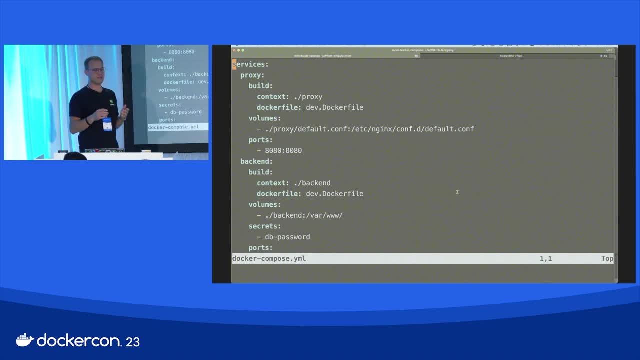 where I have this kind of directory structure created at the. it has a proxy folder, always It has a database folder, always It has a backend folder and a frontend folder or directory. So and one docker-compose file. And what does this docker-compose file do, actually? 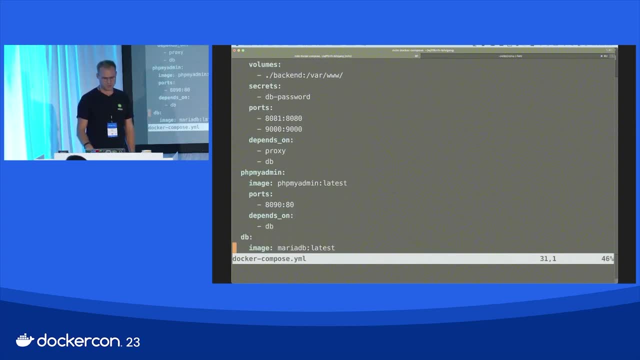 What we see here is here, for example, we have this phpMyAdmin, We have a DB, We have a couple of volumes and secrets, Perfect, And it's just for development. OK, And what matters as that most to me? 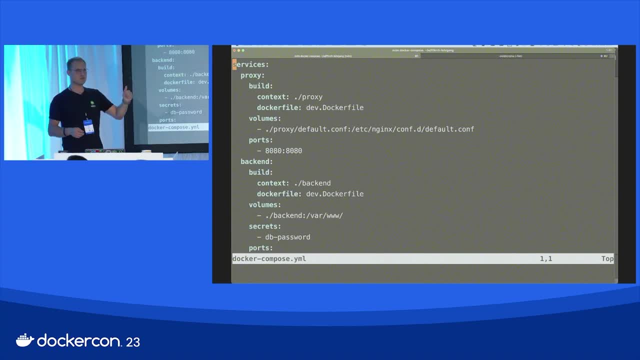 is first the directory structure. Make it meaningful, Say proxy frontend backends. Then put a lot of stuff into backends That helps people To navigate in your project and instantly understand what does it do. Second is make the compose file or the whole project. 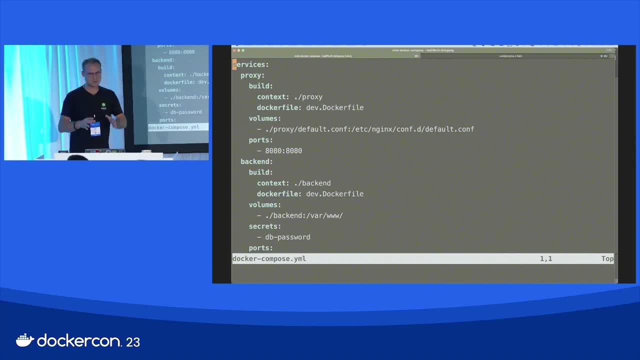 using docker-compose: self-contained. What does it mean? Show of hands: Who pulled a project from the internal or external git repository tried the build-as-h script or docker-build or docker-compose and it errored the first time because of a missing reference. 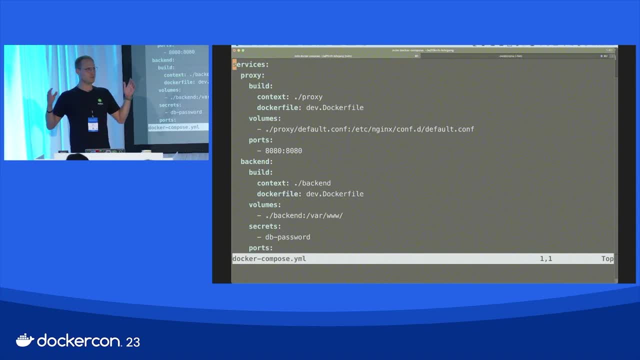 Database was empty. It was not able to build because the dependency was not there. Or it build, it started up but the frontend or the backend errored because there were no data in the database. Something like this: Right. This is not good. 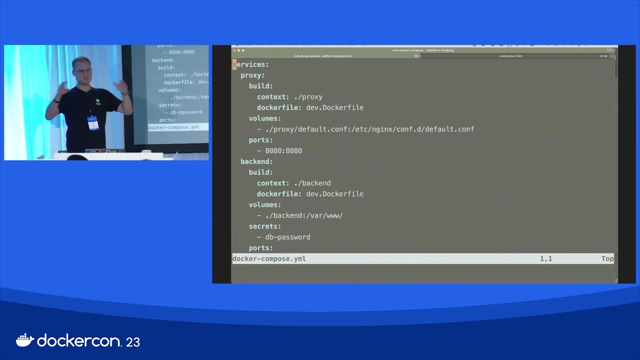 Because you're doing it. You're working on this by yourself for a couple of months and you put everything You have, for example, a database, already on your system. You have a Redis on your system, a MongoDB, It doesn't really matter. 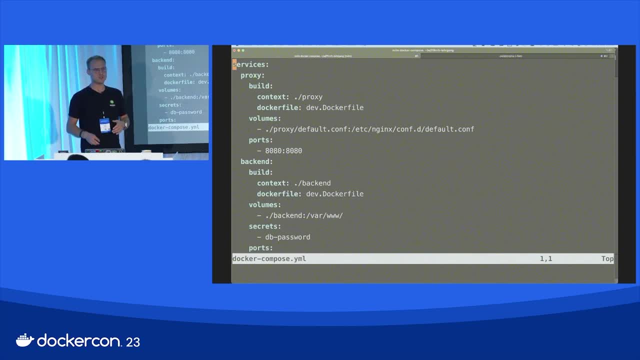 During this whole cycle of development. you put a lot of data in it. So for you it is totally fair that there is a user database table and there is a couple of data in it. It works, It just works, OK. Or you put a JSON file somewhere on your computer. 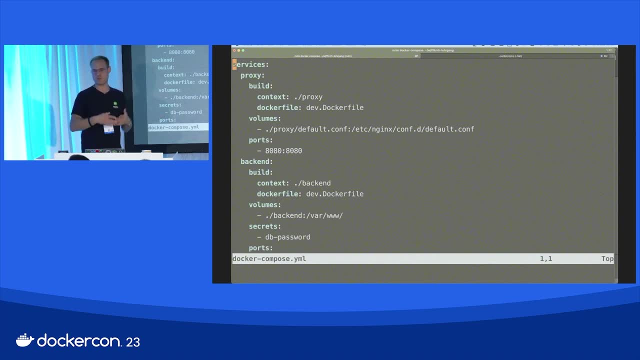 that is needed by this project, just because you know that it must be there, Perfect Good. And then another engineer tries to work on this project And the simple thing to onboard somebody is by working with the code. Reading the code is one thing. 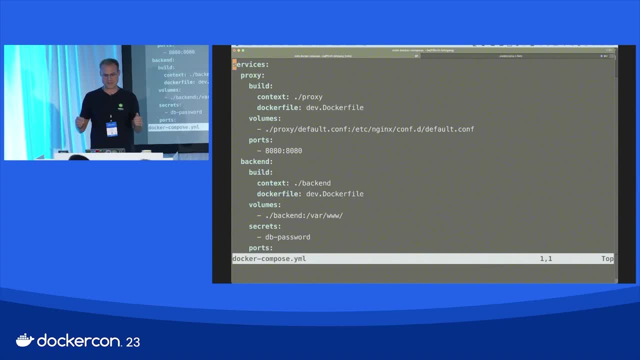 But as soon as it's very complex- and it will be very complex very fast- is you pull down the data from Git or from somewhere or from a tarball zip archive, It doesn't really matter. You have it on your system And then you can look at the code. 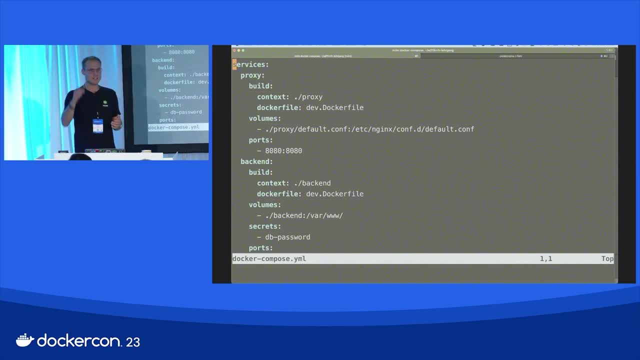 But it would be very nice if you can just run it, click through it and watch the front end. look at the front end, see how it interacts with the back end, use Postman to check the APIs and all this kind of stuff. 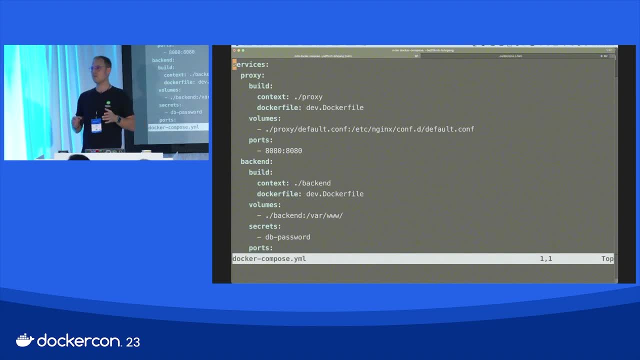 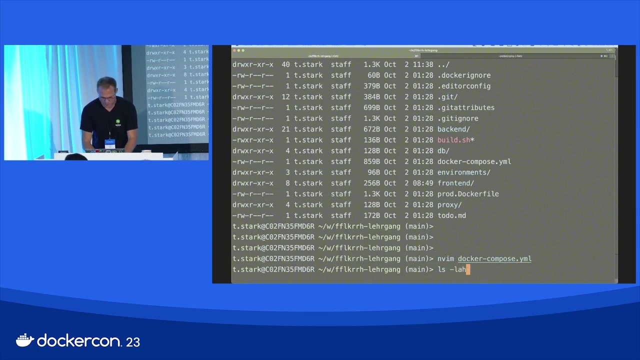 So that's what I'm saying: Make it self-contained, Push something to your Git that just works by typing docker, compose up dash dash, build. It just works, It must work. This is a must-have. If you're responsible for this, I'm calling that the level zero. 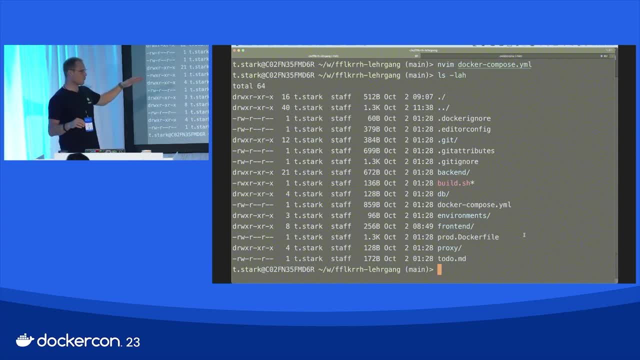 if you're responsible for this directory structure, like for the overall thing, make sure that this docker compose thing has anything in it. you need to spin up this project to run it, Everything: the database, my PHP, my admin. If you need Postgres, fine, put Postgres in. 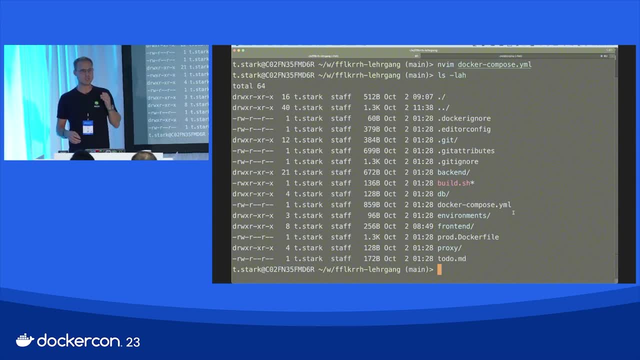 If you need MongoDB, put MongoDB in. If you need some example data, make sure that they are part of your thing here. So, for example, I have in the DB folder there's something that's called dumps. All right, excellent. And in dumps I have a SQL file that has at least the structure and the minimum set of data: default user, admin, admin, whatever. It's just for development. Don't put it with production data. of course You can dump production database and delete everything. 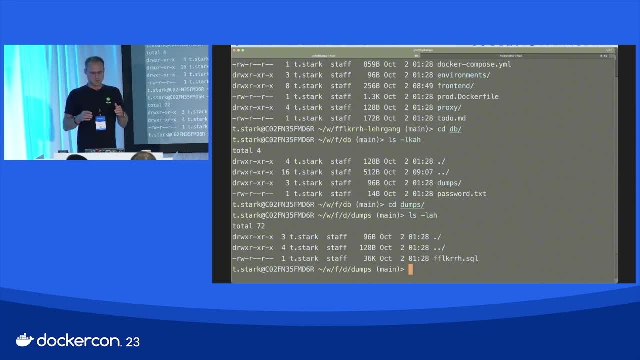 and just have some sample data in it. Perfect One thing. another option is to use some tools to generate database schemas and data while it's building. Java has- like Hibernate is a common thing where you don't have to do this database stuff by yourself. 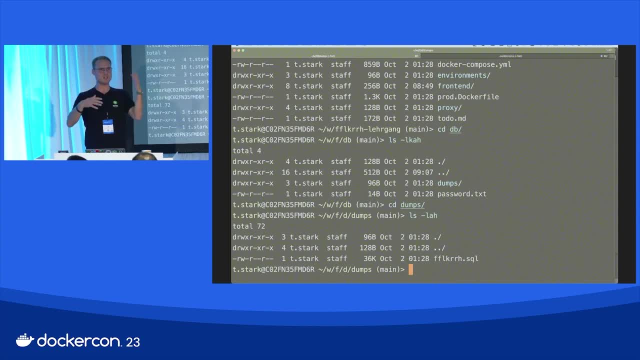 because the framework is actually talking with the database and creating schemas and inserting data. That's what I'm saying. This is not like black or white. I'm not saying you always have to put an SQL dump in your docker compose file to set up your database. no, 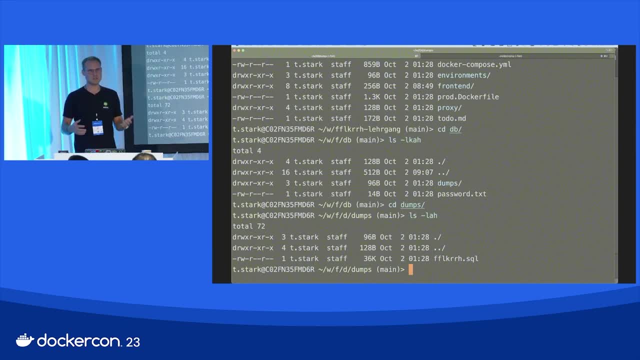 If you use something like Hibernate in Kotlin or Java or something like Ruby, Ruby on Rails has similar ideas that you describe in a file what your data or how your database should look like. then it's creating the database while it's starting up, So it detects: hey, there are unmanaged. 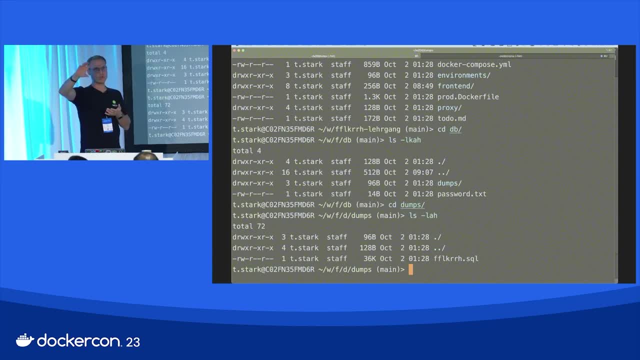 unstaged changes to the database. Yes, okay, let's do it then. Okay, But make sure that this happens, that this will be executed on startup, And this is my number one pro tip for all of you: Make sure that your docker compose setup. 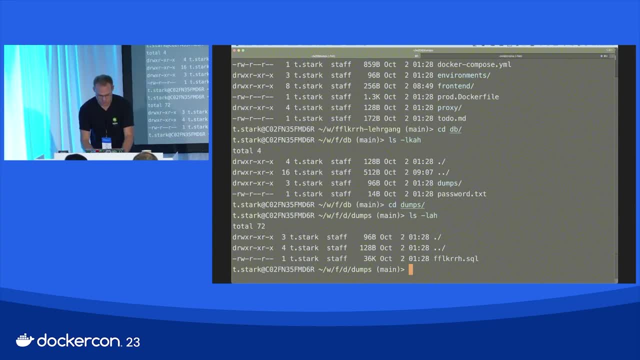 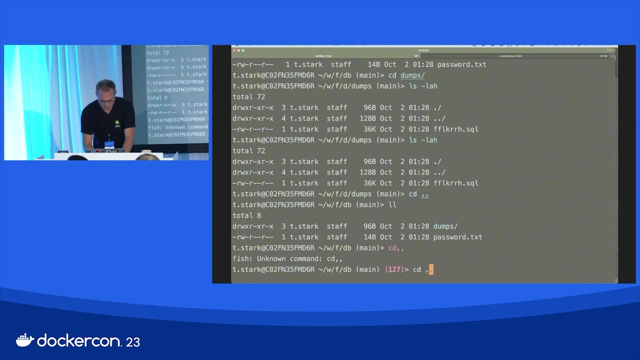 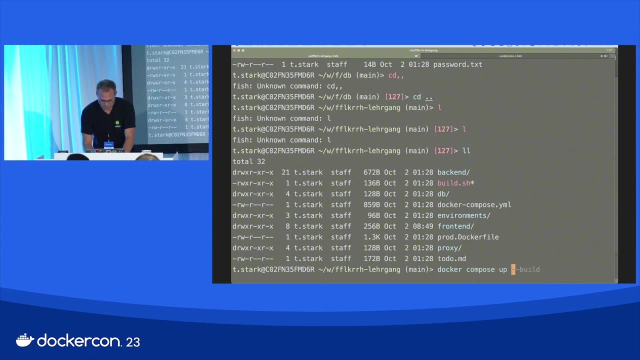 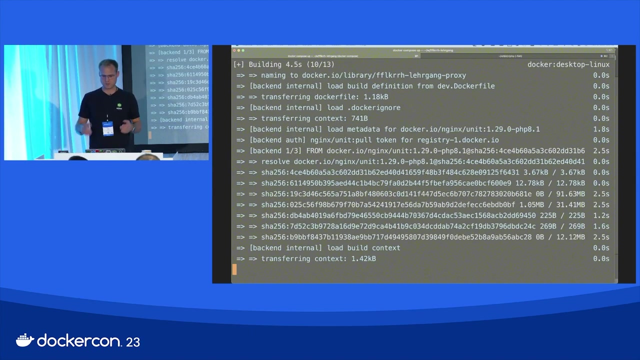 and your docker compose thing works out of the box. Let me actually see if this is working. So I'm not sure if I did some changes to this. All right, while it's pulling. this would be interesting If it fails now because of a missing dependency. 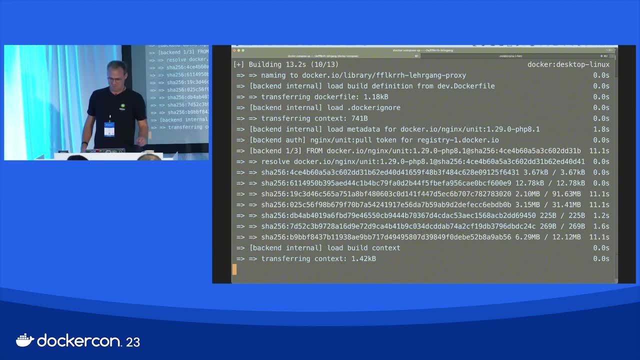 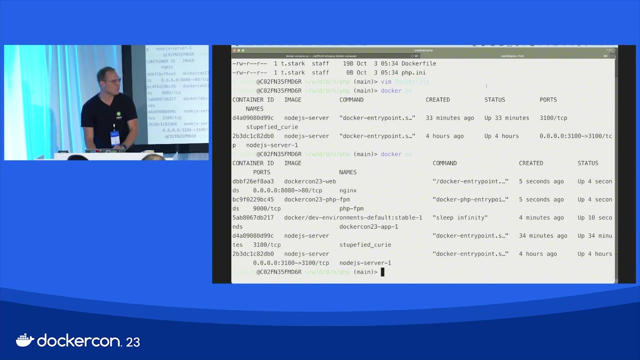 then that would be interesting. It's: yeah, What did I say? Yeah, sometimes, All right, sometimes it's like this: Okay, so while this is building, let's leave it for a minute. By the way, is black better or white better? 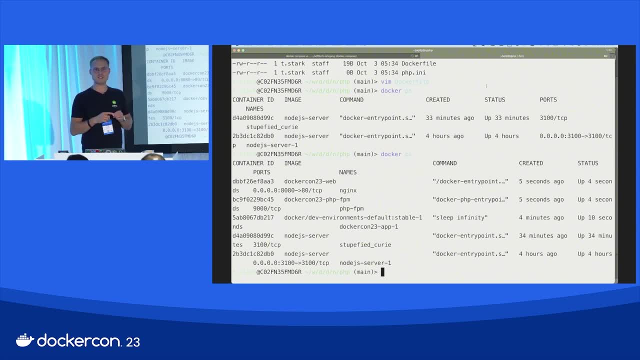 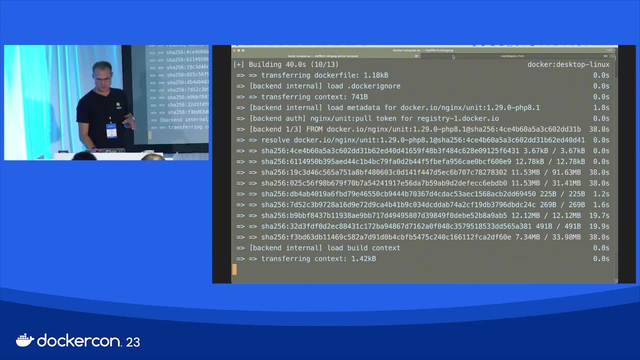 Just go ahead. I think black is better. Black is better Because, yeah, I was trying to make it like for you better to see. If you're saying black is better, I can, we can switch to black. 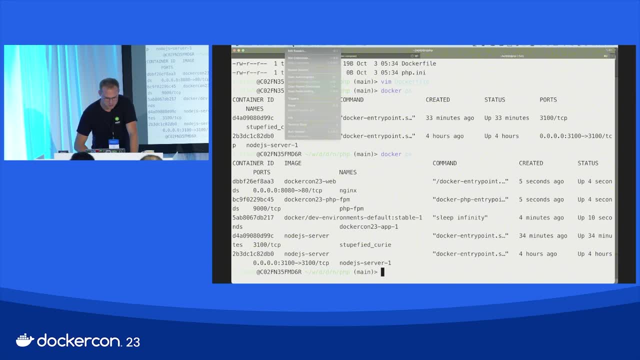 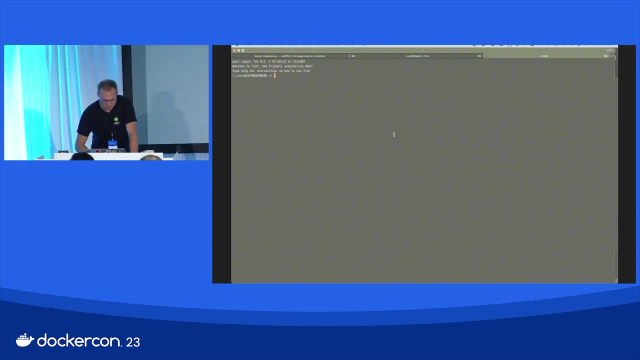 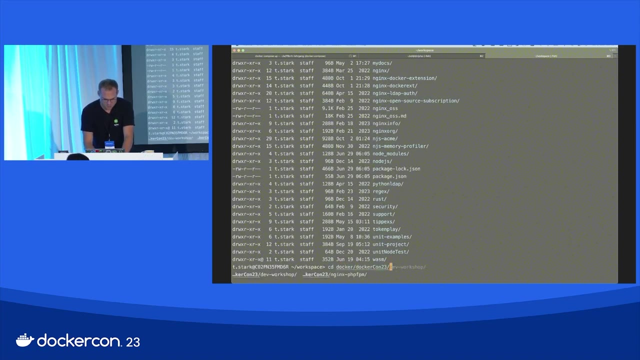 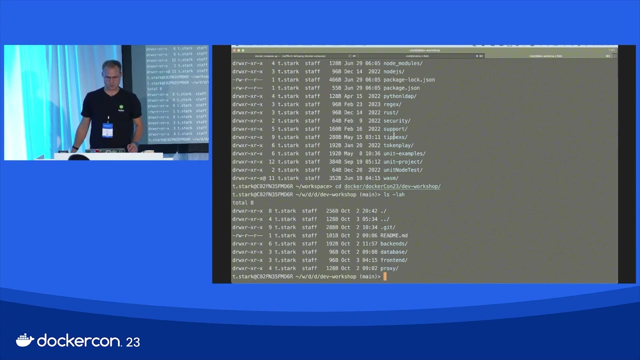 Black black Session. where's that? Where's my profile Default? All right, so let's create some stuff. All right, We have a README. So how to get started? Just create a directory. Something New project. 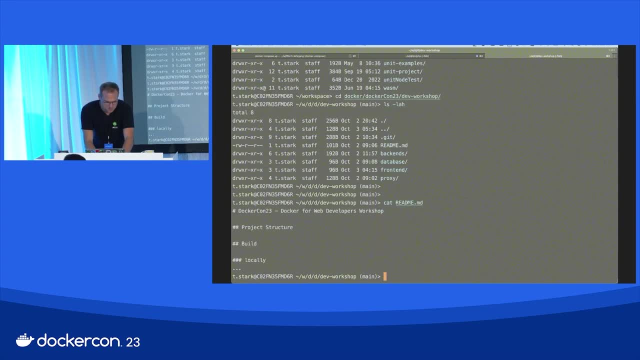 Then a README. What is in a README? actually Nothing cool. Project structure built locally. Okay, Then we create some directories, Backends or backend database, frontend, proxy. Oh sorry, What files? Yeah, Yeah. 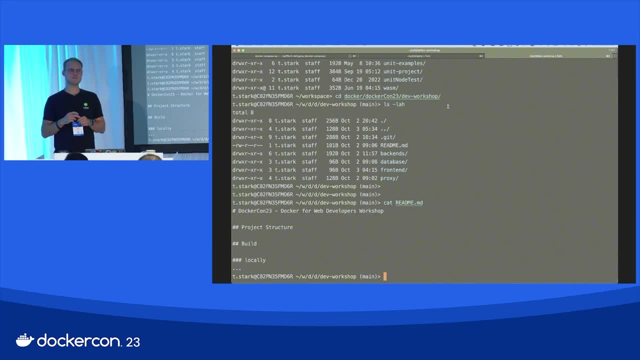 All right, good question. So just repeating the question. The question was if you have some user specific data like a GitLab token or GitHub token, access token or env file like environment files you don't want to push to a to a Git. 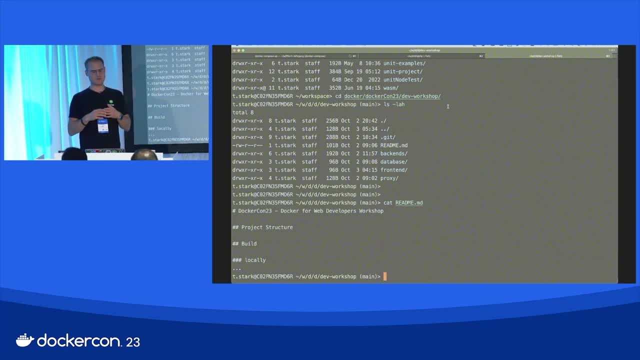 So yeah, if you have local like local host stuff, then I think an env file is possible. But this will not solve your problem because the GitHub token, if you have things that cannot be part of your compose thing, right. 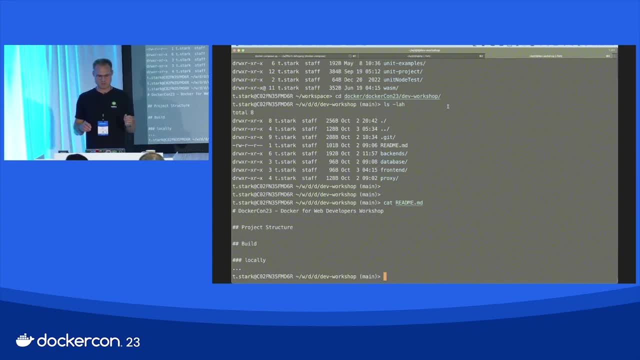 project, whatever, wrap it in. I think I have a buildsh file, or call it startsh or hellosh something, Something that works. If you have like a or a, README something and make sure it's described well enough. 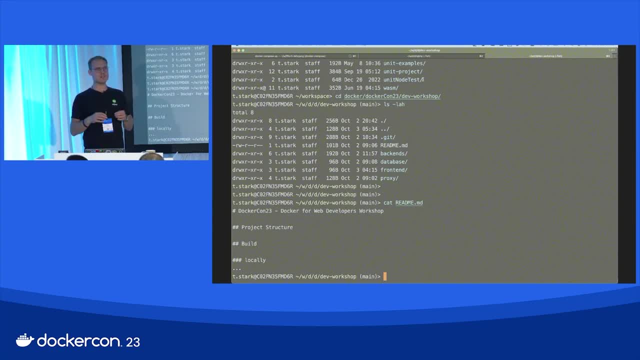 It's like, if you can't, if you can't put everything you need in a Docker compose file, then write it in the README. The very first thing say hey, thanks for working on this internal project. You have to do step one, two, three as a prerequisite. 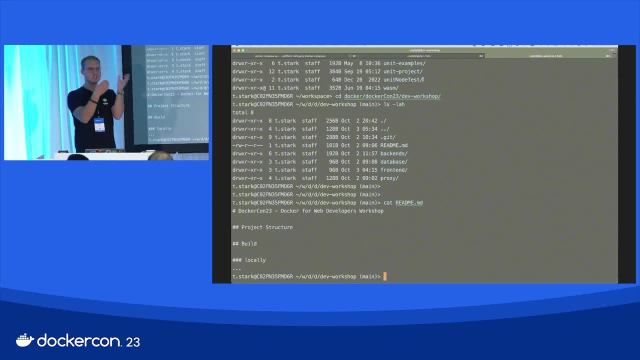 Otherwise the Docker compose will not work. So for example the LDAP thing, If you need some special credentials somewhere on your machine, otherwise it will not work, then you have to write it somewhere, and if that can be scripted in some sort cool. 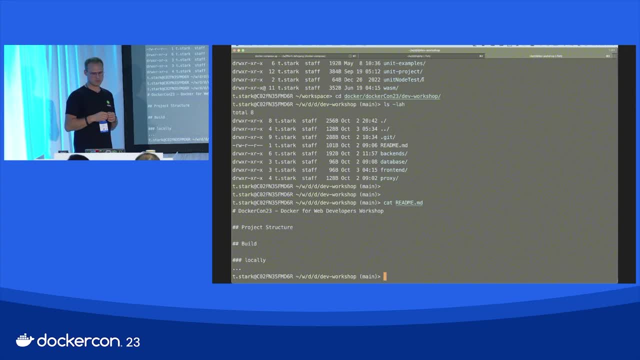 Let's do it. Another neat thing I was or I'm doing from time to time, depending on the project, I have sometimes an helper container image, like a setup container image that is doing some of these initial setup tasks, if there are any. 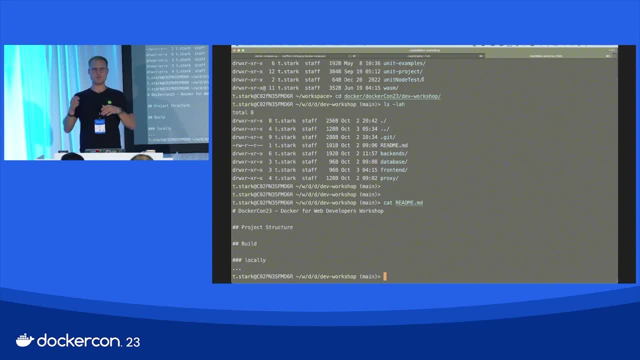 where you have to interactively like type in data. for example, You can use a container image that is commented out, for example, in the Docker compose file, and then put paragraph in the README saying: hey, if you're starting up this for the first time, 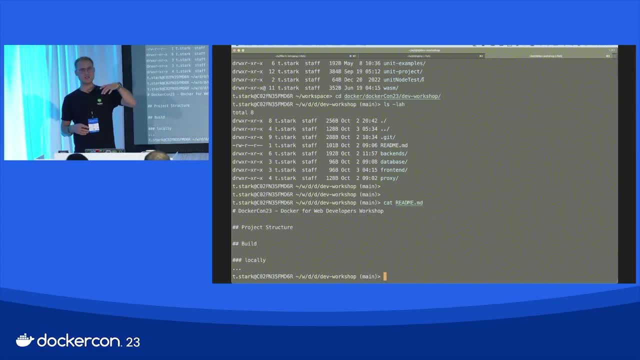 you have to pull up some credentials from the active directory, for example, or register this application at the IDP to get the handshake working. Any time you interact with a huge third party thing- identity providers, active directory like databases or something- yeah, 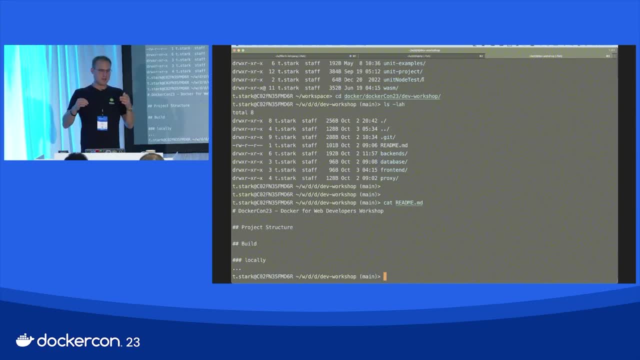 that's something. then you can wrap in a shell script Bash for Windows, another bash for Mac OS. it doesn't really matter, but just to make sure you should automate as much as you can. Not for the reason because it's then automated. 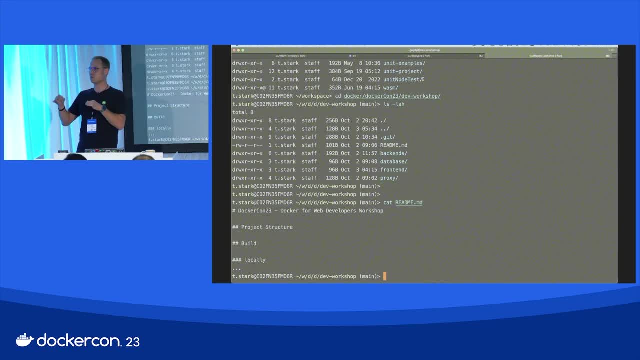 because anything that's written in a script is at the same time documented for others. If you write it down in a script, say, hey, we do this to get the credentials, then it's documented, it's written down somewhere. It's not in a Word doc somewhere or in a confluence. 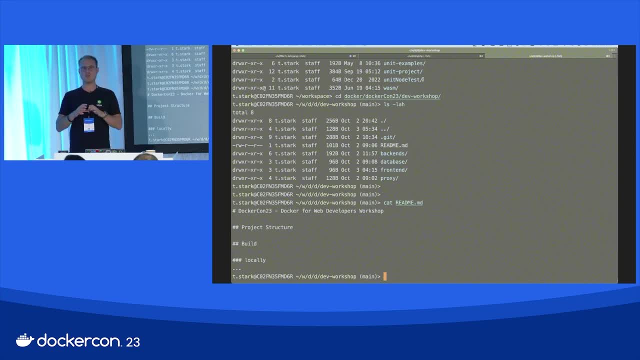 it sits with the code. So if you check out the code it says what you have to do. So sometimes you're right, it's not possible to put anything in there. You should try to do it as often as you can. If it's not possible, describe it well enough. 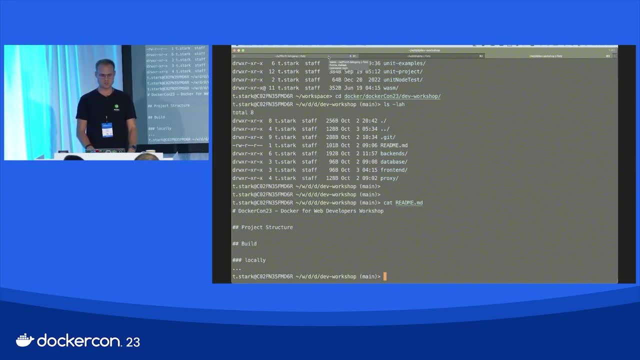 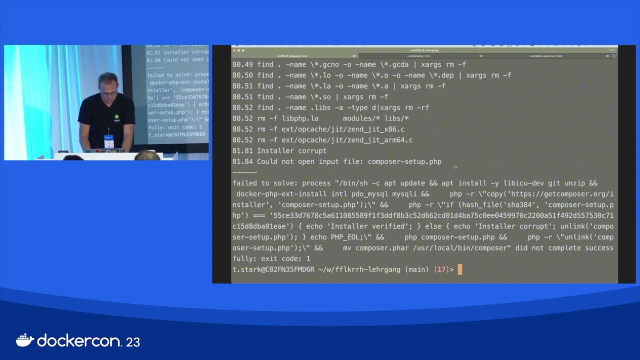 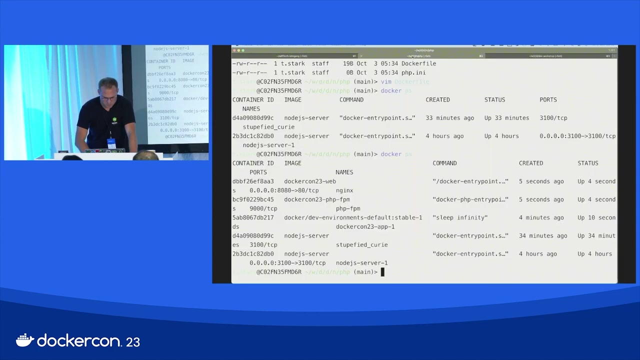 and make it easy to find those information. Cool, say: it's not completed. okay, Install is corrupted. all right, that's nice. So, okay, black is better. so then let's use black, Okay, so let's see what we can do here. 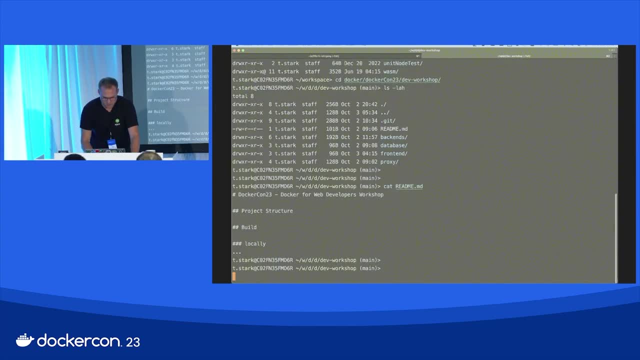 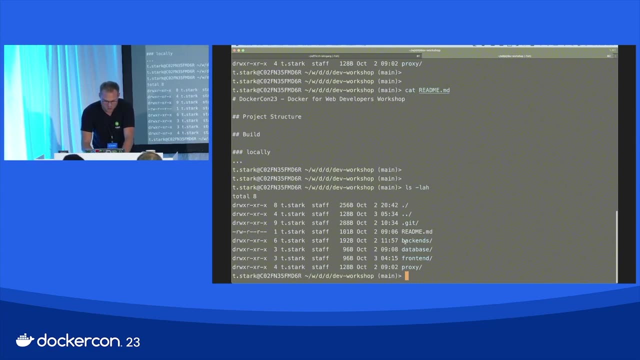 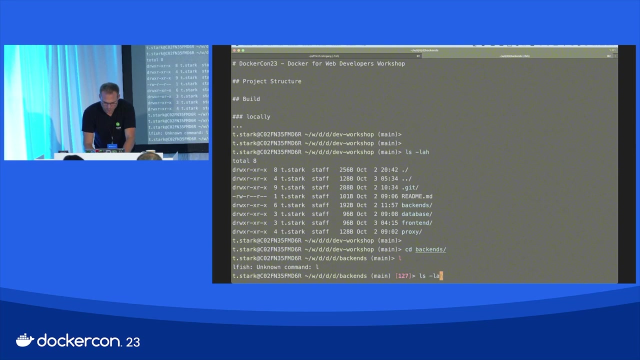 Let's see what we can do here. Let's see what we can do here. Okay, We have the database, we have the front end, we have the proxy, All right, so I think in back ends I already have Nodejs and PHP. 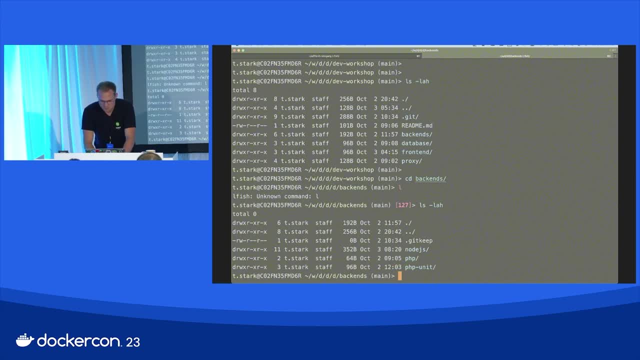 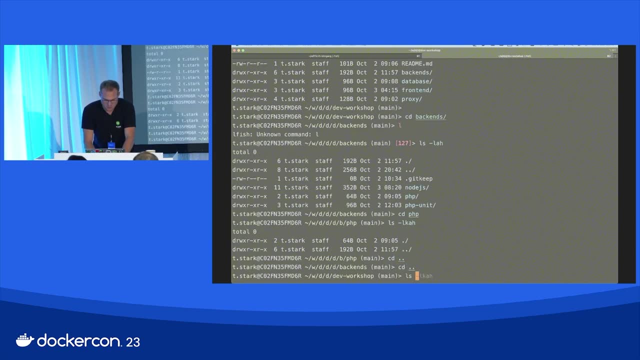 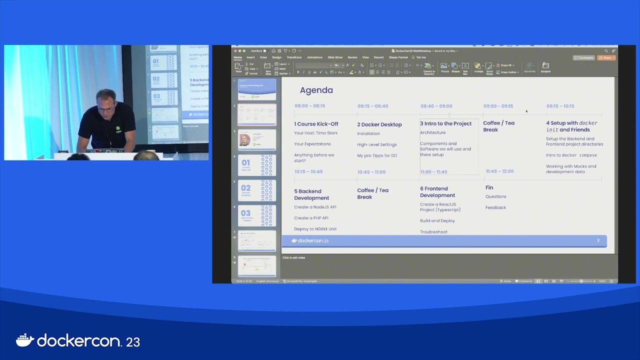 and another one with PHP unit, And I think they're empty. Yes, they are empty, So we can write actually some code. Okay, so we can start with front end. Let me actually check something real quick. Yes, We set up back end in front of project directory. 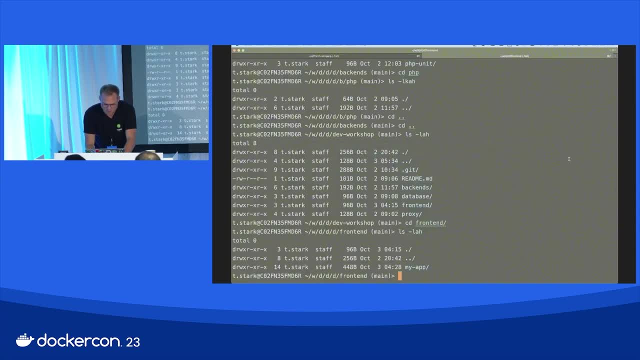 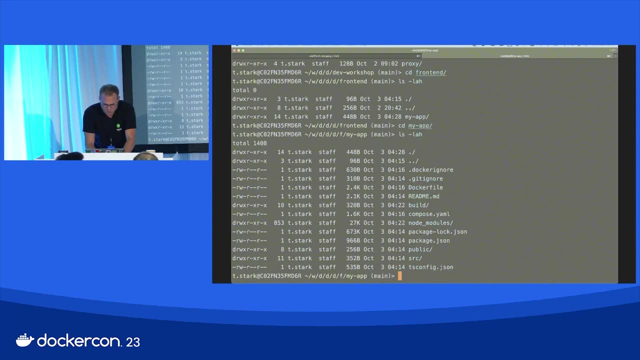 into a Docker compose. Yeah, Docker compose is something we already did. Okay, here is my app. I think I tested this yesterday just to make sure it works. Yes, So let's start with. let's start with the front end, then. 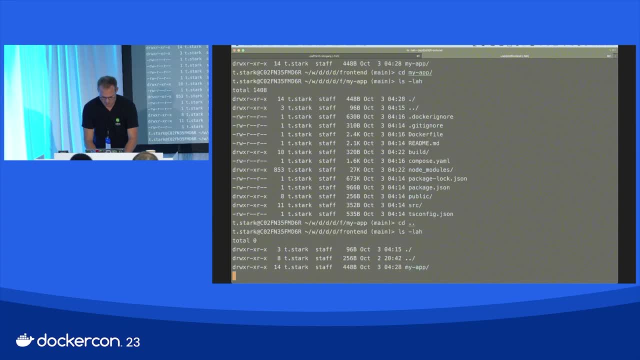 Setting up a front end is like: yeah, it's basically depends on the framework you're using In this. in our case, we are using React as the front end And to set up a project with React, there is some. there are MPX and NPM tools to do that. 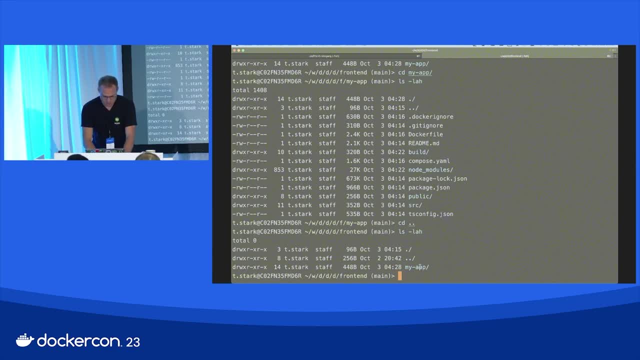 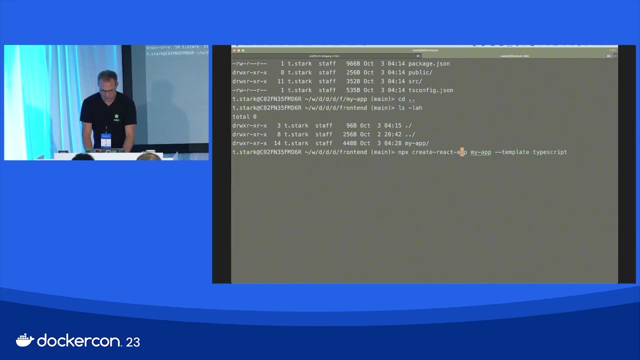 So- and in this case we can use something like npx- create React app- I think that's a very common thing- And then you just define the name: React app- my app too. So in here, and this is, this is something. 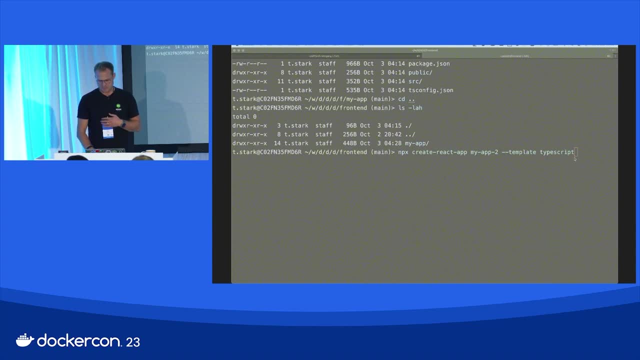 I would like to show you as well, Because I see a lot of tutorials how to use or how to bring TypeScript to a React project, And then they start by creating a TypeScript project without React and then they're adding all the TypeScript stuff afterwards. 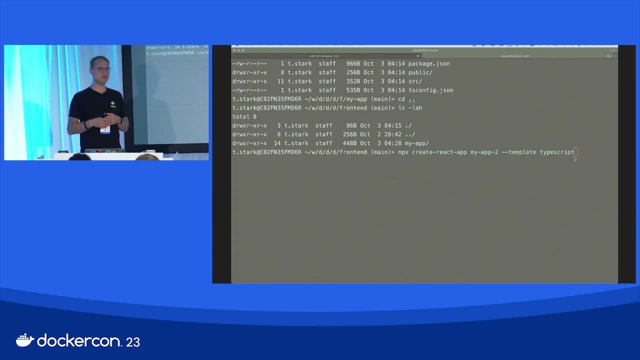 Which is I don't know. I don't know why, why somebody would do that, Because there is a template, exactly for this reason that you can simply start with TypeScript. Why should I start without and end afterwards? Doesn't make any sense. 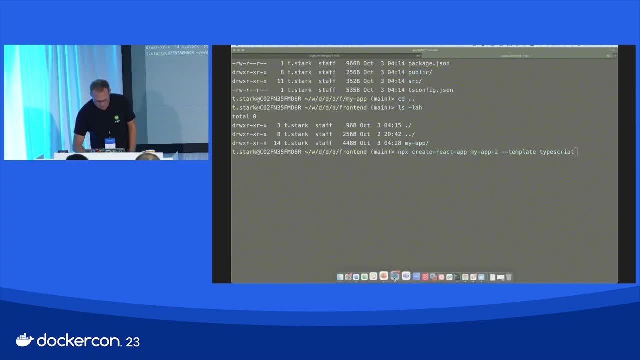 So if you would like to create a React app and start with TypeScript, quit this. then there is a template. So reason why I'm jumping on this template thing so much is because I didn't really understand what templates are, since, like for a long time, 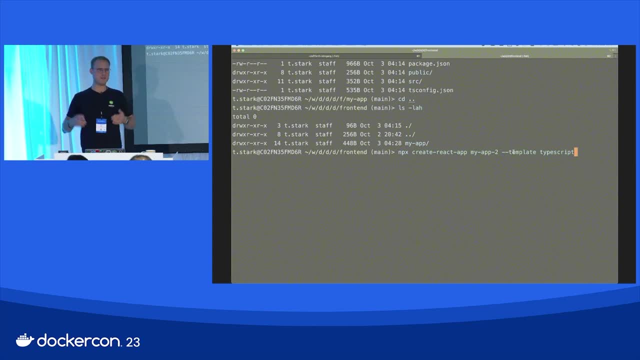 Just used it. And then I was curious at one night. I said: what is a template actually? What can I do with a template? And I said: I have a. this is what I show you. I have a lot of code. 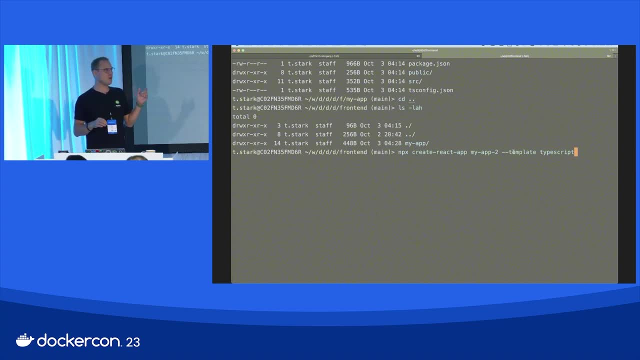 I usually have in my, in my React applications because all of my frontends are interacting with some sort of API. So I have built some wrappers around. I'm not using Axios, for example. That's a third party thing to do, Like API calls and network calls and stuff. 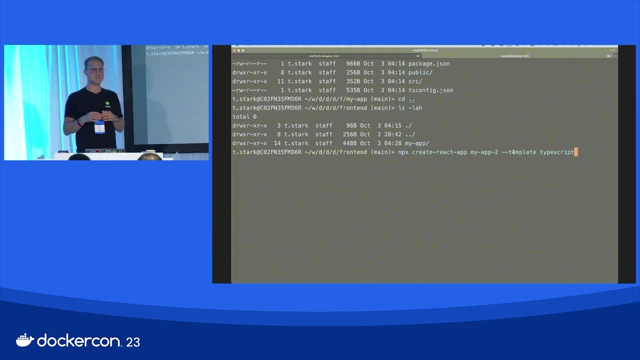 I just build them by myself. I don't like third party dependencies much. I use them from time to time, Of course, like Express for backends- we do this here as well- But I just love to build something by myself, Because then I know it's working. 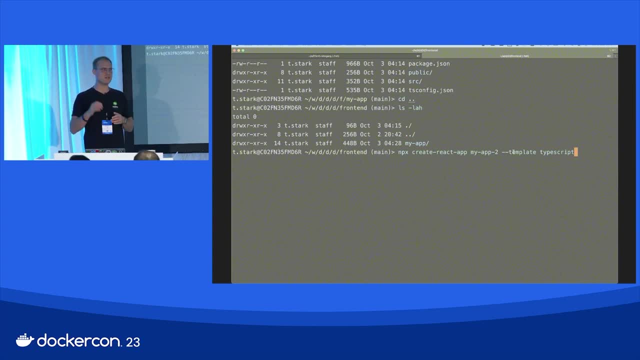 And then I know it's not. it does not come with a ton of stuff that I'm not actually need. Another thing: when you work with Node and frontend and TypeScript and JavaScript, stop doing NPM-ing. everything. This NPM install stuff is great. 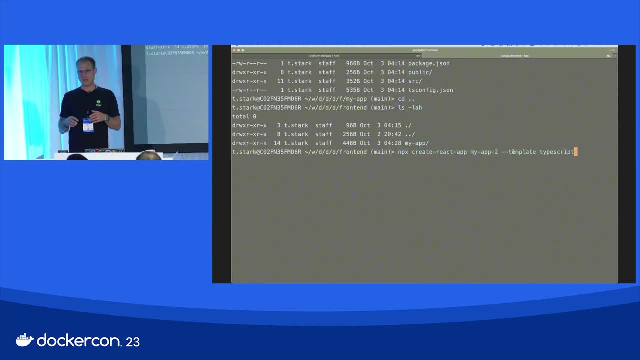 but it's to me it's like it gets a little bit out of band. I see projects where they do NPM, install a third party dependency to compare two strings Or to get parts of a string. Hey, that's vanilla JavaScript. 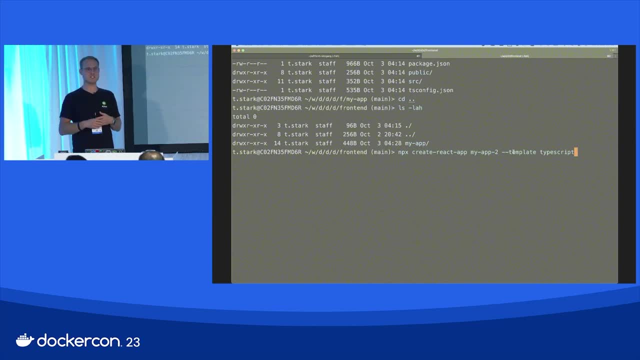 That's in JavaScript since the early 2000s. Right, That's it, doesn't? you don't have to do that. Stop, Stop. NPM install string compare. Why should you do this? Use vanilla JavaScript. That's the way it works. 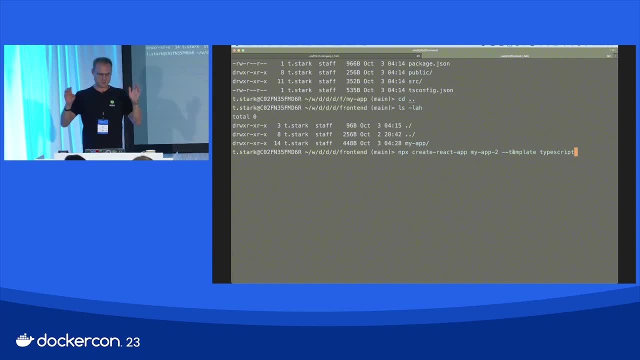 There's no reason for that, Right? So? okay, that was an emotional thing, So don't don't do this, Yeah, Right? So question was: what is the difference between NPM and NPX and YARN? 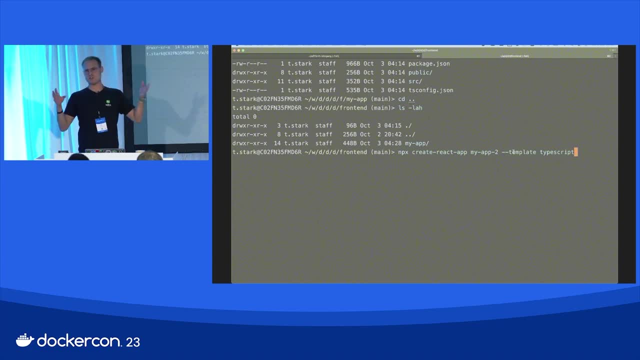 YARN is a different, is literally a different binary. It's a. it's a complete, separate project. It's not related to the NPM thing. It's a. it's a complete, separate project. It's not related to the NPM thing. 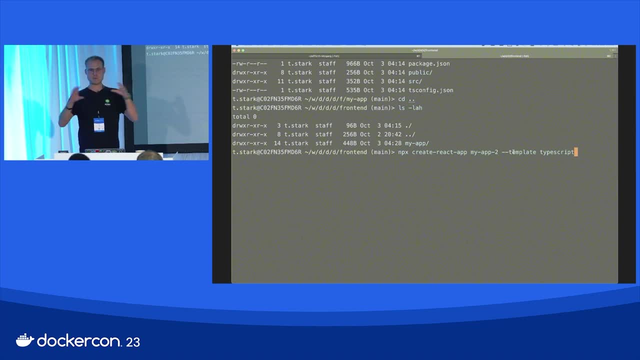 And NPM is like the package manager for for Node, And NPX is a is another binary that comes with this, with this, like it has access to this, to this templates and to this extra scripts, And in this case we have to use NPX. 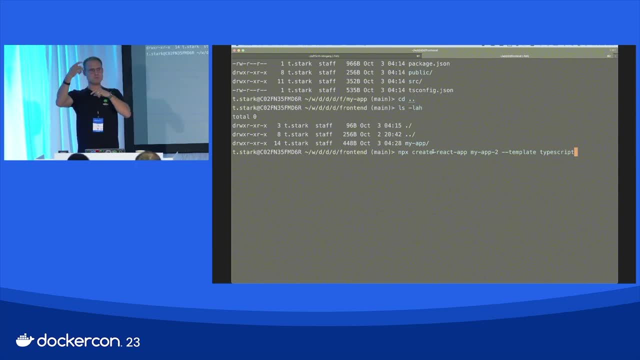 because we need this create React app thing to bootstrapping our React application. And then we say at the end, template TypeScript. So push, hit, enter. It will think for a minute, Okay. So now it says okay, we're installing the package. 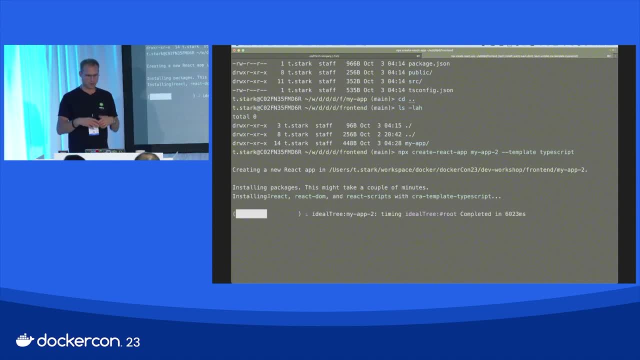 We're installing React and React DOM and React scripts And it will pull down some stuff And I prepared that already. So, just in case this is too slow, we can use it from the, from the prepared thing. But I would like to show you, yeah, how that works. 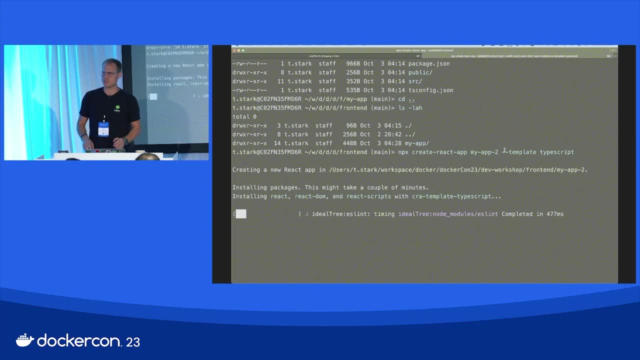 Good. So, and what is this template? A template is basically something we can use in this React. the template is something that comes from create React app. It's not an NPX thing- NPX thing in general It is. it is a feature for create React app. 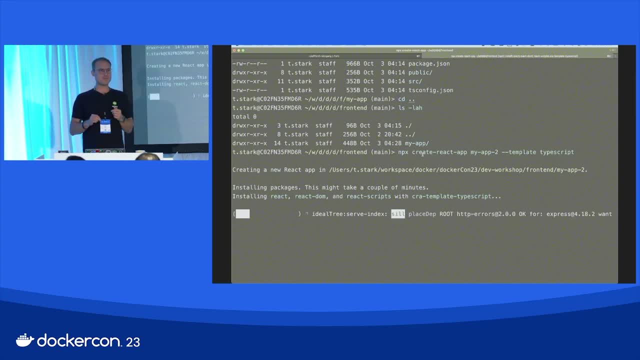 So reason why I'm saying it: I have custom templates. Because I thought, like what I normally do, is I say: okay, I have a new project, Cool, NPX. create React app. my app template: TypeScript: enter: fine. 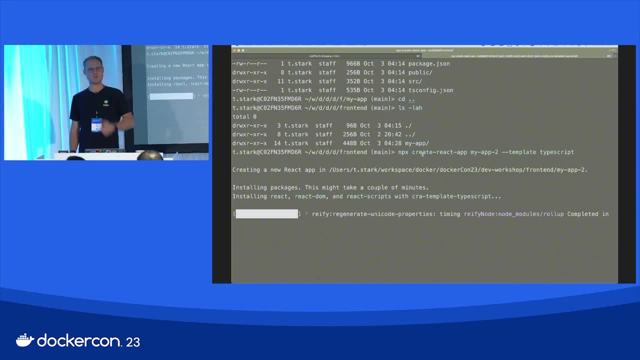 Next thing I'm doing: I open a Git repository, push everything in good. Then I open another terminal and copy all the common things I normally use, like my error handling, fetch my login handling, fetch all the things I built by myself. 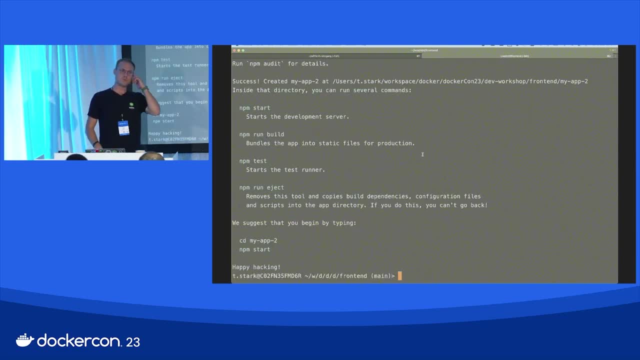 because I don't want to put them in happy hacking good, I don't want to put them in an NPM package. I could do this, yes, but I don't see a reason why I copied that all over to my, to the other projects. 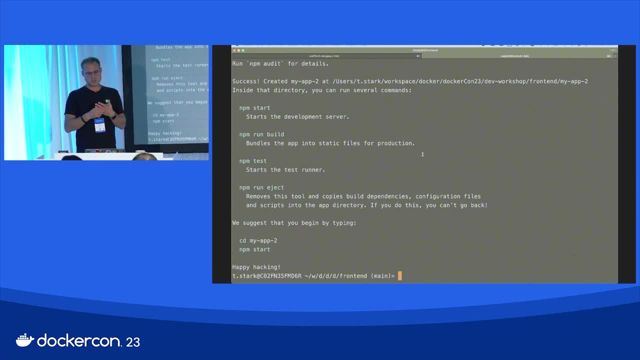 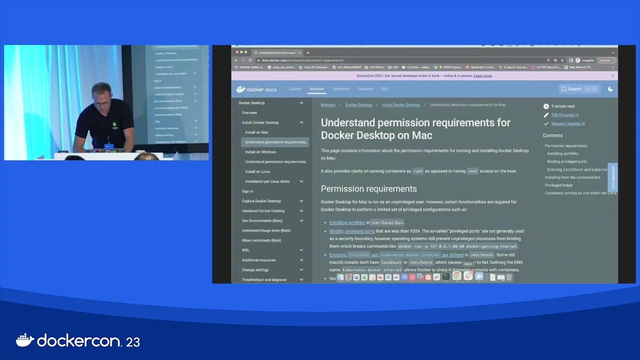 Took me some time. So then I try to understand. what is a template? Can I not do this by a custom template? Of course you can, And this is where templates come in very handy, And they're, of course, documented on GitHub. 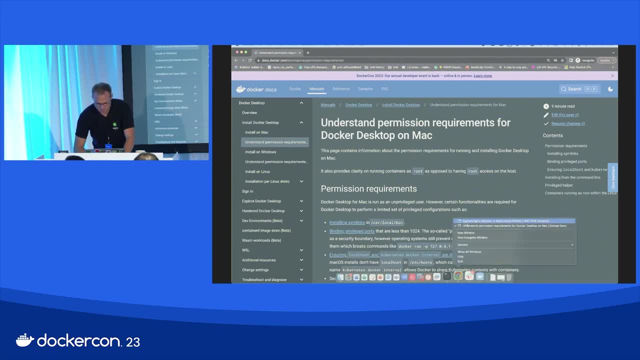 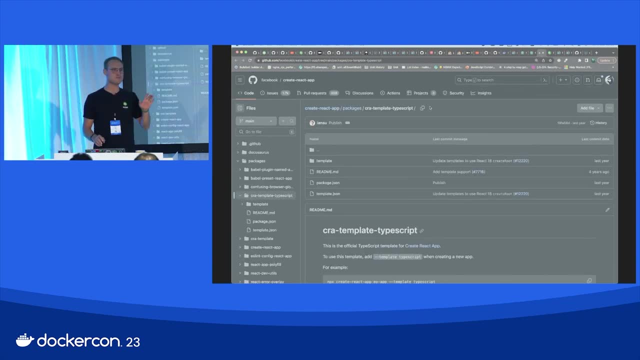 Let me show you this, Don't blame me. That's, I can at least see the fav icon I have. sometimes I cannot even see the fav icon in my in my tabs bar right. So it's not it's, there's still space left. so 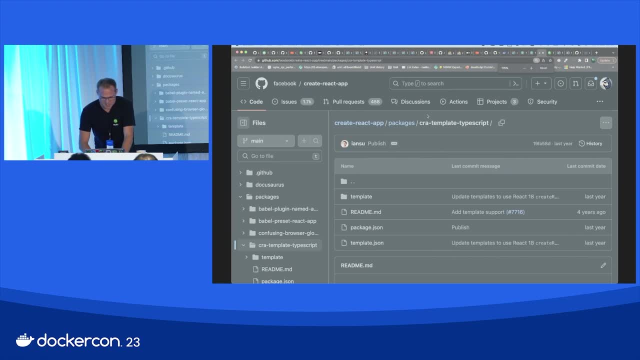 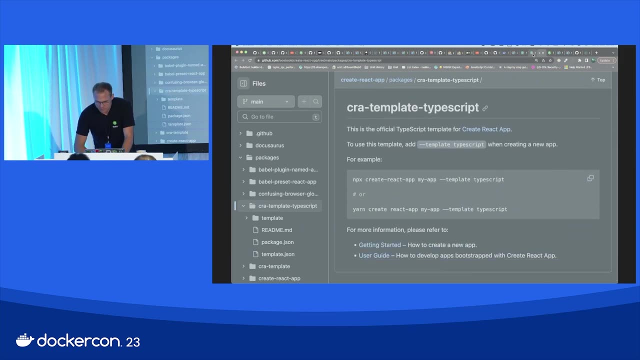 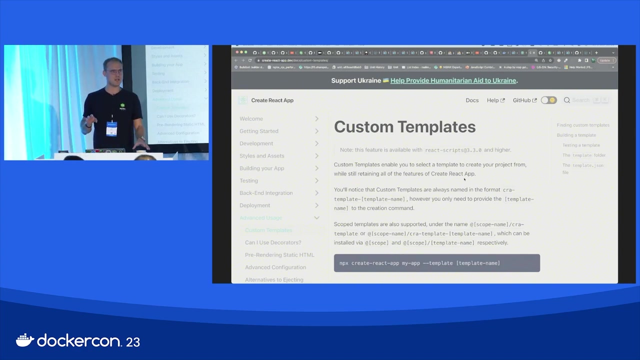 So this is: create the the templates. This is an official TypeScript template- And then they have here. It's worse reading If you have like 20 minutes time somewhere and you have and you work with front ends using React. 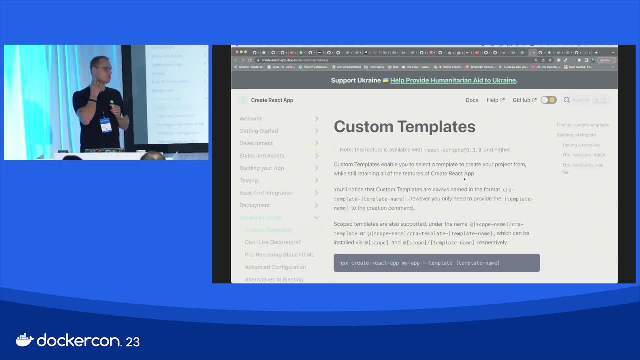 and create script and stuff. make sure you check out the template documentation. It's worse And if you have the same things and you have to add common things to all of your projects from time to time, you can use templates Or others using GitHub repositories as templates. 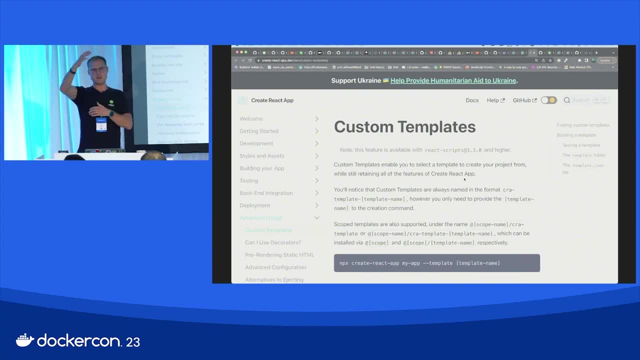 Like you can git clone an empty project with a package, JSON, all this kind of things in it. Yes, that is also. that's also working. Depends on what you want to do. I like this template idea because then I relay on the 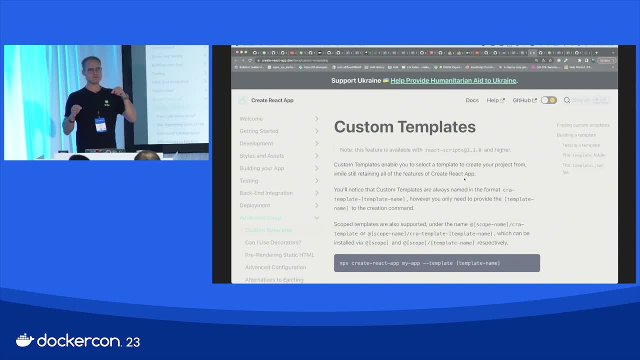 on the create React app thing And use? if so, let me tell you why I don't like the. I have a GitHub repository and I do npx create React app once. then I push everything to GitHub and share this with my team. 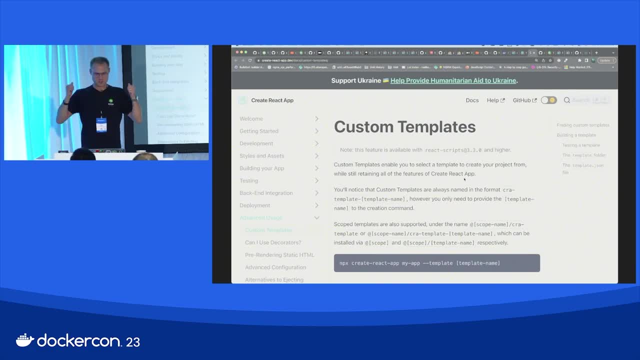 and they use the GitHub repository as the template. So they use this for like a couple of, a couple of months, years, whatever, And then of course they can npm update on their local machines. But if I got new features, 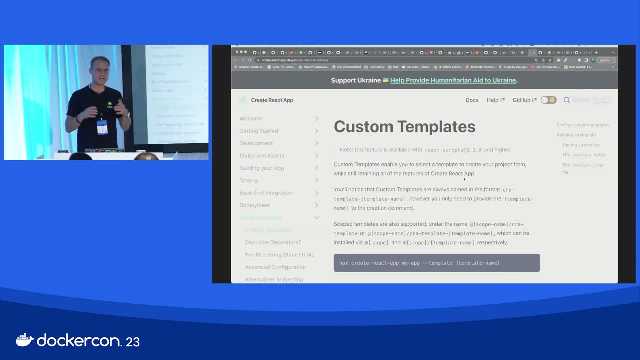 or different kind of setups in this create React app script that I'm using. this is not part, this will never be part, of this GitHub template, because I'm not executing it every time, I'm just doing it once, And an npm update will not fix this whole thing. 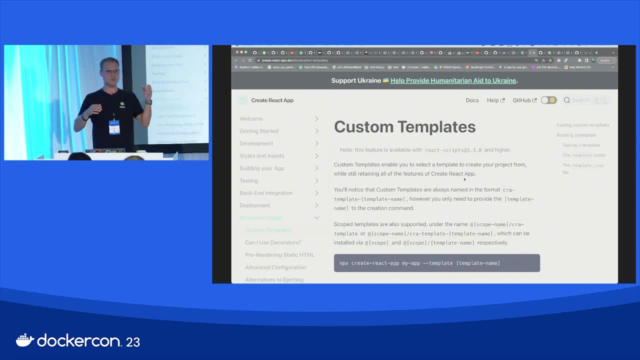 It will update dependencies but it will not generate. it will not get new features and structures from this create React app thing. With a template, we are using create React app all the time and adding our custom template at the end So we make sure if they push some new stuff. 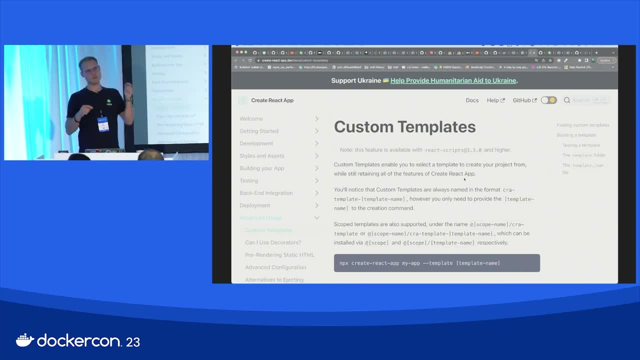 to create React app. we make use of it Right. So that's why I think a template is a better idea than just sharing a GitHub repository. others can consume and pull. And another thing that happened, like a lot of times, with people using this GitHub idea. 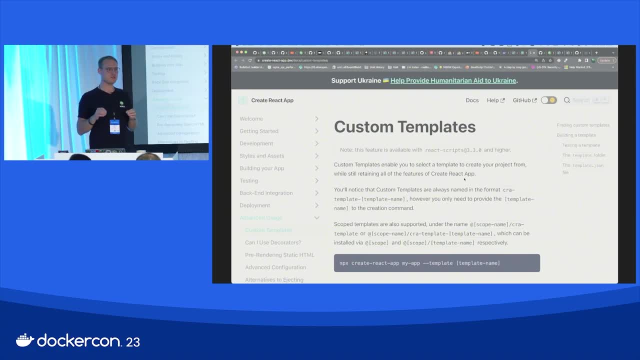 I mean, the chance that somebody will override your template on GitHub is nearly by 99%, Because they will not. they will not switch. it's like it's written in the readme. of course It's saying, hey, clone the template. 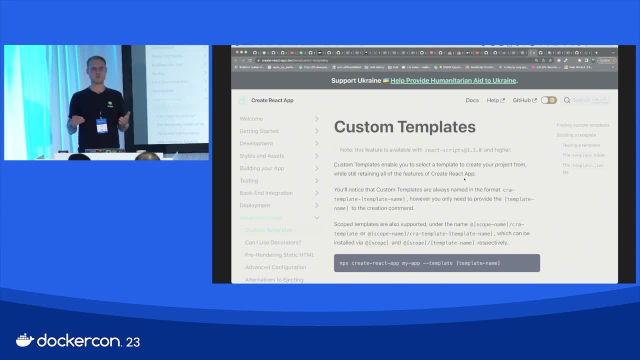 delete the git directory and do git init and create your own GitHub repository. If you over-read this little sentence, you will do all the stuff you get: push okay, oops, sorry, we have accidentally overridden your template. Can you maybe like merge it like? 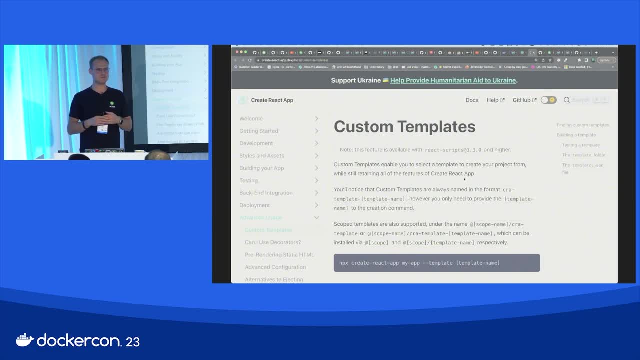 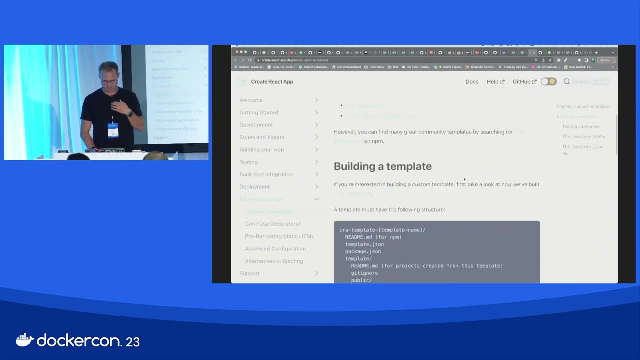 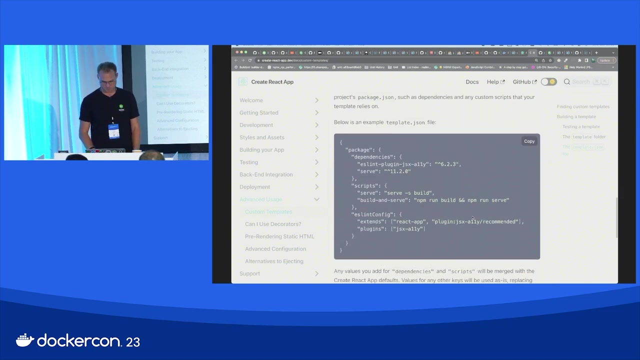 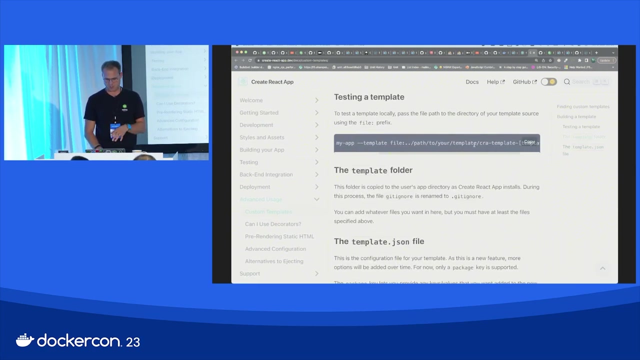 can you do it like backwards? maybe Is it possible. Annoying No, that will be executed once. This template will be executed once. As I said, there's a very, very, very interesting documentation about custom templates and how they work. 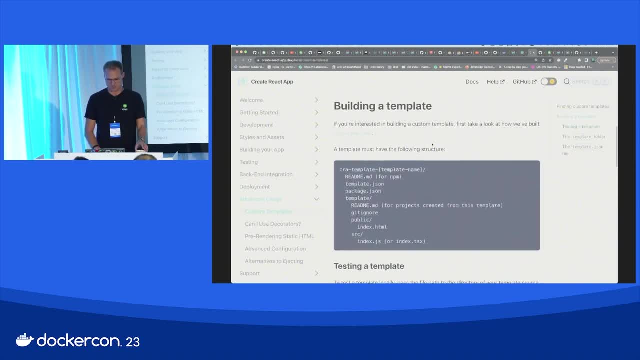 It's worth definitely a read. So here, for example, a template must have the following structure: A readme templatejson, a package, a template, public source. And this is what I mean In this source directory. you can put basically in whatever you want. 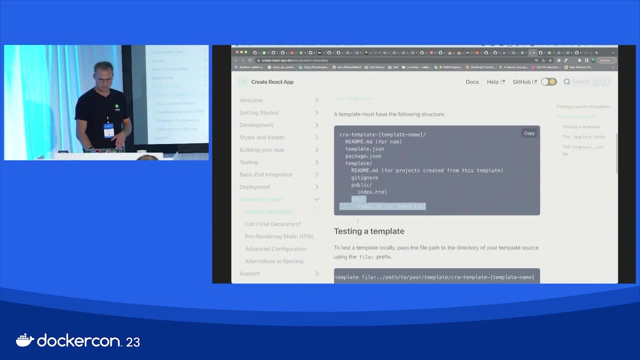 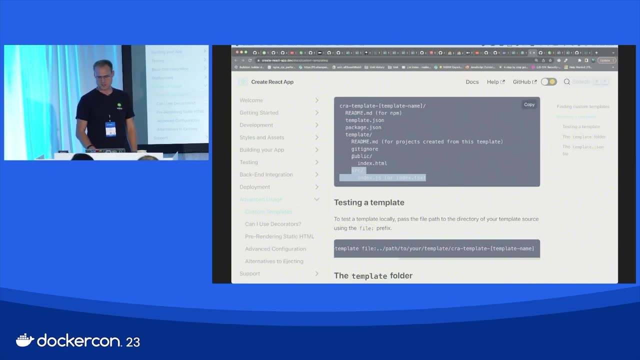 And if you have in source something custom, like your custom TypeScript file, just dump it in source. Or another thing I was doing for a company was like they set it up a front end and all the time they were looking for logos and icons. 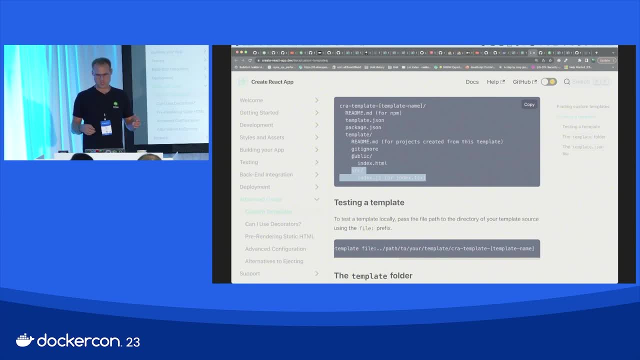 and fonts and all this kind of stuff, And of course we can say just reference them by a CDN. but sometimes it's just super important to have those files locally on your machine And to me it's better. and this is another. that's what I was saying always. 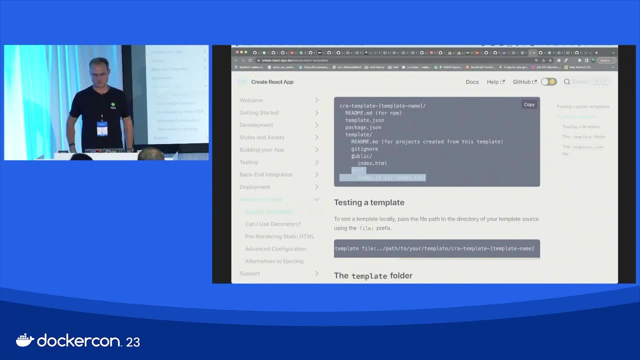 because I went through this valley of pain a hundred of times. If they are not part of it, you just clone the repository real quick. you pack your laptop in, you go to the airport, you're on the flight, you make it up. 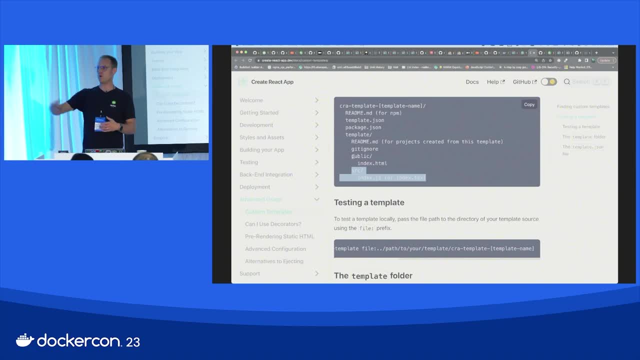 yeah, it's not working because the font is not there, the logo is not there, and you are now 12 hours on the plane and you're about to do something and you cannot because the font is not there. stuff is missing. 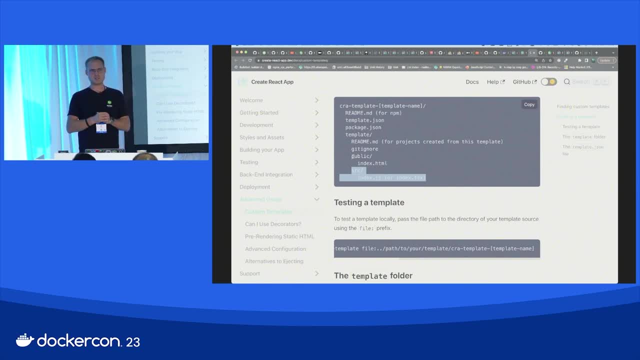 I could have checked it earlier, yes, but I expected that I cloned this thing. it's everything included. That's what I'm saying. you want to have a lot of files, font images, whatever, so that somebody that spins this thing up. 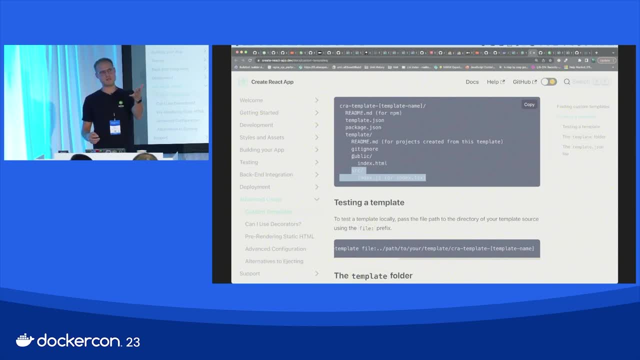 can work actually with it. It's not hard. It's a little effort for somebody who's doing it once, but it will help a lot of people just cloning their repository. All right, so this was about React app. That has actually nothing to do with Docker at all. 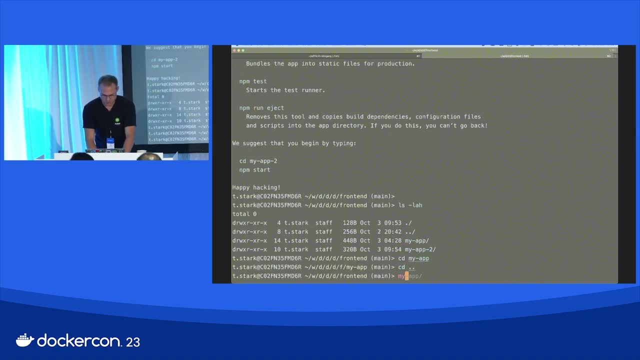 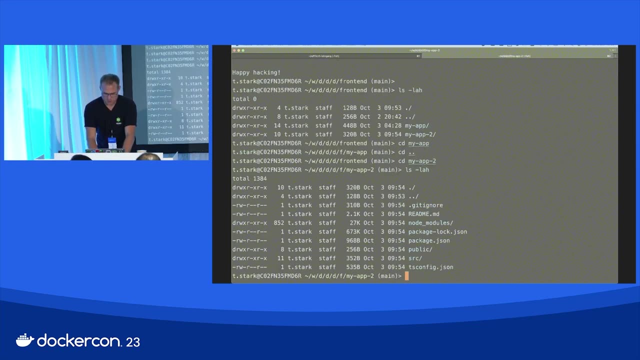 but it's super important. Okay, So then we have now MyApp2.. MyApp2.. Jesus, Good. So we have no modules, we have readme, we have a package JSON, we have public source, tsconfig, whatever. 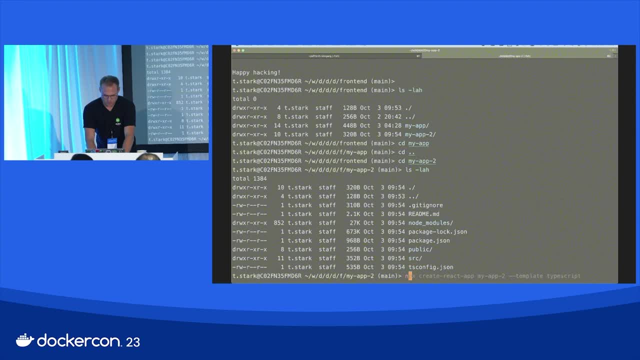 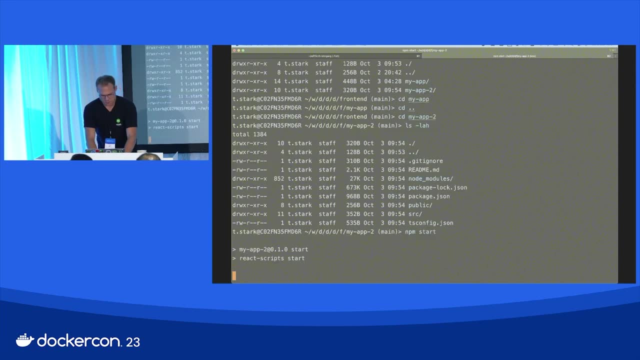 So next thing is basically, if you would like to see what this frontend looks like- I see a couple people doing this npm- start. in this case, it works. Another thing I would like to share with you is in this case: 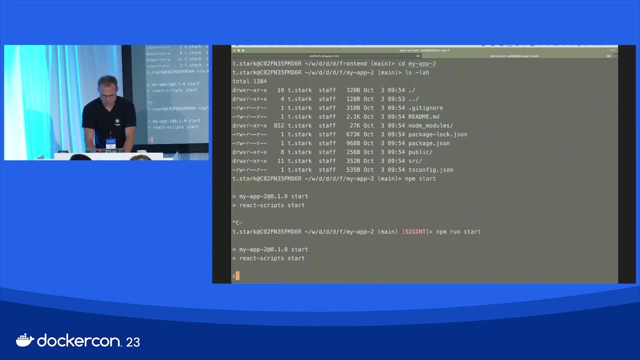 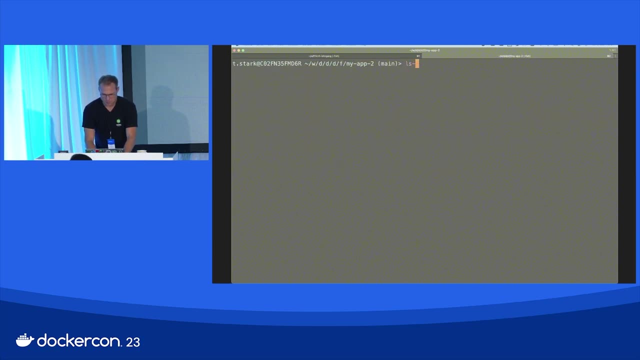 both works, Yep. So this is another question I see from time to time. What are the difference between npm run and start, and why does it? what does it mean? What is run? Why not use run when not Good npm start, in this case? 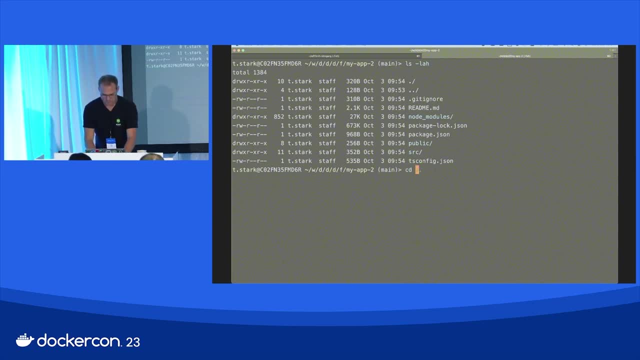 is part of the like the npm ecosystem and it has some common files. It will execute and look for when you just type npm start If you have some special things, like with nodejs, and you have a server and a large project. 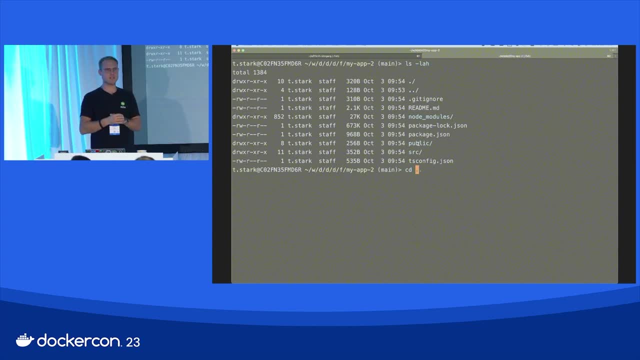 and you would have the same experience for an engineer and say, hey, if you type npm, start, it should work. Okay, You can define those things inside of your package JSON, and I recommend you to do that. There's a script section. 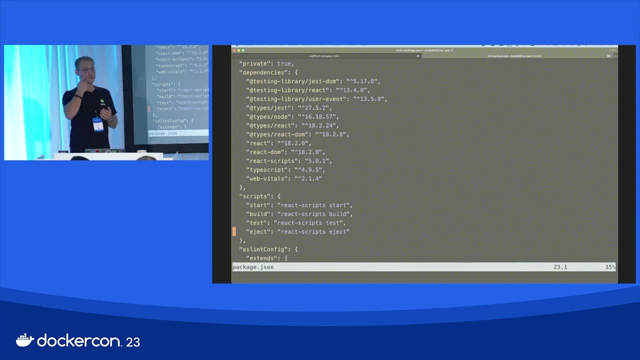 And you can put as many things in it as you want. Make sure you do it. If you have a nodejs, like a backend API, that needs some special arguments, for example for a node like. let me show you this. 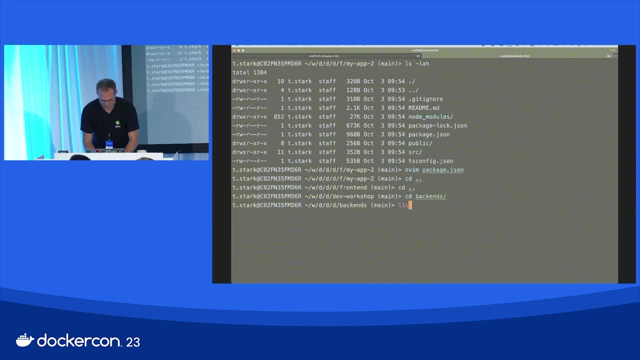 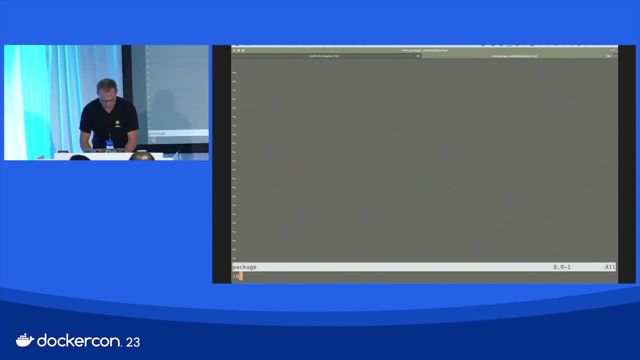 I've already prepared that. Sorry for jumping around, but this is. this is another thing that is really painful if you not do it. That's why I'm telling you that. So package JSON Here. So if you initialize a new node, 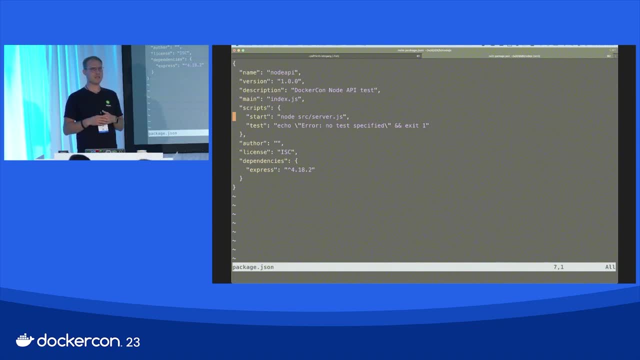 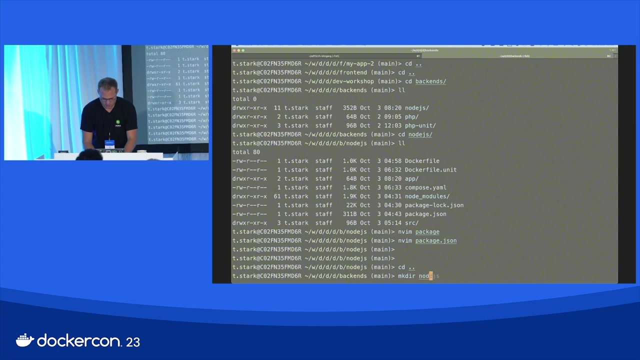 API using express. you can type npm init. It will generate a package file for you, And then we simply do express: Perfect, Let's do that actually, So you can follow along. So we mkdir nodejs2.. Then we do nodejs wrong. 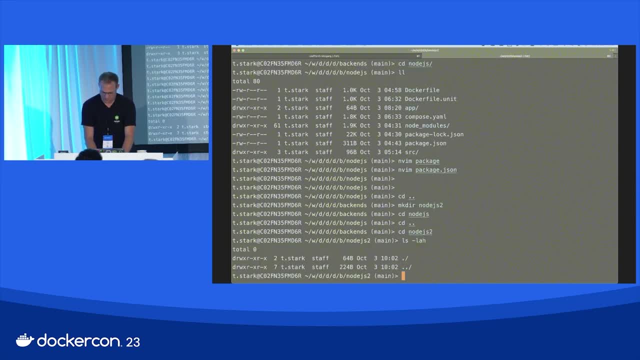 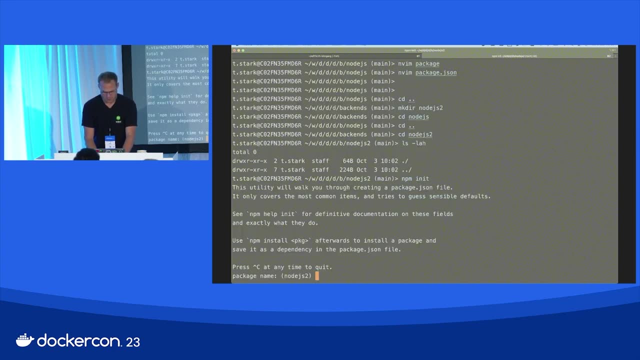 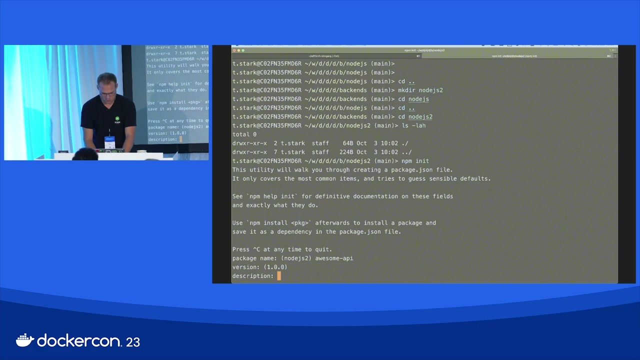 Nodejs2.. And it is empty, All right. So now we do npm init, All right. So what is the package name? Right? This is our awesome API. Of course, version is fine. Description- meaningful, Meaningful description. 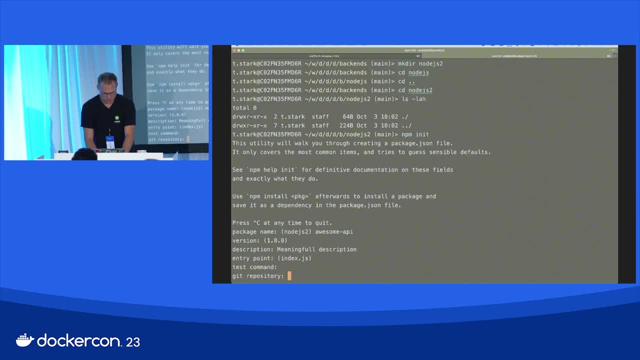 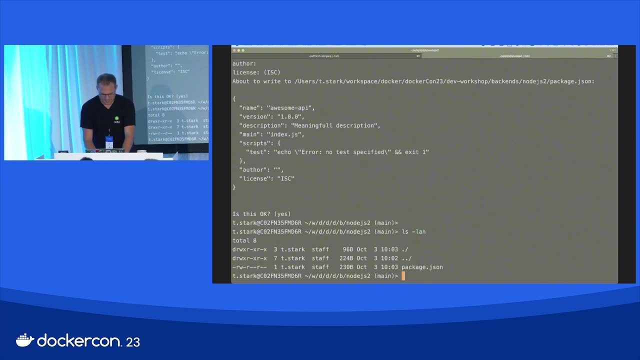 Enter Index is fine. Test command like: hmm, hmm, hmm, So good. Now in this package JSON we see there is a a main file that's indexjs. Good, So that means it will look for indexjs in your 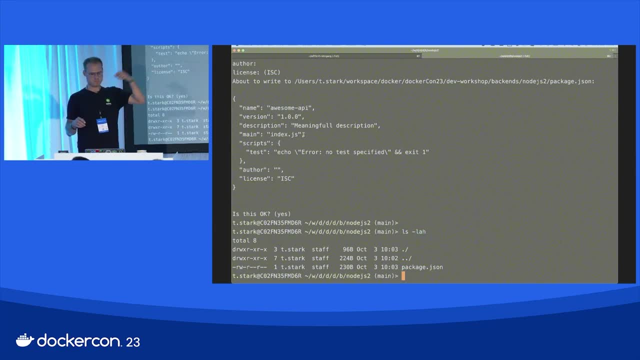 in your directory And when you type npm, start, it will check what's the, what's the main, In this case indexjs- It will execute it Fine, All right. But if you have some larger setup and you would like to in like, 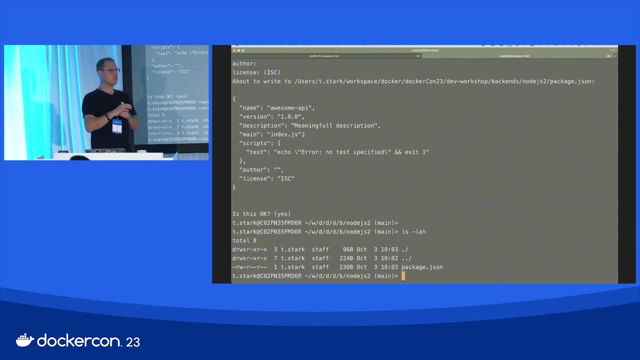 for example, you have some mock servers and you would like to give the engineers a way to spin up a mock API server, or what was the case with the identity provider, If you have a mock server in your, in your backend API. 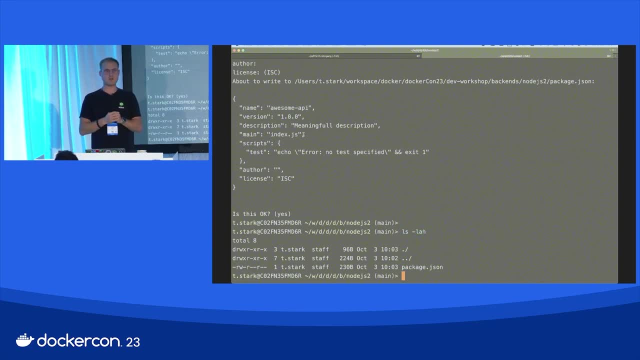 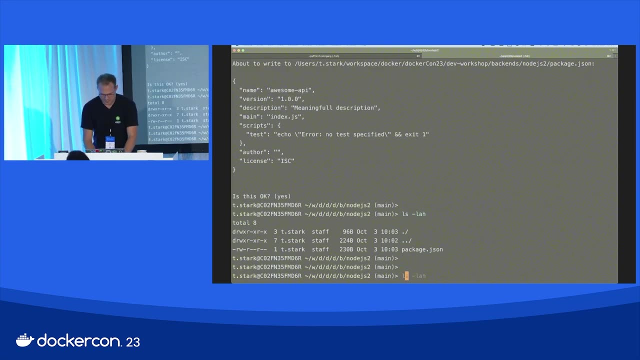 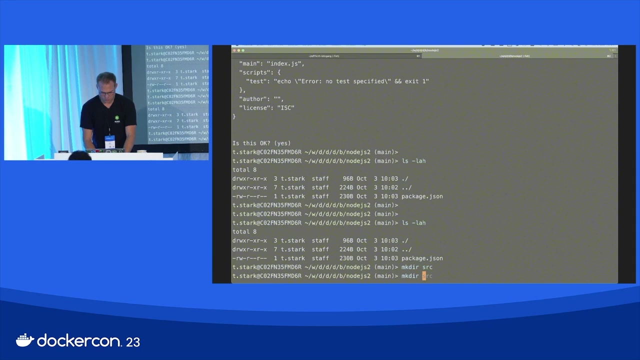 that mocks some sort of servers and that's a separate Nodejs server, which is definitely possible, then I would put it in the script section. So let's say we have something in source, Then we do. let's call that fake IDP, for example. 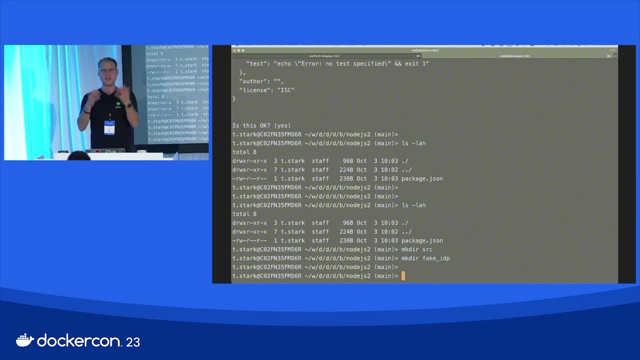 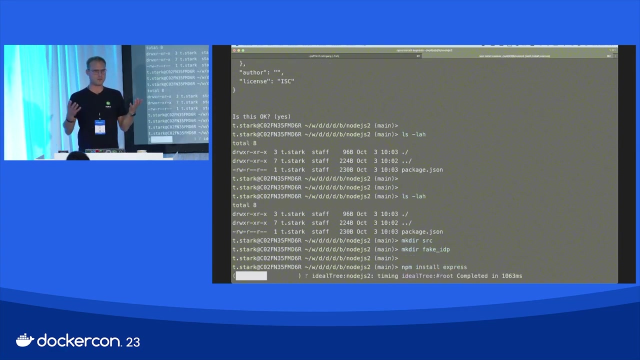 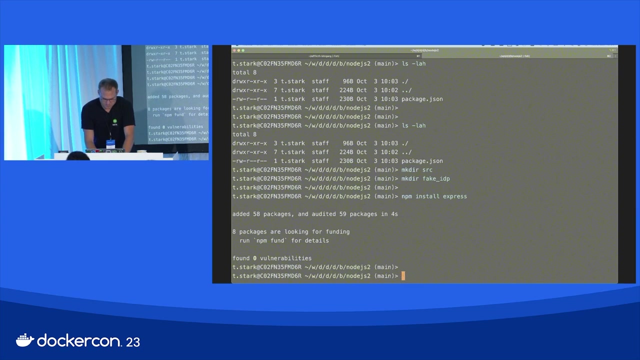 And in fake IDP we can build and fake IDP server, That is, serverjs. Let's first install npm, install express. That's the. that's the framework we can use to build like APIs using Nodejs. So now we have express. 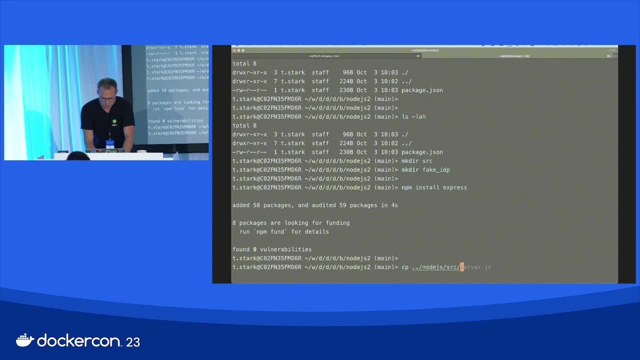 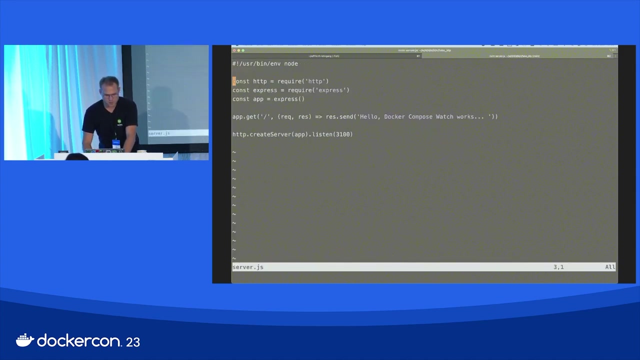 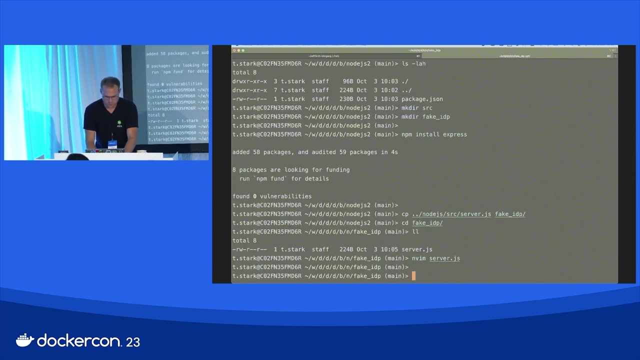 So now let's copy Nodejs source serverjs into fake IDP And this is not really doing anything meaningful. It's basically just using express and then saying: get on slash. and then let's say: hello from fake IDP. Perfect. 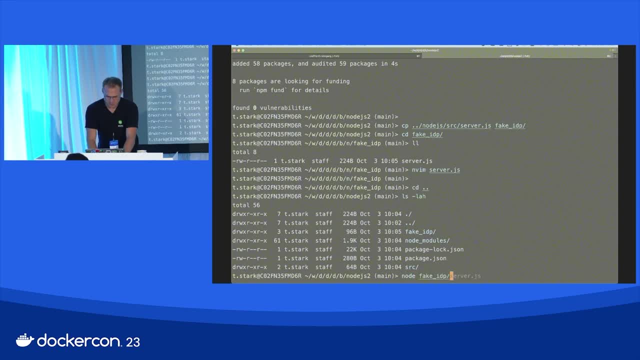 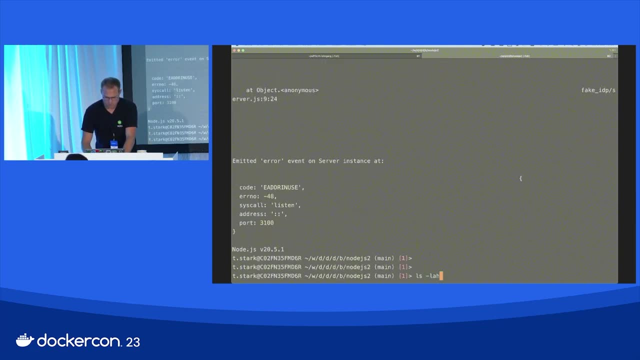 So, and I can do this- I can say: node fake IDP serverjs: Okay, already in use, Change the address. Let's use something different, Let's use 3999, for example. So now I can say: you know as an engineer, okay. 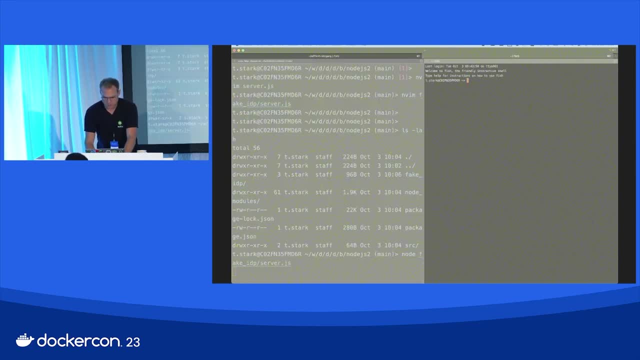 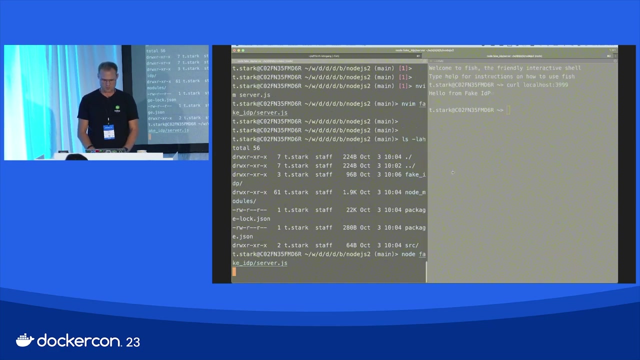 I can use fake IDP serverjs and it will boot up And then I do curl localhost 3999, and it says: hello from fake IDP. Absolutely amazing. Okay, you know that And you know that it's working like this. 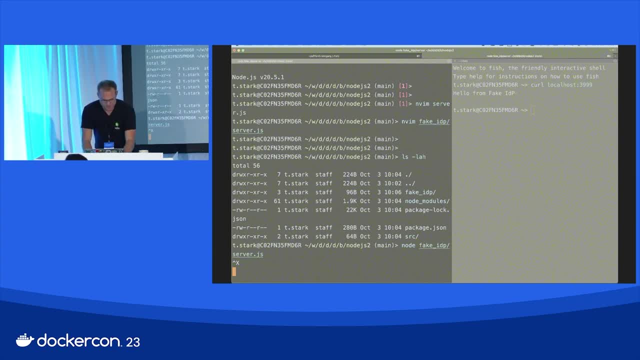 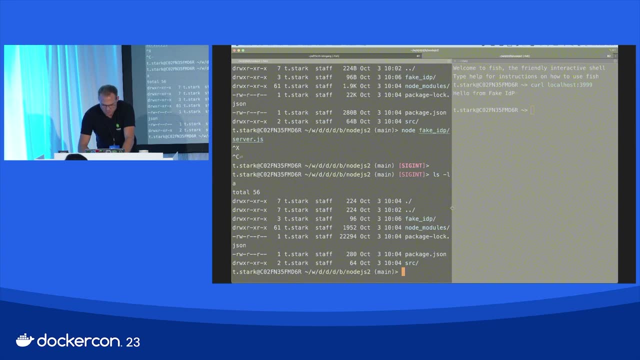 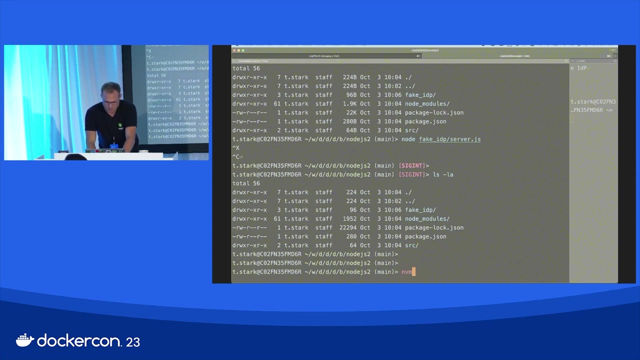 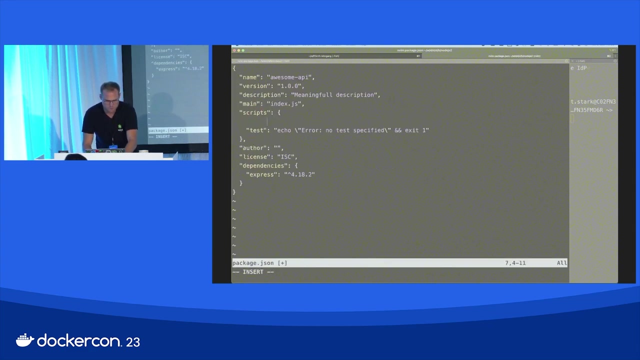 Like this. So the question is: does another engineer know that you can spin up this fake backend in a similar way? If not, you can do in the package JSON in scripts. you can just define one here and say IDP, for example. 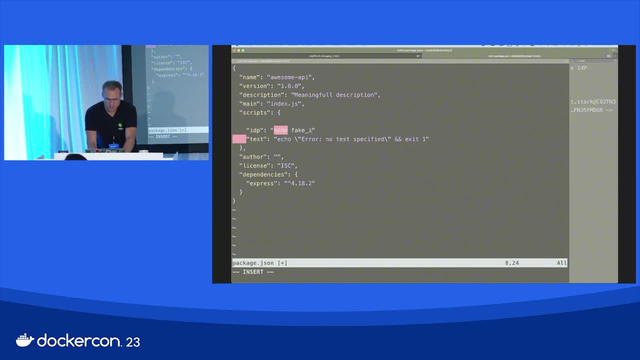 And then you say: okay, I want node fake, IDP slash serverjs, And if you need some specialties like what port, what environment, some other environment variables, you always specify it in here. You say: IDP, node fake, whatever. 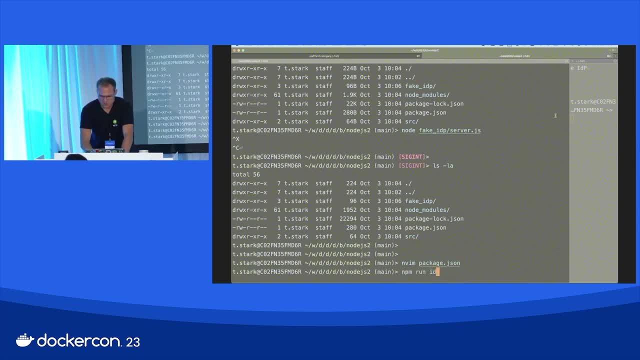 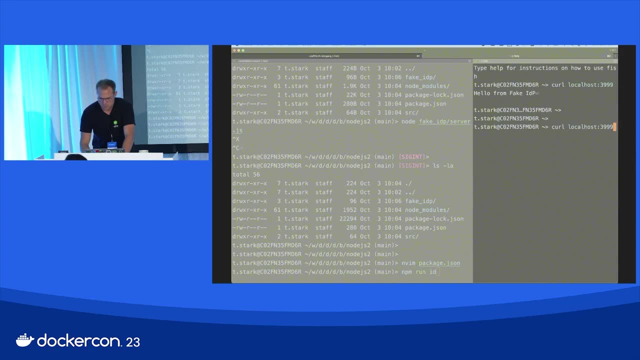 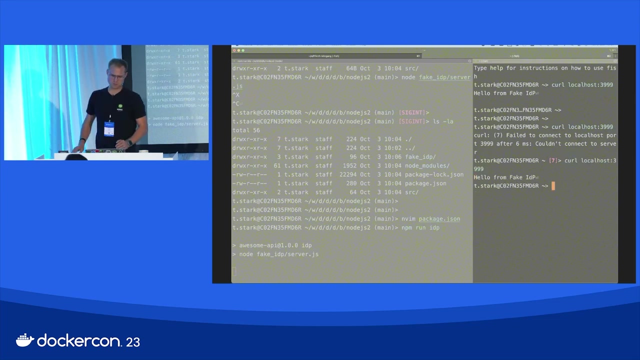 So, and then when you do npm run IDP- oh now it's already running, isn't it? I think we stopped it, Yep stopped. So it's npm run IDP. and then we say, okay, it's working. 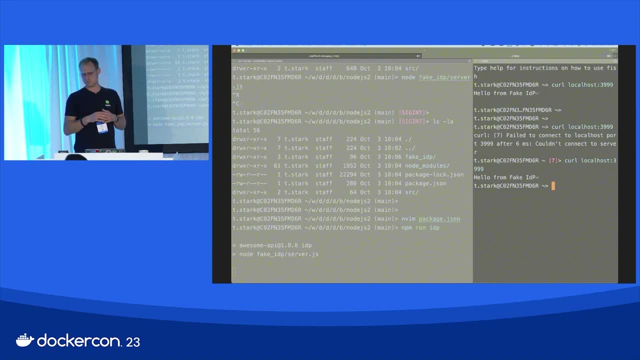 Again, it's very, very, very small thing to do, Just adding it to the package JSON, but it will help another engineer to understand what you're actually doing, Right. So put it in for what is worse, And this is the. these are the difference. 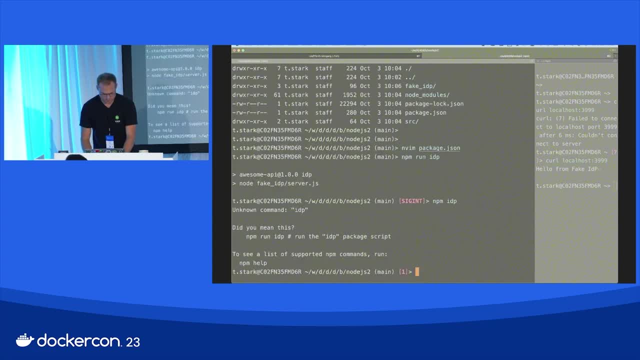 If we do, it will basically tell you what the. I have no idea what IDP means, But it would know what start means. but it would look for an indexjs file because that's what we specified in the package JSON. So anytime you need to execute a script. 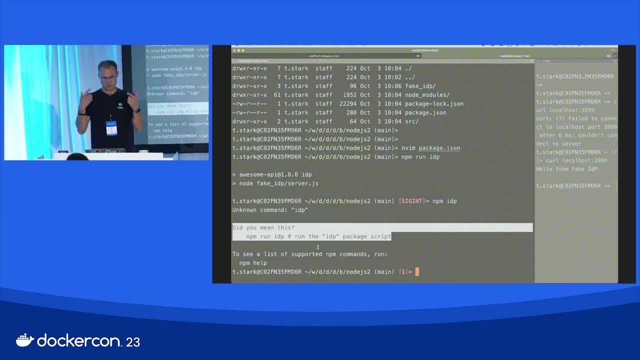 and that's basically what this thing is saying here. if you want to do this from the script's package JSON thing, you have to tell npm that you want to run a custom script and that is in package JSON. So npm run. IDP works in this case. 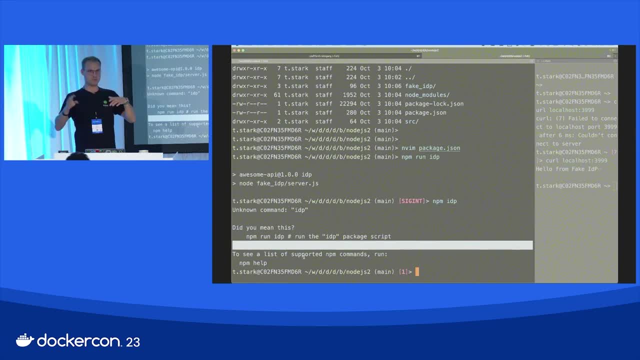 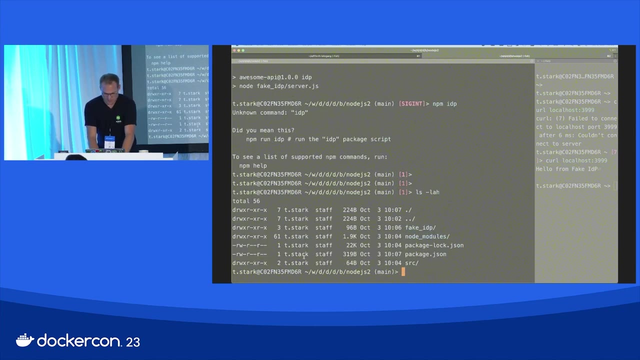 Okay, Just, I see this question from time to time. what are the difference between npm run- start and npm start For start? nothing For something you create. it will not work without start or run. Okay, Good, So now we have this API. 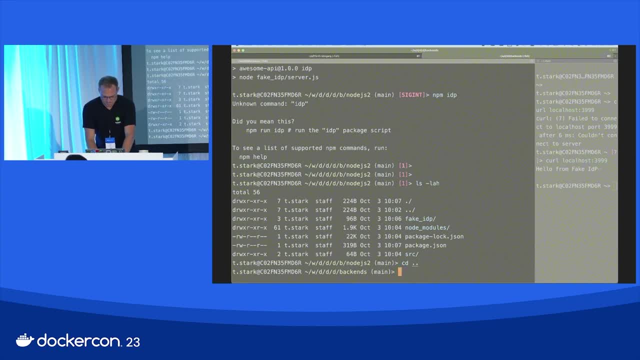 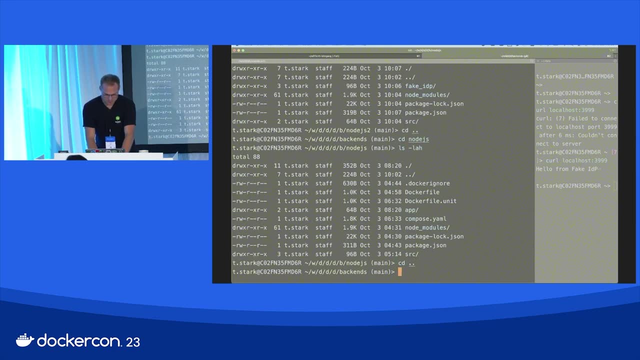 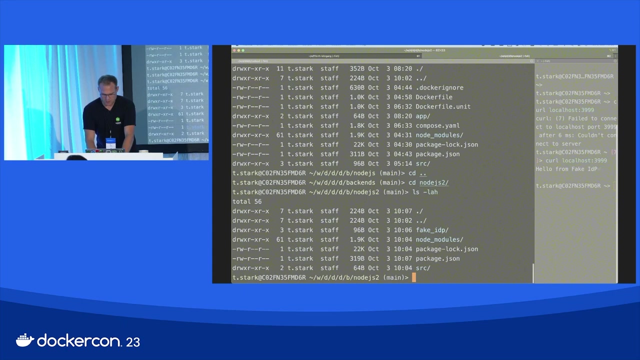 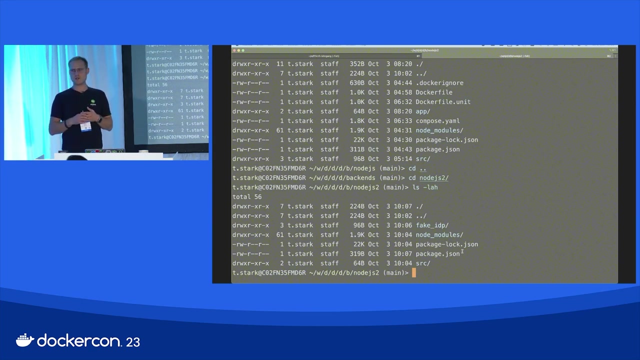 Amazing. So let's check nodejs and use docker init In our nodejs2 thing. So there's no docker file in it, There is no docker compose file in it, and now we can create this by ourself. or, if you would like to get started with something like this: 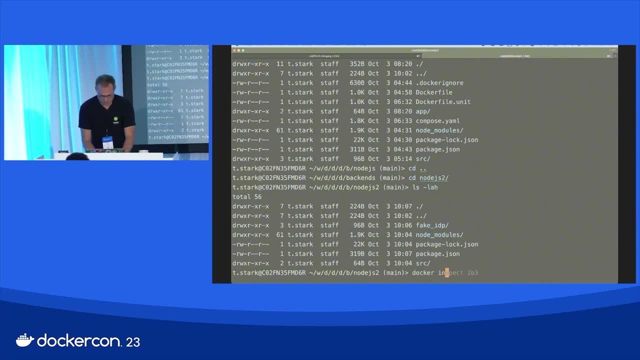 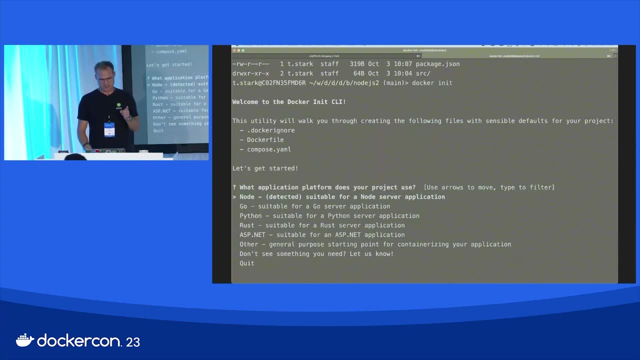 we can use a new command that's called docker init. It's like npm init, Just. And one thing that is important: I'm just hitting enter, it will initialize a docker project. but one thing that is important when using this: I'm not sure if it's this behavior for all the languages, because I haven't tried all the languages, but for nodejs and PHP. thank you for nodejs and PHP. it is super important that you do the npm init or the composer stuff first. 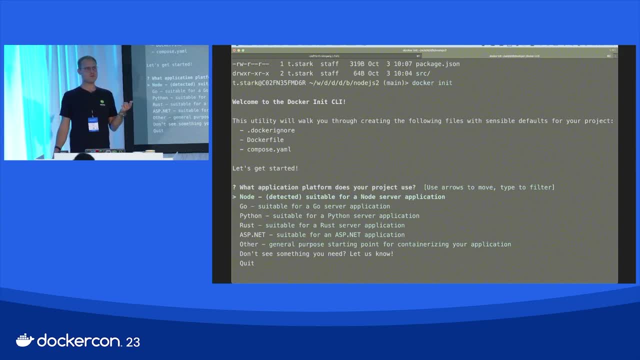 and then do the docker init. If you do it the other way around, for example, if you do docker init first and then do npm init, it will tell you: hey, there are already a docker file and stuff in this directory. I can't create new files. 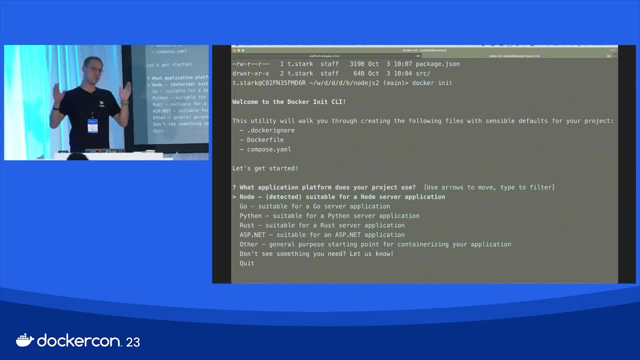 because I might override things, which is bad. Don't do it. That's why the ordering here matters. Do your npm init first and then, if you're ready, do the docker init afterwards. So in this case we type docker init. 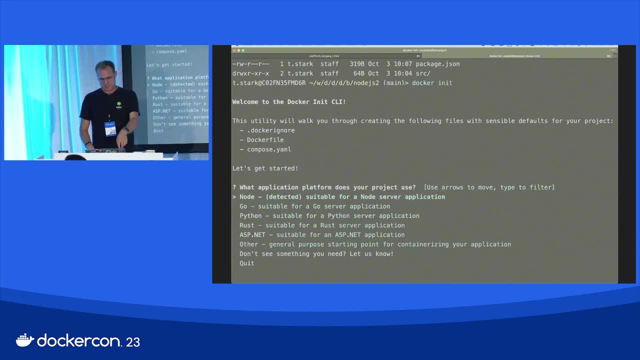 and then we can see: okay, And another thing here: you see it detected nodejs because there's a package JSON in it and there's common files in this directory that lead to the expectation that this could be a nodejs project. 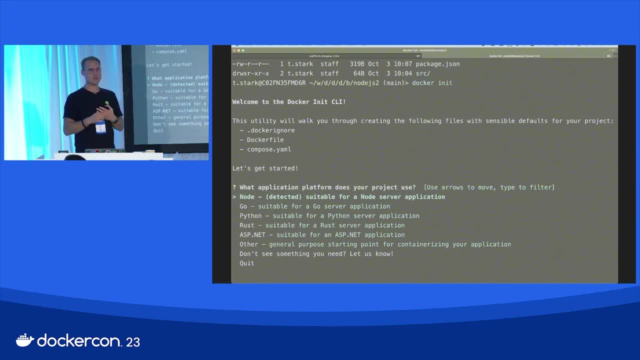 So nodejs will already be on top of this list, Another reason why you should always start with the project code first and then do the docker init. Okay, nodejs is right. Perfect, Enter. What version of node do you want to use? 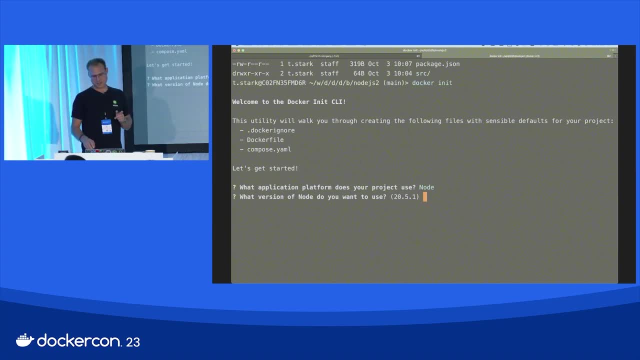 Okay, now look at the version 25.1.. And I will tell you another thing that is super important when working with docker and engineering in general: Enter: Which package manager do you want to use? That was your question. We can use npm detected. Perfect, Or we can use yarn, which is another package manager. Please don't ask me which are better Personal preference. It's like if I ask you if you like green or red, You like green, I like red, Whatever, There's no reason. 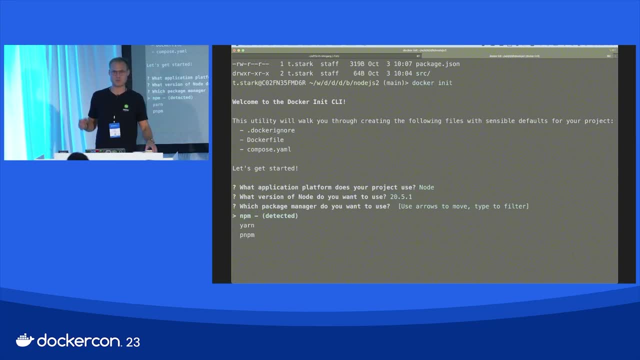 It's: you love red and I green. That's fine. We can live very, very good next to each other. Yes, We can have a chat about it at some later time. It's the same question that people ask me: Should I use Maven or Gradle? It depends. As always in software engineering, it depends Whatever you want. There are some things that work better in Gradle than in Maven. There are some things that work better in npm than in yarn. For the normal use case it doesn't matter. 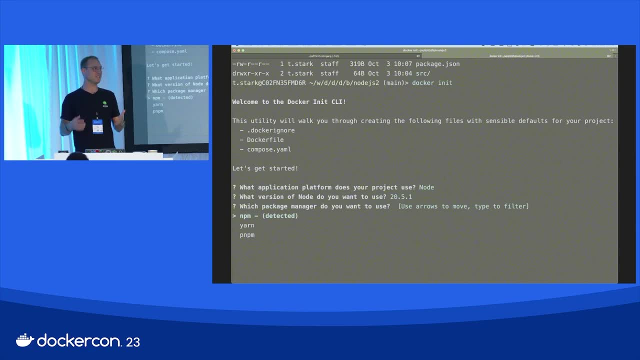 For some specialties it matters. That's why I'm saying it depends. In my case, I'm starting most of the time with npm. Good, What command do you want to use to start the app? So now it's saying node indexjs. 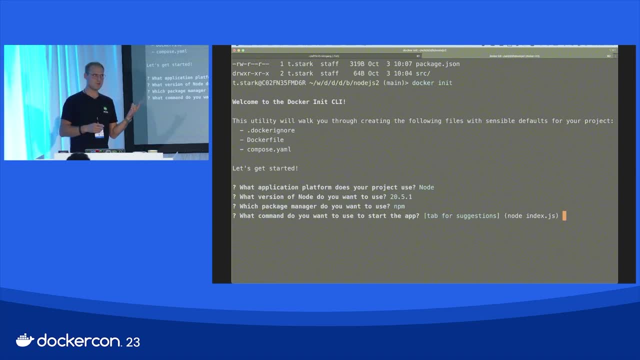 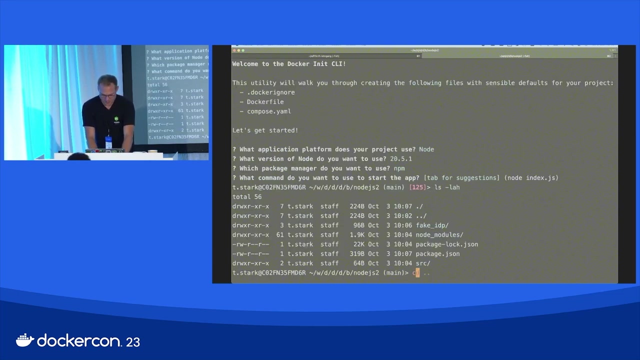 Okay, If we remember what we did previously in this thing, it was some. We did not create an indexjs file, Okay. So actually let me cancel that and do something. We have this fake IDP, which is fine. We have in source. 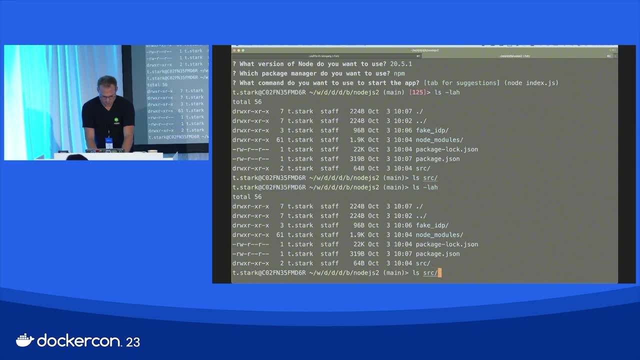 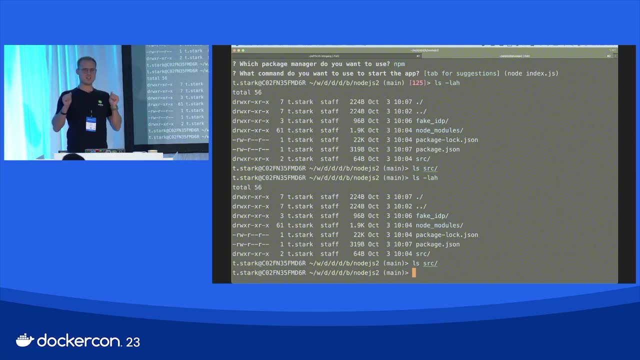 We have something in source. No, it's empty. This is another thing. People try to put an indexjs file into this root directory. I don't know. You can't do this. Technically, there's nothing wrong with it. 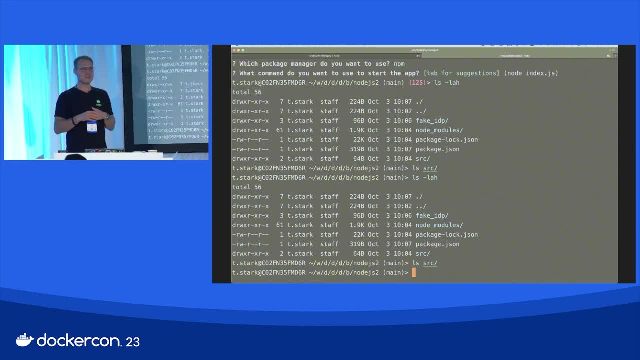 I just don't like it. I don't like. To me this is like I don't know An indexjs file in the root directory that's. I don't know It's. I would feel better if it's in a source directory. 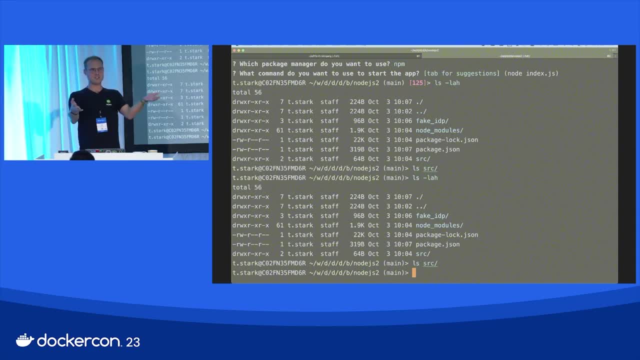 Something that tells me: hey, there's your source code And the indexjs is part of the source code. Maybe that's my little monk in like, for whatever reason, But this is Yeah, Let's create it inside of indexjs. 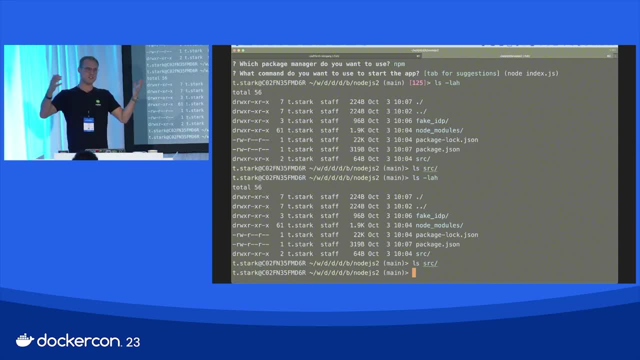 Hmm, And then you can think of: is it indexjs? If it's appjs, is it serverjs? That's totally up to you. Just make it. Index is the index of the project, which is fine, Call it mainjs. 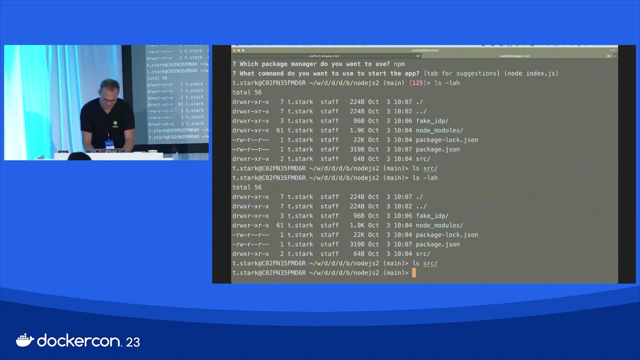 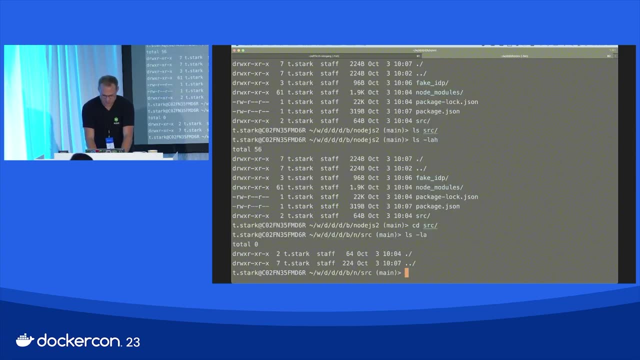 Call it whateverjs, But don't put an indexjs file in the root directory, for whatever reason. It's Create a source directory and I'm fine with indexjs, Right, So So let me actually use the serverjs. 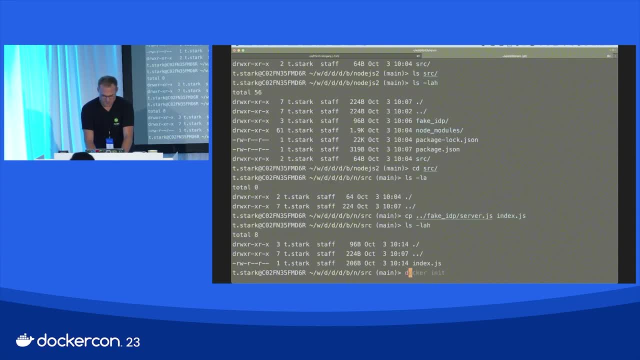 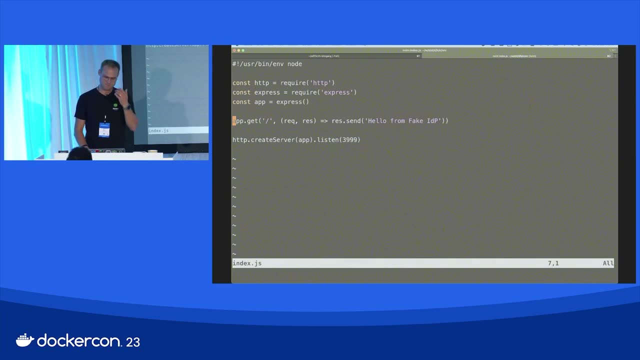 And I will use indexjs, not server. I use server for whatever reason It's- I don't know why It's- As it spins up a web server. I use serverjs Because it's a It's a server. 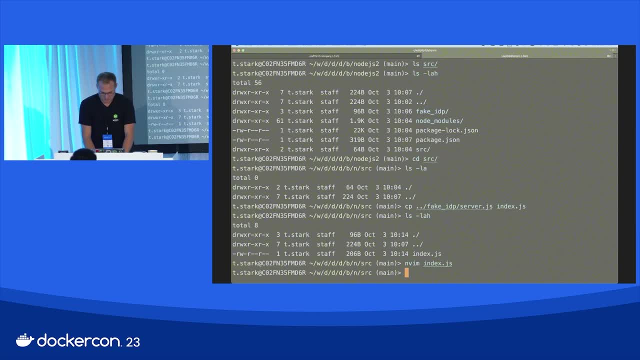 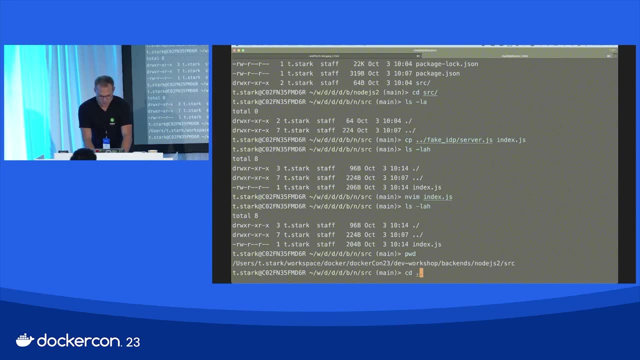 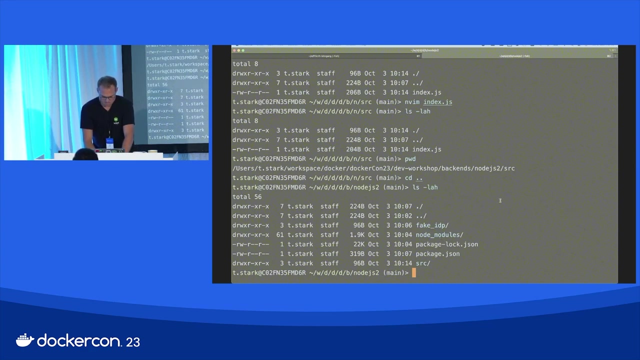 It's like, Okay, Good, Now we have inside of this directory, we have indexjs And we are in backends nodejs and source. Okay, And if we run now inside of this, The docker init again Node Fine. 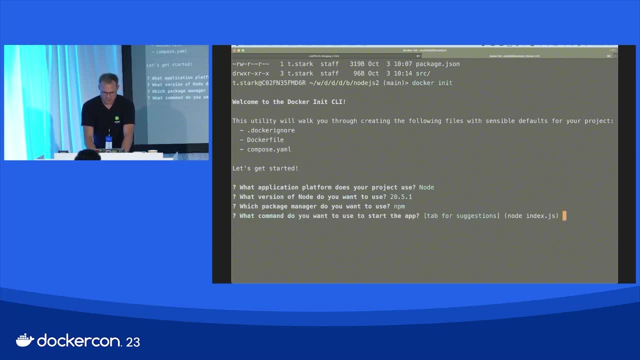 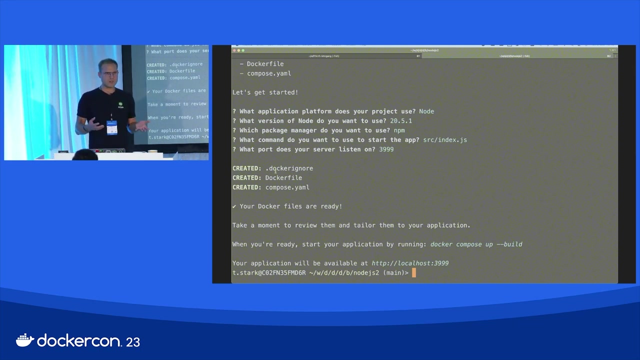 Yes, So it tells node indexjs. And now we have to tell him it's in source indexjs. And what port do you want to listen on? It was 3999.. Good So, and now it automatically created a docker ignore file. 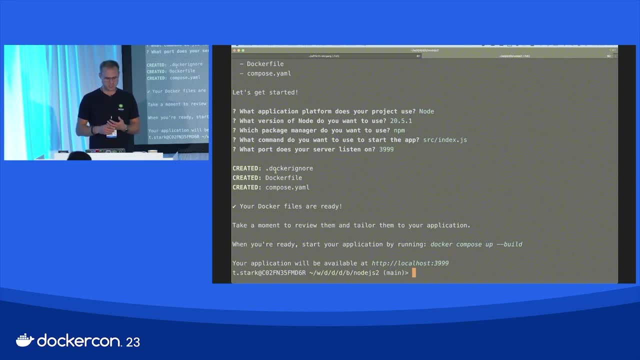 which should have the node modules in it. It has a docker file now and it has a composeyaml file. The composeyaml is the new name of the docker-composeyaml. It was docker-composeyaml a long time, for a long time. 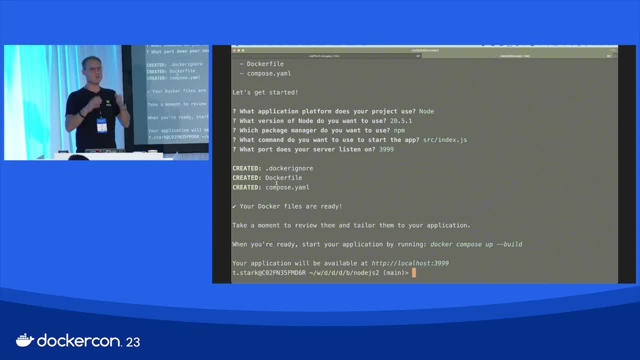 and now it's just composeyaml. It will work with docker-composeyaml as well. Side note: right, But I recognize while using docker init that docker now names it composeyaml. So all the directories I came across I have created. I'm about to rename things to composeyaml. I just want to avoid that with some newer compose version they deprecate docker-compose and if you not have a composeyaml in your directory they will not work anymore. Another tip If you see something like this happen: 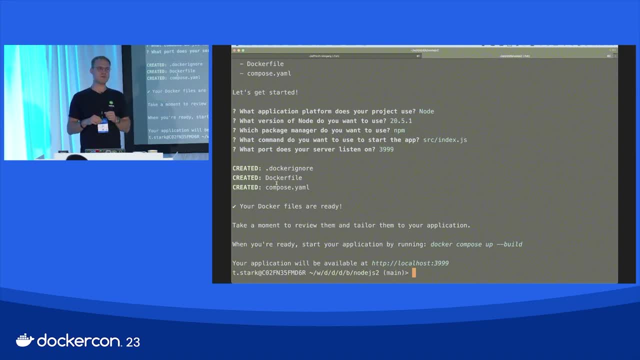 from time to time. make sure you spend at least a minute to think about: hey, why is it now composeyaml not docker-compose? Try to research things like that and understand why is it like this. And if they tell you on the website, that's fine. 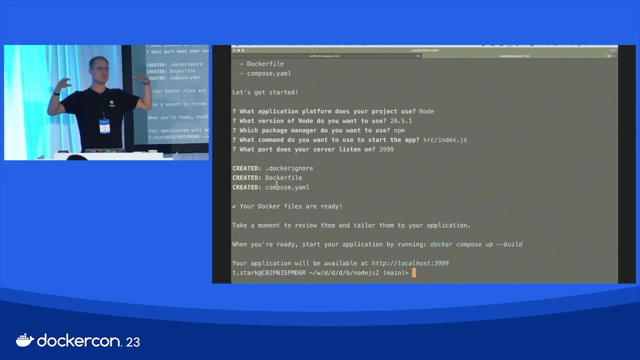 docker-compose and composeyaml are identical and we are not about to deprecate one of these, fine, keep it. But if they are saying, hey, docker-compose is old, compose is new, and we will deprecate docker-compose, 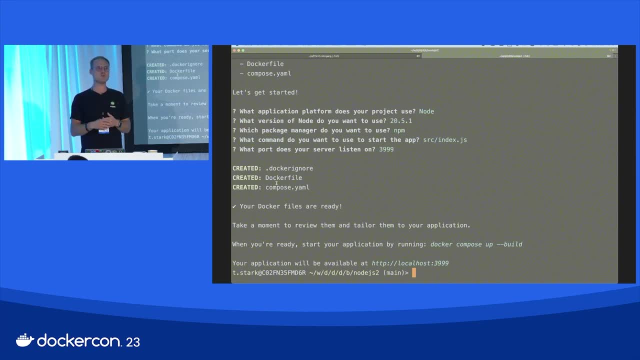 in one of the newer versions. make sure you spend some time renaming things Just to make sure it will not fail one day after Christmas just because we have a wrong file name. that would be bad, All right. so now let's check what they did. So docker-composeinit created a docker file, a docker-ignore file and a compose file. So now let's check what's in docker-ignore. Okay, what is docker-ignore? Docker-ignore is similar to what is git-ignore. Git-ignore prevents. 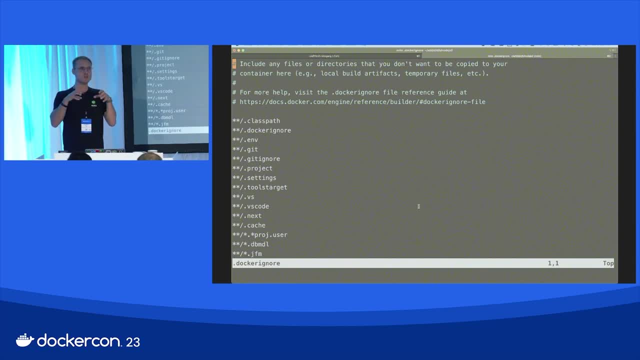 specific files or directories from being pushed to the remote repository. Right, Clear, Okay. Git-ignore or docker-ignore is something that is similar to what docker-build is doing when you have a copy command in your docker file. In your docker file you have copyto something. 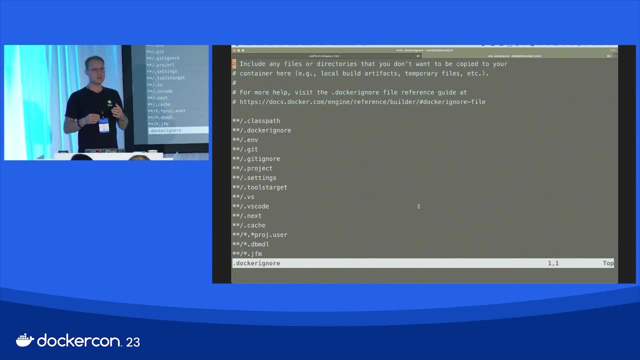 inside of my container image. If you do not have some stuff in your like- there's nothing defined in docker-ignore- it will basically copy everything that's in your directory into your like container image. Sometimes you don't want this because a docker file. 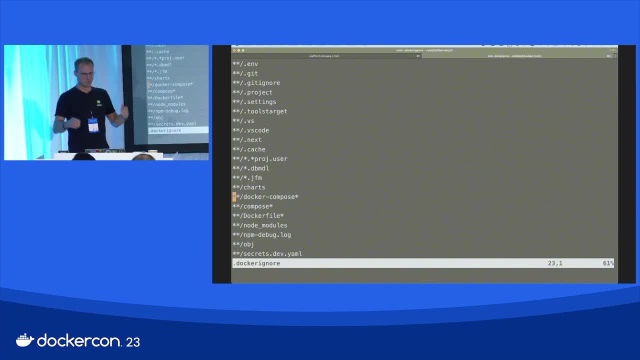 here a docker-compose file like vs-code, next settings, project git-ignore, like build, whatever stuff is. you don't want to have that in your, in your production image, Neither the docker-ignore file, Right. 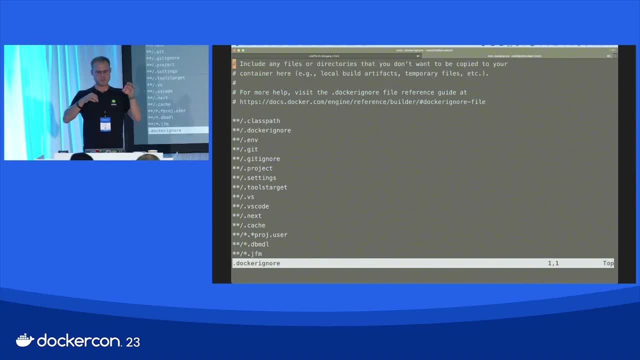 So- and this is when we type now docker-build- it will look into this directory and will not copy the files and directories that you mentioned in docker-ignore. Reason why I'm saying it: I saw at least a hundred times where people are doing copy slash source to slash source. 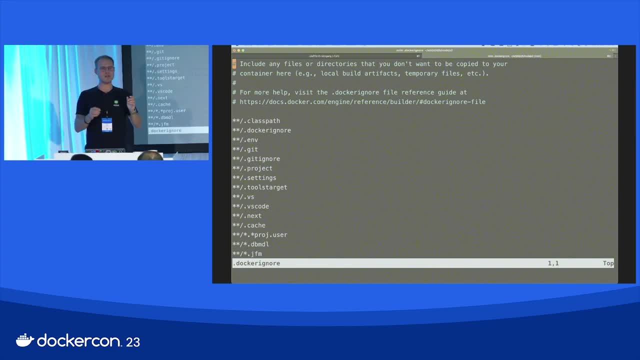 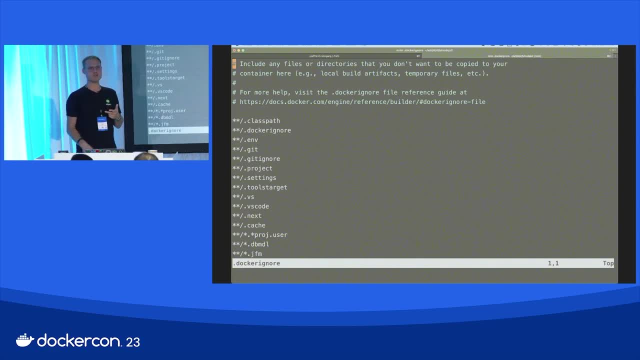 All right. so you wrote 150 lines in your docker file just because you don't want three files in your image, and you never thought about that. there must be a better way of doing it. this way Interesting. Let me tell you what. 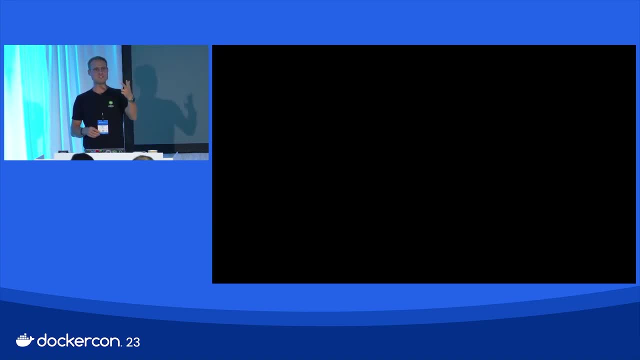 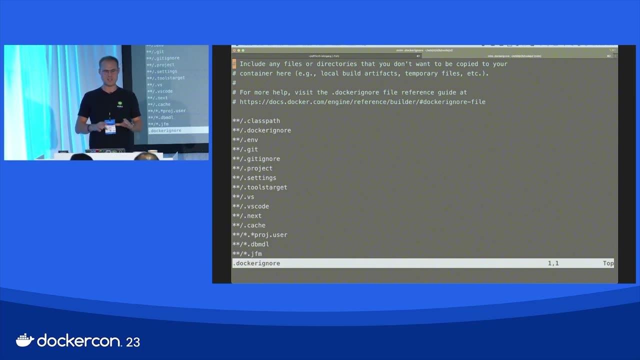 You can simply use a docker-ignore file, put these three things in it, delete 150 lines from your docker file and just copy dot slash to whatever. It's amazing If you look in the faces of people when you explain something like this. that's amazing. 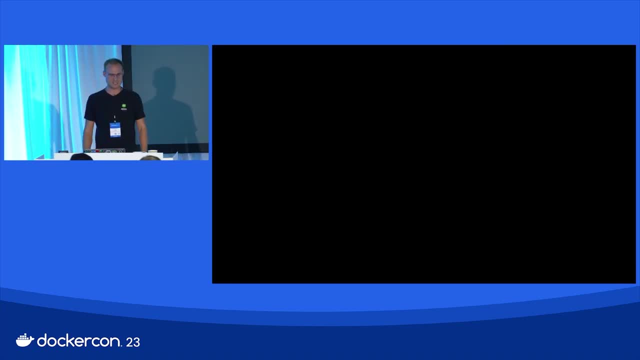 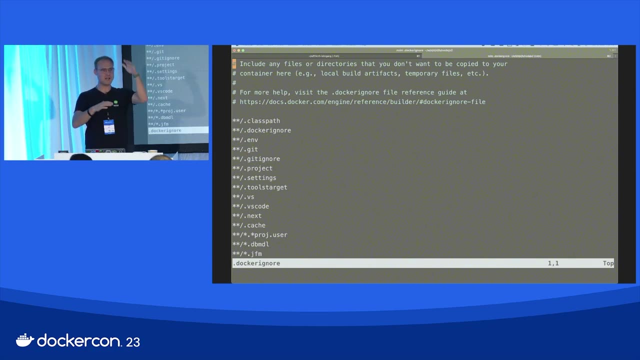 It's like: are you kidding me? Are you real? Yes, it's real, Yeah, fine, Okay, thank you for nothing. That's why I'm saying it: Use docker-ignore. Don't put 150 lines in your docker file. 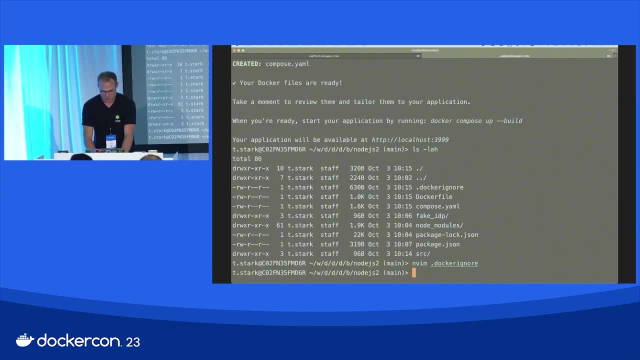 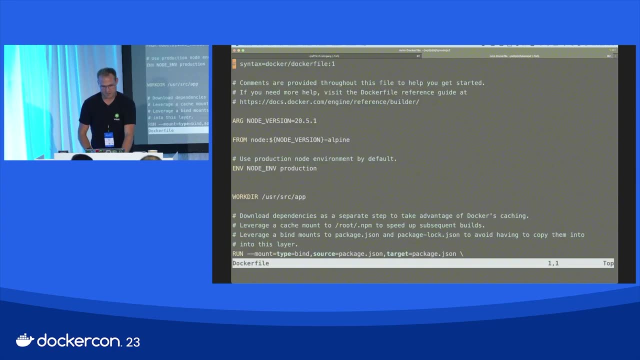 I mean you can do, but it's not efficient. That's why docker-ignore exists. Okay, so that was generated. And now the docker file. Yes, Why is the docker file with a capital D and everything else with a lower d? 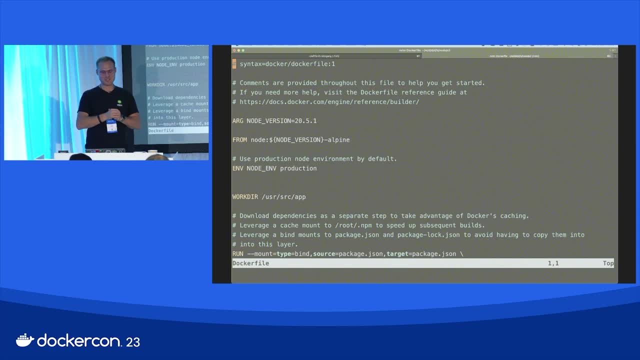 Jesus, that is a good question. The question was: why is the docker file with a capital D and everything else with a lower d? That's interesting. I'm pretty sure we'll find out over the conference. I have no idea. I've never asked myself this question. 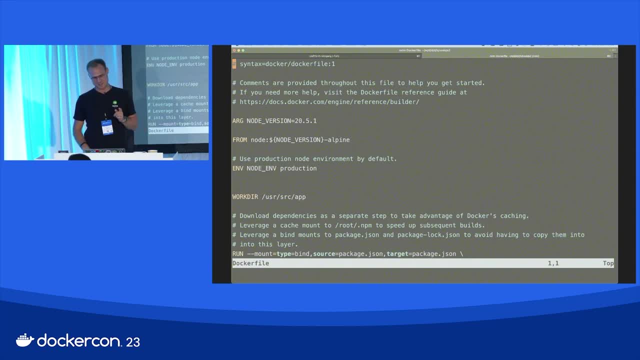 Now I'm a little bit embarrassed to ask this question- Why docker file has a capital D? That's a very good question. I have not the answer to that question, which is: but I, that's amazing, because that's I will have definitely. 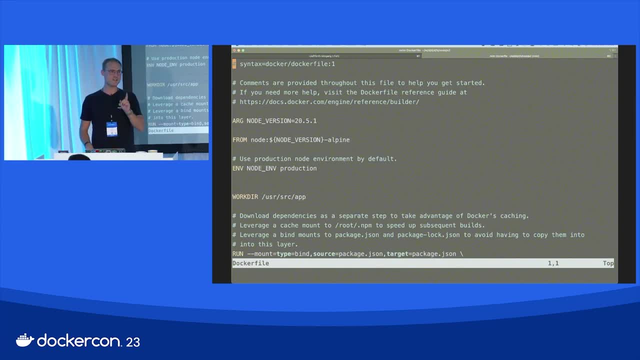 learned something new at this conference, because then I know why. I hope we will find an engineer that will tell me why we have a capital D and not a lowercase d. I hope we will find the answer, but I don't know. Okay, good point. 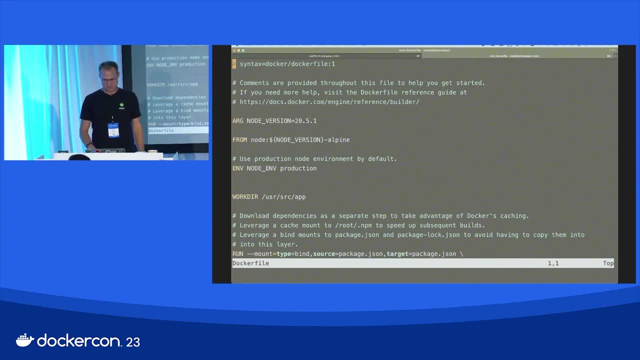 Good, Now we have a docker file. All right, It looks a little bit different from docker files, you might see, and this is because, of course, docker init uses docker best practices. Makes sense, right, If we have something from docker. 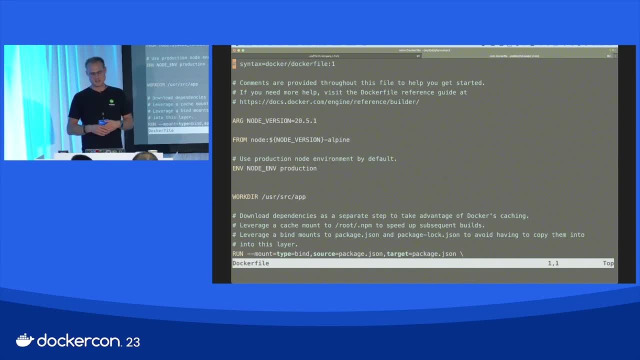 that's called docker init. it would be great if it generated a docker file that uses best practices, but most of all, they put a syntax docker docker file in it. This helps vim, nano, nvim, whatever- to detect or to understand. 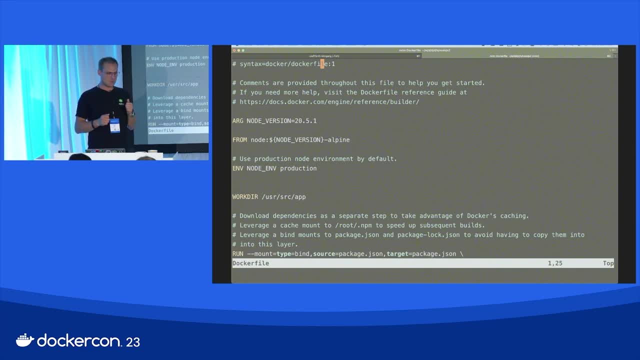 what is written in this file, because what you can do is you can write your docker files in a way: capital D docker file, dot, production, dot, def, and sometimes, if you don't have this syntax thing mentioned in this docker file, this example will not show. 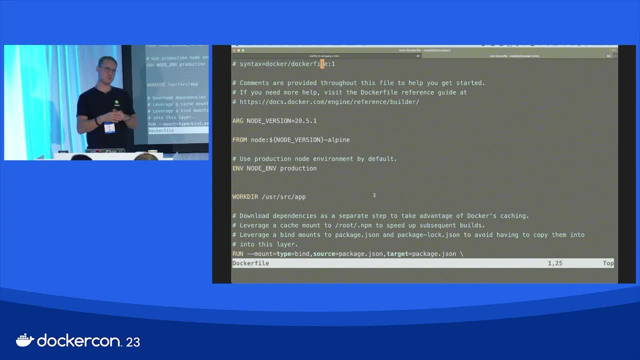 nice, shiny syntax highlighting because it says, hey, this is not a docker file, It's a docker file dot production. Don't know what this is, So that's why, from time to time, it's important to put this syntax thing in it. 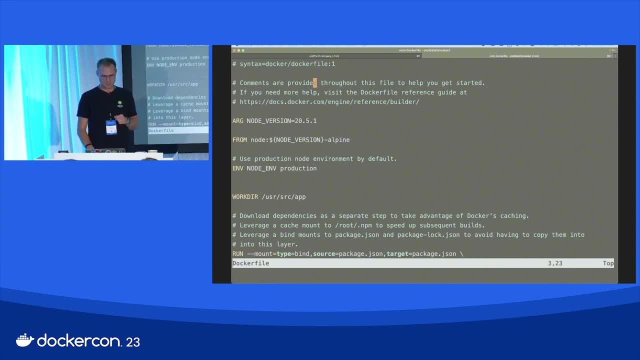 It does not do anything with the docker file, It's just for your editor. okay, So, and then we have an argument that is node version 25.1.. Good, Then we have this from which says: node colon: node version: dash alpine. 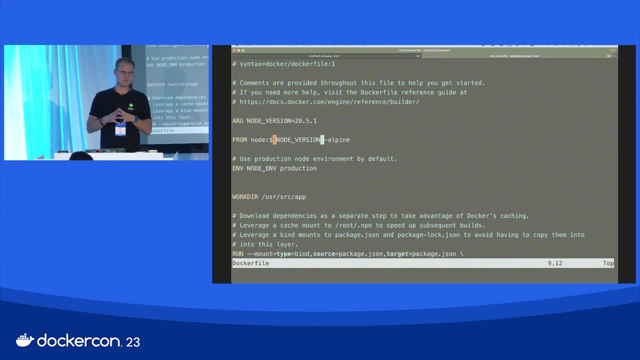 Good, So show of hands. Who in this audience uses in the docker files in general from something colon latest. I used that like a million times. It's not a problem, It is dangerous as something. Why is it dangerous? Why you should never, never, ever use. 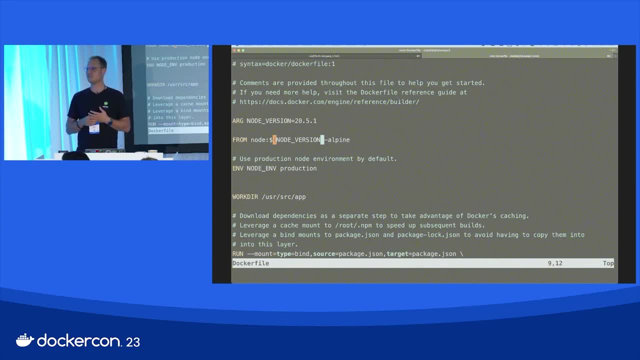 latest. Yeah, It will pull the latest, Sorry, Oh, you don't know what I'm talking about. Okay, Then I will explain what I'm talking about. If you take one thing out of this lesson, then please stop using from latest. 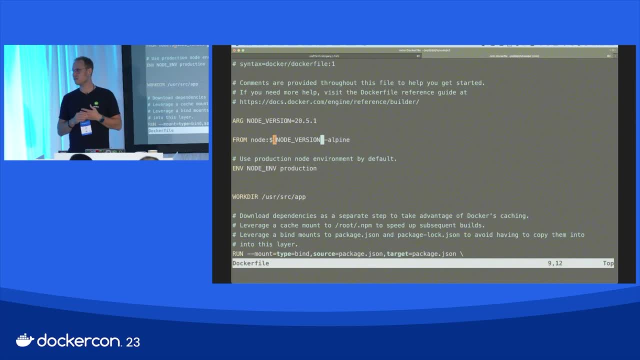 And I explain you why. Yeah, For example, right, So I can tell you what, And this happened a couple of times to me. This is why I'm explaining it. That's the most lessons learned from this session, From, and then node latest. 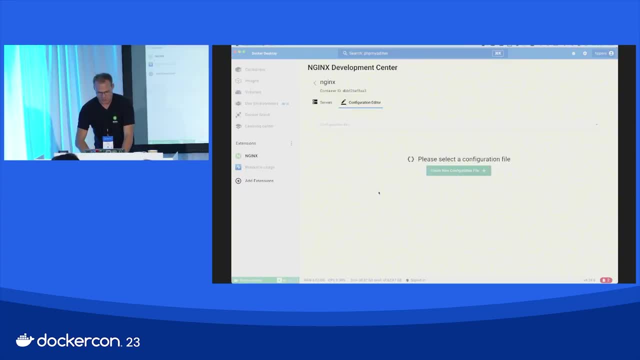 What will it do? Let's use our nice docker desktop thing And go to images, And you can, and you can, or to search and then search for node js Or node Okay, So we can do This here, or same thing. 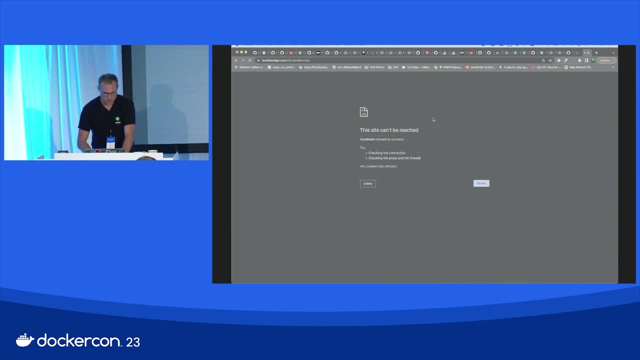 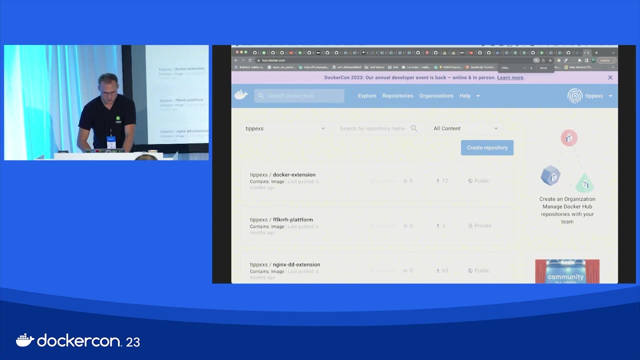 because I've just learned it's. we do not have all access to docker desktop right now. Let's use the docker hub. then It's the same thing. Go to docker hub, We load it, We type, node Good Tags. So 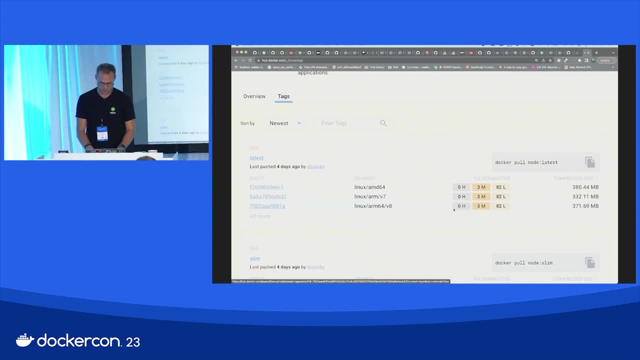 So Tags are like versions we can define for given docker images, And latest is a good thing, Right, Latest. if you use it, Then latest is a good thing Because it will always pull down the latest version of a given image from the repository. 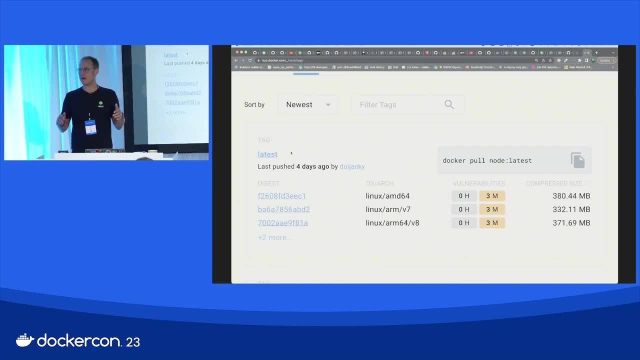 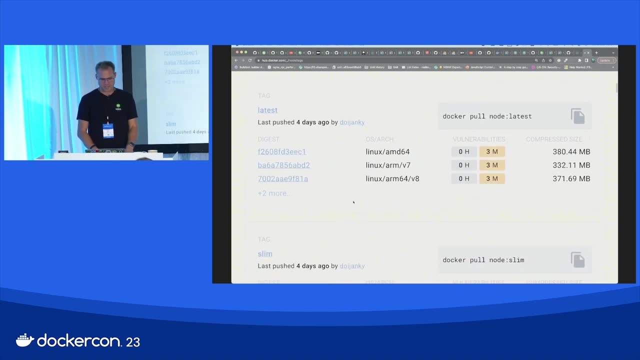 If you would like to use the latest version with all the updates in it, you can totally use latest Good Perfect. So, For example, Latest was updated four days ago, September 29th, at 4pm. Perfect. So Then we have some other tags. 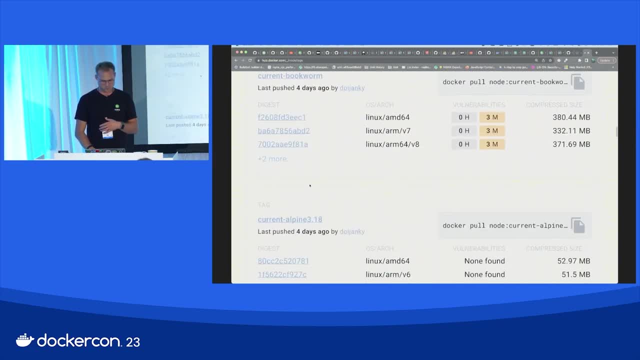 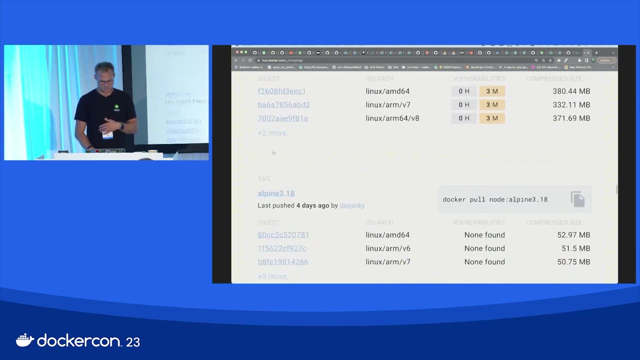 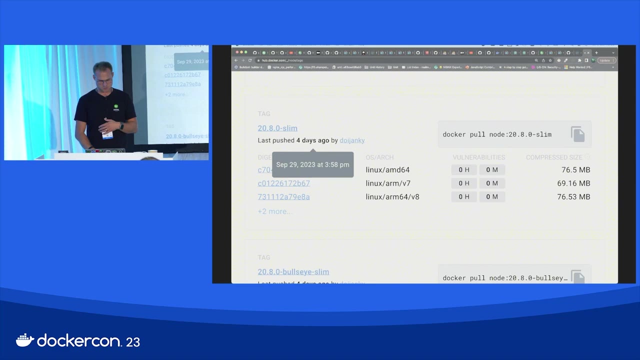 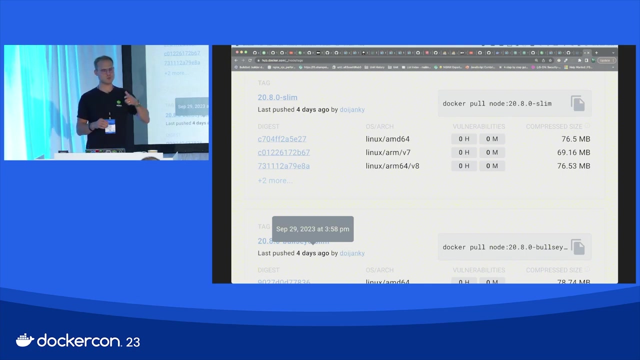 We have slim, which are basically like smaller containers, And then We have current Alpine. We have current Mm-hmm, Mm-hmm Alpine Alpine. So So this is like this was two minutes before the latest one. 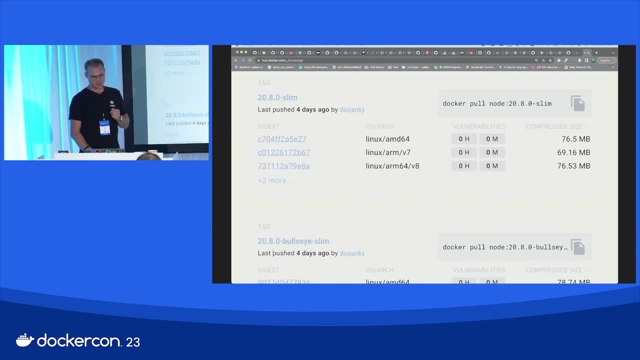 So that means that maybe, maybe or with high chance, the note version in this latest one is 20.8.0.. Agree, Likely, If we pull down the latest image, it will have 20.8.0 in it. Perfect, Good. 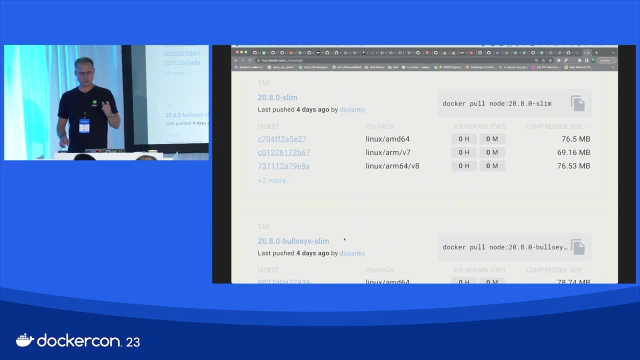 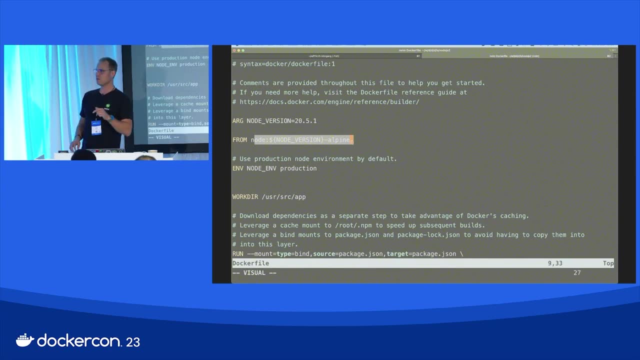 So If we use latest in our build image, like in our from here, You run docker build today And you will get 20.8.0.. You run docker build three weeks, four weeks, six weeks ahead, You will get maybe. 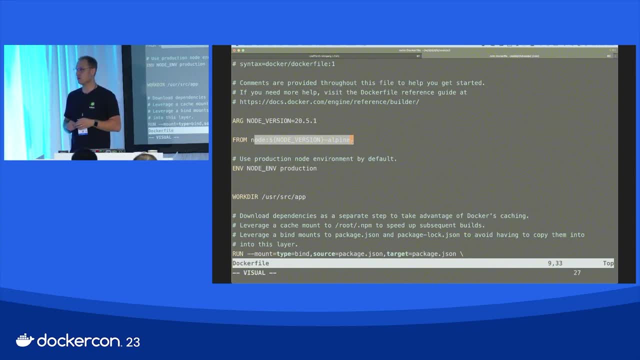 20.9.. something Or even worse, you will get 21.something, with a breaking change that all the things you do with 20.8 are not longer working. Not nothing, Not at all Like nothing of the stuff you have used before. 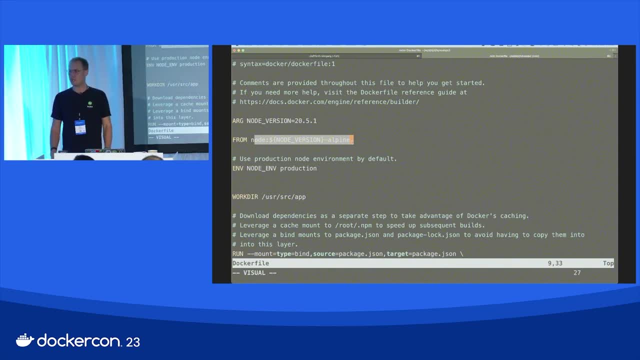 will work with no 21.. Maybe, And you will just find out by starting the image, Because the build might be fine. It will probably build absolutely fine without any issue, But you push this thing to production server and it will not work. 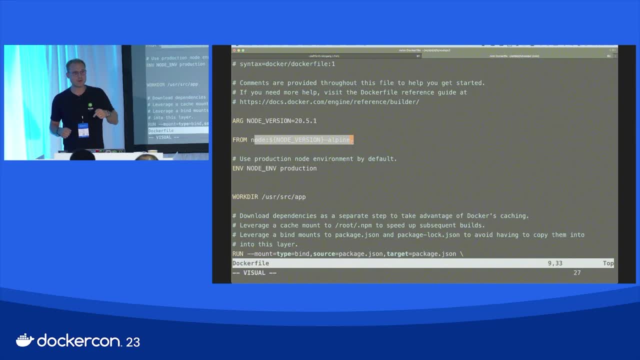 Or, even worse, some parts of your application will work and some parts of your application will not work. But you will not find out by the first hour or like the next two hours. Sometimes you will find out like hours, days later that something is somehow. 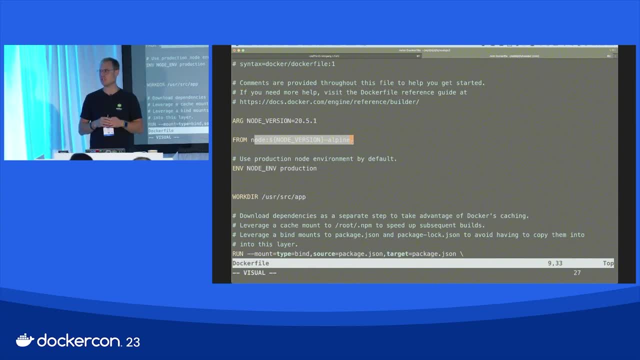 not working as you expect. Then you are trying, investigating and say: why do we have no version 21 in our like? who tested no 21 with our application? Nobody. So this is why, if you are doing it locally, you can definitely give latest a try, right? 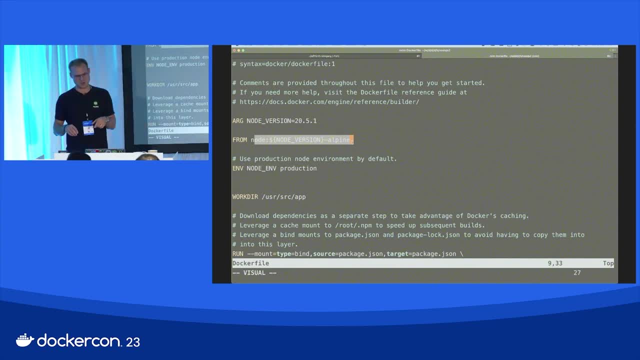 To get the latest version. But the reason why I am saying it: be careful with that. Start doing it right from the beginning. Stop working with latest. if you are doing stuff, Go to the docker hub or docker desktop extension and see what is the latest version. 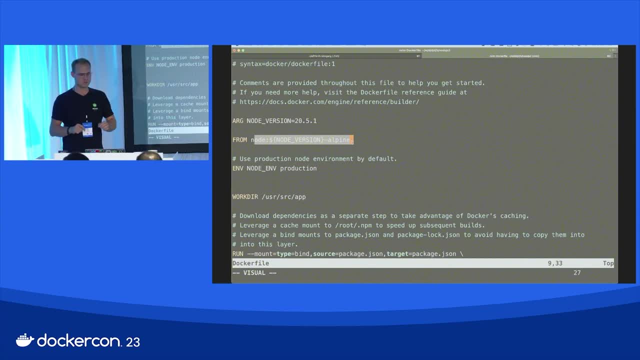 and then define it explicitly. I want to use 20.5.1 dash Alpine Good And if node comes, for whatever reason, to the crazy idea we don't want to ship a node like an Alpine version anymore, this build will fail. They have to delete. 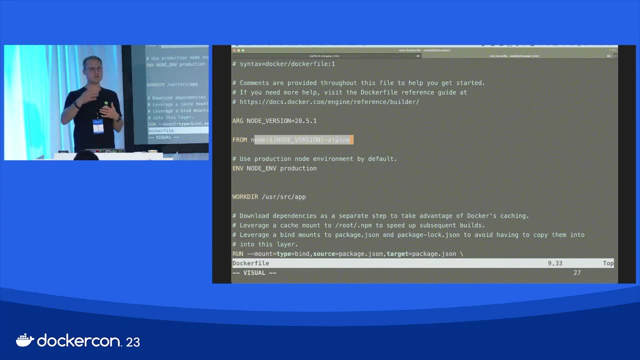 the Alpine image from the repository. but then the build will fail. You will not push anything into production that is not working anymore. You will recognize it very early in your stack that something is not working well. So that's why this argument from thing here is one of the most 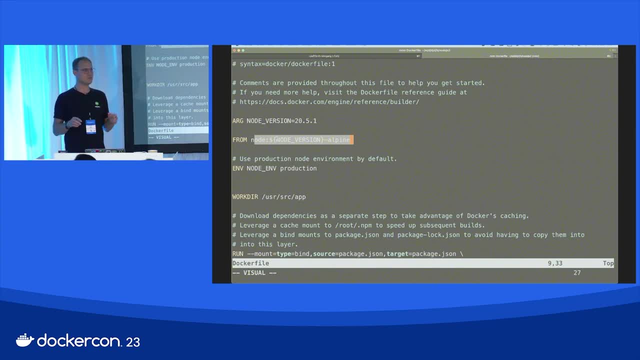 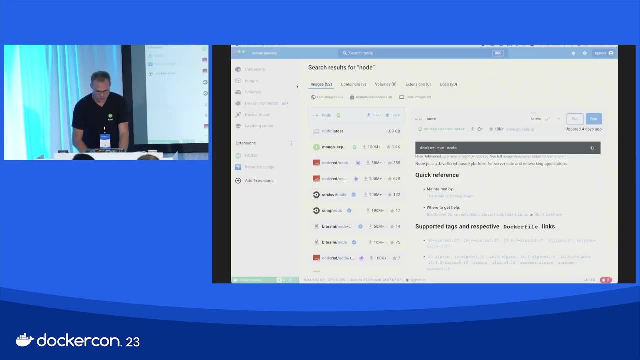 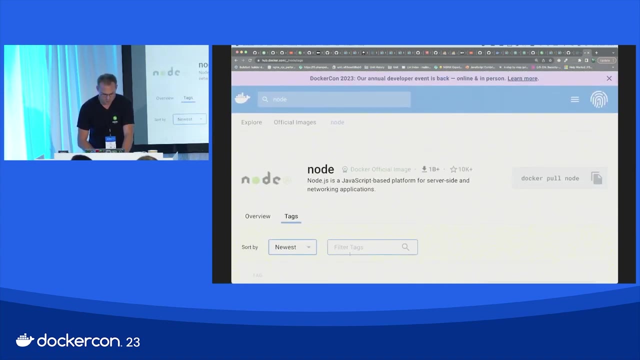 important things you should learn to use. Define a version that you want to use And the node version. for example, they come with this tagging: there is probably a version that is called 20.5.. I'm pretty sure there is. They have 20.5.1. 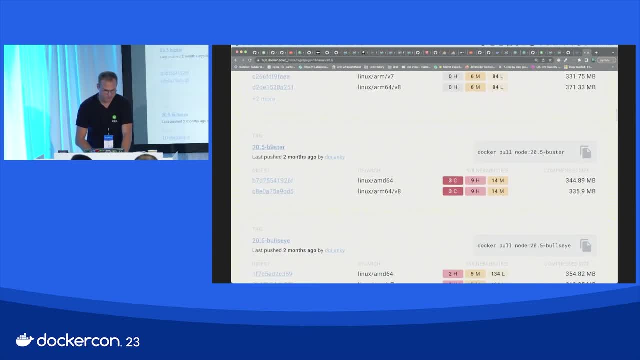 20.5.1, 20.5.1 here, 25.. What does it mean? If you define 25, that means if they push 25.2 tomorrow, you will get 20.5.2. if you use 20.5. 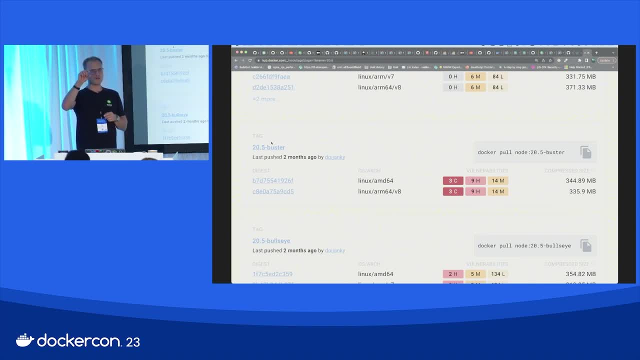 in your image. You will get the smaller version updates, but you will never go to 20.6.. Never, And this is something you have to think about. If you're fine, because not, and this is again usually- usually it will not break These smaller. 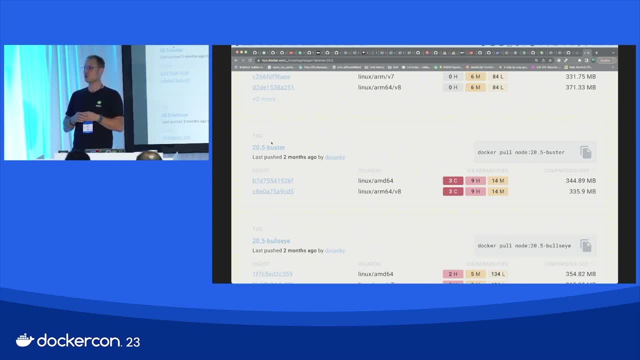 version. changes from 20.5.1 to 2 should not have breaking changes in it. Should not have breaking changes in it. This is something you can tell your boss why you have to be in the office at 3am in the morning. 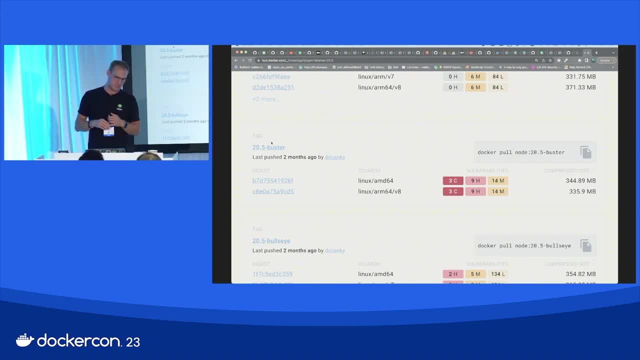 because, hey, we reverted the image. It's now 25.1 again. What was it before? It was 20.5.2 and it should not have breaking changes in it. but it had breaking changes in it, so I've reverted it, So it's. 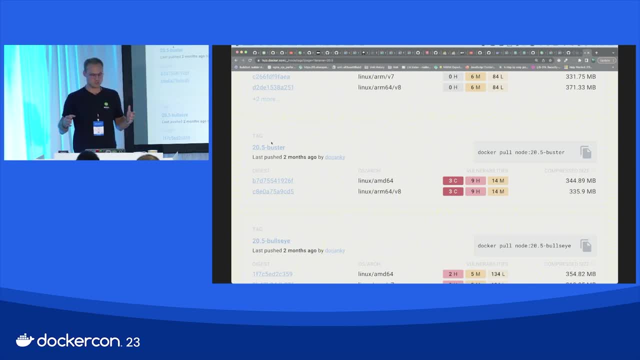 all working again. Okay, perfect. Can we do something that avoids this issue? Yes, we defined 20.5.1 the next time, So just to get an. I saw everything like this. I had problems with versions that were like bumps. 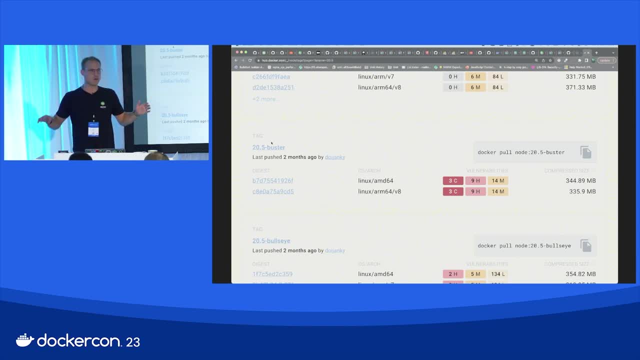 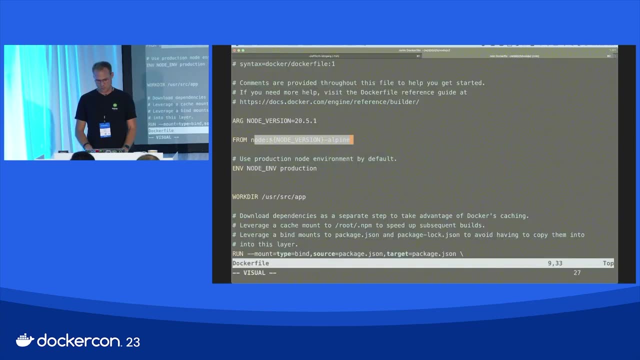 from 20.5.1 to and it was not working anywhere. It was a breaking change, even it was a small one. So that's why I'm saying: be careful when doing this. For what is it useful when we come to CI CD pipelines, for example? 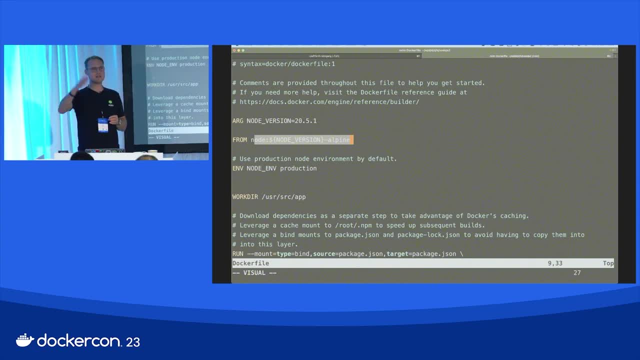 It is very useful if you have nightly builds of your application running it in some integration tests, Then you can use 20.5 always, because then you can see: hey, if you have your set of integration tests running at night you can, and then you can see is 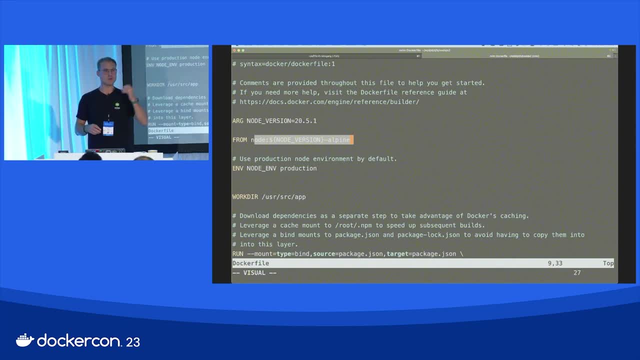 20.5.2 working or define 20. for example, Is my application working with node 20 in all major releases? they do from .5, .6,, .7, .8? Perfect, Then define node 20 in your pipeline. and build it every night and do the integration testing with node 20.. Or use latest in the pipeline and try if your application always works with the latest version of nodejs. for what it's worth, You can totally do this. That's why I'm saying it's not. 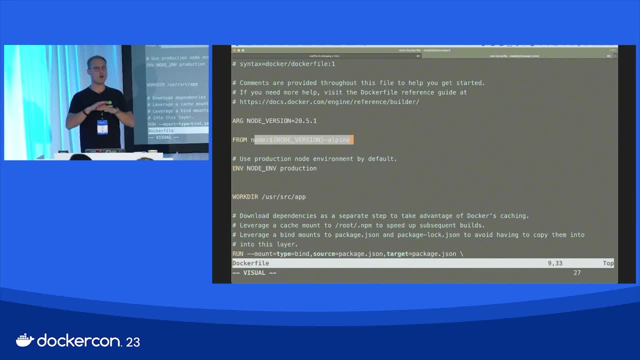 saying that latest is completely wrong always. It can be useful in very, very, very specific cases For your production builds in your pipeline. latest is not right For your nightly builds in your integration test pipeline. it is absolutely a nice thing to do, Just to be a little bit ahead of us. 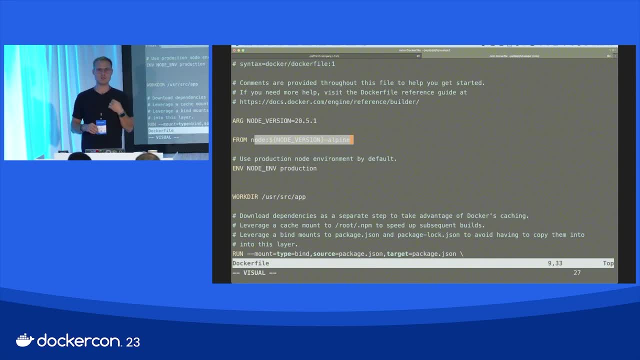 We at NGINX, for example, we have pipelines that use like better versions for PHP, Release candidates for Python. We have an application server- that's NGINX unit, and I would like to understand if our implementation of PHP and Python breaks with a future version of PHP or Python. 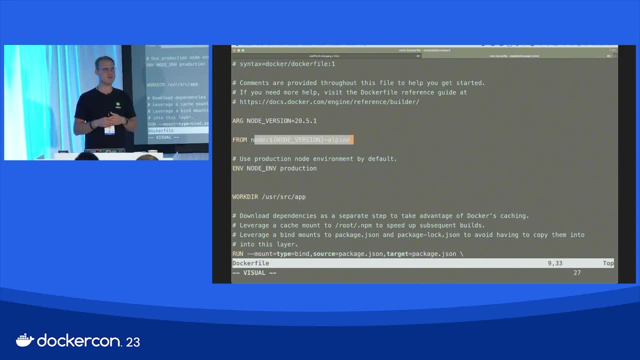 So I use the Docker images they ship with release candidates to test our application server against those versions, just to be a little bit ahead of the development, saying hey, if they have a breaking change in their Python or PHP 9, for example, which will come out soon. 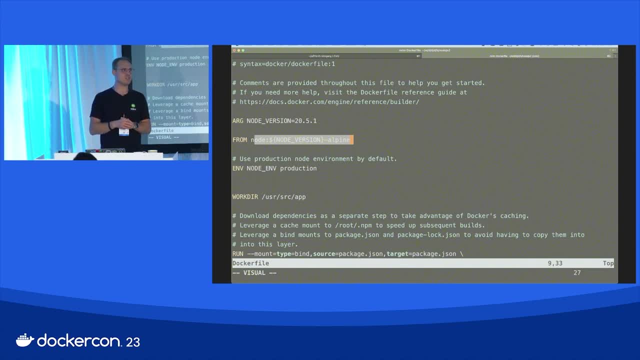 I would like to understand if my application server is still compatible with PHP 9.. So I use release candidates sometimes in our pipelines as well. Good So, this is super, super important. Good So, then we have Workdir. that's basically doing a CD inside of your build process. 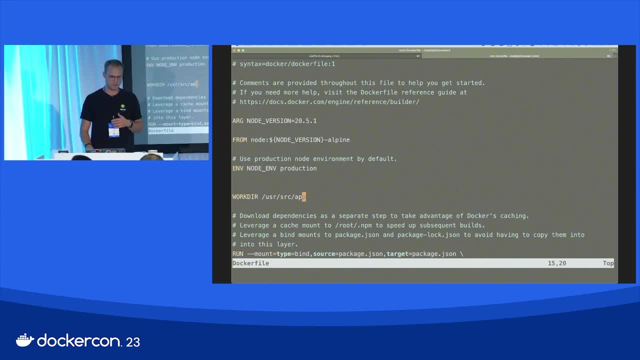 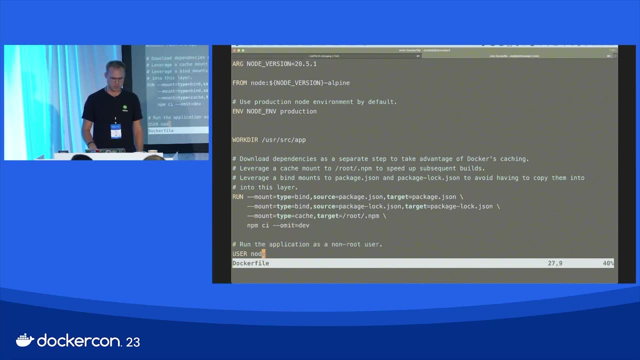 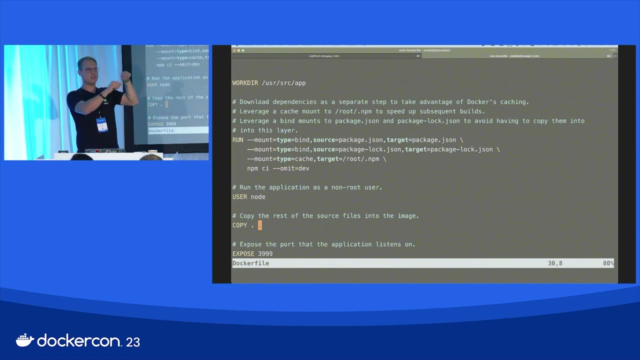 in your container. Normal Linux command like tell the Docker container. hey, this is my work directory and any time you're doing copy here will copy from Docker dot, like from the directory or Docker file is currently located. this directory into dot means into the work directory. 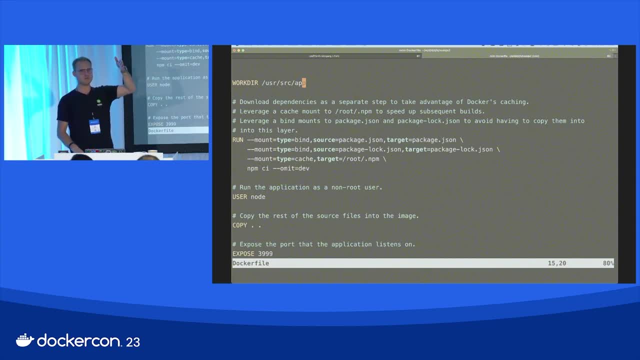 If you do not set work directory, it's root slash Okay. So this is another important thing that are not used so often, but it's very powerful when it comes to caching. If your images are small, it doesn't really matter. If your images 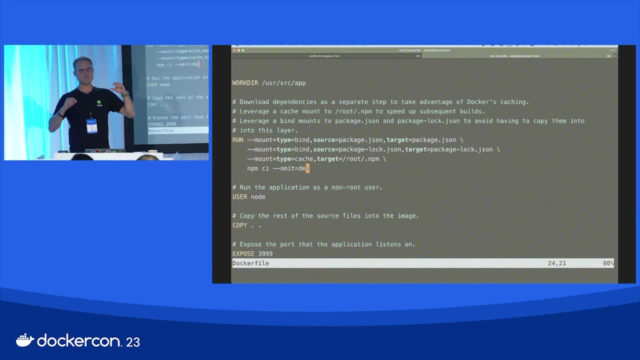 are bigger and you do a couple of changes in your image. I have to explain you first how that layering works and what happens if you change one layer. So the Docker image- there's a nice picture and it's too bad. I haven't it with me, but you can imagine. 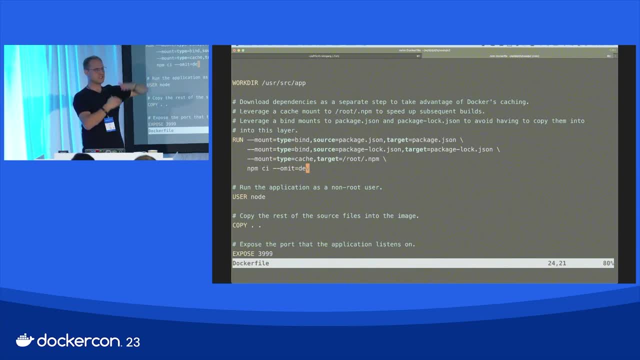 like and it's like a sandwich. and Docker container is like a sandwich. you have a slice of bread, which is your base image, and you put a lot of stuff on top of it, like salad and cheese and whatever you like- onions, and at the very end, if you start up the container, 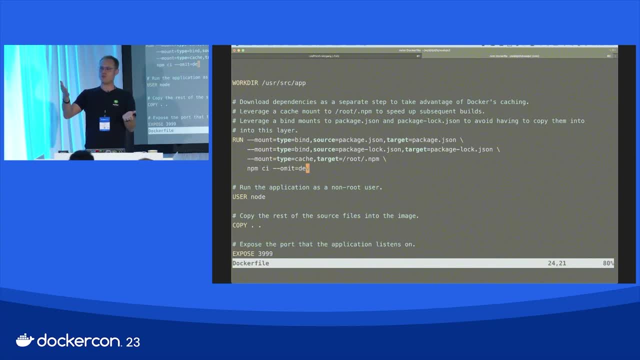 if you type this Docker run thing, you will put the slice of bread on top of it. Any time you run, you run your container, you will always put another layer on top of it because all the changes you do in your container, like creating files, changing- 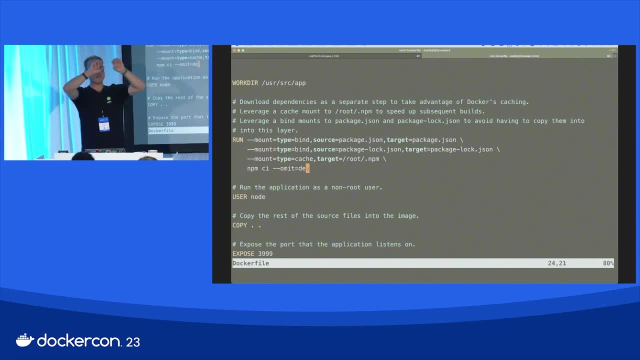 things will be represented in this top layer that will be generated when you type Docker run. If you stop the container, this layer is still there. If you remove it, it will be gone. It's not part of the image, It's part of your. 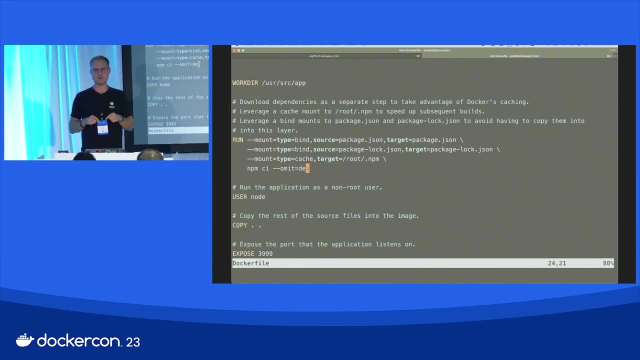 like it's a runtime thing. It's just on your host. It's not part of the image itself. This is how a container image works with this layered file system, So consider it as a sandwich. Okay, So if you have a sandwich with, 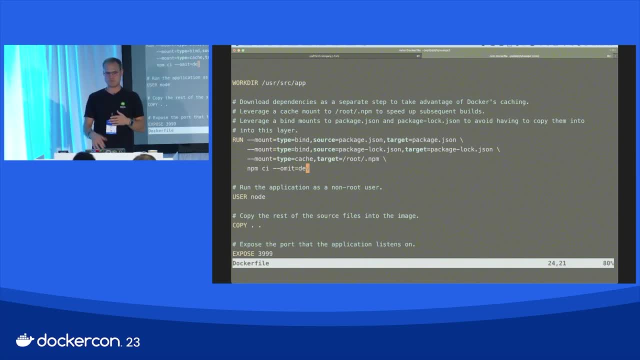 three layers, like cheese and peppers, like whatever ham and onions, slice of bread on top and you don't like cheese. what you cannot do is, in Docker like you cannot just pull out cheese, You have to like, get rid of the onions first, then of tomatoes, then ham. Okay Now. 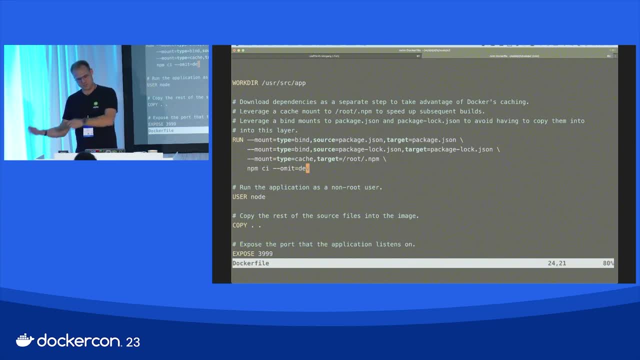 it's cheese. Okay, Let's put cheese back, like of the sandwich and now put all this stuff back together. Okay, And this happens when you type Docker build as well. If Docker recognizes there's a change in this cheese layer, it has to pull like it will change. 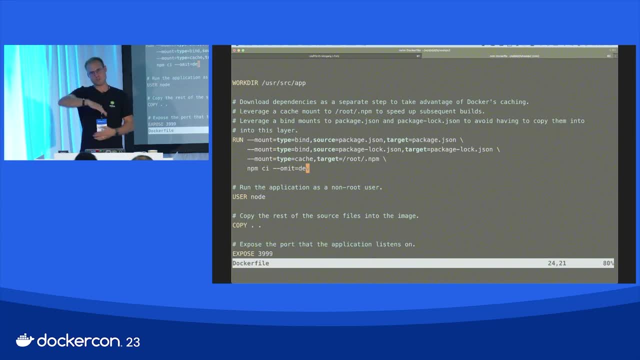 the cheese layer, but it has to pull back all the other stuff on top of it to make this final sandwich. It cannot say, okay, I'm changing just cheese and all the rest is untouched, I don't care. So this is important when you create your Docker. 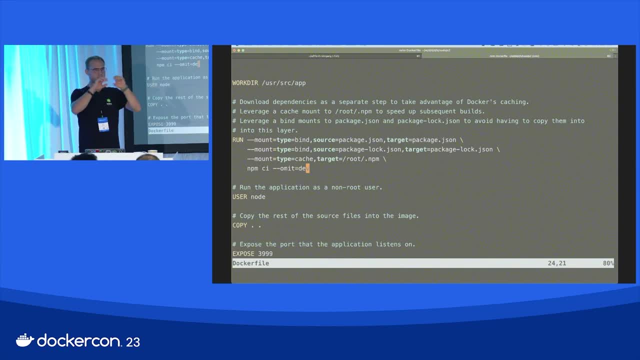 files. If you have a change in a layer and each command here like run, copy, expose, not, but copy and run is a separate layer in your Docker image. If you do run something, another run something, it will generate layer per layer, per layer per layer. That's. 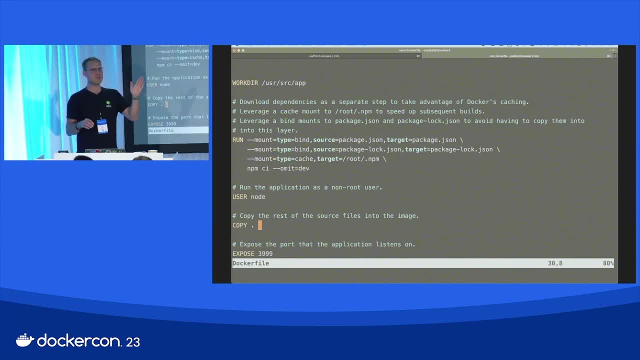 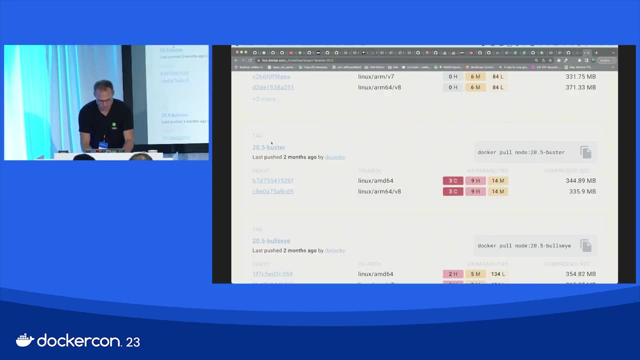 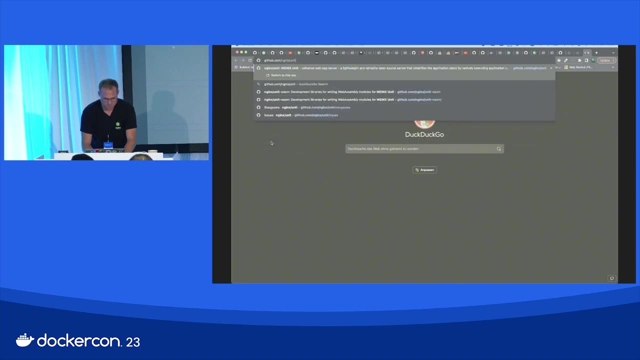 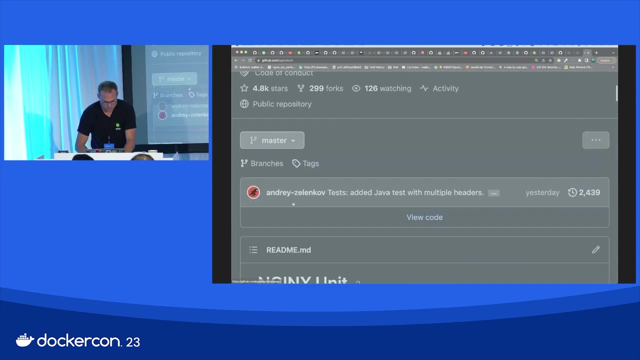 why you see in most of these Docker files, this little, this thing of run up update end, end up, install end end and have a list, like can show you how what I mean. Let me show you that in our- give you good example here- Packages occur. 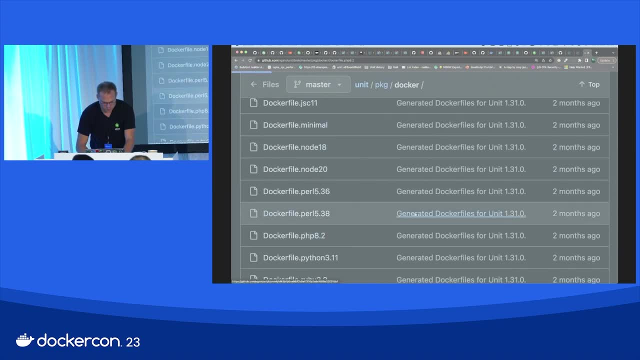 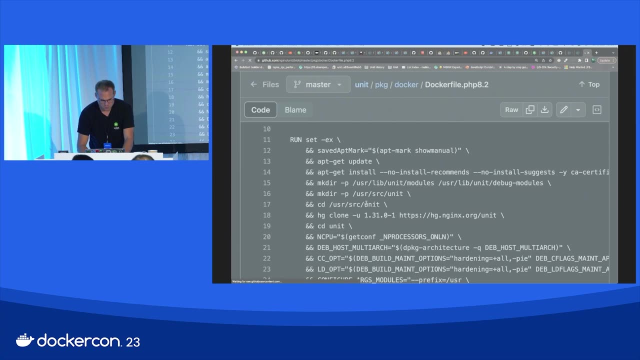 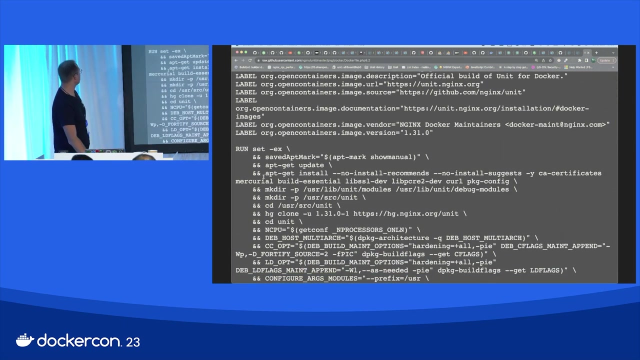 Let's see PHP 8.2.. This is what I mean. You say run, and then you chain all those things together Because now it's one layer. You can finally say: run HD, clone, run CD, run this, run this, run this. but every run command will generate. 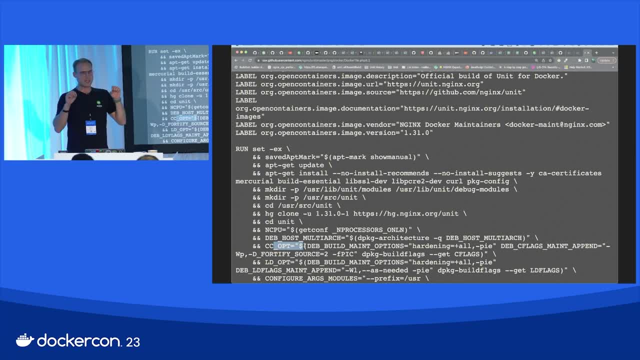 another layer in your Docker file and all layer, like every layer, comes with a little bit of operational overhead. Not much, but a little bit. And if you have like million layers in your image, this will add a million times this little operational overhead to your image. 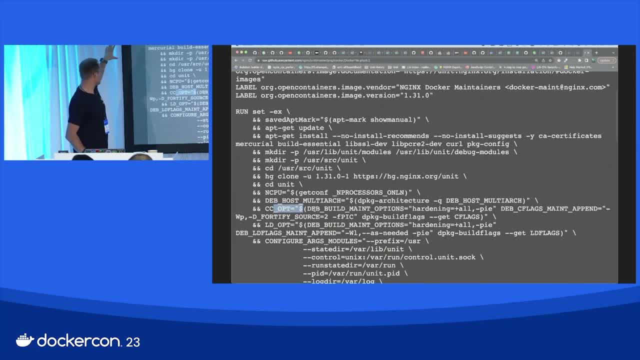 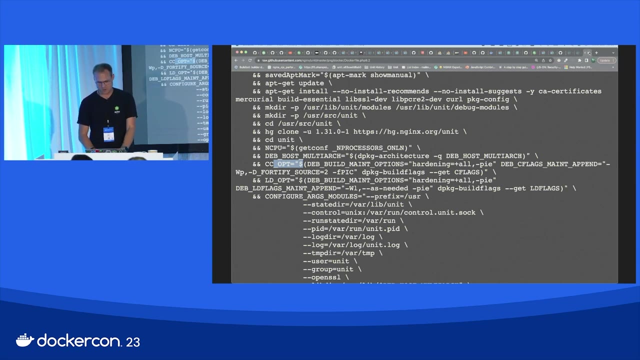 So this is this crazy, this crazy chain thing you will see in most of the Docker files from bigger vendors. This is the reason why they're doing it, because they want to generate a single layer that has all the components in it. All right, Right, So 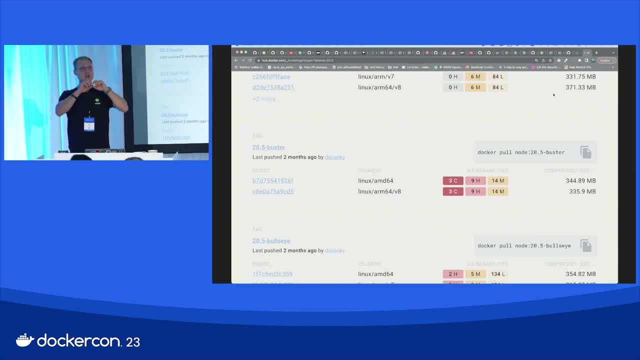 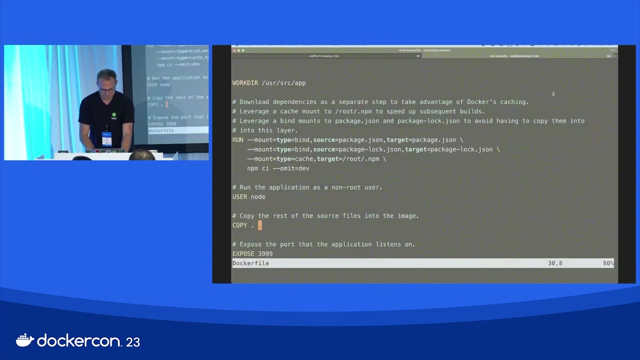 and the thing with this layered file system is that any time we change something in this, in this cheese steak, like cheese stack, we have to touch all the layers that come above the cheese stack Right. That's why the caching comes in handy, because it will. 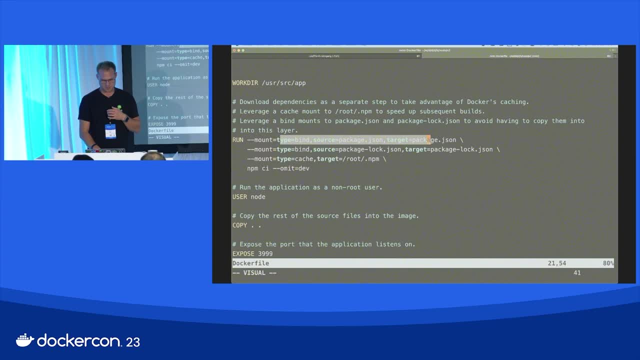 it will download basically the here, the again. so this is the: we mount things here, like for example the package JSON log, and then we have here in specific mount and we cache basically and everything that is that is here in in in the MPM thing. So that makes 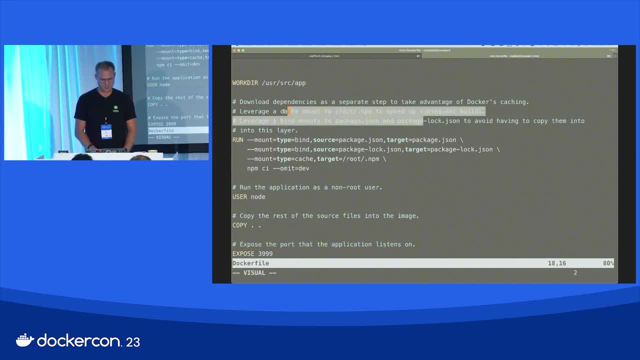 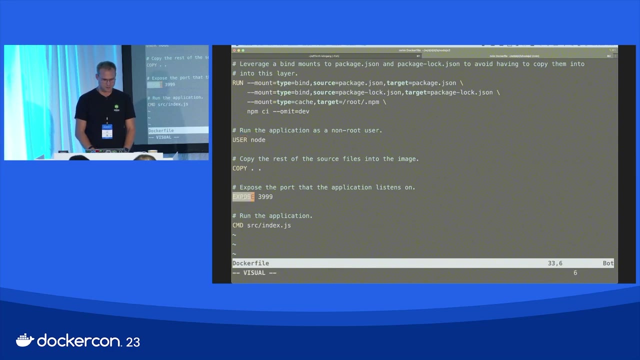 that makes use of the leverage, a cache mount to root NPM to like, yeah, to speed up subsequent, subsequent builds, that we can use what we have already created over multiple builds. that says a run user, and then we have here the expose thing, and here you see, we made a mistake. 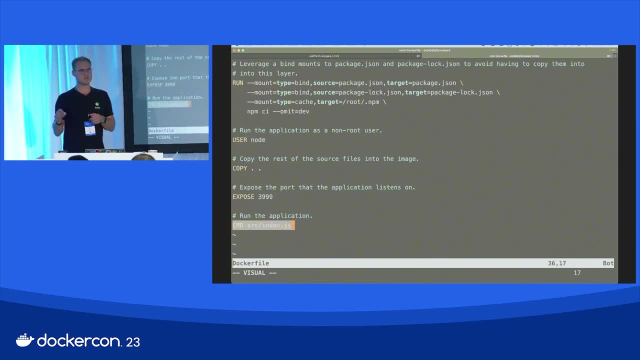 or I made a mistake. We type source indexjs, which is not right, because now it's the. the CMD line of our container will execute source dot source slash indexjs. we need node slash, like node space, source indexjs. I did that wrong at the time. 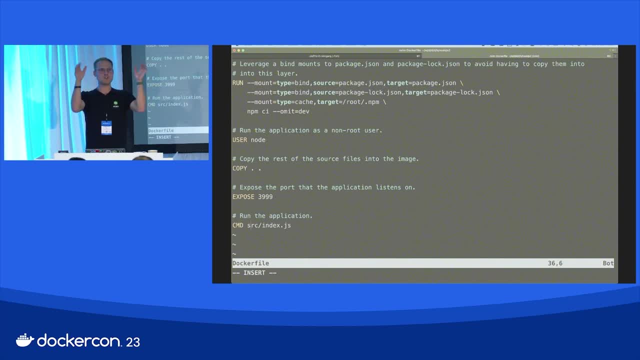 we did this docker init thing where docker asked me: hey, what is your startup thing? and it had node in, like node in, in, in brackets. and I don't know I- and this may be a good feedback- because I thought node in brackets means, hey, that is node, and now tie what node should do. 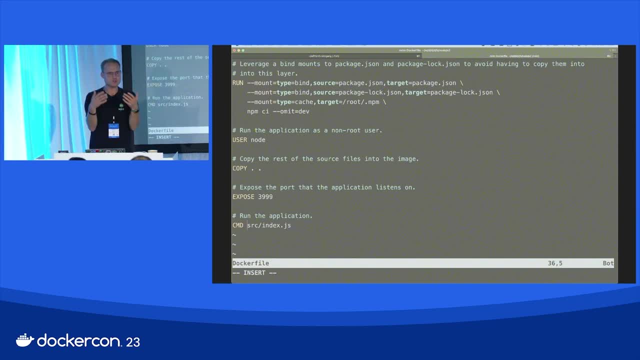 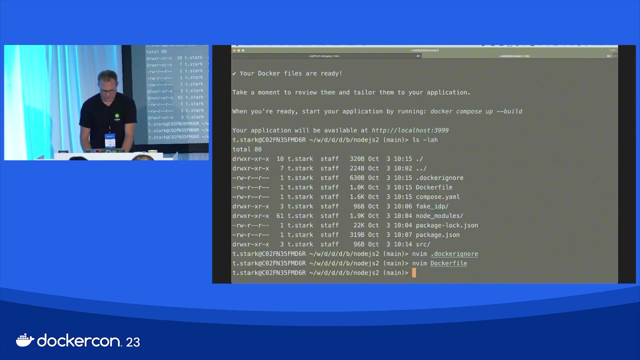 It's not, it's like a hint. should it just be node? So Let's do node. source index, dot js. All right, So now let's for development. we can get rid of this one. Okay, Now we do it. So now we have the docker file and 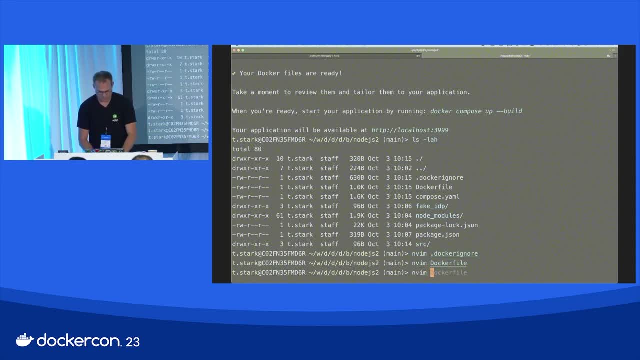 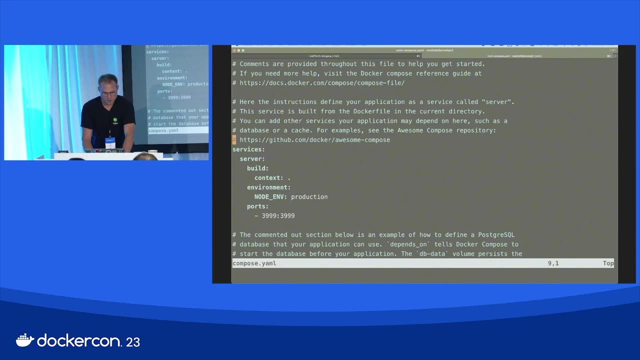 now let's have a look inside of. we have like five minutes to the next break, So that's something we can do. Let's look here. So we have a couple of comments, Um, And then we have services is the server and we 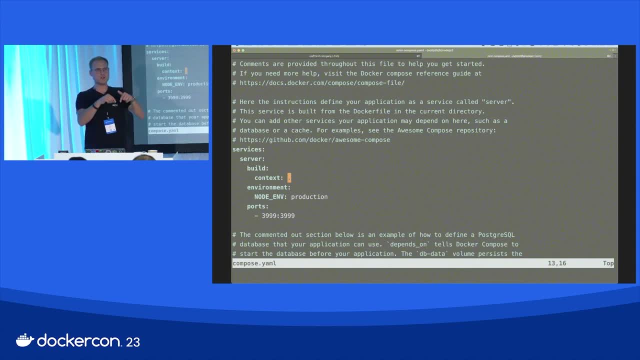 build context is dot, So that means we will look in the current directory for a docker file. basically, Um, We define environment variable that is set in the node end to production and then we, we export, expose port three, nine, nine, nine to three, nine, nine in the container. 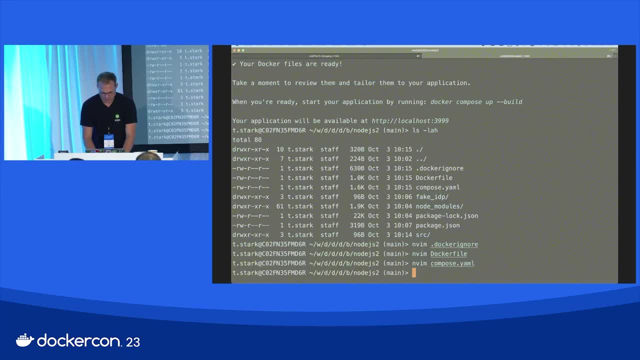 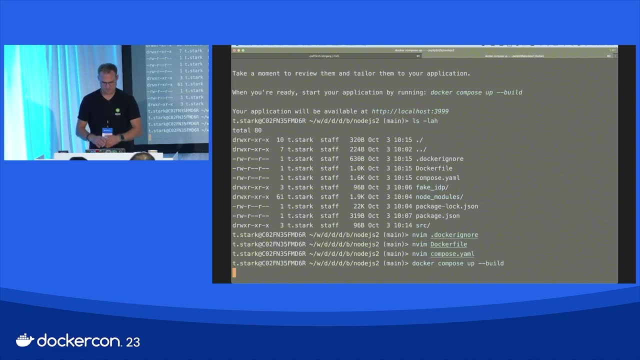 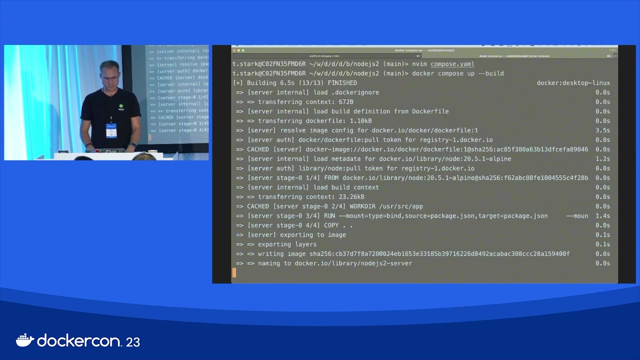 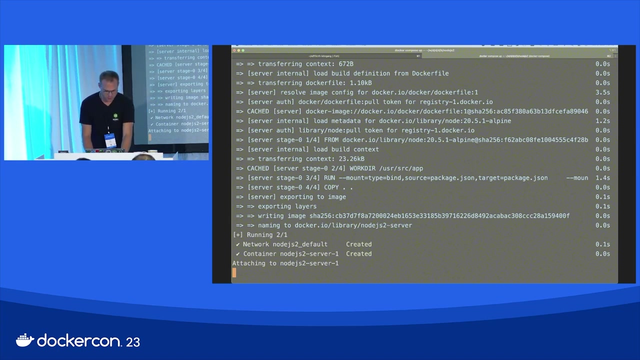 Okay, Good, And not touch this one. So now, when we do docker compose, compose up, build, That's basically what docker init is saying. It says at the end: run now, docker, compose up, dash, dash build to spin up the project. All right, So 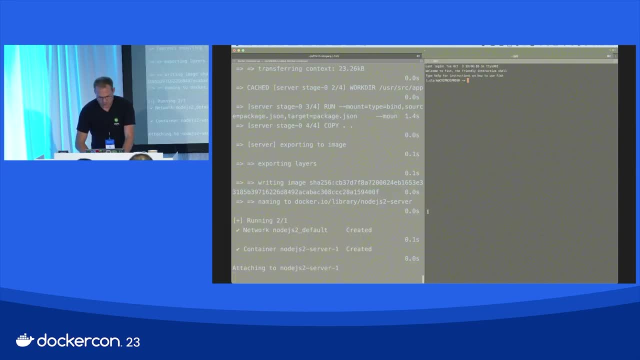 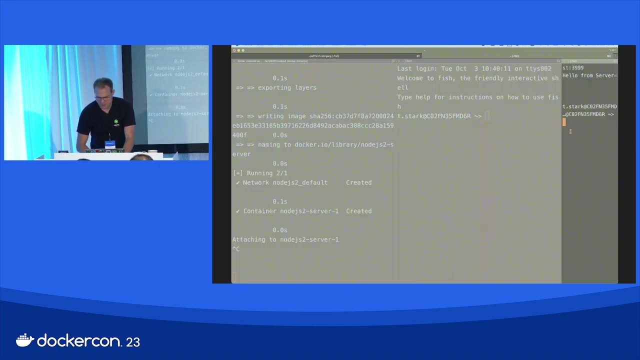 now it should work On three, nine, nine, nine- Let's see Curl local host. three, nine, nine, nine, Perfect Works, Okay. So what have we learned just before the break? Um, Creating, basically To get started with a node based API. 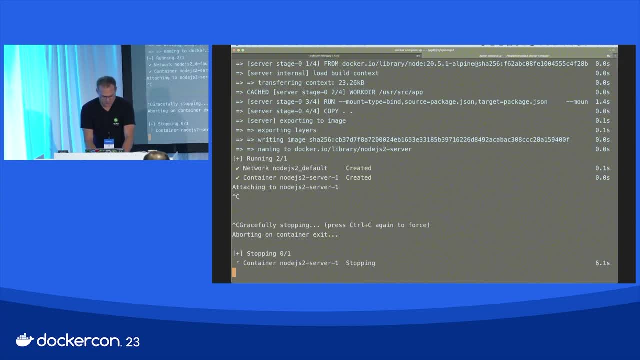 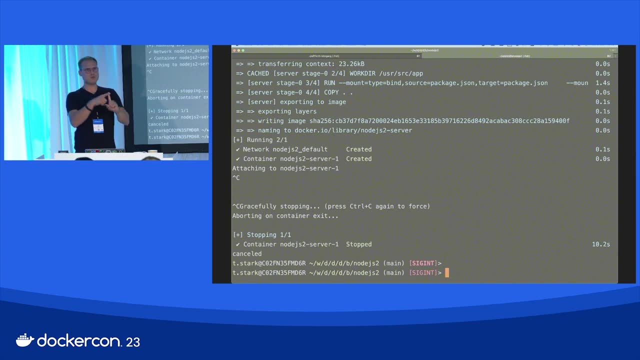 which we can then use in the project. in a little bit is: we do first npm init, Then we do all the stuff we want, And then at the end, if we want to dockerize the things, we type docker init, enter and then it will detect. 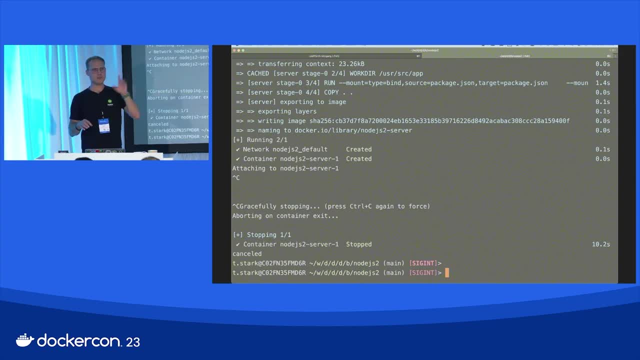 automatically: hey, that's a node project, amazing node. then we define the entry point. a couple of other things. we hit enter and the benefit we get is: it will generate a docker file that is following current best practices. It will generate a docker compose file that is following current best. 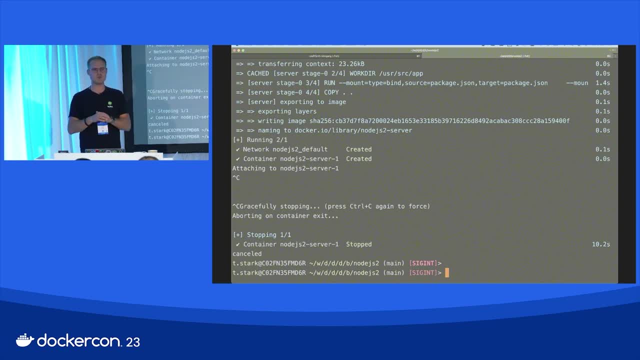 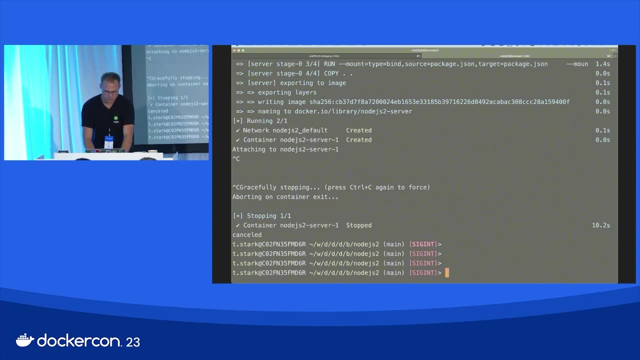 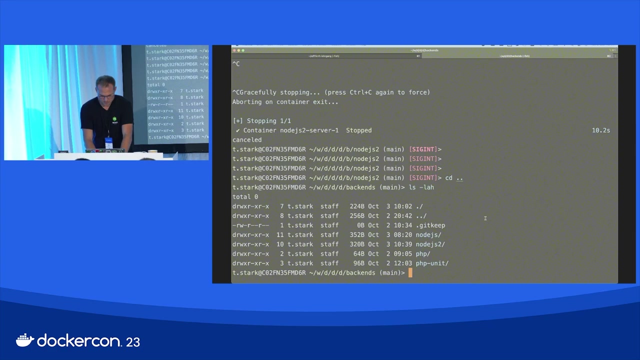 practices and it will generate a docker ignore file, not to put everything in the image. we probably don't want to. So this is the benefit of what we get when using um, when using docker: docker init, All right, Good. So next would be php. 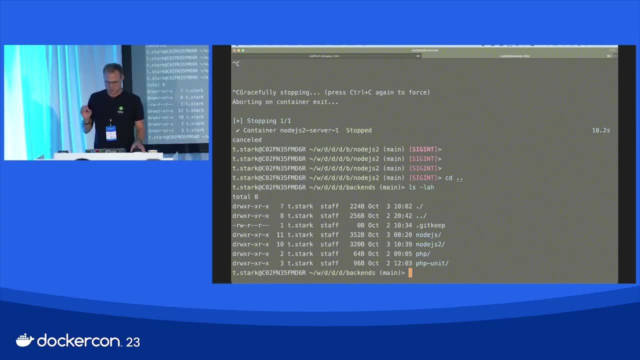 fpm and I would like to spend the next four minutes to show you the old way how I use php. Who's using php in production or still for development? So is it interesting if we do the php stuff? Yeah, Good. So I mean I'm using php. 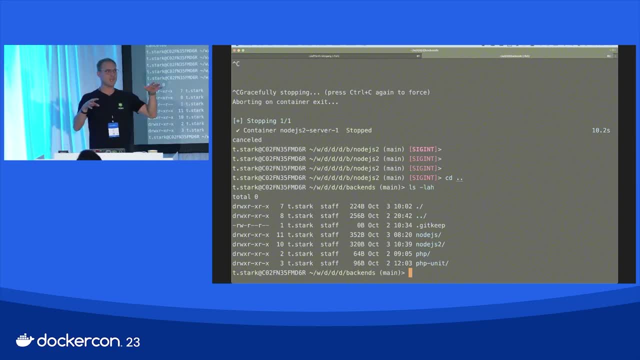 since I was 12 years old, so for a very long time, and I still love the language. by the way, It will not convince me not to use php anymore, because I love the language still. It's: yeah, sorry, I'm not smoking or not drinking, but I have. 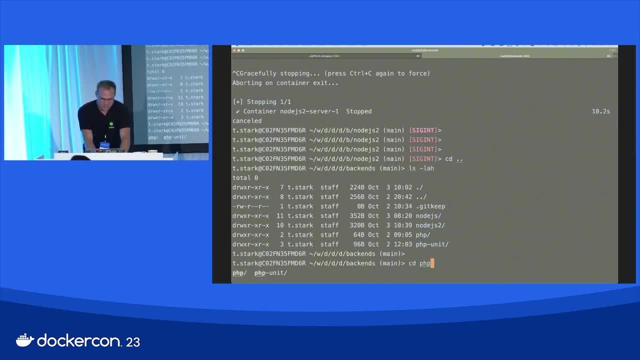 I love php, right, so good, Um in php. basically, what we cannot do is we cannot, like I mean, nginx cannot- read php code, Even if you, I mean, it's part of this nginx thing somehow, but we cannot see, we cannot interpret php code. We need an interpreter for this one, which is: 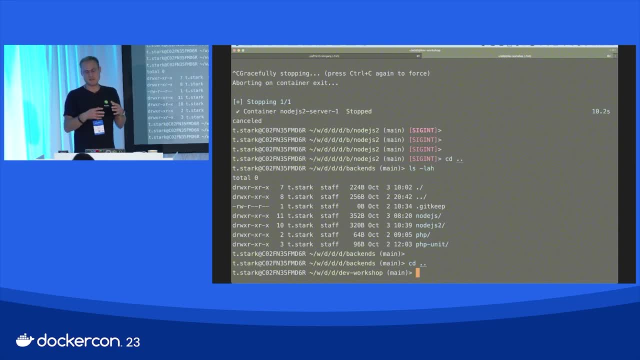 called fpm. The process manager for php, is one of this, and it implements the server api of php. So what we do is we request at nginx: hey, I would like to see the, the content or the, the execution of this php script. Nginx will take this script, sends it over. 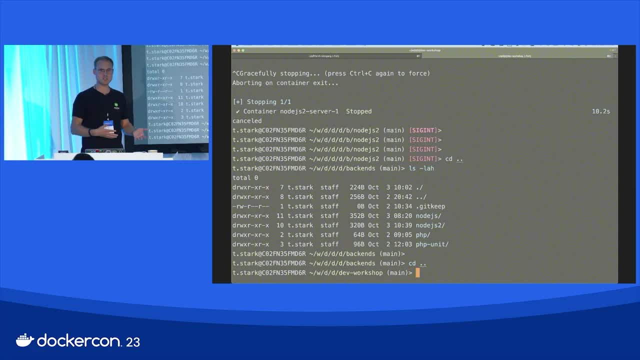 to the fpm. Fpm will do the php work, send back the response to nginx and we send it back to the client, Something that's called an fcgi proxy. That's what nginx is doing in a nutshell by reading php code. All right, so, and if you would like to, 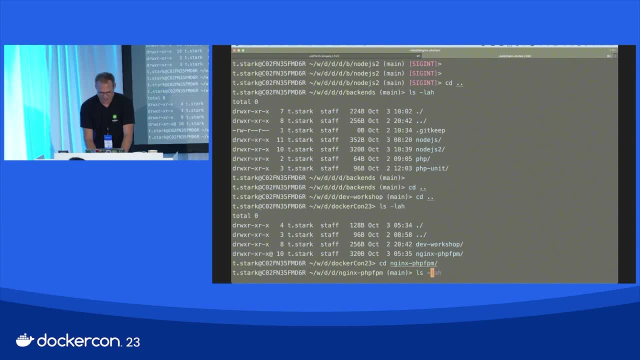 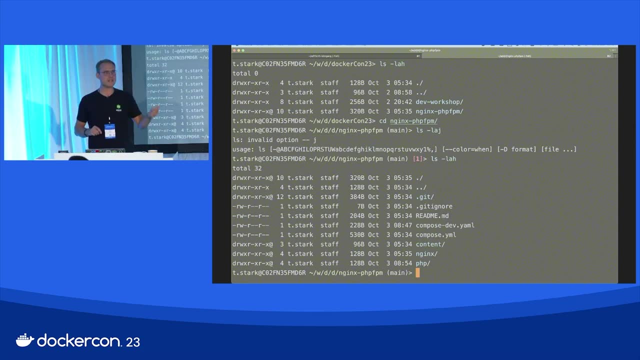 do php in docker. there are a lot, a lot, a lot tutorials out there how to do it. One is: you can put nginx and fpm in a single container, but then you will end up with this nice little problem of having multiple, multiple processes in a single container. 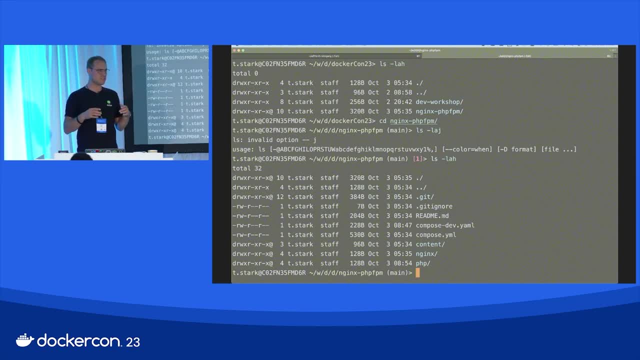 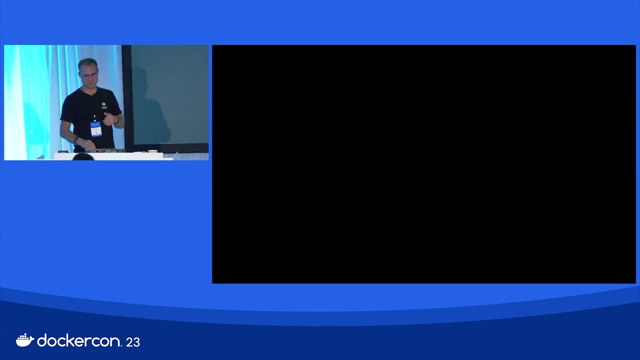 And if, if there's one thing that is against most of the standards from docker is that you have multi process containers, If you're not using something like supervisor or something that will be a single process that will be executed. Now it's blue, Okay, but I can. 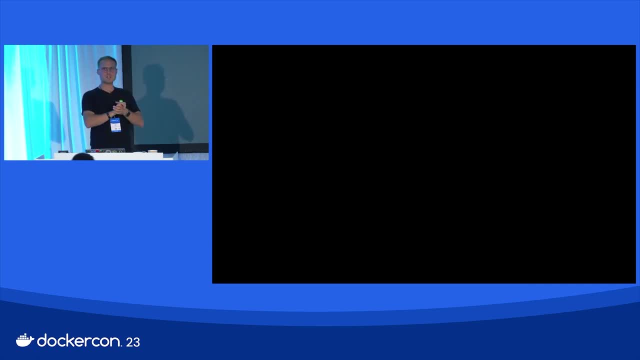 can talk about it. That's a single process that will be executed and then starts other processes. That's basically what supervisor is doing. Okay, another thing that you see a lot more often is you have two containers: One is nginx, the other one is. 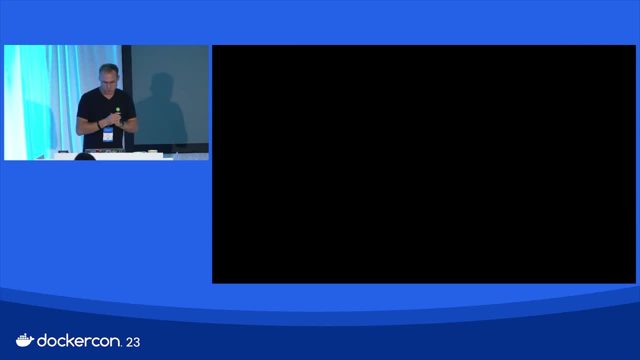 the fpm like the process manager from php. Problem with this is that your nginx must have access to your files, like html or index files, whatever- and the php fpm also need access to the php file. So you're ending up copying things into two different. 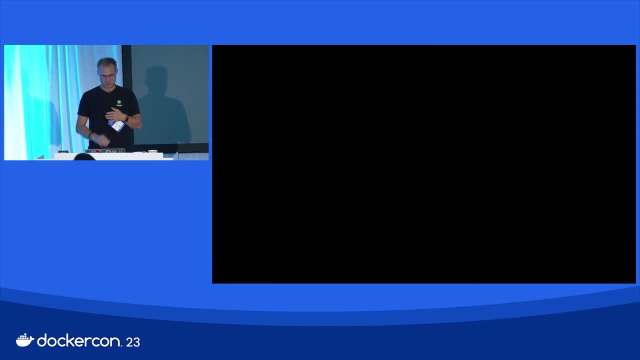 containers at the same time. So let me see if I can fix that by doing the same trick. as one minute left, Let me see. Nope, Nope, Now it's gone. Okay, Screen is already doing a break, Okay, So after. 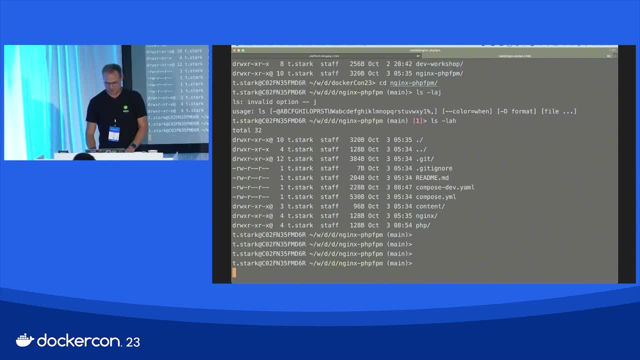 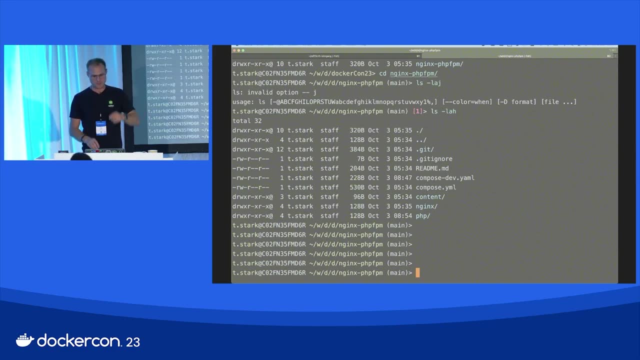 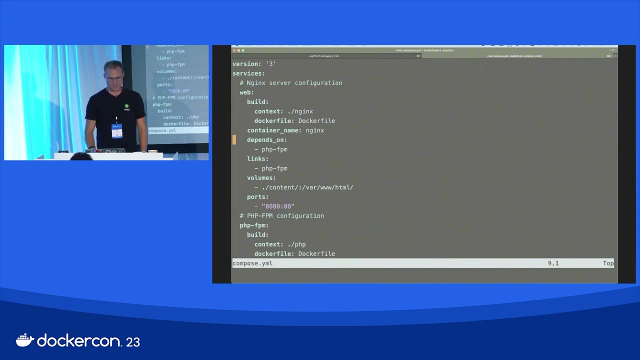 the break. I will. No, it's back After the break. we will look into this setup and we already did that, basically because that was the pull we did earlier by using the this docker compose file with the like: this is nginx, which depends on fpm. 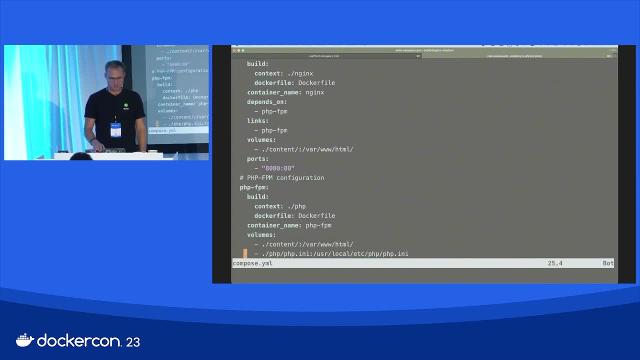 and then we have the fpm container. Does this sound familiar to most of you working with php? this like two tier setup thing, and I have used it for a long time since I have discovered nginx unit, and this is what I will show you after the break: how to use nginx. 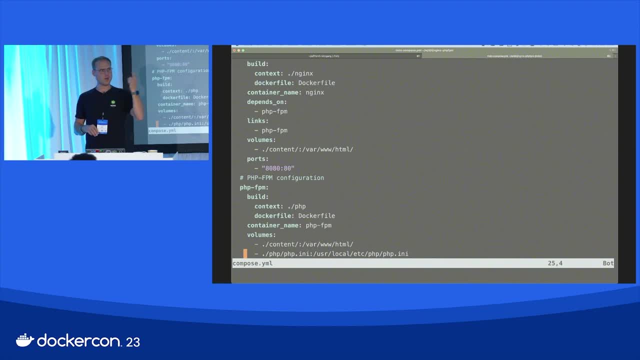 unit, because with nginx unit we need just one container that can run seven different languages in a single server binary and is a web server in a single thing. so we can. we don't need fpm anymore at all. so it's just one thing, and this is something I would like to show. 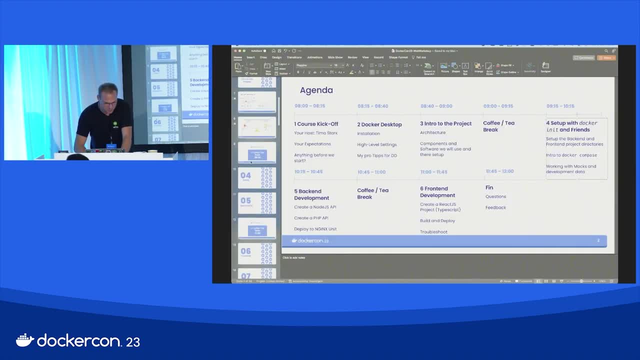 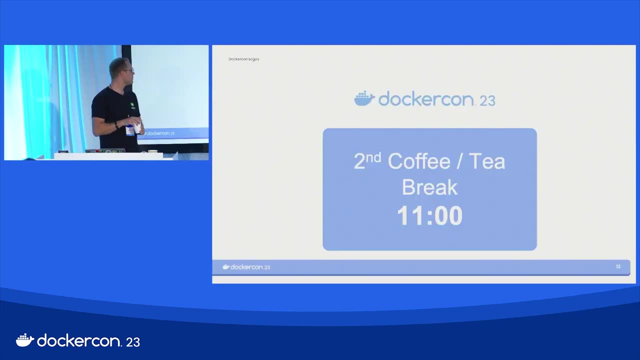 you after the break? Perfect. So see you, and I have a slide for this, actually for the break. Nope, There you go. So yeah, 15 minutes, That's what I'm saying. I have not much slides, But I have at least. 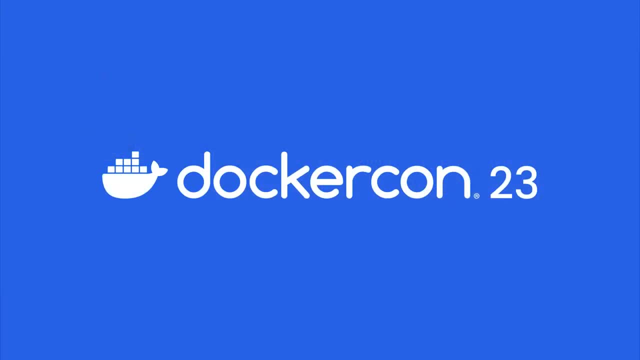 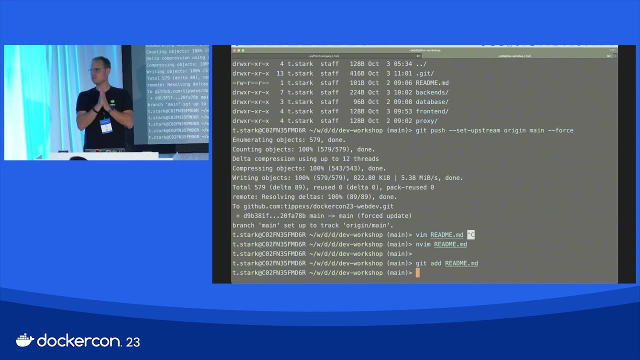 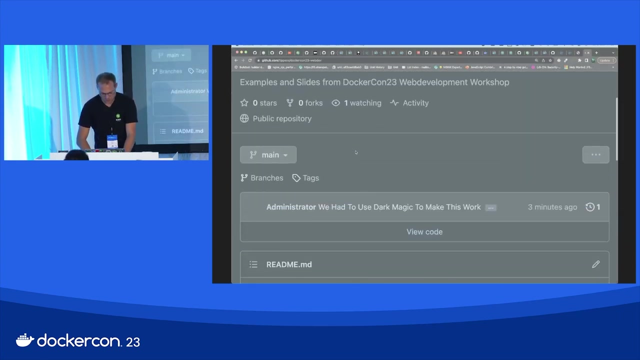 the break slides. All right, So it's 11, the last hour, And actually nice that you're still with me, so it's not too boring. then That's good, All right. I have created a github repository so I can dump all. 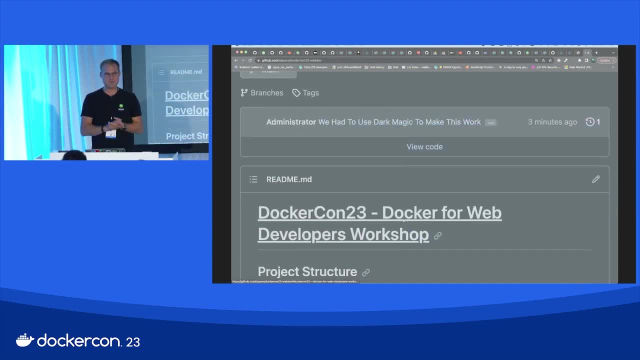 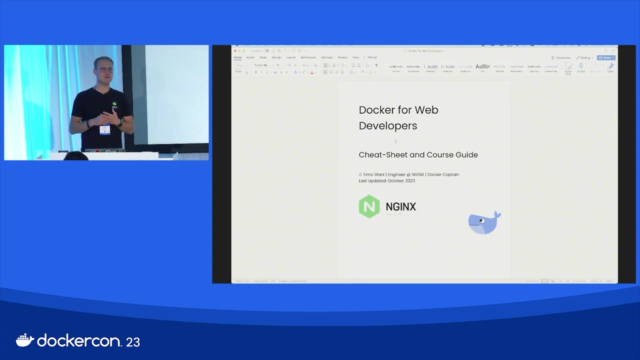 the examples and pdf this little word document I was working on Here, So, yeah, I will finish this one, maybe on my way back home in like 12 hours flight. That's perfectly for doing writing like this, So expected this pdf to be in this github repository. 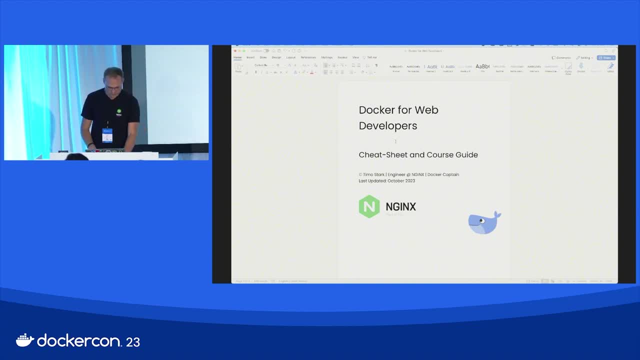 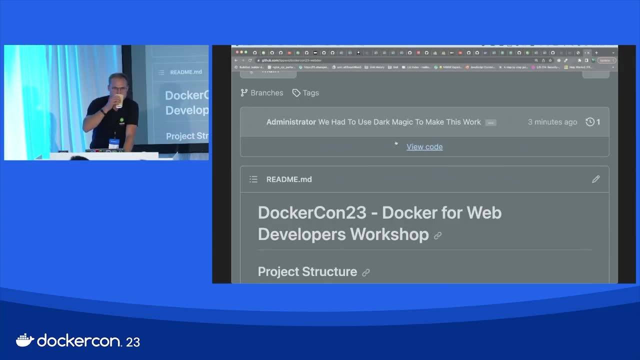 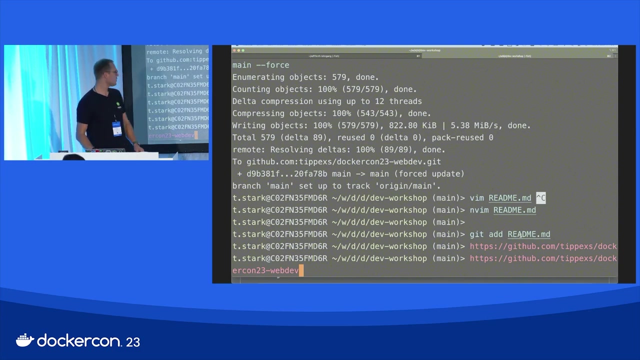 somewhere the next week, Okay, And I will make sure it's including all the examples and stuff. All right, Amazing, Hmm, Good, Let me make this bigger so you can actually see that. So it's again in my repository And then. 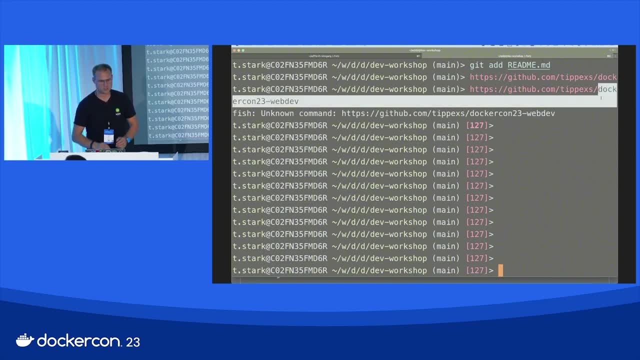 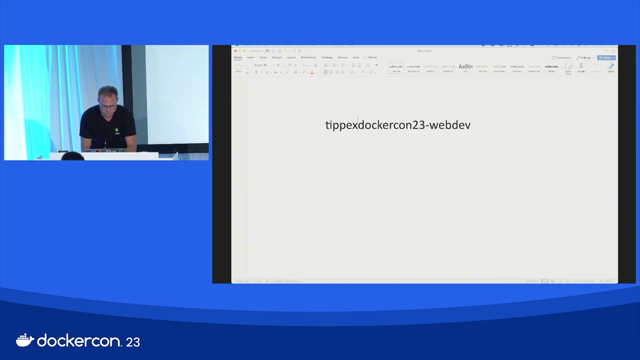 it's dockercon23-webdev. Okay, I can put that maybe in here as well. Let's see, Yep, Yep. So I will keep this thing up at the end, So Good. So, As promised, let's jump in the PHP. 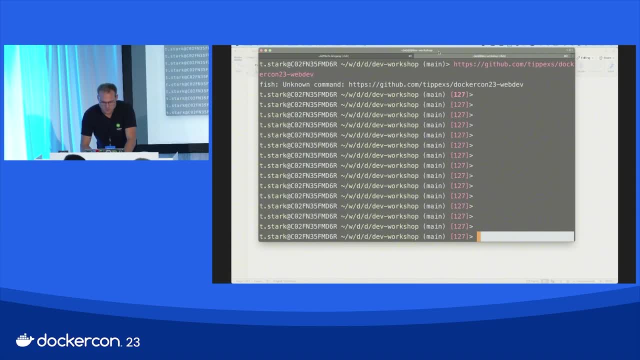 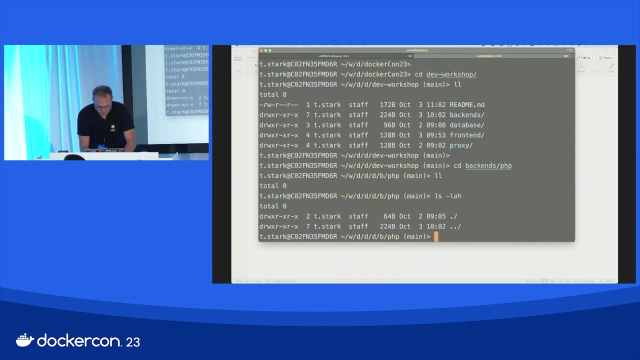 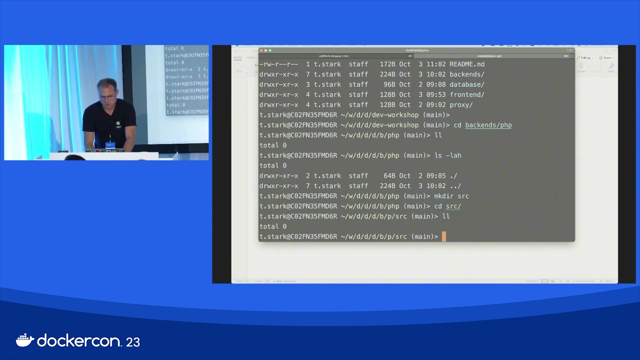 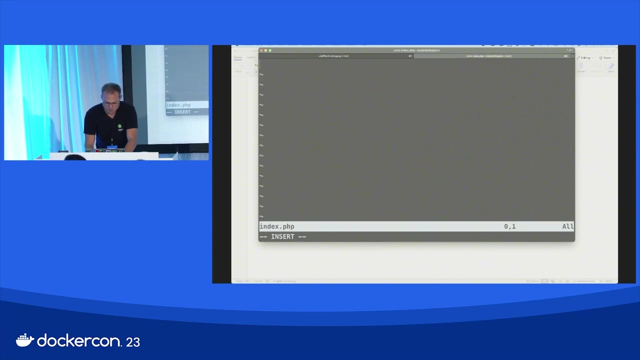 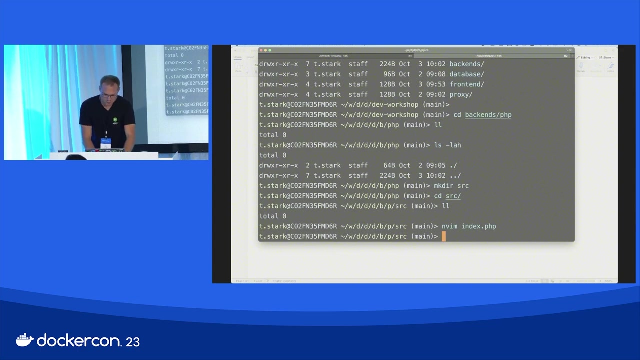 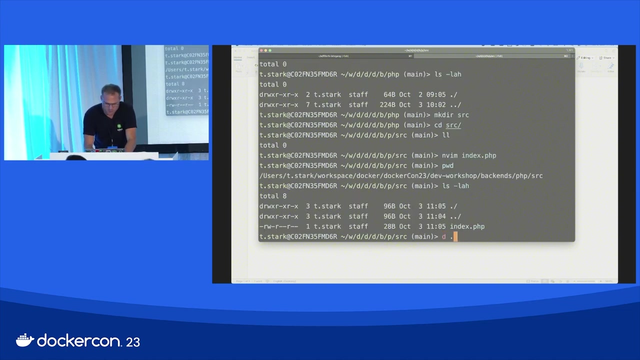 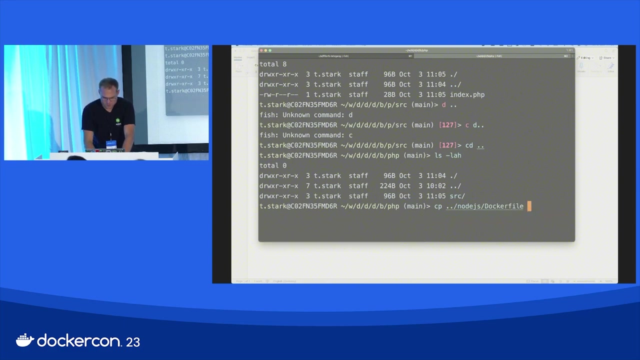 world then Good. So in backends Let's copy the docker file. 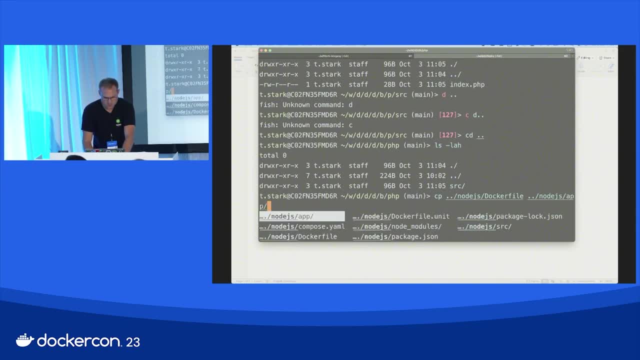 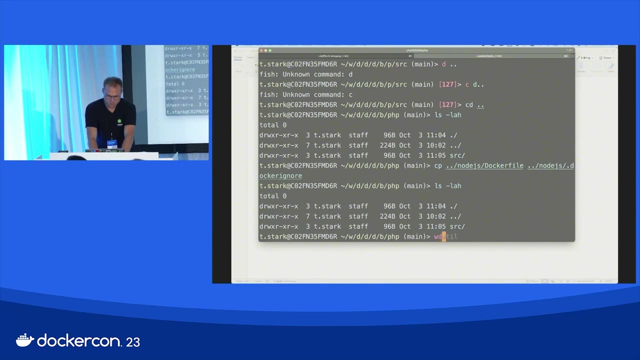 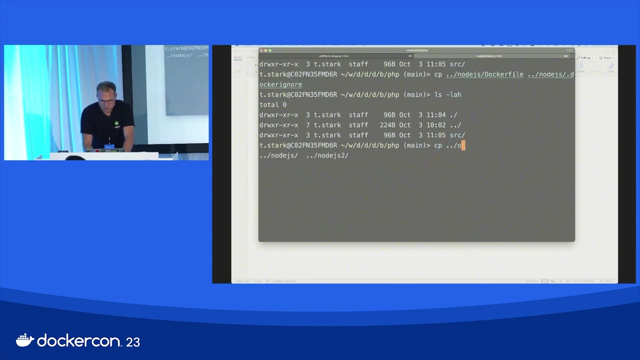 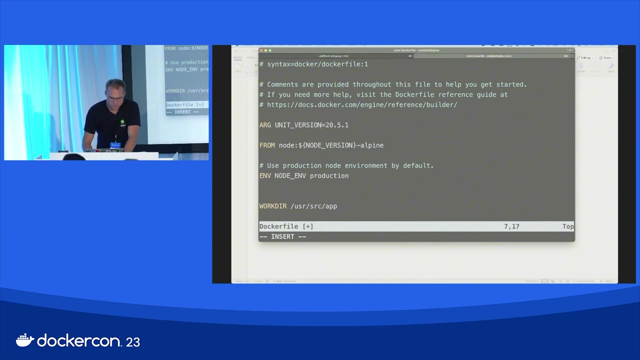 And let's copy the docker ignore thing for the moment. Where's docker ignore thing? Good, Oh, node, js-docker-file. Let's do 1x1.. Good, Good, We keep this. We rename this to unit. 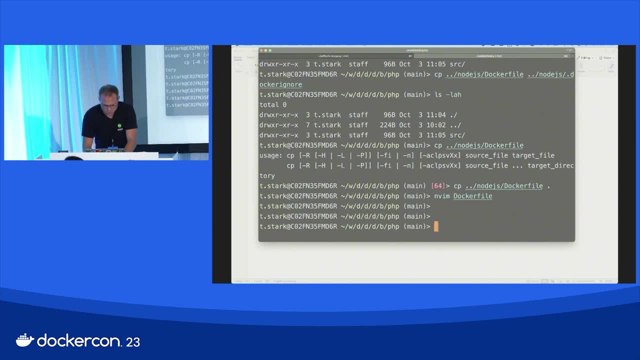 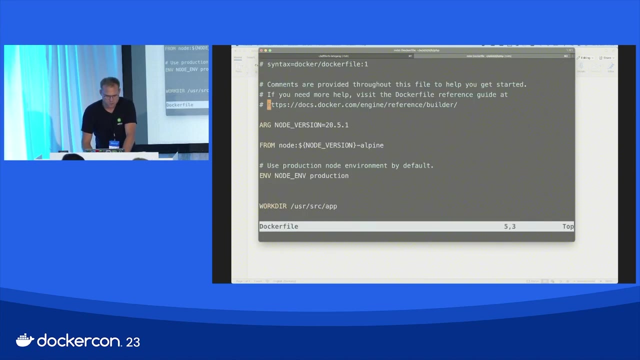 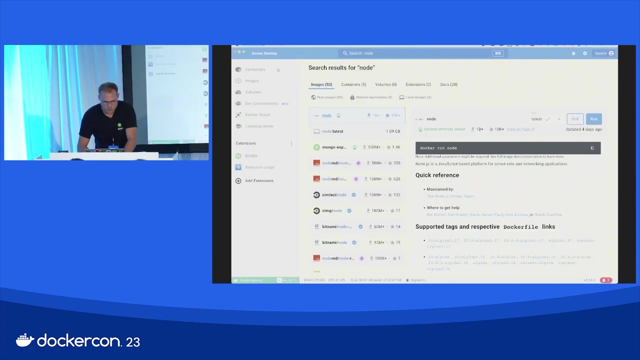 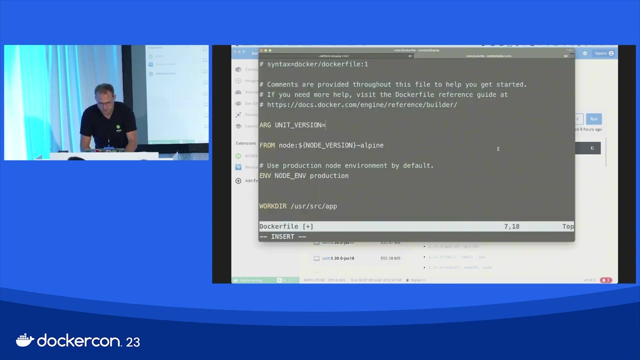 Oh, actually, Uh-huh, Nope. Okay, Good, So we renamed this to PHP or unit. So now we would like to know what is the unit version? Right, So we use unit. Then there is 1310, PHP 8.2.. Okay, Fine. 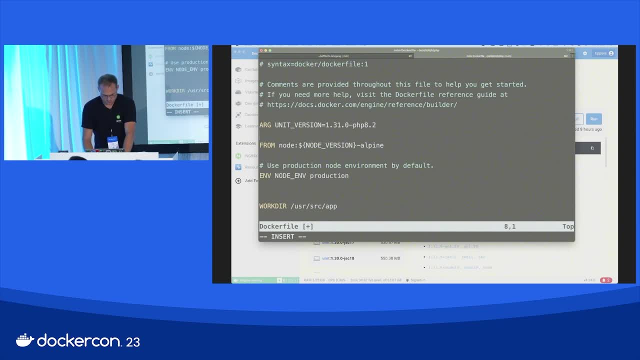 Okay, Put that in Good. Then we delete this. And then we say this is unit. We don't have this. We can keep the work here, No worries, As this is very simple. we don't have caching right now. Delete this, Do this. So then we copy everything We expose. 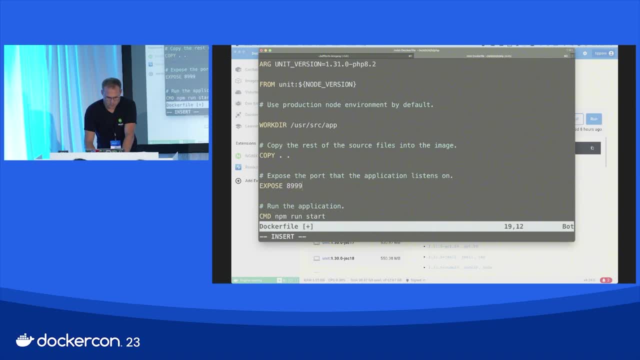 8999. Should be fine. And here now we would like to start the unit application server to serve PHP without this FPM stuff. Good, And this is another thing. If you have something like this, a base image, you can, you don't have to put. 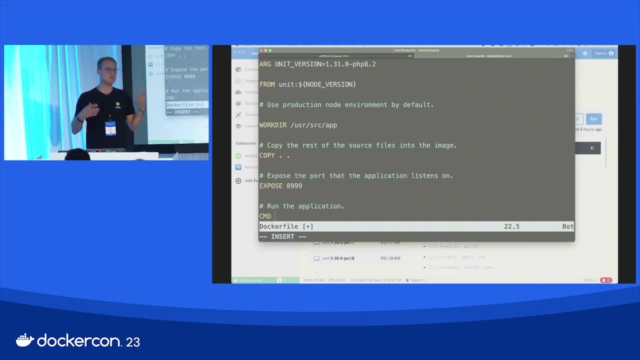 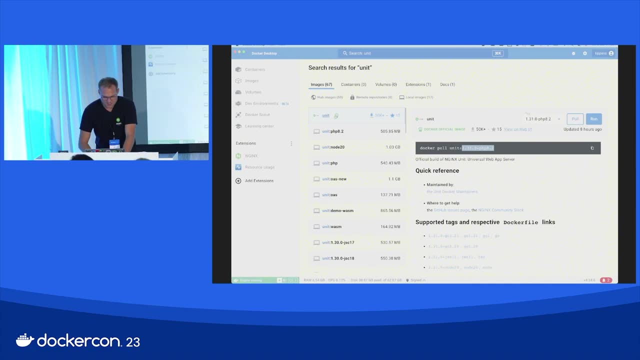 the CMD line in it, because your base image already comes with a CMD line, maybe. So therefore, it's sometimes pretty handy to go to the GitHub repository because you click on this. Yeah, It's not, it's not showing here, It's not showing you the different layers, So 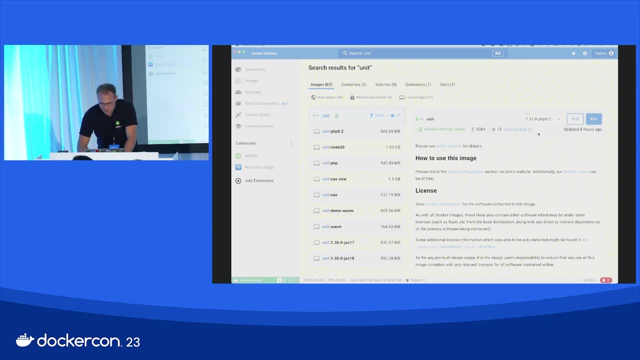 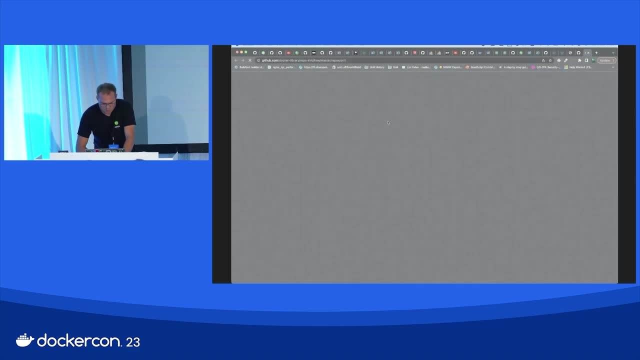 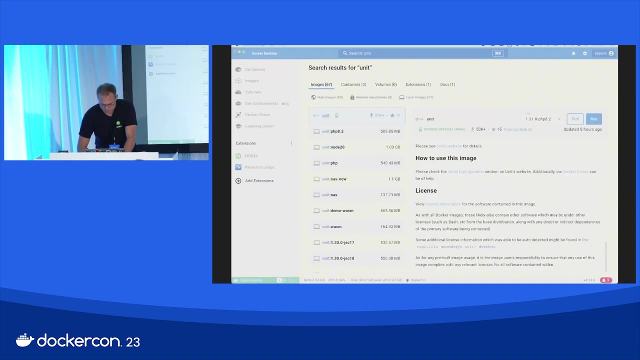 you basically do, then I can show you this here. You can go on hub or there's sometimes repository And this is the info. Okay, So now we're going to show you how to do this. So we're going to show you how to. 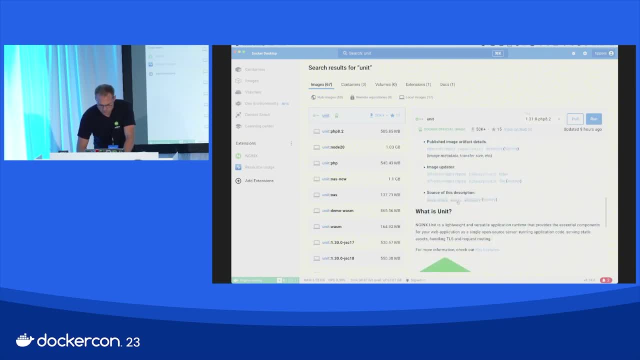 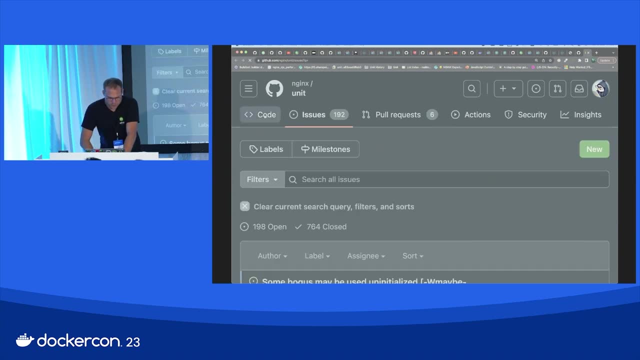 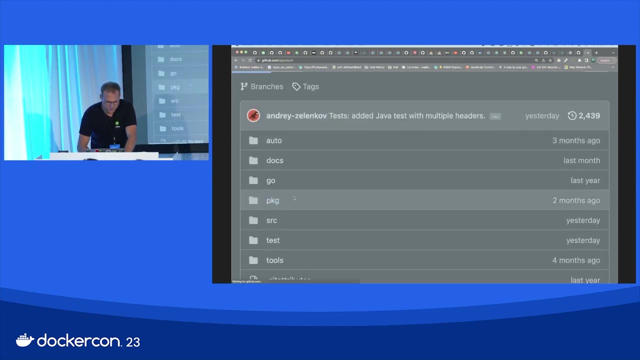 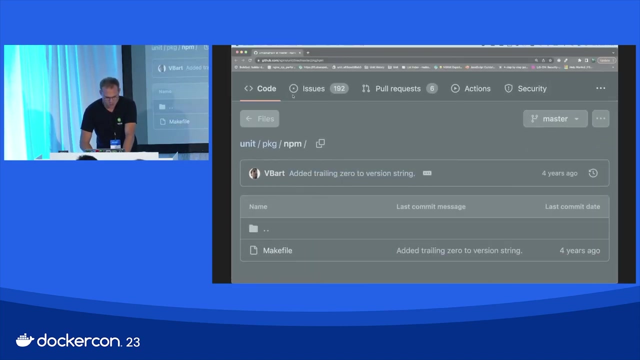 do this. Okay, Where is the link? So we click here And then in code, we do packaging And don't be afraid of doing it, It's, it's, it's, like most of the time, pretty, pretty straightforward. 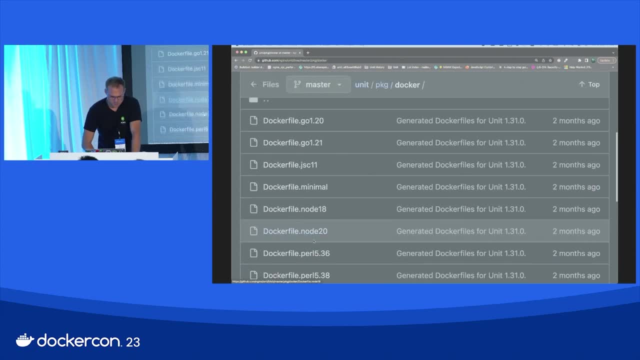 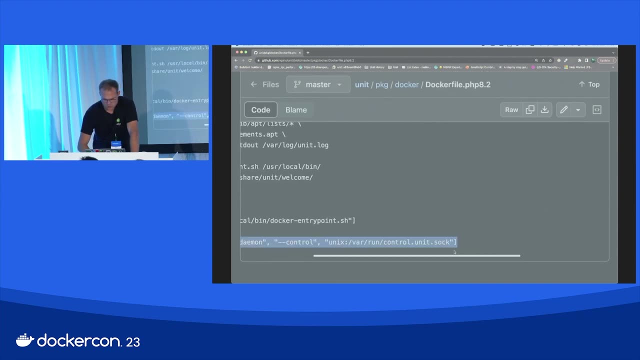 Docker. So we click here And then like PHP 8.2, then scroll on the very bottom And here it says: okay, This is the CMD line. If you want to use it like this, just don't do anything. 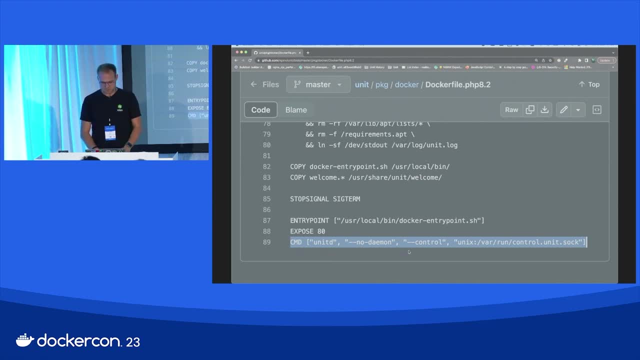 You don't even have to specify a CMD line, But in our case, what I would like to do. unit is an application server from NGINX and normally it's control API, because you can reconfigure it, and that's different to NGINX. 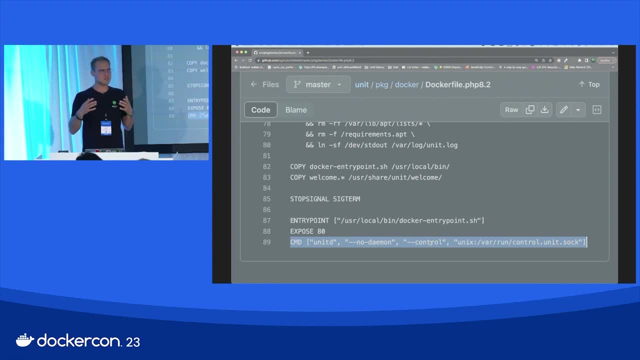 next, you can configure it with an API So you can send JSON payloads to the server to change what it's doing without reloading anything manually. And in this case I don't want to have the control API listen on a socket, but I want to listen to it on IP and port. 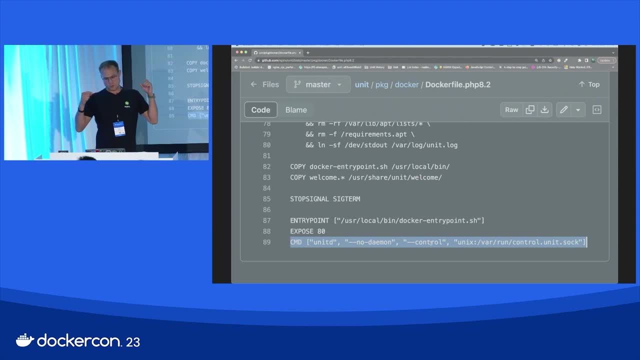 The reason why we have it per default to a socket is because of security. We do not have any authentication at the moment built in this control API. That's why we keep it with a socket, because it's then very unlikely that, even if you just run it on your production. 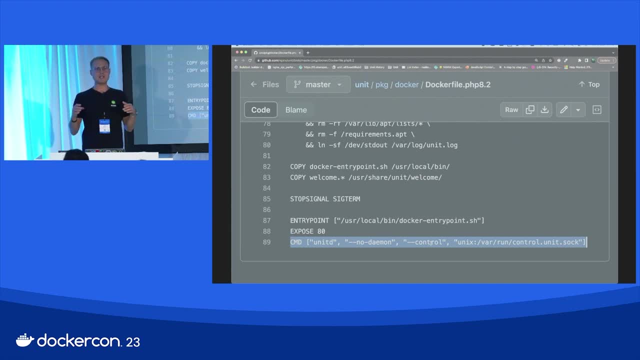 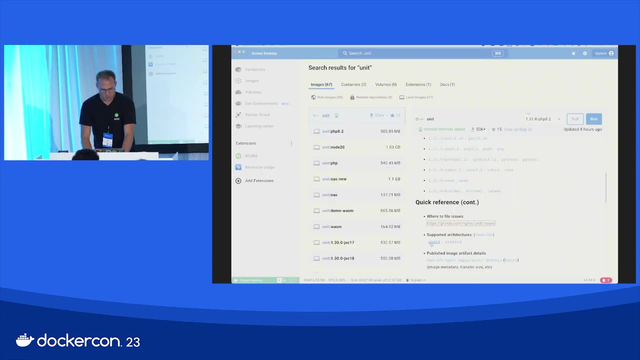 server and not looking into what actually it's doing, it's very unlikely that you expose and port to the internet, So that's why it's a socket. But I don't want to be that. this is a socket. So what we do is we copy this whole CMD line. 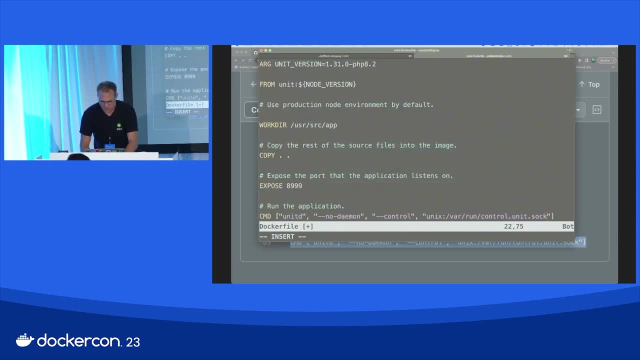 And then we just copy that in here. So in here we now say: no, daemon is fine, And then we do: okay, that is 120.. Now let's do 9000.. Good, And now I show you a neat trick. We can do this expose thing Fine, And we copy everything we. 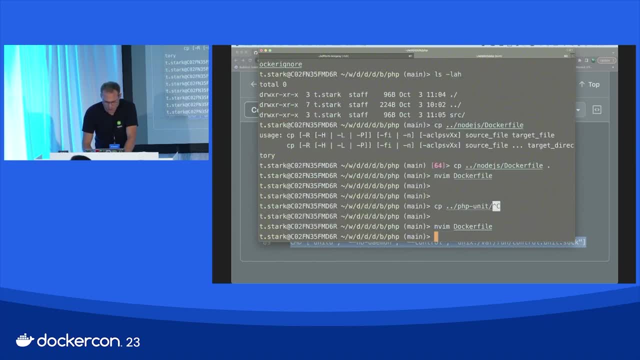 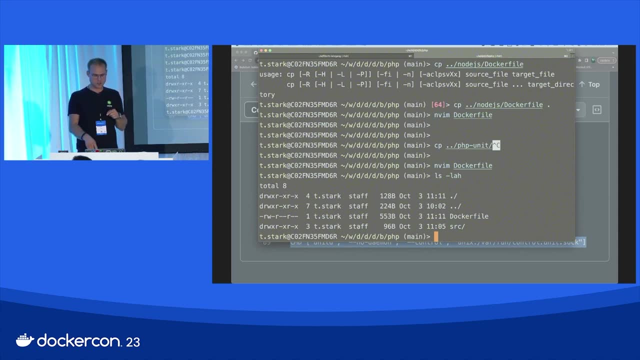 have in user source app Also fine, And I will not use the feature we have in Docker. in unit for Docker You can copy a configuration JSON to the Docker entry point D and it will configure the application server automatically without doing anything manually. But this wouldn't show you how the API works. That's why 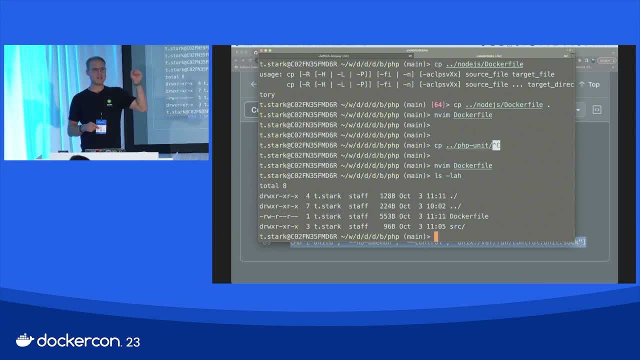 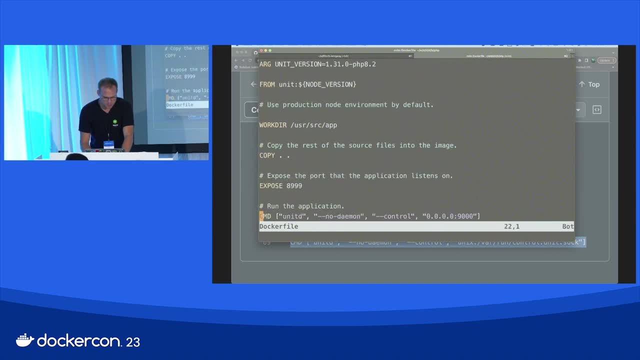 a writer. Did we not copy that? All right, Jim at Docker energized the thighs. Take a look, Hey Jim, right here, You all right here. Yeah, I'm hi there. Okay, Another slide. that came in the суп of R too. now independent of split. 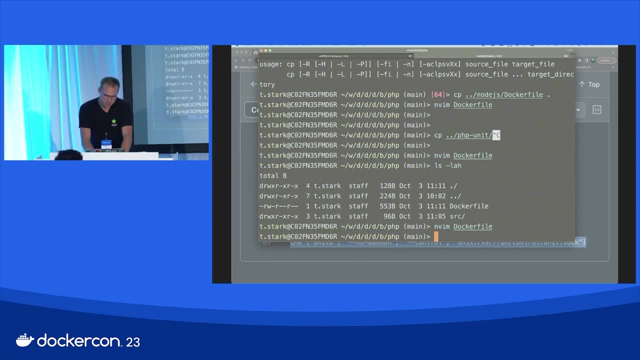 That's my laptop application: square People who don't know where to0. What are we doing here? We are using the Docker file. We now have one line that says we expose port 8999.. That's fine. One line that says we expose port 8999.. 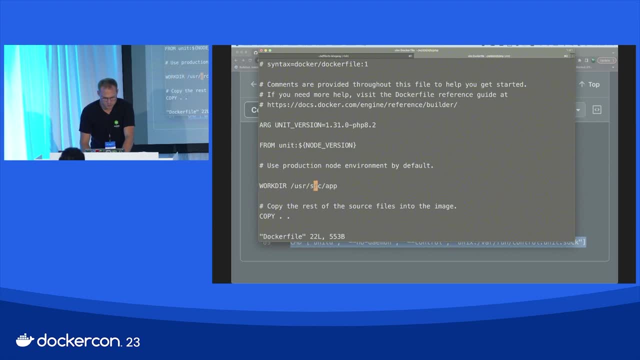 Perfect, user source app. Okay, that is stupid, So we do, I don't like that. actually, User share unit, That's much better. Sorry, Oh, you're right, Thank you. Okay, That would fail. Perfect. Thank you very much. 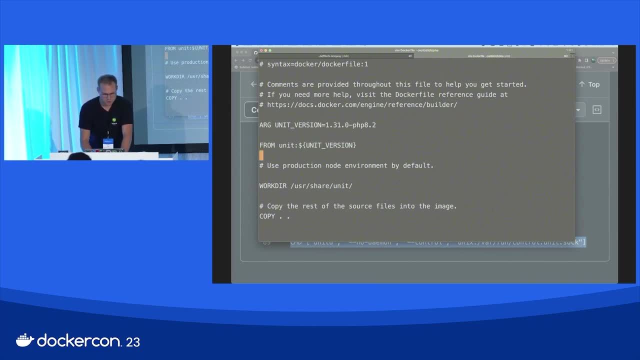 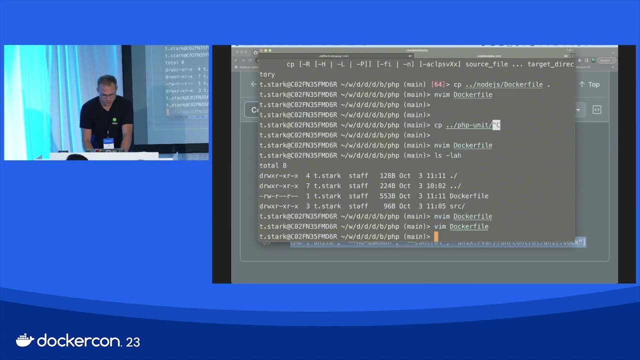 Okay, So good catch, It is unit version. Thank you very much. So we have unit unit version. We have user share unit. That works. So now, when we do docker build, dash t is tagging, so you can. 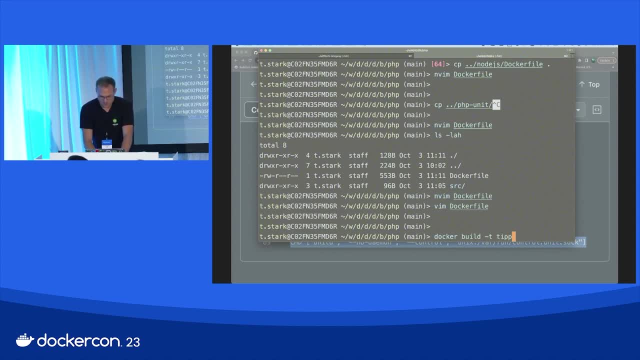 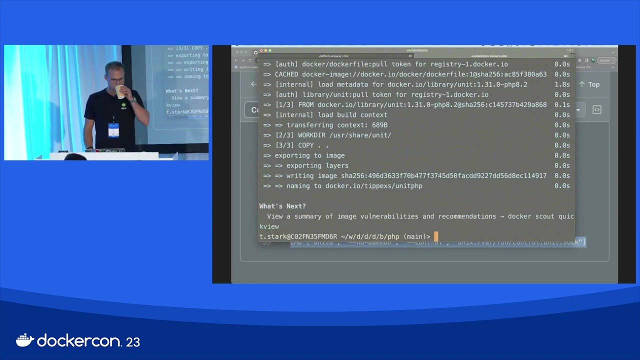 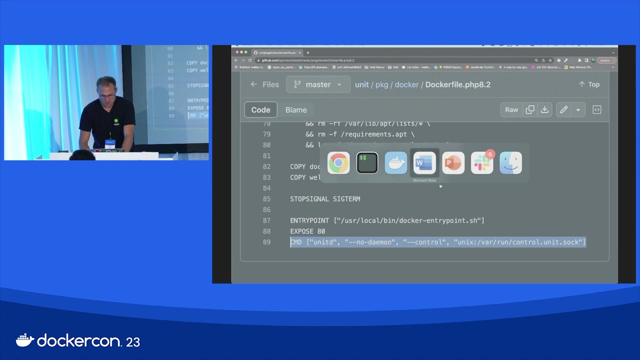 define whatever you want to do, So we name it: tivx, slash unit, unit Jesus unit, php dot. So now it's So, it's here. So when we do docker images, that looks also awful, So now we do this. 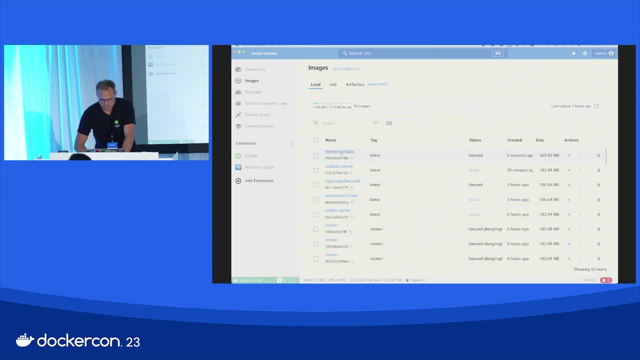 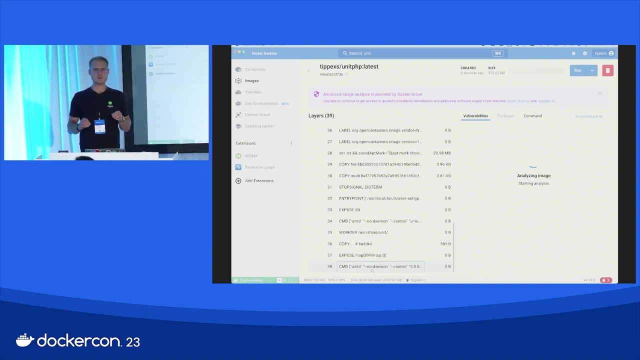 and go in images. So it says it's unused, It's this size And basically when you look in here in the image you can actually see the CMD line. That's why I'm saying docker desktop is most of the time. 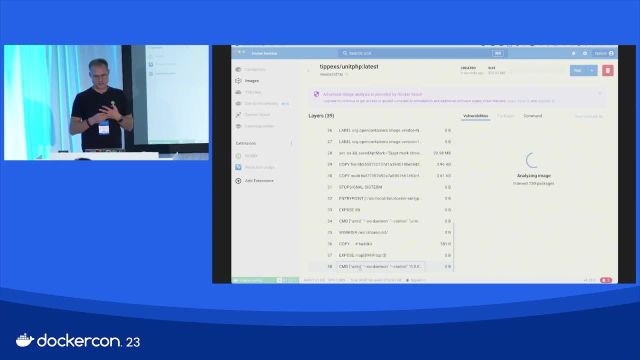 so much more efficient than doing it manually, because it will tell you automatically: hey, that's a CMD line. And while we are here, I will just tell you something about this vulnerability scanning thing, which is also very important because this is something new to docker desktop. 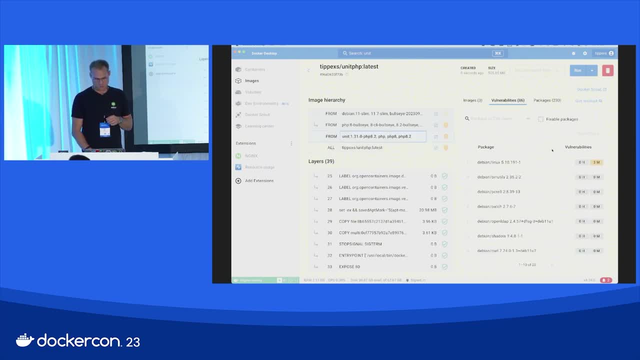 We can see what vulnerabilities come with what like image or layer in our image, So you can do this as an engineer. You can see, okay, what are the vulnerabilities And you can see, okay, what are the vulnerabilities in this application. Vulnerabilities in a whole, like not just in the image, but if you have known CVEs in the code as well, like in the library, that will be detected as well. Docker desktop will not find vulnerabilities you write in your code. If you have SQL injection. 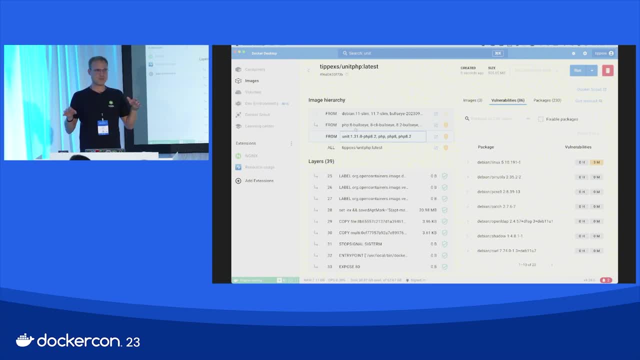 something, or in cross-site scripting thing we like. docker desktop cannot find this one, But it will find common vulnerabilities in packages. So in this case we will see that our image tibx-unit-php-latest is based on unit-131-php-8-2.. 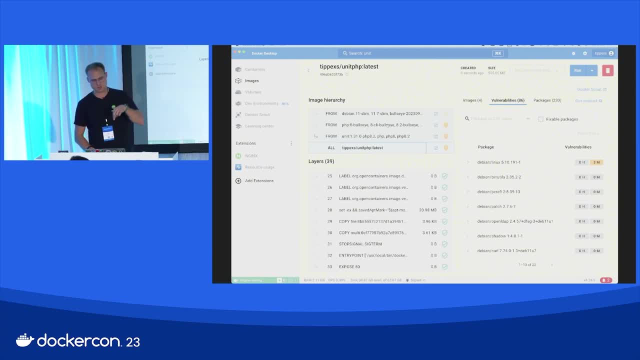 This is based on php-8-bullseye and this is based on Debian 11 slim And this is one of the most interesting things I like on docker desktop: This is the first time I can see the chain of what base images were used, even on the vendor side, I mean. 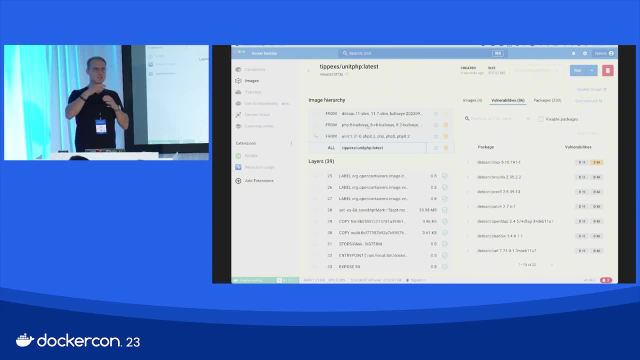 we are your vendor, we are NGINX and we say: we define, we give your image, but that means we use the official PHP image And the official PHP image used the official Debian images So you can easily spot if there is. 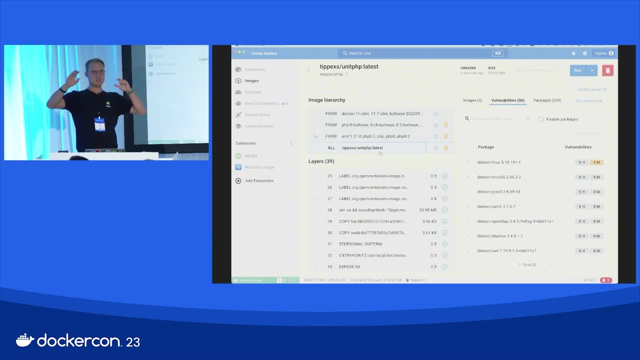 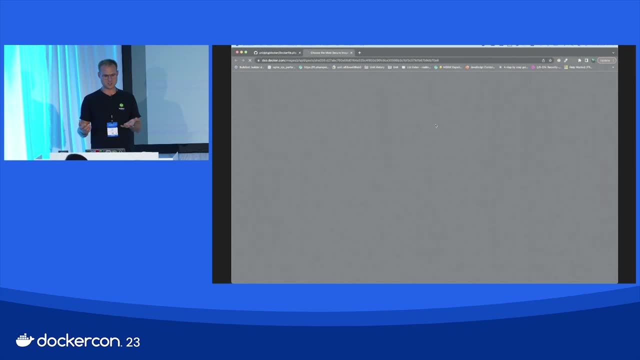 some clunky, weird base image in your stack saying, okay, what is this? Then you can click on it and you can easily find out what is this base image like. what the heck is this thing doing, right? So that's why I'm saying this: 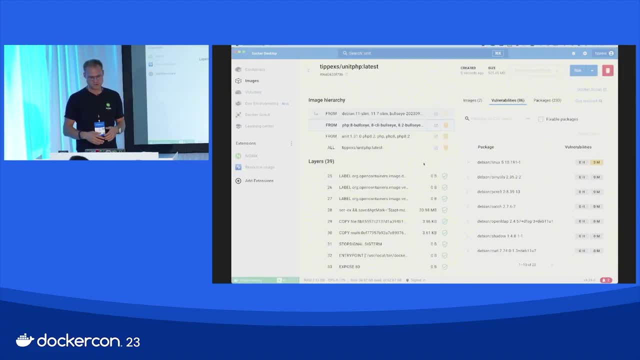 This whole docker desktop thing makes it just super easy to get a visual view of your images. And this is the vulnerability. This is the vulnerability view, so we can see we have different vulnerabilities. and where do they come from? Like they are in the Debian package: Debian Debian. 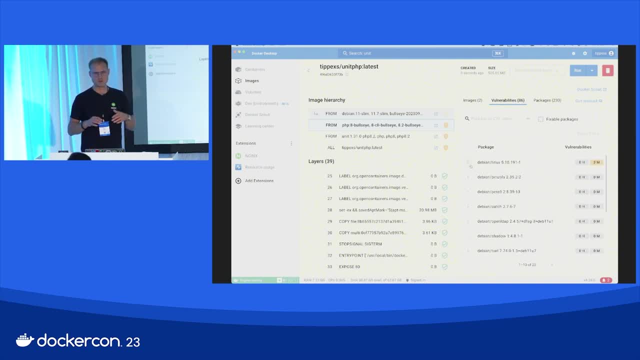 Debian Debian. Debian Debian- fine, So we are not adding any vulnerabilities by ourselves. They are all coming from the Debian base image, which is this one, right? That helps If you have a scan in your registry and it tells you you have vulnerabilities. 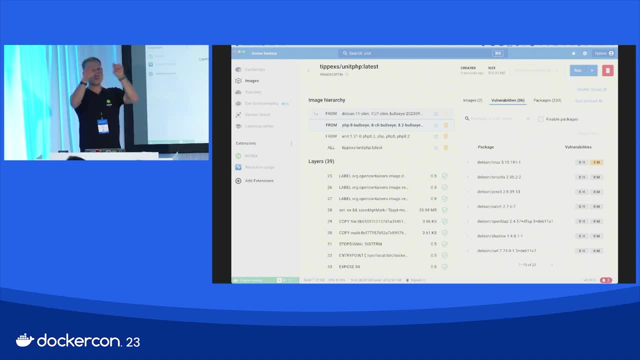 in your image. it does not tell you in what part of the database right. It tells you in what part of the database right. It tells you in what part of the database, in what part of the base images, you have this vulnerability. 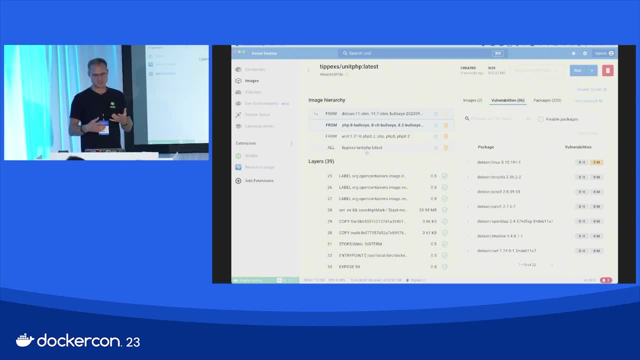 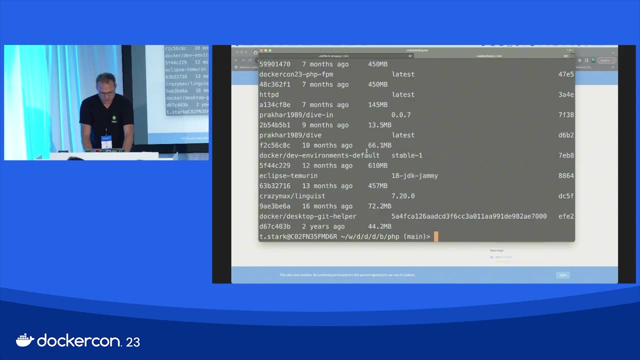 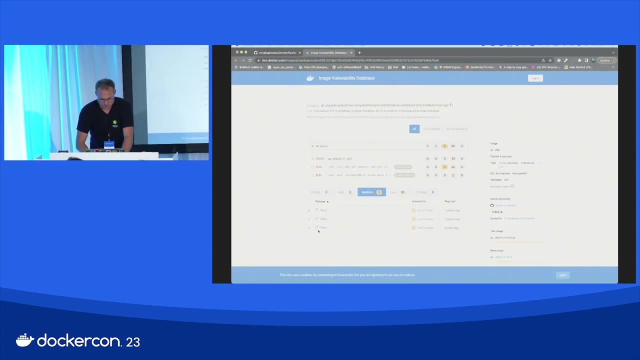 It just says: you have vulnerabilities, And here you can easily find out where those vulnerabilities come from. Okay, So we have this, and now we have we have this tibx unit thing, which is good. So now what we do. 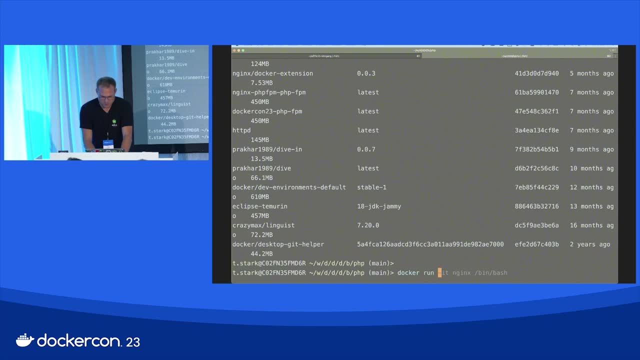 is? we just started up. We can do docker run and then we use and we can dash P, and then we can do, for example, nine, nine, nine, nine, two, eight, nine, nine, nine, and then we had nine thousand, Was it nine? 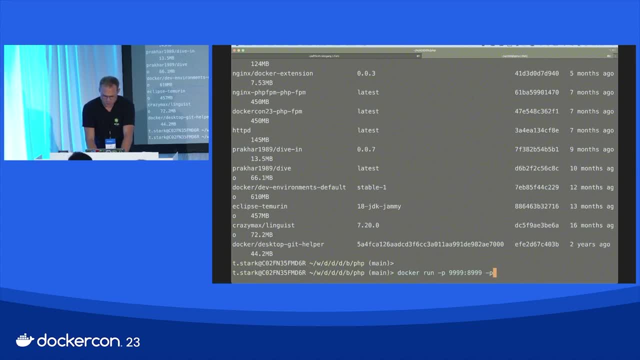 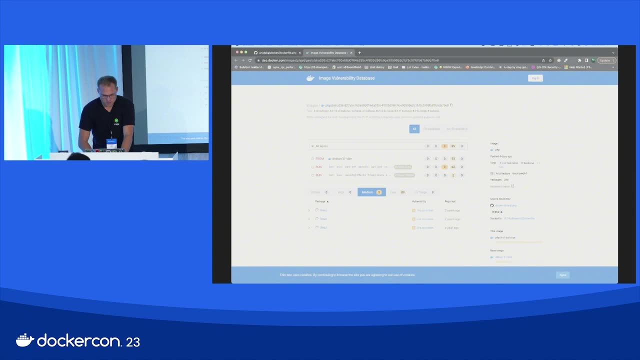 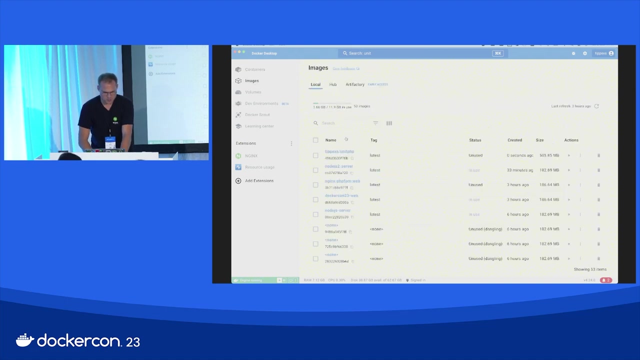 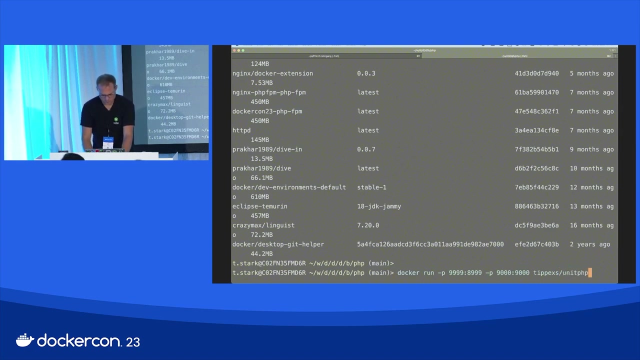 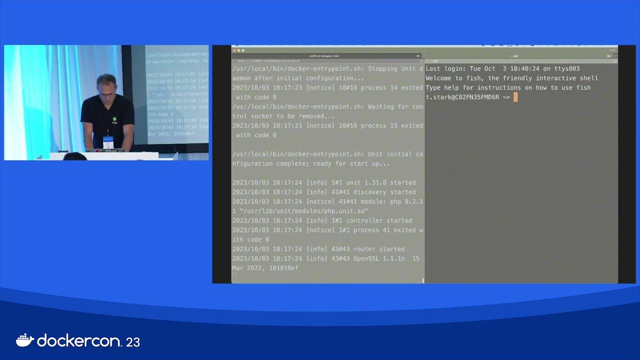 thousand? I think so, And with P we can do. we can forward ports from the host into the, into our container, And I'm not sure if we have a networking. Let's talk this time here, Let's see, Okay, PS. 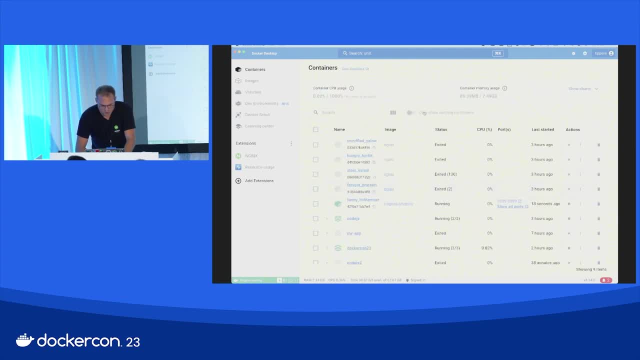 Okay, let's use Deco Desktop, That's more convenient. okay, All right, all non-running. We have the funny literature man, okay, And we have two ports: 9000 and this one, Perfect. So you see, this is why Docker Desktop is just amazing. 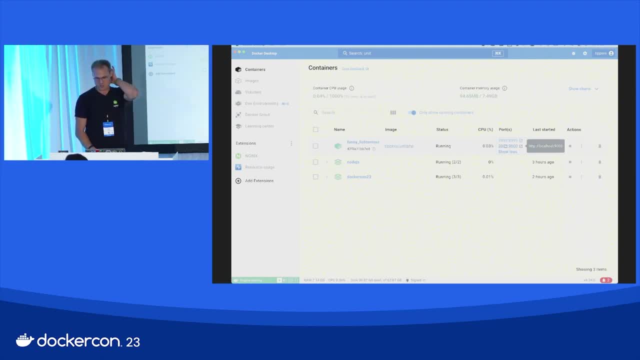 You can see the funny literature, man, which is our unit PHP container is running and we have two ports. We have this one and this one. All right, cool. And this 9000 one is the configuration API. Good, All right. so now I'm gonna show you. 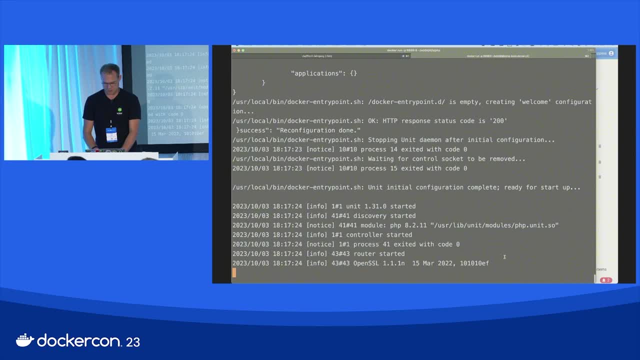 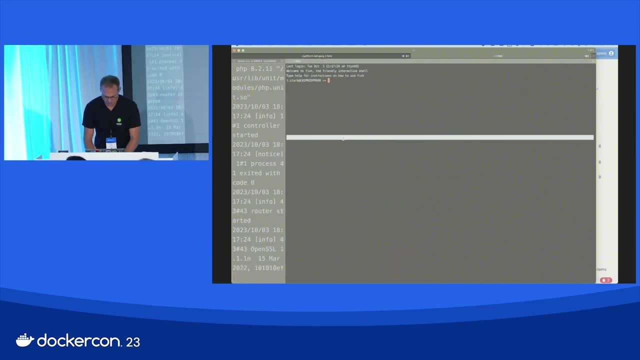 what you basically just have to do to make PHP work without juggling with multiple containers. So okay, as said, we have now local host. 9000 is our configuration API in unit So, and it already exposes port 80 with our default configuration. 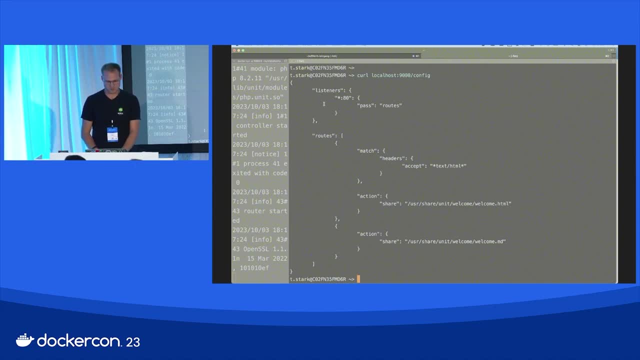 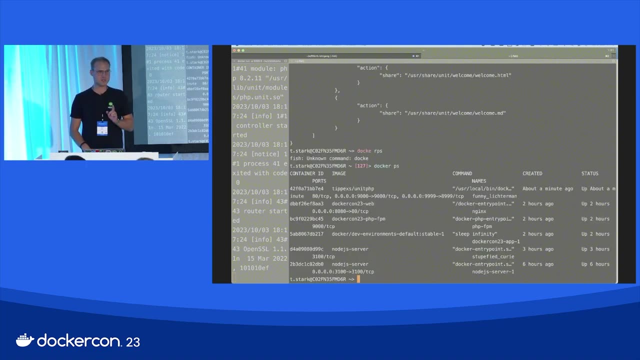 and should print now: hello world. So this is the thing, but it's on port 80.. Okay, too bad, And this is one thing. there is none. there's not an existing solution right now. still, You cannot easily bind now another port. 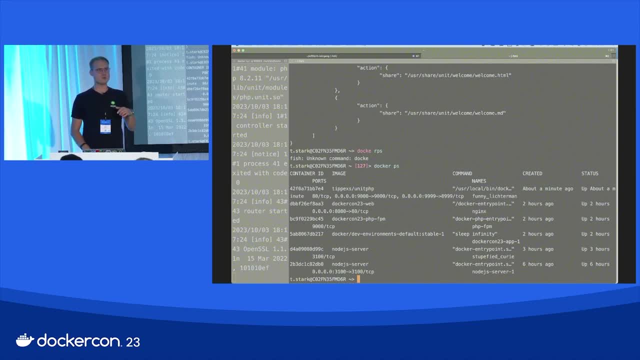 to an already running container Not working. You can do with IP tables and juggle around a lot of. there is not a single solution that works right now, Like saying, okay, we have exposed port 9999, that goes in the container to 8999, but now we 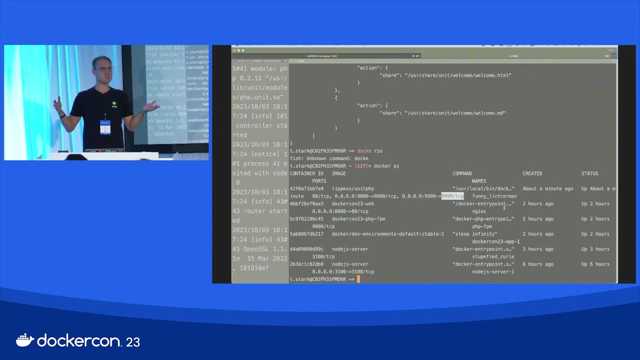 we recognize it's port 80. Only thing we can do is stop the container, recreate and now listen on another port. There's none. there's no good solution that adds ports to the to the already- yeah, already- launched container because of the way Docker manages networks. 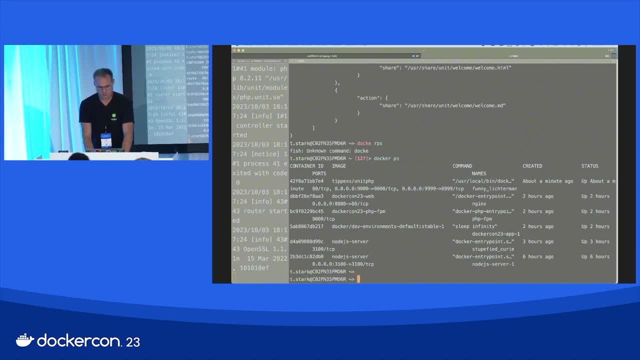 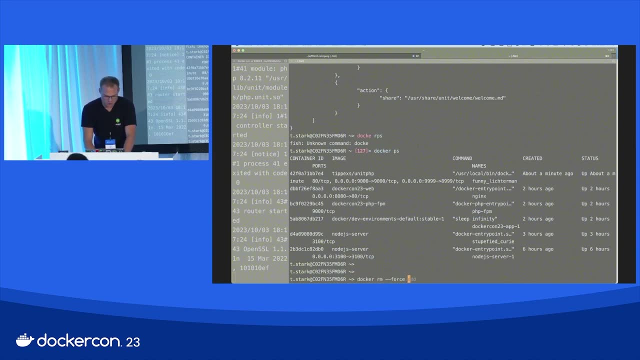 and all this IP table stuff. That would be. that would be nice if we can expose ports dynamically. Okay, The quick and dirty way is always to do docker-rmcom. Okay, The quick and dirty way is always to do docker-rmcom. Okay, The quick and dirty way is always to do docker-rmcom. So now it's like I don't care if it's running or not, That's it. So docker-rm, dash, dash force will stop the container and delete the container. 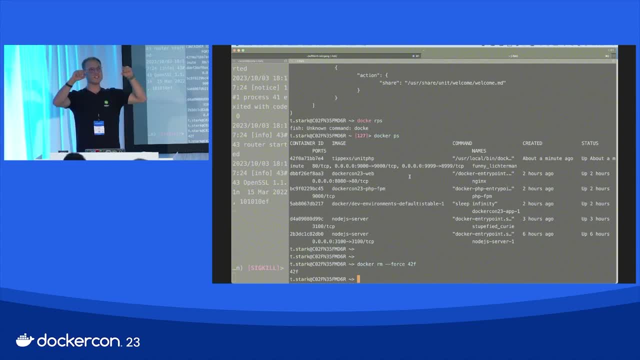 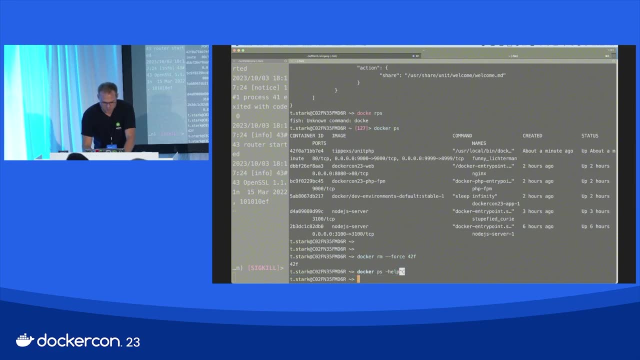 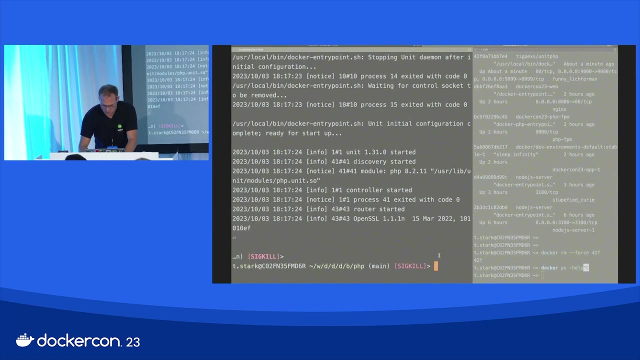 Make sure that you save everything you put in this last bread slice, because with this command it's gone. Okay, Very, very important. So now let's start. let's start the Docker container with port 80 actually. So let's start the Docker container with port 80 actually. 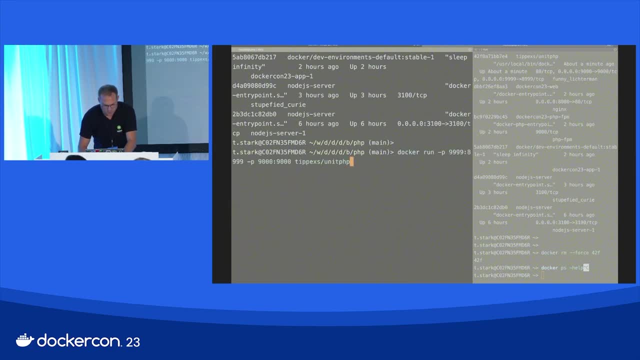 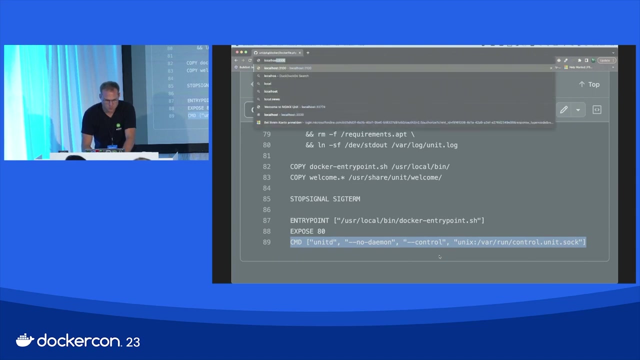 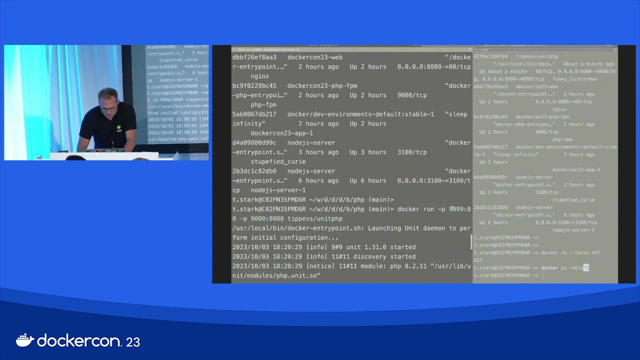 Docker help. So we keep 99999 and now we do 80.. Running Perfect. So that means, when we do now local, local host 89999.. What was it? Oh, it was 99999.. Okay, 99999.. 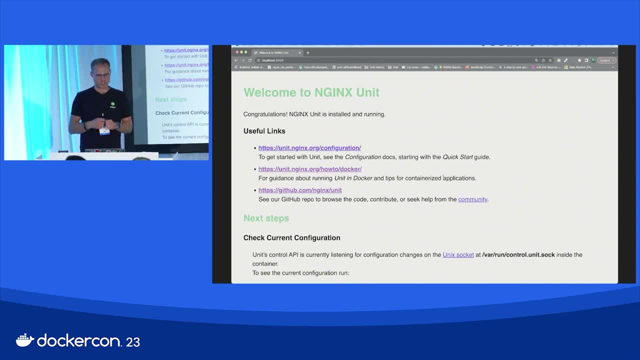 Okay, Good. So two things. We have successfully launched nginx unit. Perfect. We see the default hello world page- Awesome. And we recognize that with dash P we can override literally anything that somebody else defined in this expose command in the Docker file. 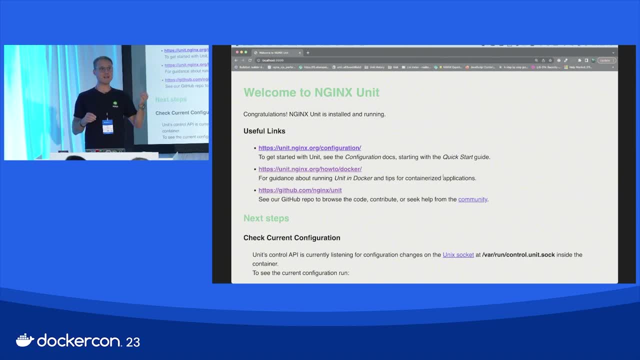 Okay, Because we defined something to expose port 8999, but we are not using it at all. Right? So if you define Docker run dash P or in Docker compose, you use the ports command or this dash ports, you can expose any port from this container. 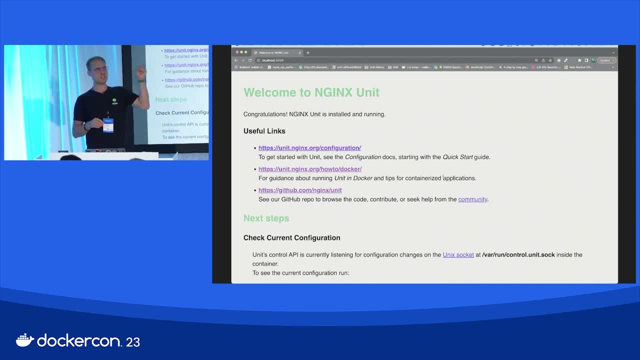 That's on you, That's your choice because it's your nut network. You say dash P, this port, independent from what the administrator of this Docker file or the creator put in the Docker files, expose command. Okay, You can always expose any port you want. 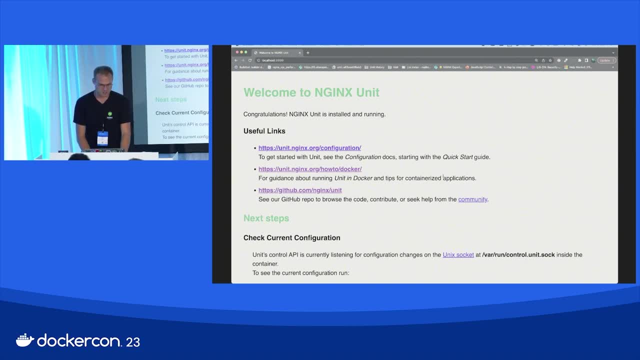 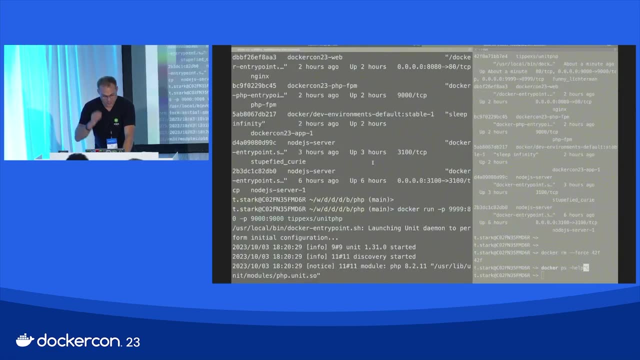 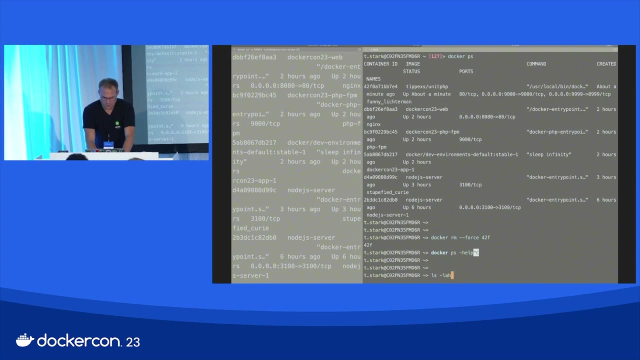 to your host machine with dash P. Okay, So now we have 99999, which shows our nice little thing here, but we would like to use PHP and make it easier than just things. All right, Good, So let's make that a little bit smaller. 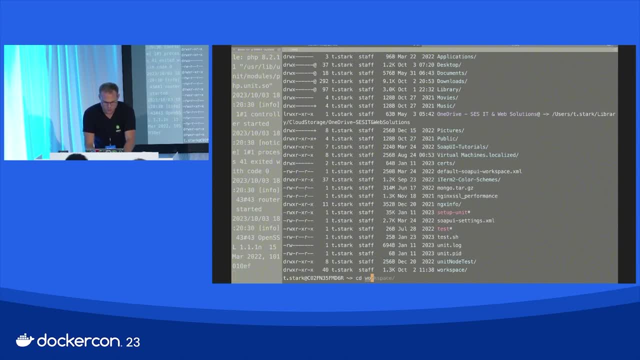 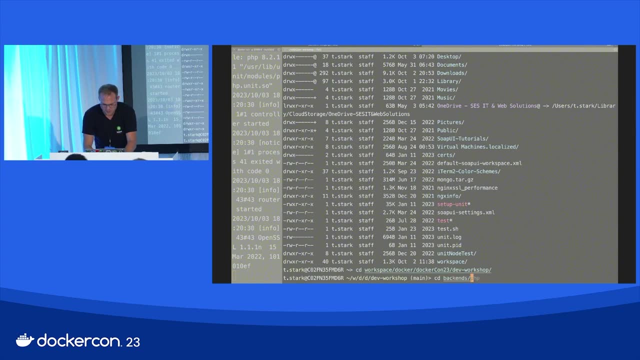 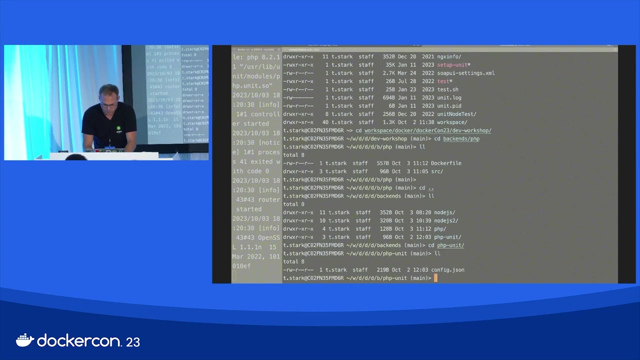 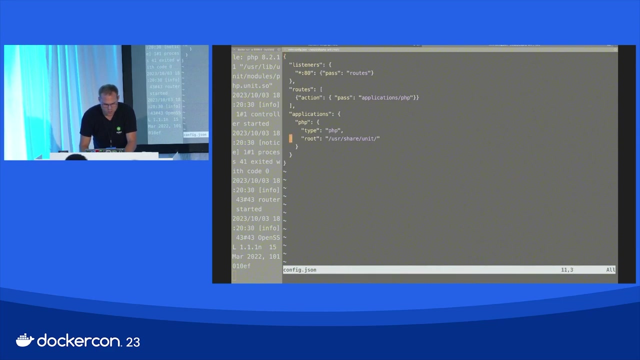 and configure unit to work on PHP. So we do workspace Docker con, Docker con dev, workshop, back ends PHP. I think PHP unit is there: Route action, pass, user share, All right, So this is a I've already prepared a configuration. 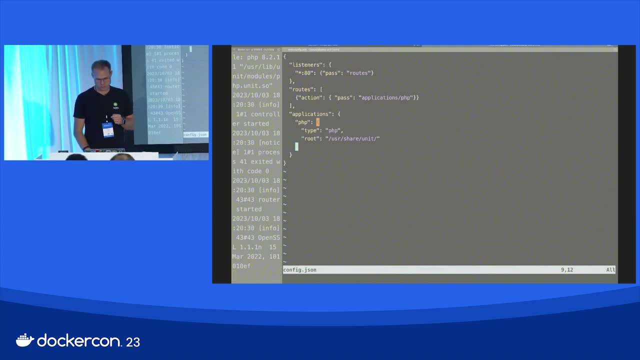 That's nice. This is the JSON configuration for Nginx unit And this is all we need to like to run in PHP application Docker container. No more FPM, no two containers that are connected to each other. Nginx unit one. 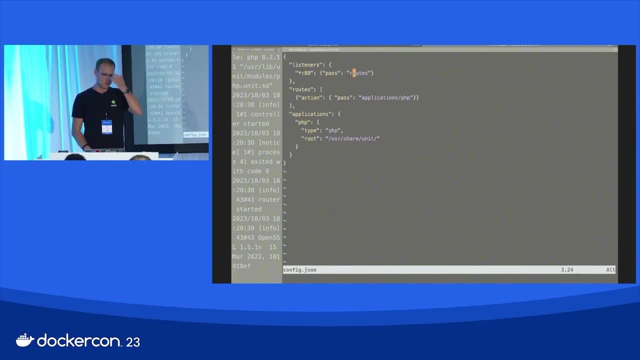 And then this configuration And that says we open up a listener on port 80. The route here is- I will show you that in an example in a minute- The Nginx unit router. that's a very powerful thing, because what we can do is. 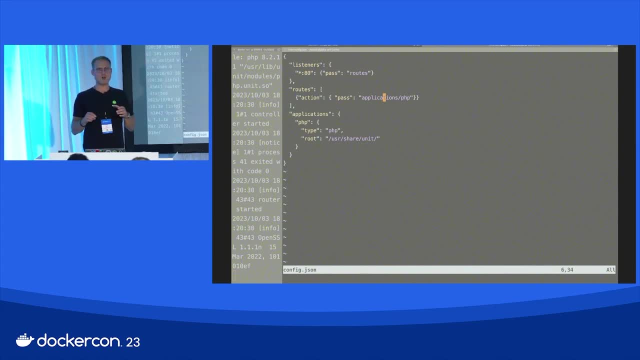 we can inspect every incoming HTTP request and can get all the information on the metadata, like host name and URIs and arguments and cookies, and make decisions where to send this request to based on quite all the metadata of that request, And this is fundamentally different from NGINX. 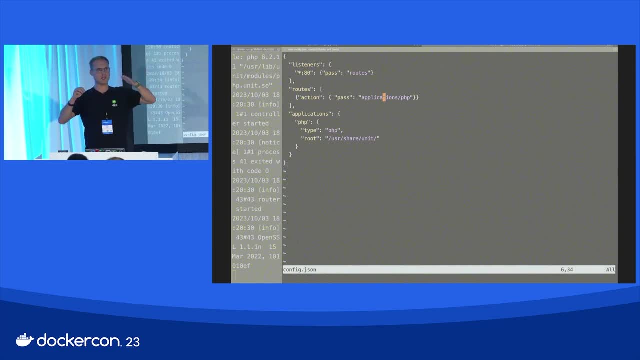 because NGINX is location-based. Anything that fits well in location, like slash, location slash- something that works perfectly in NGINX. But if you ever try to map requests by HTTP header or cookie or argument, try to match something that is in an argument. 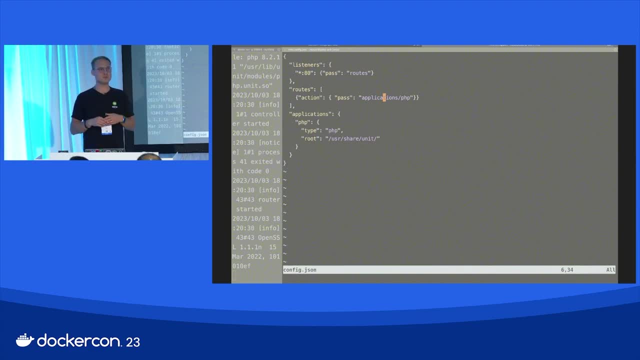 inside of an NGINX location. Literally not possible. that easy, Because in this location matching in NGINX, you do not have access to arguments. You can write a map or use NJS. That's really annoying. So with NGINX unit it's super easy. 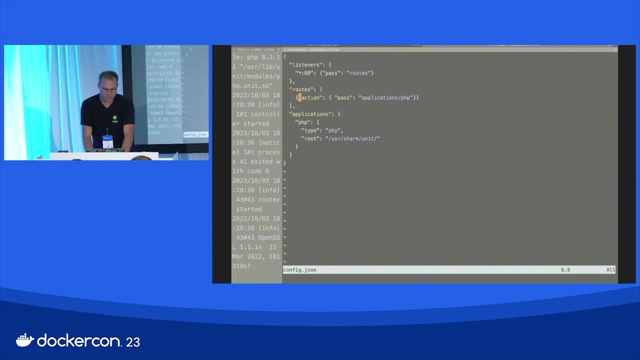 because you can put in this routing objects, we have action, good, And next to action you can put a match block which is match, And then match is another, another thing, And then we can do URI, something is test, for example. 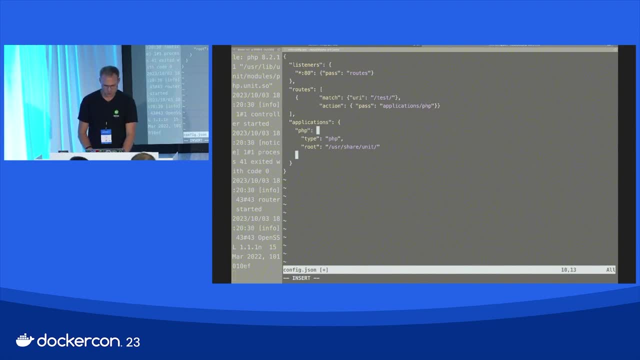 And if URI matches test, we invoke this action, Or we can put arguments in here, We can put HTTP headers in here, And we have implemented the NGINX JavaScript runtime to unit as well. So we can- either we can even define here. 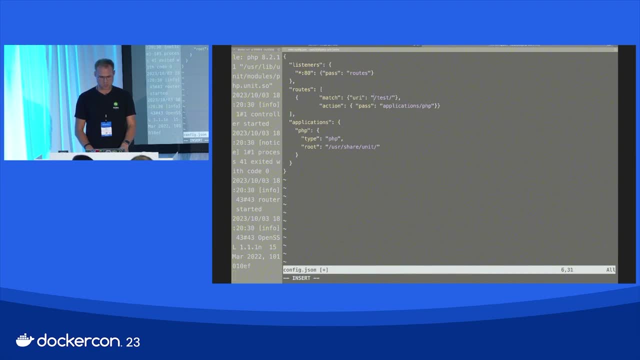 template literals in this block and can invoke JavaScript. We have implemented the NGINX JavaScript function to do very fancy stuff with matching, like and like, whatever you can think of, Like. really, that's just super amazing, And I'm just afraid that it's like. 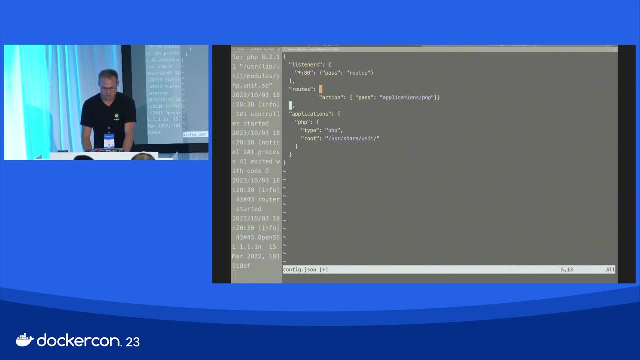 we already had four hours. that is crazy, And I could tell you for another four hours. that's cool. So we stick with the action and say: pass it to the application PHP, A thing that let's call that app, for example. and then here we say, okay, that is applications, app, app and the type is PHP, the root is user share unit. and then we can do: okay, the index is indexphp. 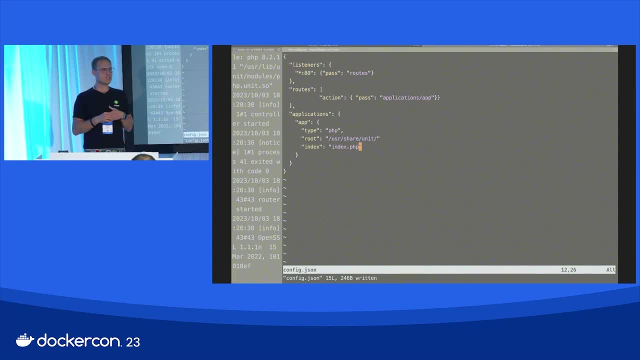 Done, Okay, perfect. So and as Nginx unit implements the server API for PHP and the API of eight different other languages, you can run Ruby applications in Java and Perl and Python and PHP and WebAssembly since a couple of weeks natively on unit. 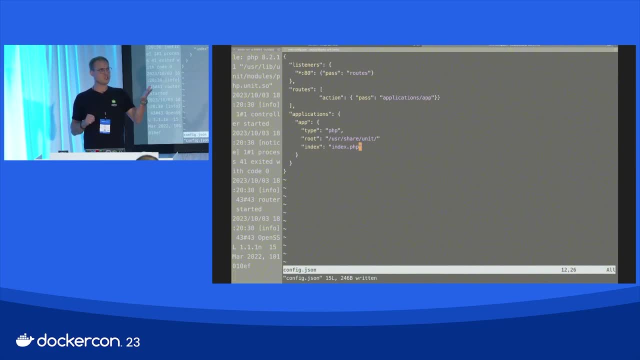 So it's just in a single container- Nodejs, for example, as well- and you can share static files, and I hope I can show you that in the next 30 minutes so that we can see how easy that is. Because this is this makes it very efficient to work with images, because you have a single server binary or a single container image. that can do a lot of things for you. 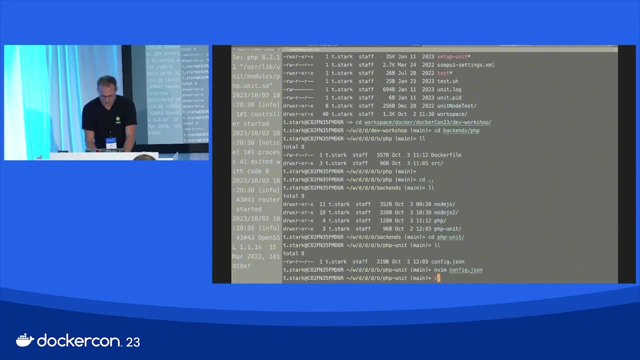 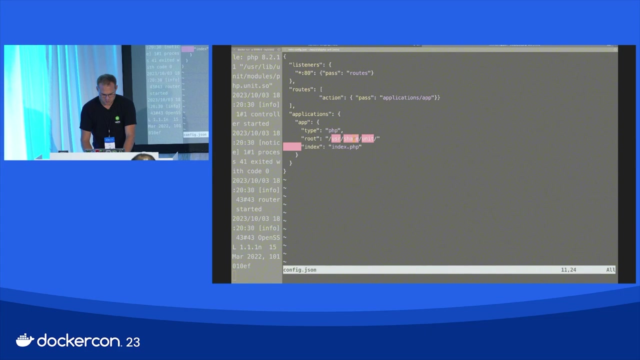 Okay, so we write that and now we try to send it and there is a unit CLI we can use or we can. I have a typo again. I have a typo again. Oh, Oh, Here is a missing comma. 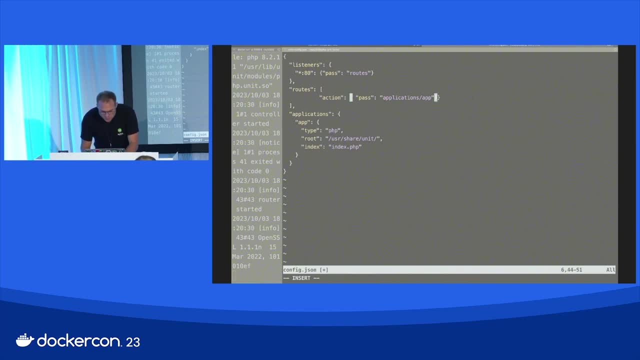 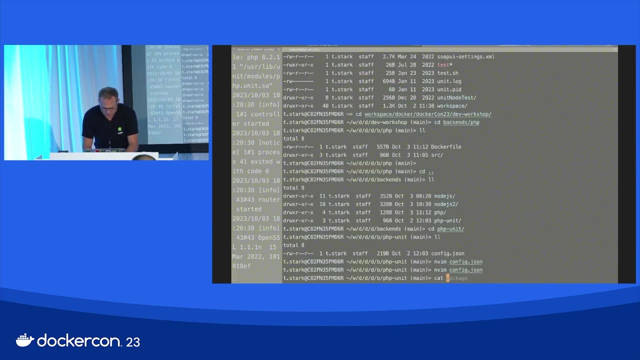 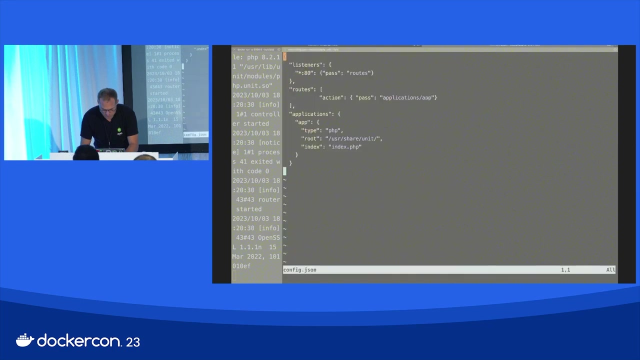 Let's see. Thank you, Let's do cat config, my friend JQ. All right, That's what I mean: Always, Always. Where is it? Okay, we have pass. This is the action. Oh yeah, there is a. there was a, okay. 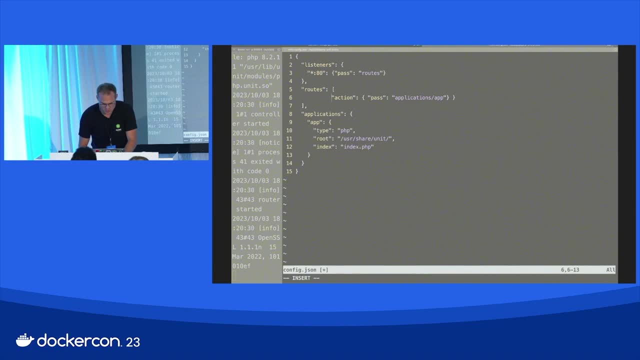 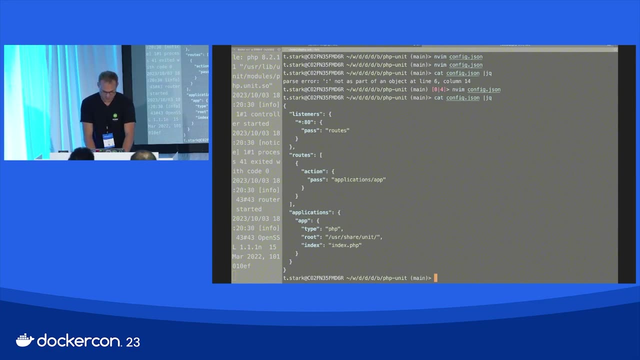 This was needed, but I've deleted the. yeah, it needs the action, the object here. All right, That's far better. Okay, Amazing, Good, So that works. So now we can send it over, Like we cat config JSON and we pipe it to curl. 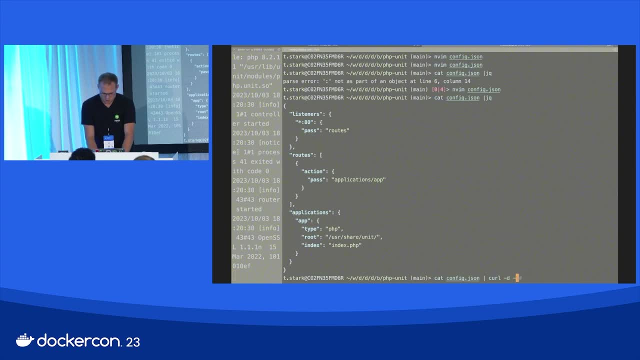 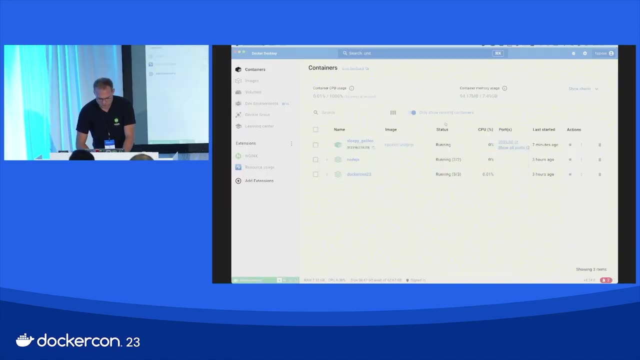 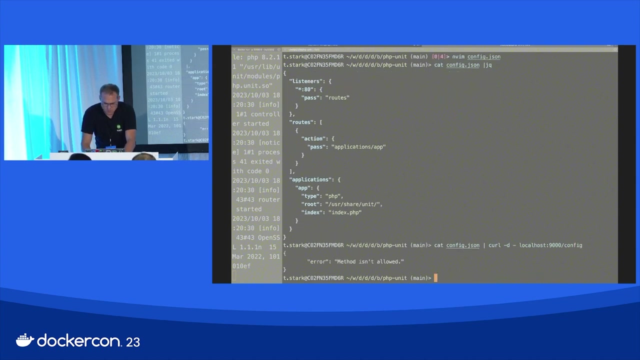 Dash, D dash to local host. What is it? Nine, nine, Jesus, I can't even remember what ports I've used. 9,000. 9,000.. Oh, I'm sorry You're using put, Not put. 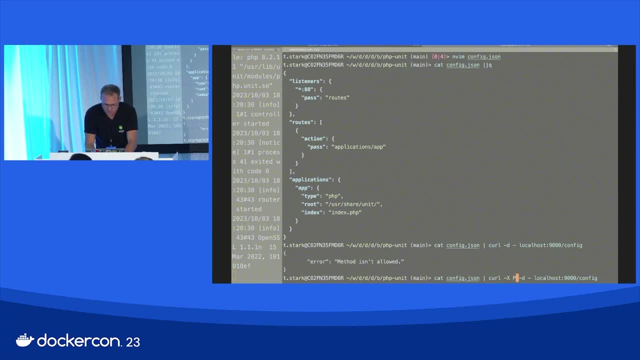 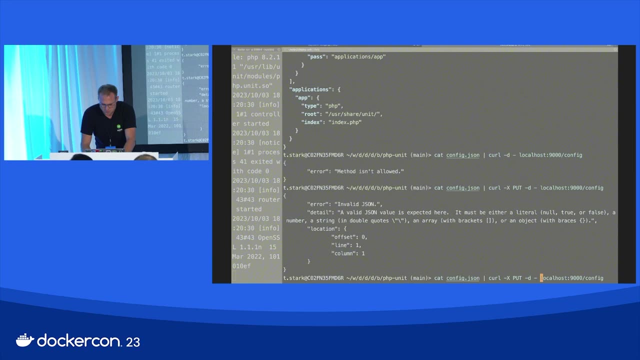 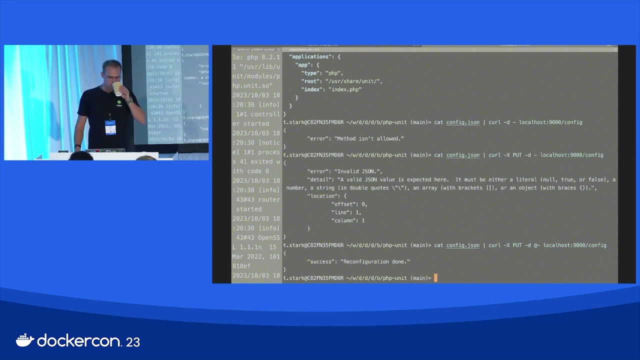 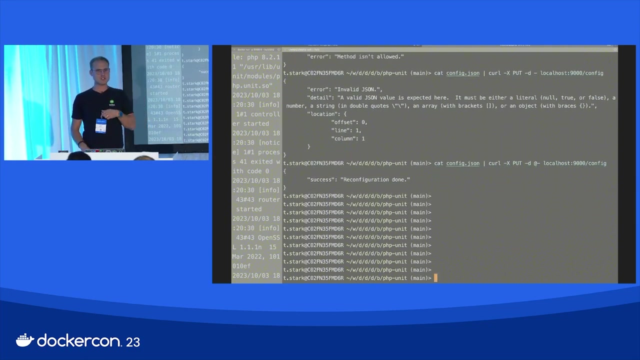 We need put So access, put Good, All right, Good Jet lag kicking in, All right. What we do here is- you see, I love working with the Linux command line- We cat config JSON and pipe the output to curl and send it with this add minus like. 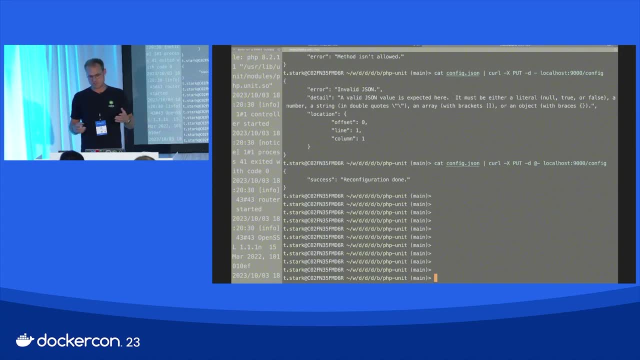 the stream we had from the first command. We just send it over to curl. You can use curl dash x, put dash d for binary data and then you define a file name. That's also possible. But if you want to do some fancy stuff before that, you can use. 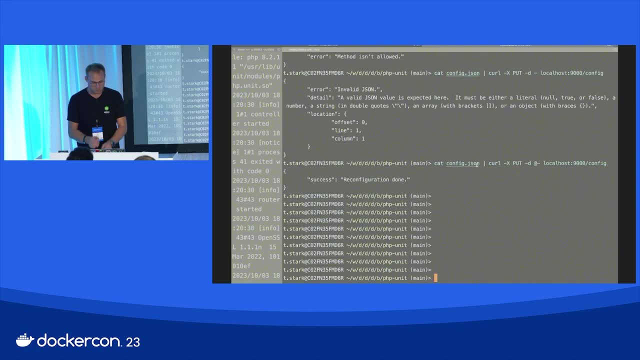 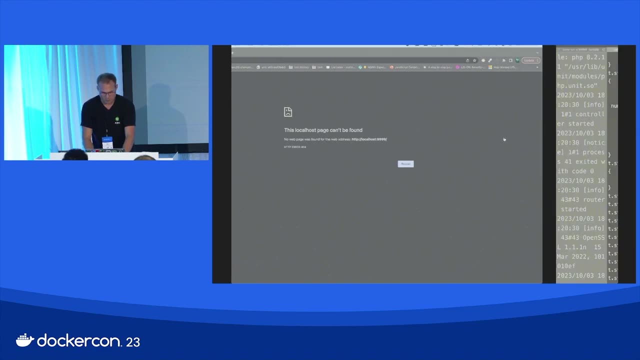 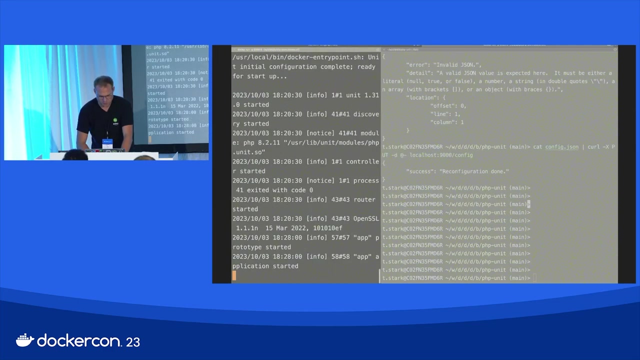 Okay, You can use this pipe thing to just send it over. Okay, Good, So we have reconfigured unit and now let me see, All right, Saying 404.. That's because I think I have copied the index PHP file into a wrong location, but that's. 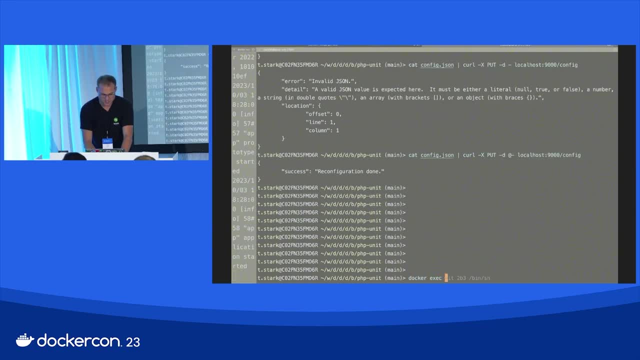 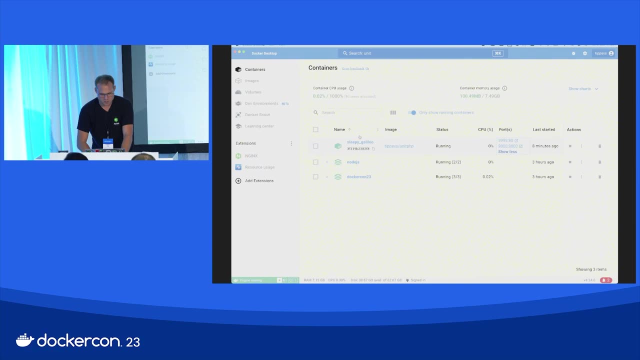 something we can easily find out because we can use Docker exec. Or let me show you another thing in Docker desktop. that's super awesome. You can click on that And you have bind mounts, Nope Files, Yep, So, And this shows you what files were modified during. the container is up and running. 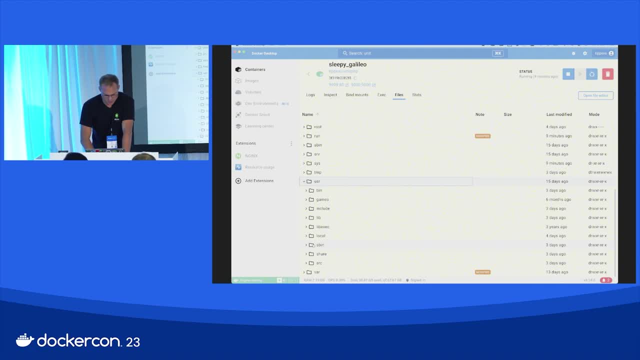 And we have user, I think, And then we had share And then we had unit. So see, we don't even need exec, We can use this little neat file browser Unit, And there's a Docker file in it. 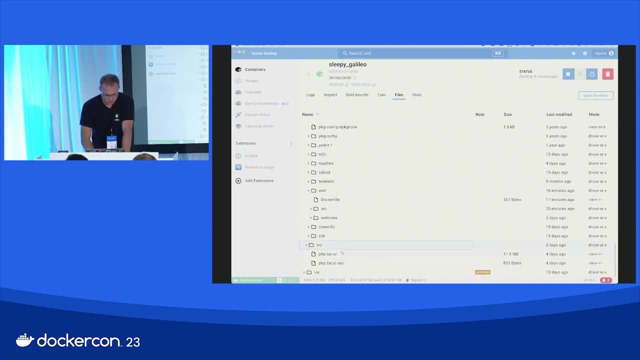 But I Think We had it in source. Where did we copy the files actually? And then I think this is Yeah, Then you can, If it's a real file, you can actually, You can actually edit it. 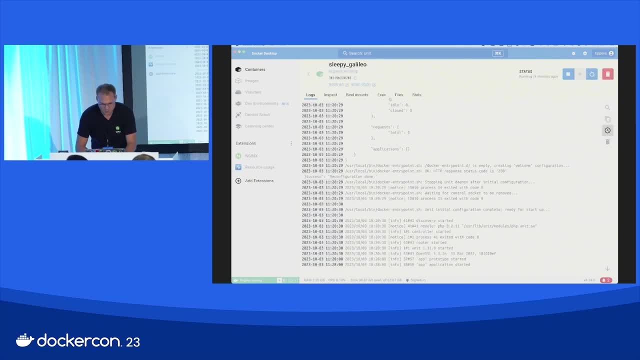 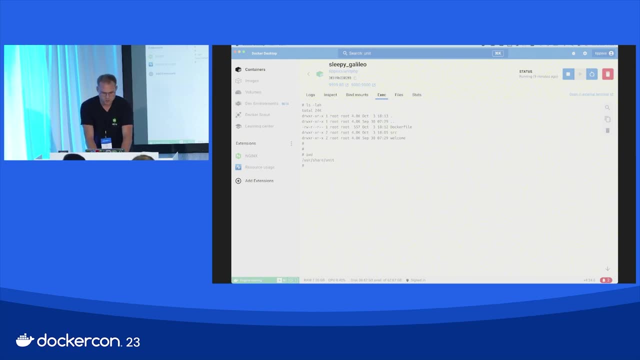 But now we do containers: Sleepy Galileo, Exec. All right, Print work directory is user share unit And I think Let's do Source. There's the index PHP. So it's user share unit, source And then index PHP. 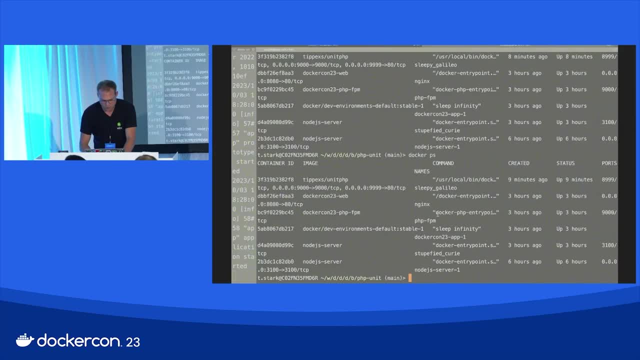 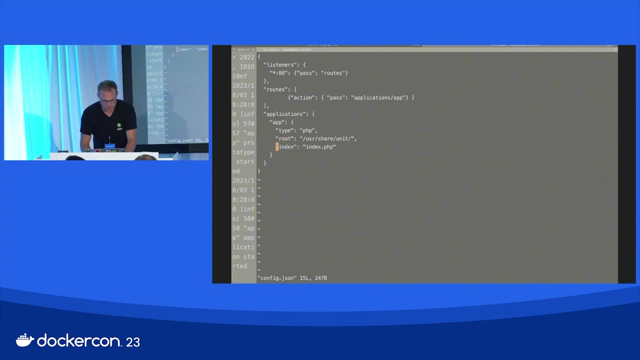 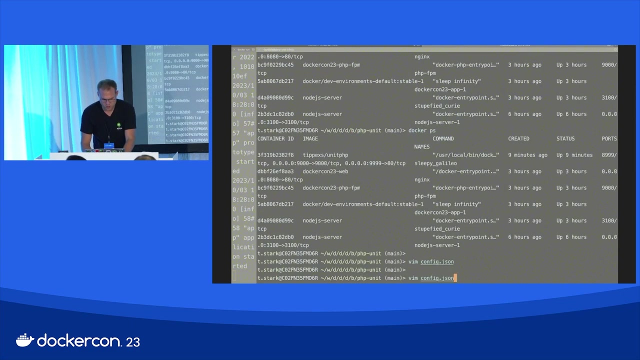 And I think that's wrong, though. So I think we have the wrong Path in here. Yes, It's just user share unit And then we need source, But this way I can show you how this dynamic reconfiguration works. 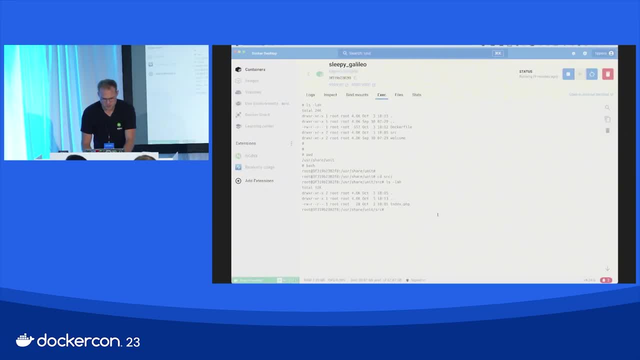 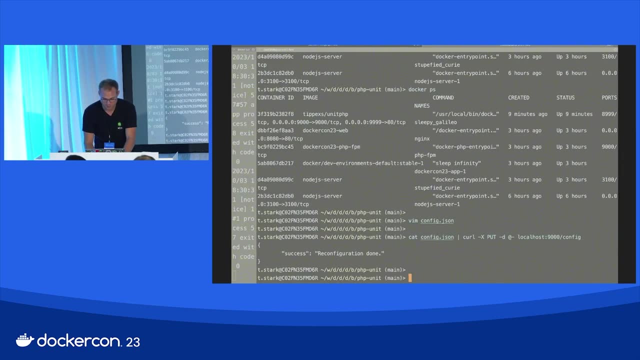 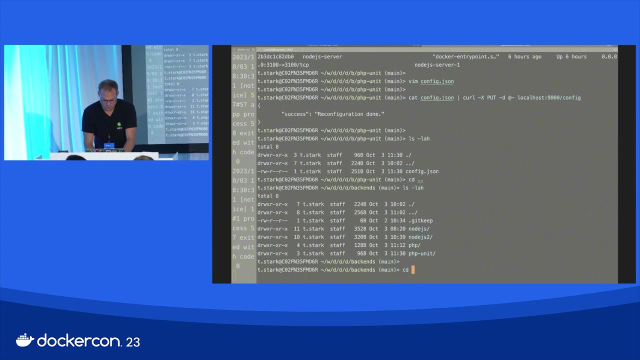 So we just send it to the config API. We're not reloading anything And it just works. Even then, I have a parsing error. We have double quoted string in my PHP file, which is another problem, But this is now something we can fix in Docker desktop as well. 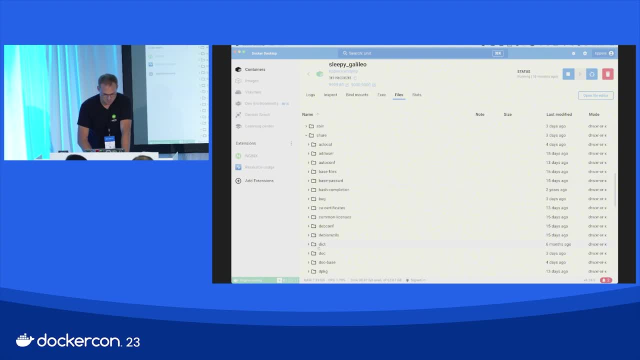 So we go to files And then, But just, We are now working in this last Bread slide, So if we remove the container, the changes we do right now are gone, Right, Just make sure that if you test something here, that you move it back to your host machine. 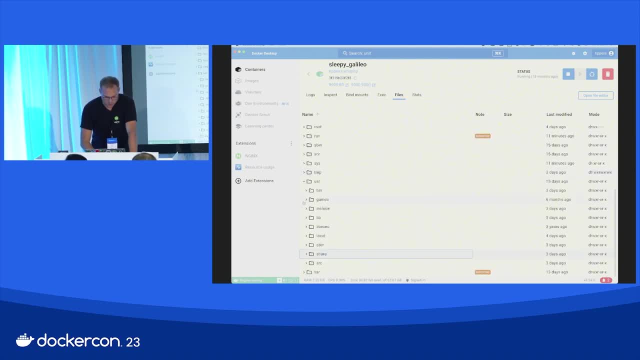 Otherwise it will be gone. So it was share- User Share, User share NGINX. Okay, Now I will submit A feature request. I would like to have a text input here where I can navigate to the things. 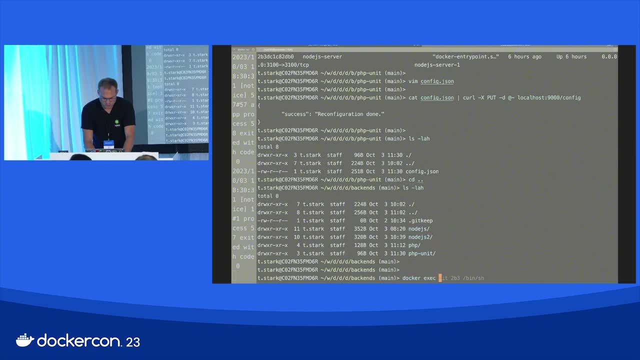 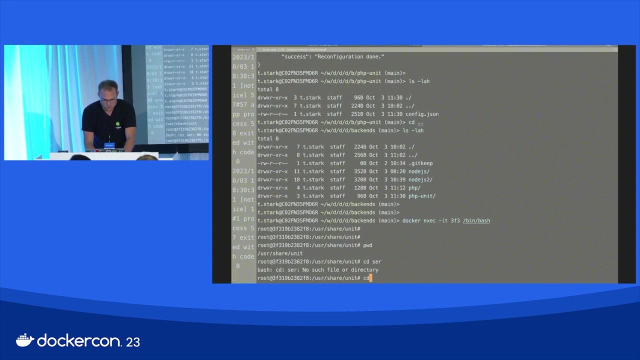 Okay, Now we do it. What's the container ID? 3F3.. 3F3.. Then we do bin, bash Right, Then we end source. Amazing, I thought we have Vim, But it's not a problem. 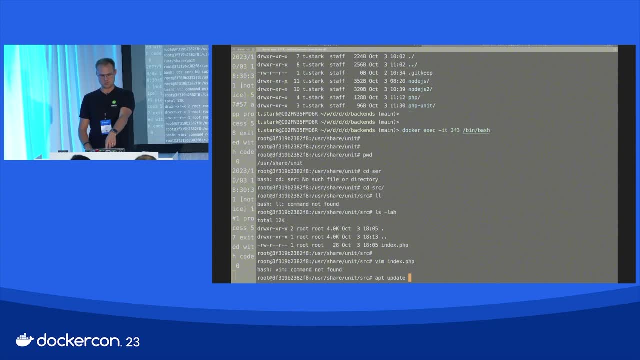 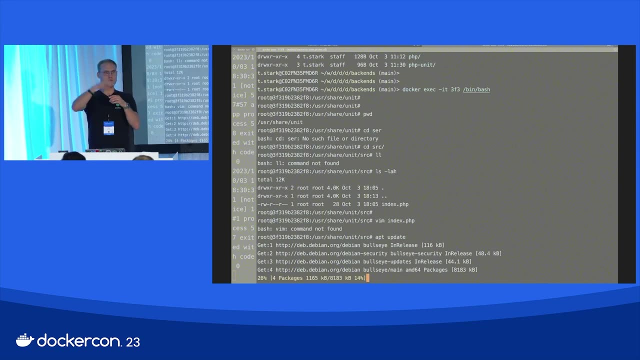 And this is what you can do, Actually with your LDAP stuff: You jump in the container while it's running where you have problems, And then you do update, Because everything you do now is you're putting this in the top slice of this sandwich. 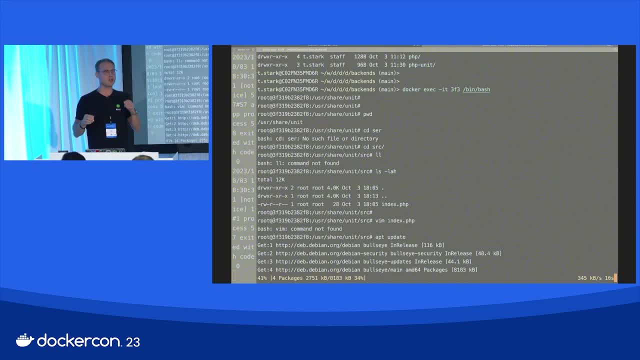 So it doesn't matter If you restart the container, remove it and recreate it. it's all gone. So you don't screw up with any of your official images. You're just playing around. That's basically what we're doing as well. 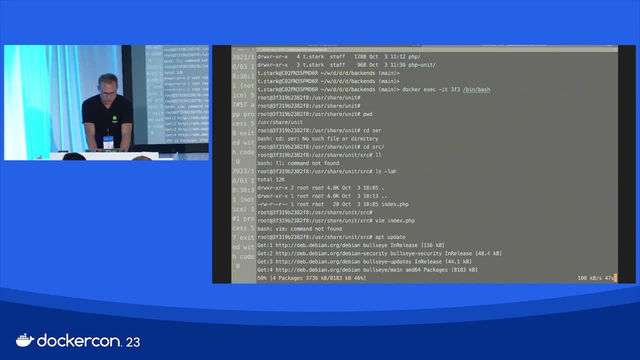 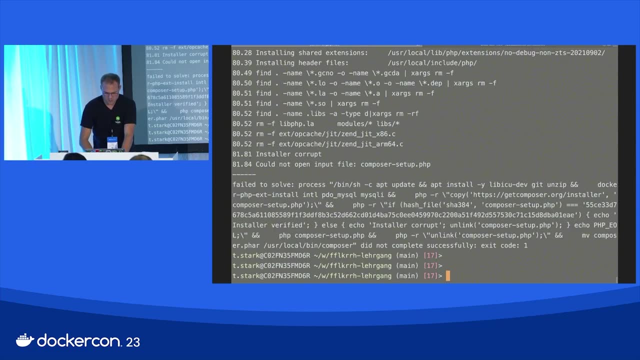 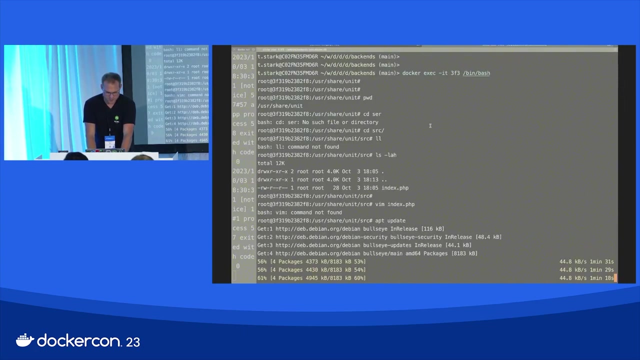 Now let's install Vim. Another thing is, we can now fix the index on. We can fix the index on our machine and then just rebuild the image. That works as well. But let's fix it inside of the container, actually, All right. 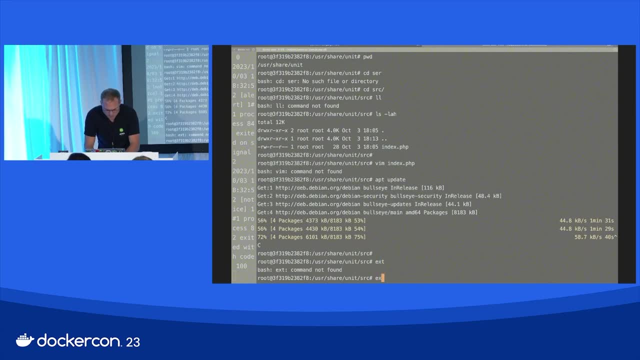 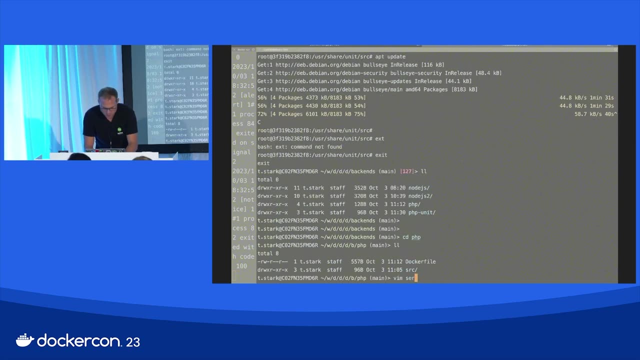 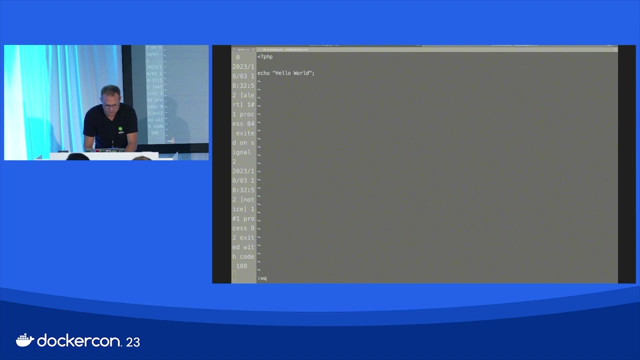 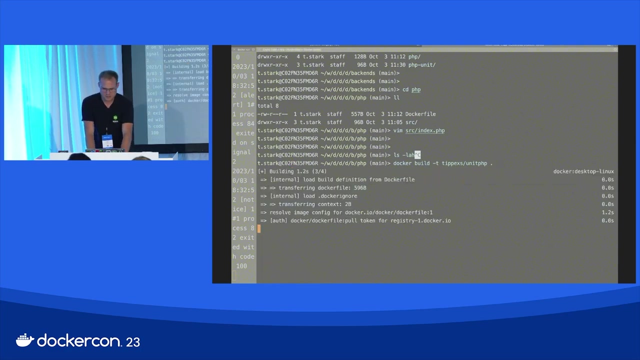 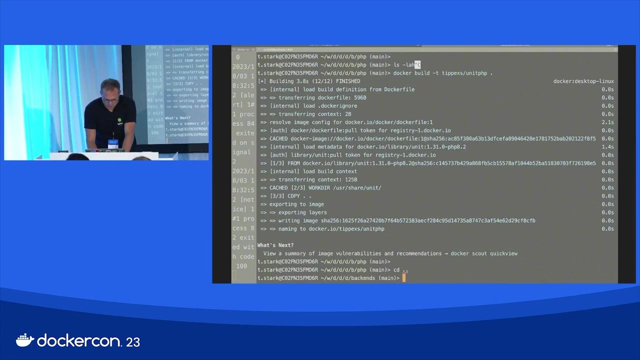 No, that's slow, We don't do this. We don't do this. Okay, Oops, There you go, Build it, And as the config file is not part of the, We can do it. Let's do that Okay. 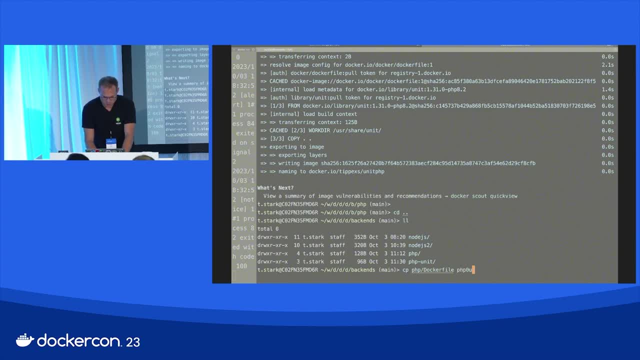 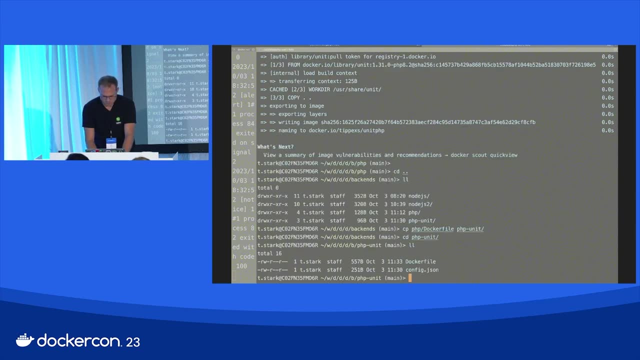 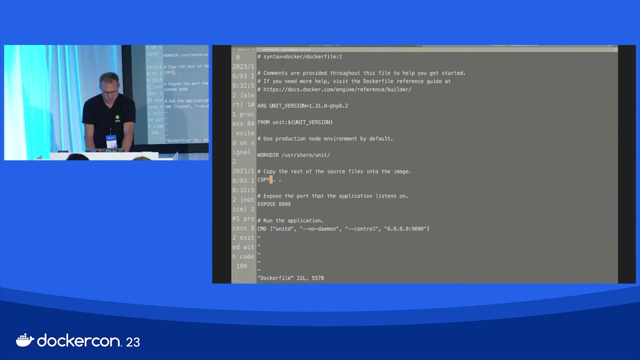 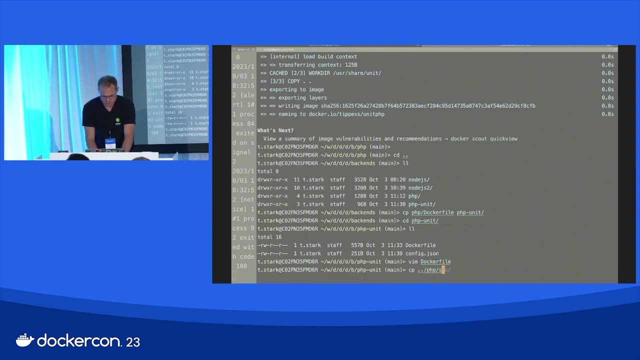 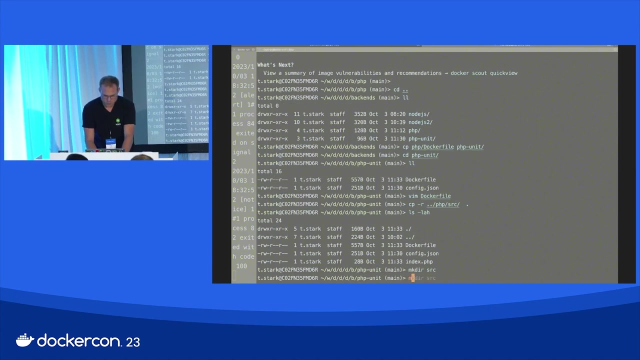 PHP slash Docker File into PHP unit. So here we copy everything that is in Let's, then do PHP source, Let's source. then we move the index to sort, thank you. now we move whatever that is into indexphp. 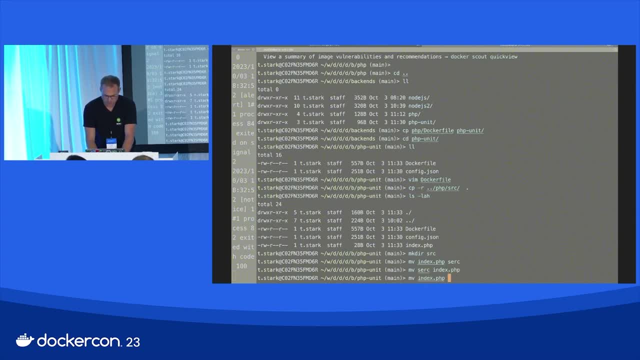 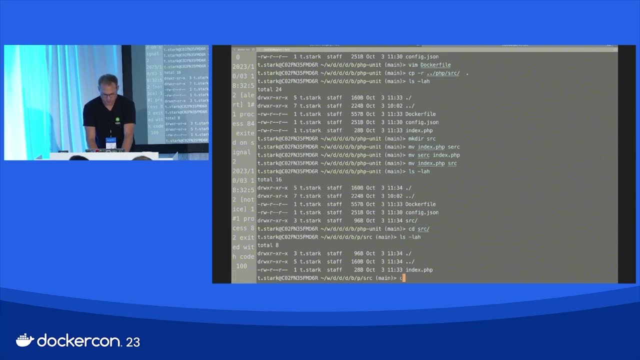 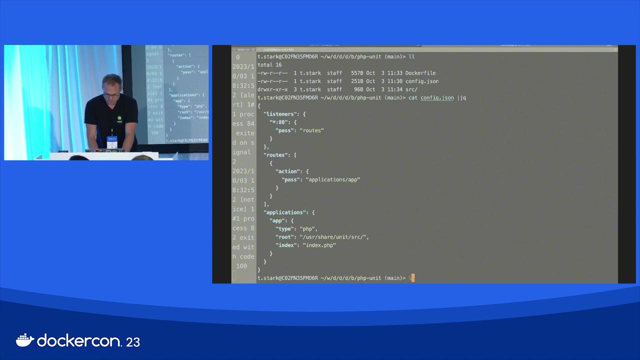 holy cow. then we move the indexphp back to source. okay, that works perfect. now we check. if it's correct, it says echo, which is fine, good. so now we have the configjson pipe to jq, because now I can show you this docker entry point d thing. because now, if we would build it. 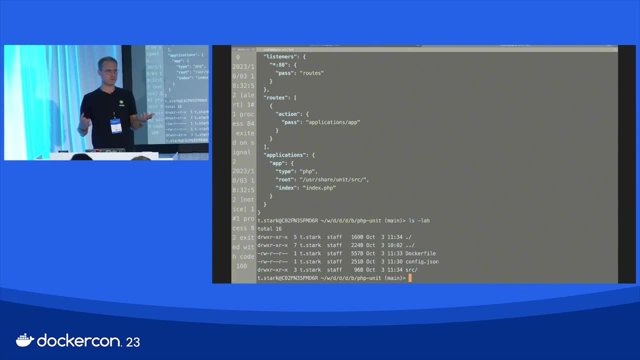 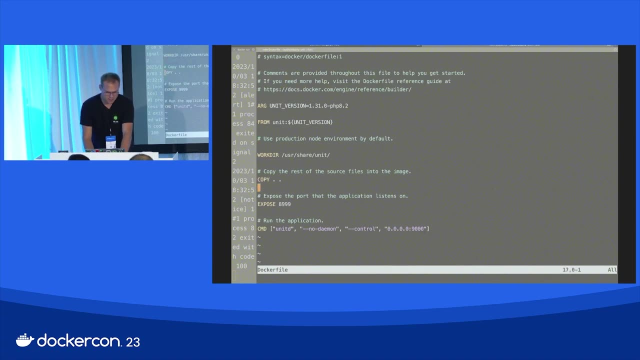 and start it up, it would be empty, so we would see the hello world page, which is not really useful. so what we can do is we can vim the docker file and we copy everything that is in here. and, yeah, one thing that is now super, super important. 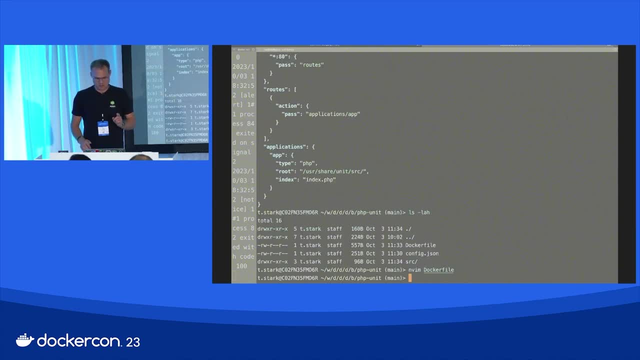 that means we would have the configjson inside of the source thing, which is sometimes not really useful. I would then do in this case, because if you put it in the docker ignore file- you can- it will not copy it anyway to the container, right, it will just not be there. so 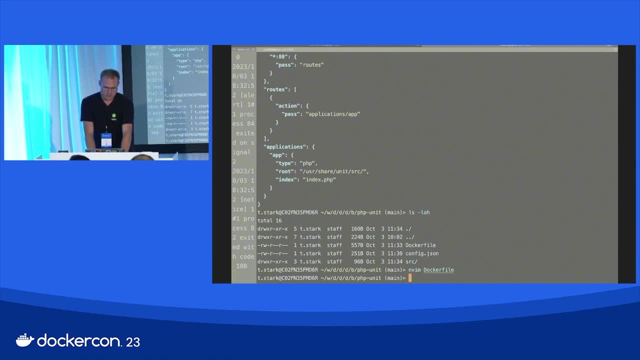 what do you do? What you can do is basically a two-layered build, like one directory that configures the container- if you have something like this, and the other one is just copying the data in it. you know what I mean. if, like a multi-stage build, one is using one is using nginx unit. 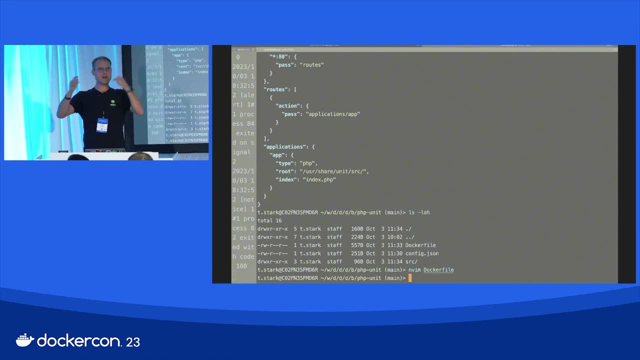 and then you copy it to the container and the other one is just copying source into the container and not and not the rest. but yeah, or in this case, what we can do is docker file and then we do. okay, we do not. 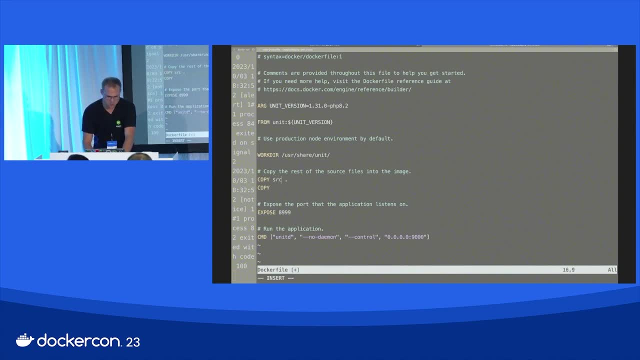 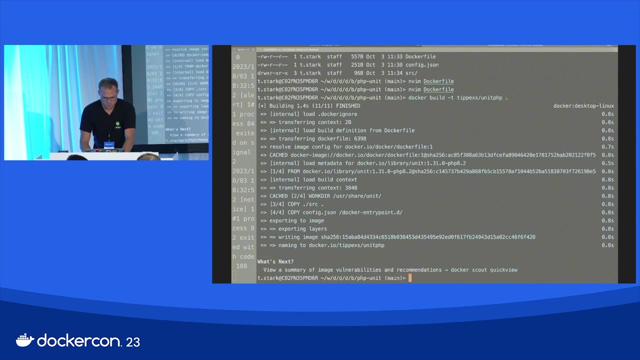 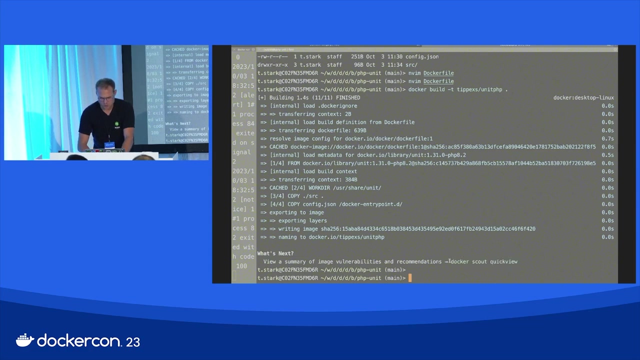 we do not copy everything we do. we say, okay, anything that is in source goes into dot, and then we config. we copy, configjson goes to dockerentryd. All right, good, So this is new docker scoutquickview. it's like that will scan it for vulnerabilities as well. so if you build an 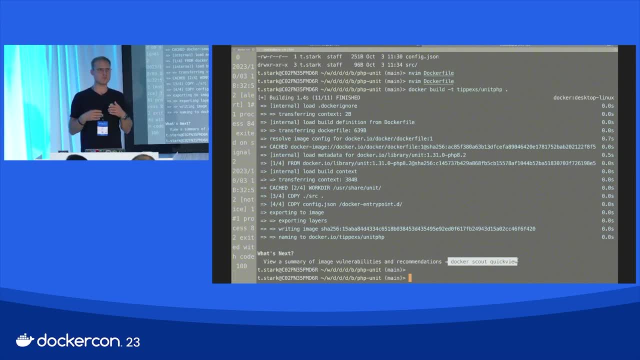 image and type dockerscoutquickview. it will just take some time because it loads data from the internet of CVEs. this will show you a nice little graph how many high, low, medium vulnerabilities you have in this image. pretty neat. it's similar what you have in dockerdesktop. 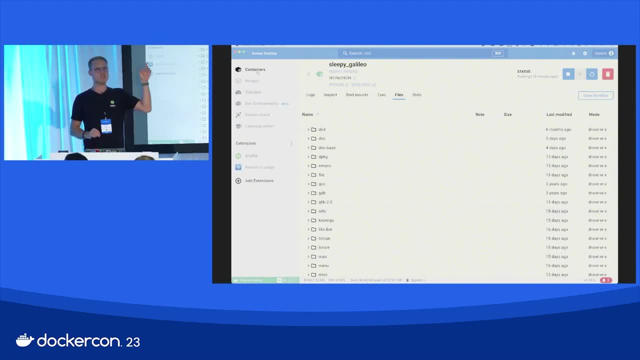 but this will also work in your CI and CD pipelines. you can use dockerscout in your CI CD pipelines, Because dockerdesktop is something you cannot use in your docker in your pipelines, but dockerscout is something you can use. 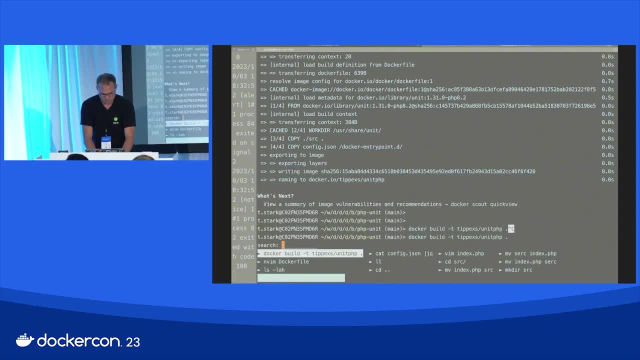 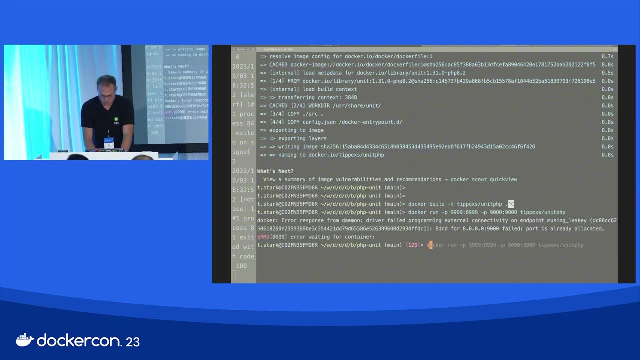 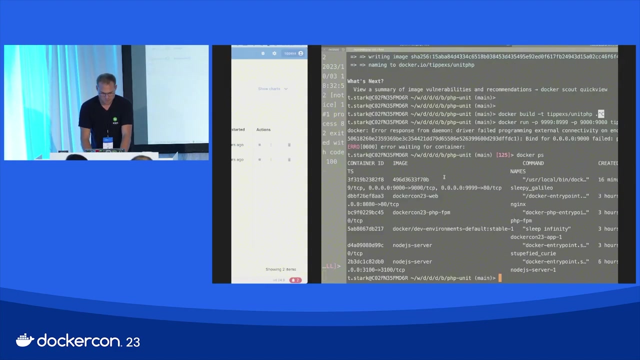 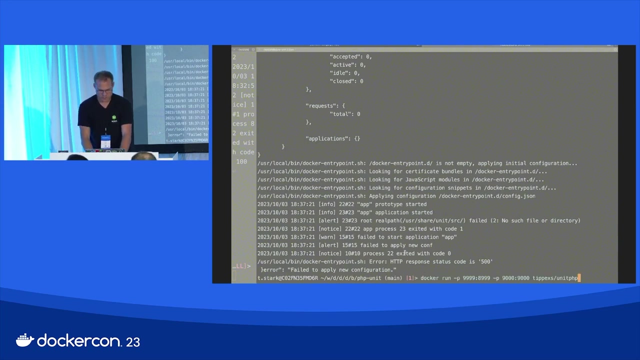 Good, now we have builded the image, So now let's run it again. Okay, still there, da da da container. where is it? Delete forever. Okay, this 500 is now because of. we have changed the path, we have not modified the. 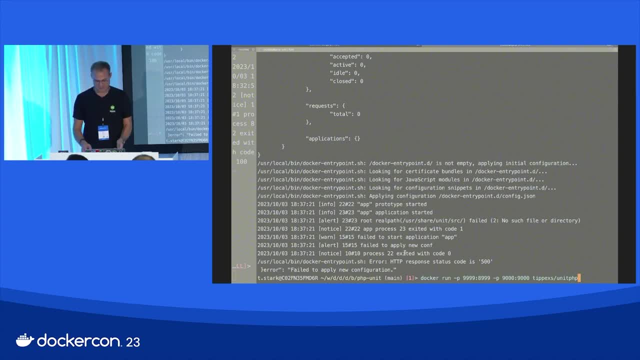 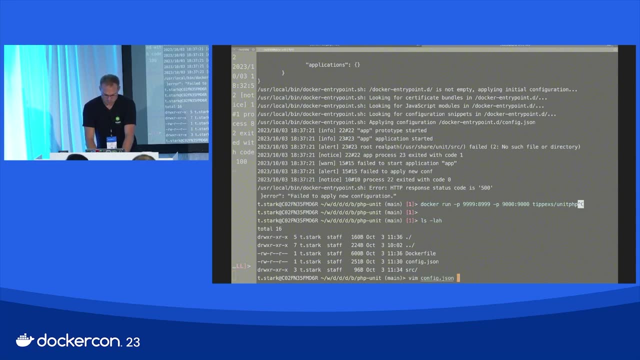 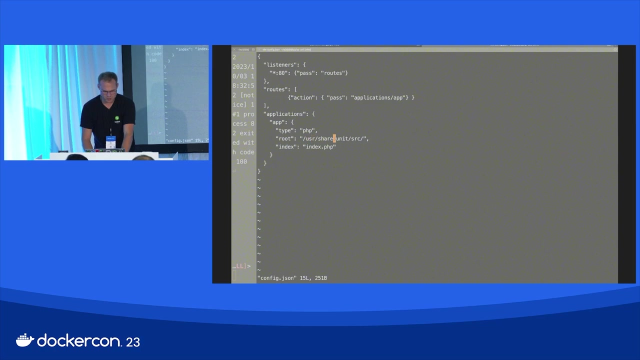 configuration. so now unit cannot find the indexphp file and will fail right. So because we have now, we copy source, so it will now be unit share, unit source source, which is wrong. so we do this. 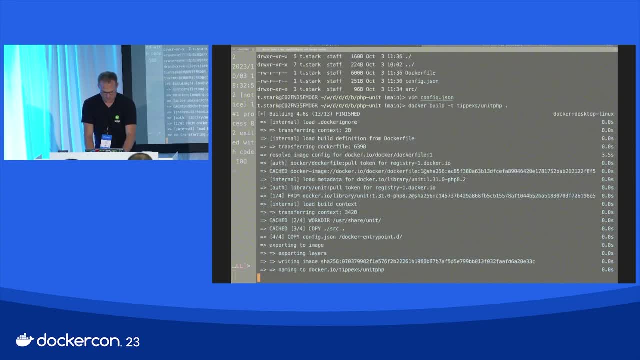 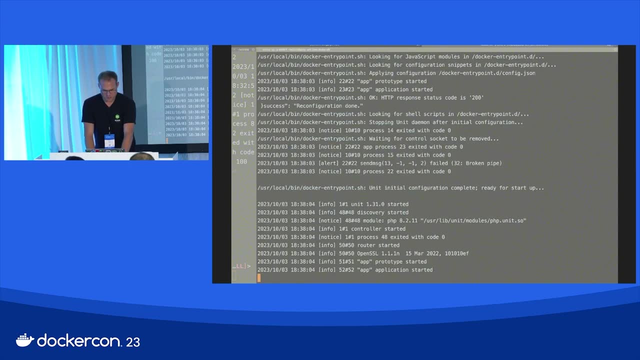 And then try it again, and if it still fails, then I can show you now it works. what could we have done before. It fails with an HTTP 500, exits the container. Okay, so it means we do not specify anything specific, but something fails while starting. 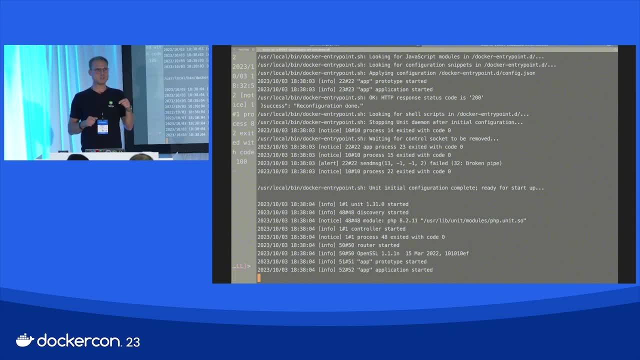 What we can do, then, is we can start the container using an alternative. entry point does mean docker run something And at the end, dash bin bash. that will not execute the CMD line, but we have an interactive shell in the container. 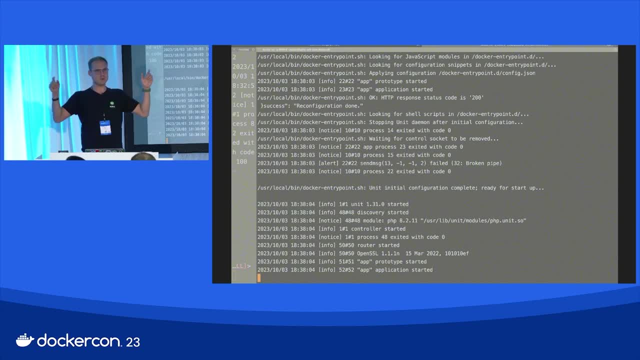 Then we can execute the CMD line manually by hand by just copying what we have like unit D: da da da control. It will fail. but then we can go in the container and do. is it clear? should I show how that? 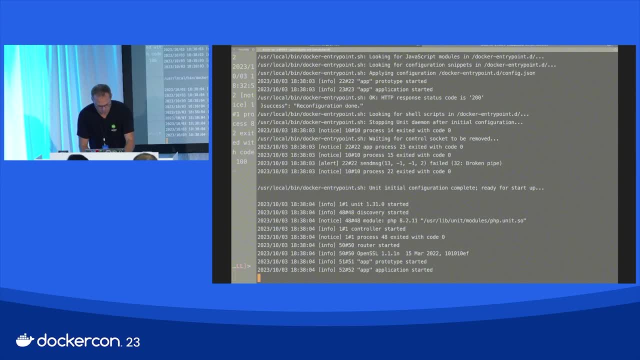 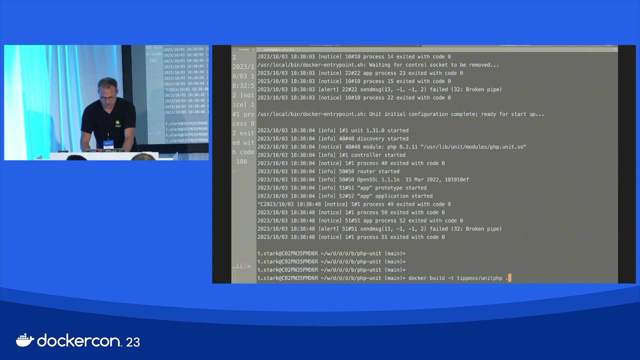 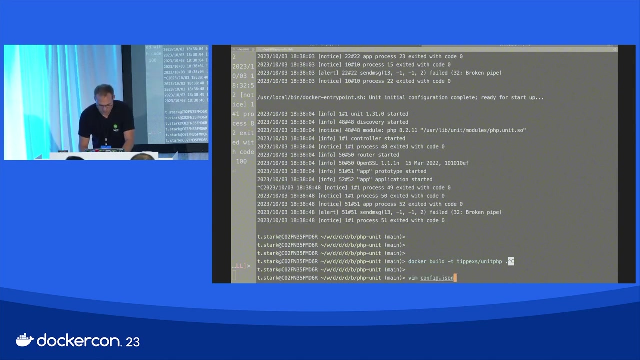 works. It's clear, isn't it? Okay, let me show you how that works literally. It's really simple and it's super helpful. Okay, So it fails for whatever reason, right, And we think there is some. and it's not even booting up, it's not starting. 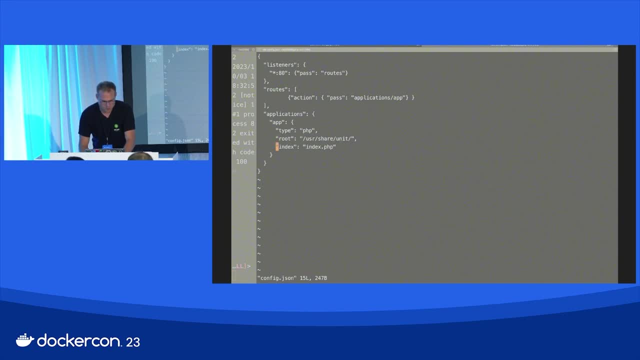 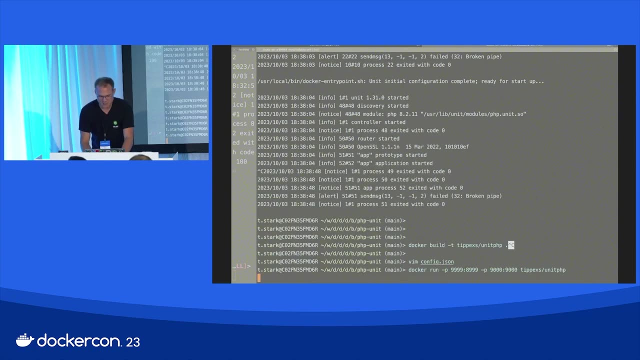 So this is very important. So we do unit share unit and then one, two, three. This directory does not exist, But this is a runtime thing. It's not on build time, it's on runtime, So docker will just build the container, fine. 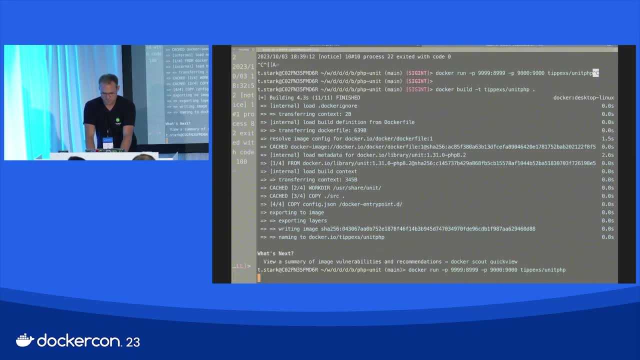 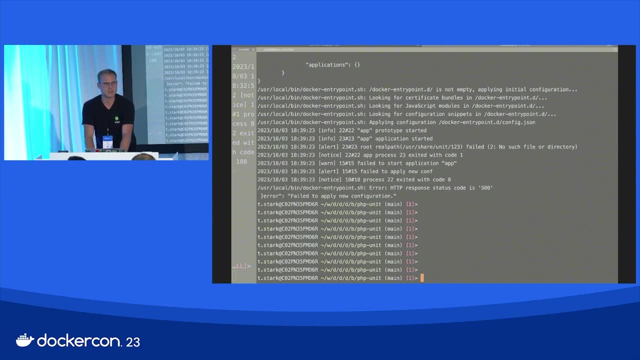 And then when we run it, So Okay, Okay, Okay, So it will say: HTTP response code is 500, and see, It's gone, It's not even started. So how do you find now the problem? Now we define an alternative entry point and say: you know what? 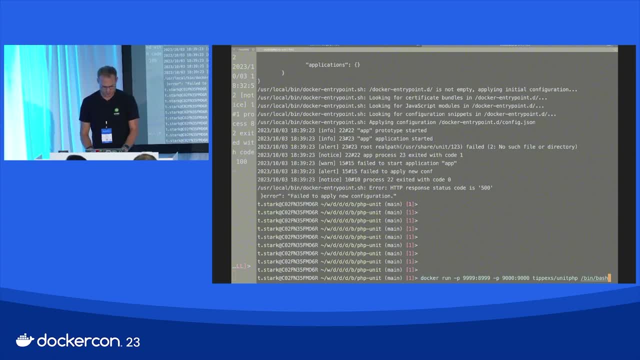 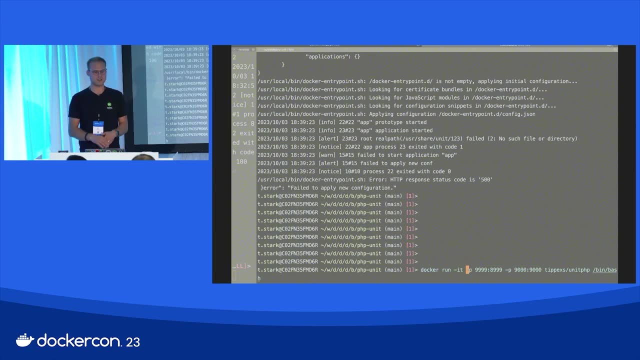 Do not start unit, but just give me an interactive thing which has been bash, and then you have to put dash IT in front of it to have this interactive TDI Enter and we're in the container Because bash is there so it can start. 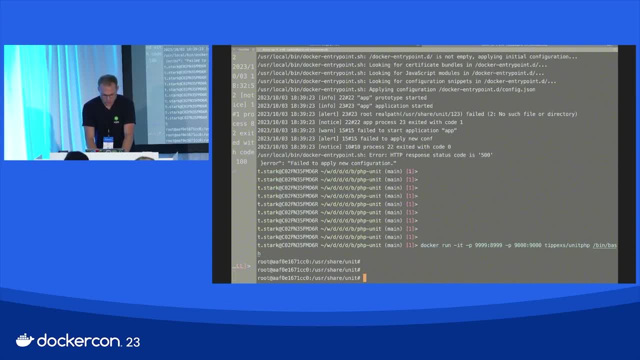 Okay. so now when we look into, okay, where's our configuration file, It was inside of Docker. what was it? Entry point D: oh, there's a config JSON. Okay, fine, there's the config, it's in. 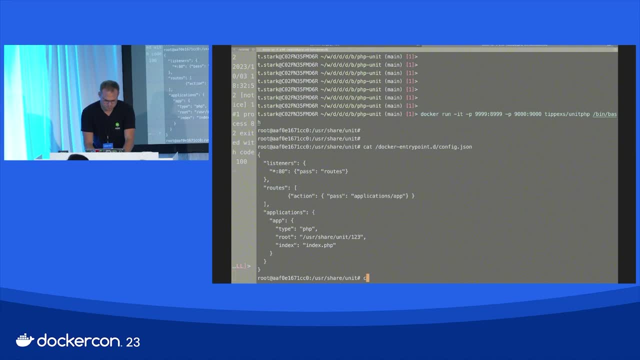 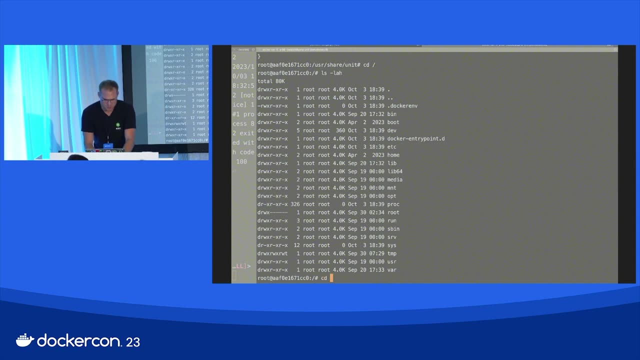 And then we must look into the base image, what it's actually doing. and it's normally running this Docker entry point SH script. Okay, no matter where that is, it is somewhere. Somewhere is a Docker SH script and that runs the configuration that is in here. 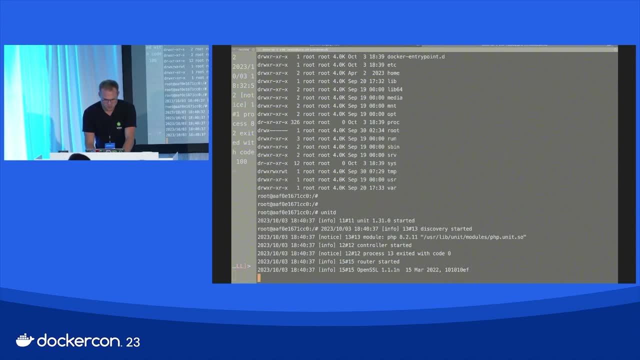 So that means when we do unit D. so that starts up just fine, right. And now, if we then try to apply the configuration, we will see the same error. but then we will see, hey, there is the wrong user. share unit. 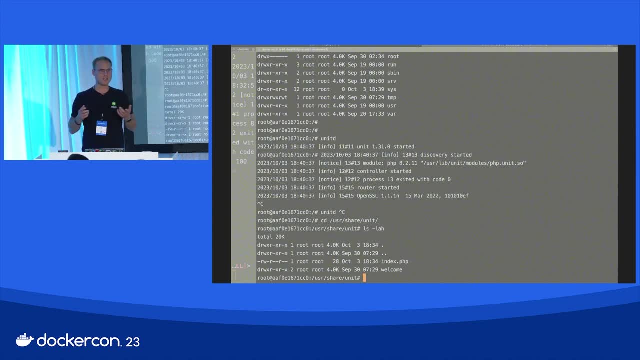 Oh, it's without source, it's just an index. Okay, right, So we can go in the container see why is it failing and then see, okay, it's in. user share unit is the thing, and there's the index PHP. 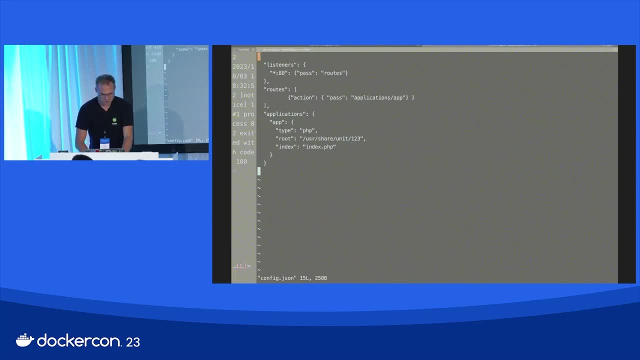 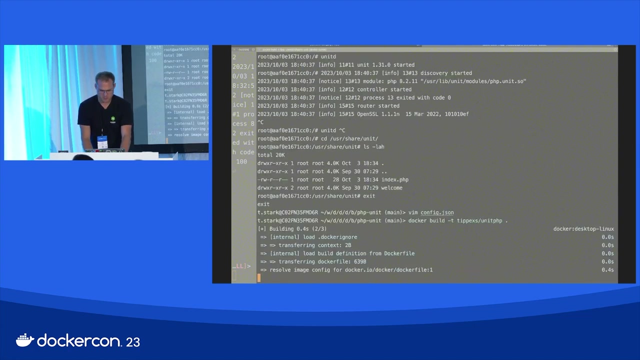 Okay, let's see. Okay, it's just user share unit without anything else, And in this we have the one, two, we have the index. Let's try this. Let's build it again, run it again and it works. 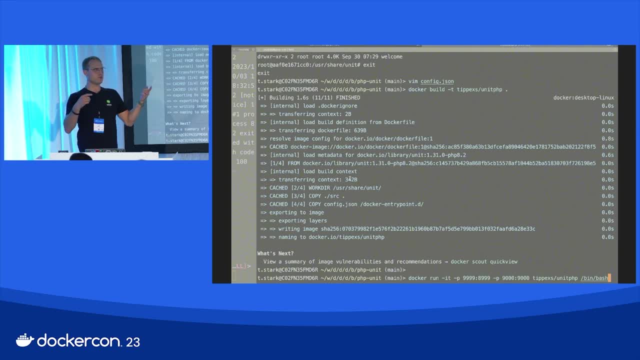 So this trick here is very neat when you have a problem in your created image and it's not even starting up but you have to debug why is it failing, Just bashing in. do this stuff manually and see why. And especially handy when you do copy commands. 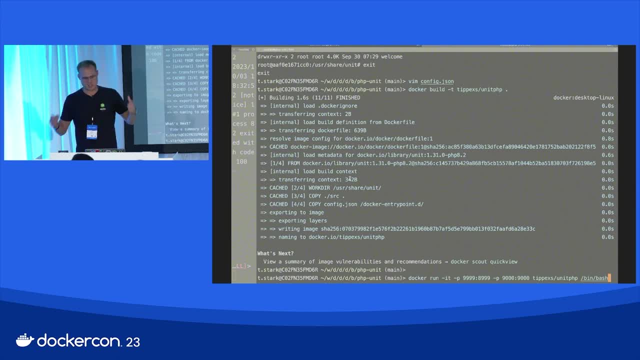 copy files from somewhere into your container and it's not working because of some reasons, And most of the time it's literally something like this: You copy source from to something and there's a slash in your Docker file so that you're not copying the whole directory. 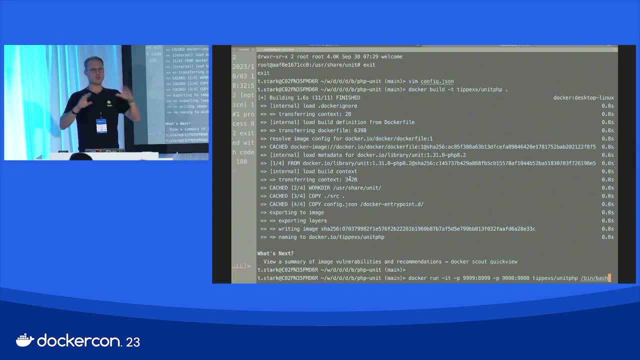 but just the files and that it's not starting. Don't bang your head against the wall Just doing bin bash. go inside, check. if it's there, fix it Easy, Not a big problem. All right, let's start this up again. 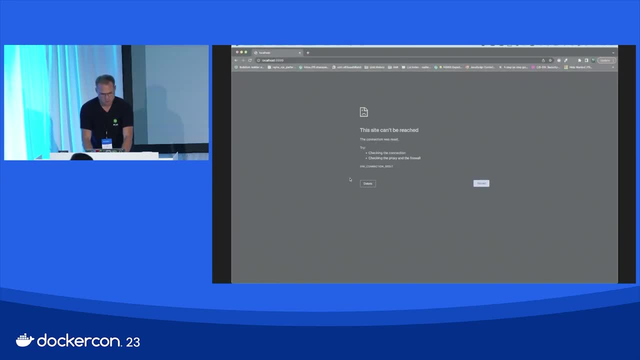 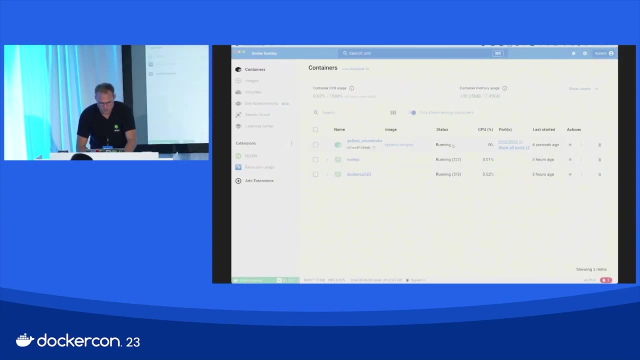 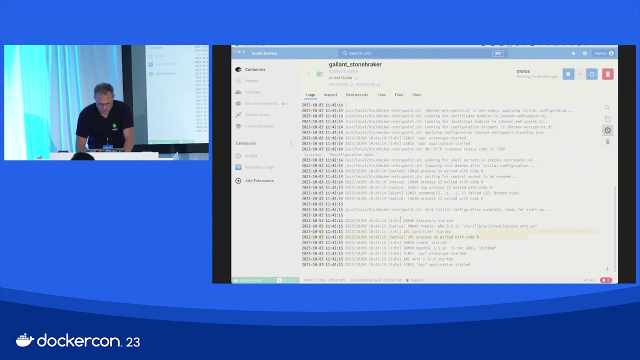 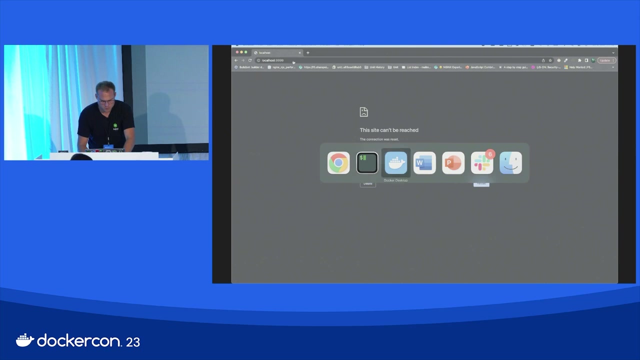 Start it, Perfect, Perfect. And now let me see. Now let's see what did we do to do in containers. App started, Initial configuration is complete, So we have config. port 80 goes to routes. routes goes to app. 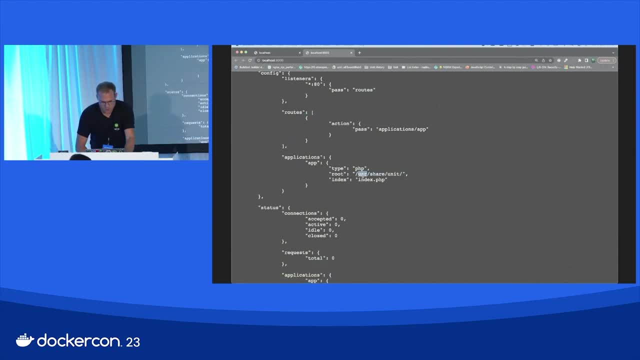 and app is doing type in type php, user share unit, and then we do have index php. Why is it saying connection reset? Okay, that is important. That's interesting. That's the demo gods They're leaving us. 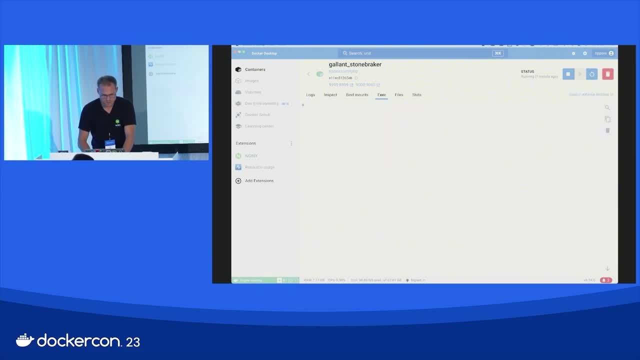 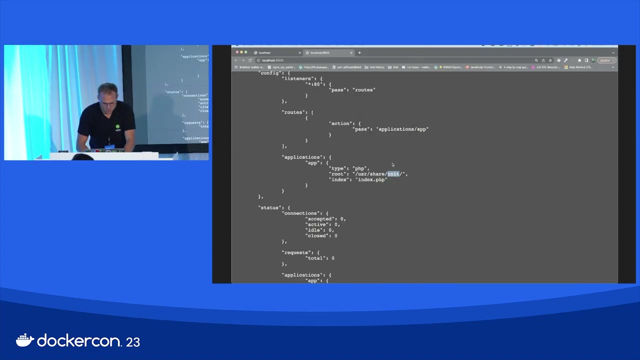 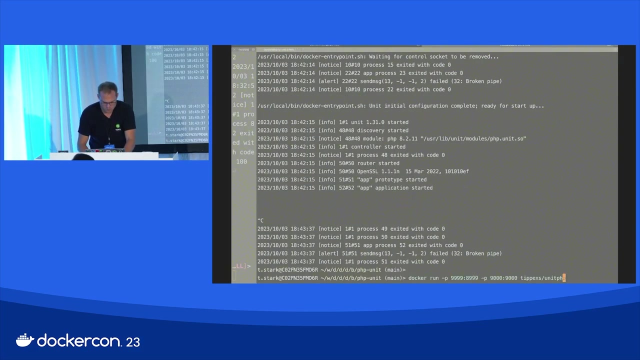 User share. Well, I'll fix it real quick: User share. So we've got this, We've got the indexingphp And that is indexphp, which should work, And we're gonna do over here, we're gonna do, do run. 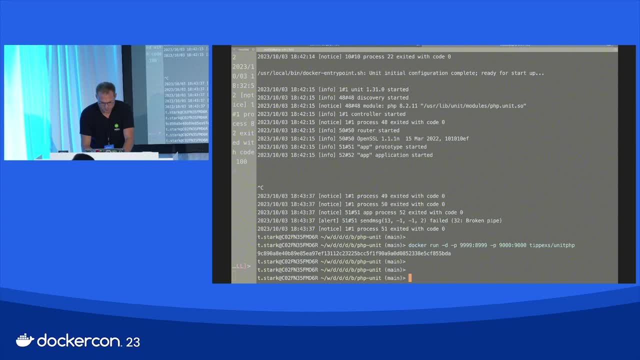 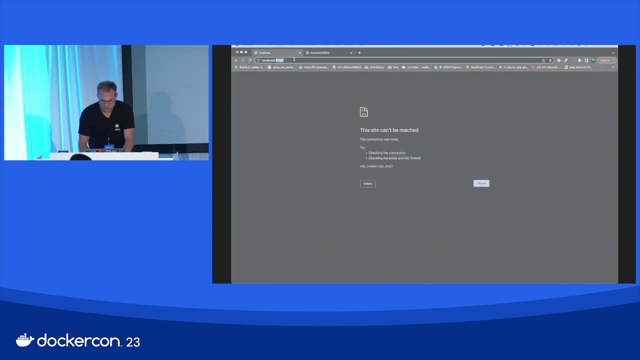 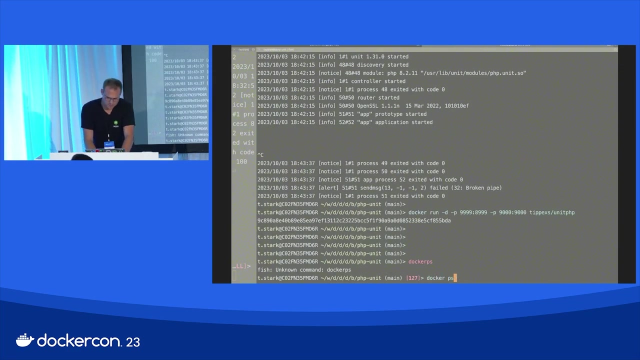 p run, let's do background, do run, let's do background, and then we have a deep ID, and so let's do run and then let's do do run. This is actually the most important part for me for the demo, and that is not working. 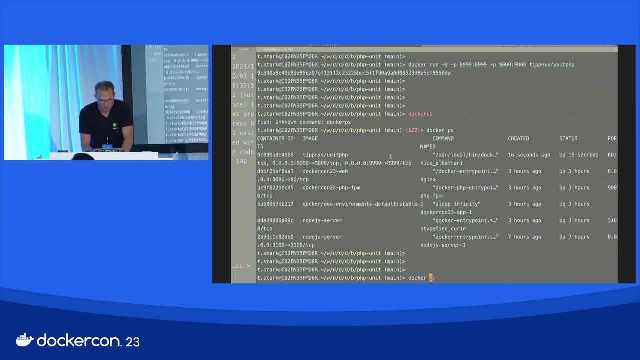 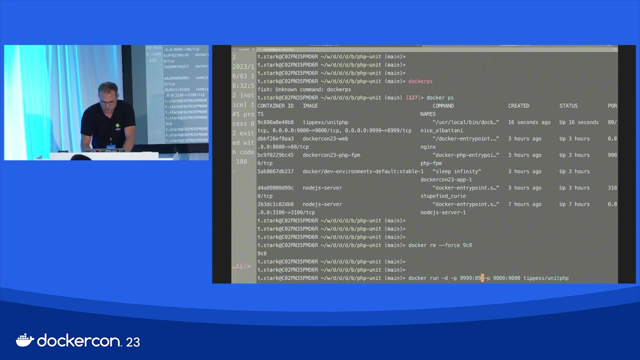 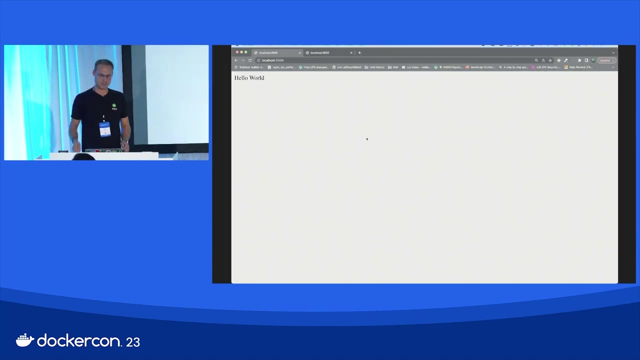 Oh Jesus, I'm using the wrong port. See, It was 80 and not 9C8.. Yes, We should use a. It's like: yeah, technology is amazing. If the TCP can connect to the port that actually is open, then it simply works. 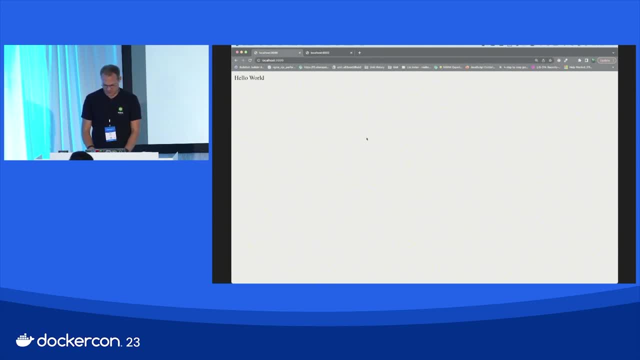 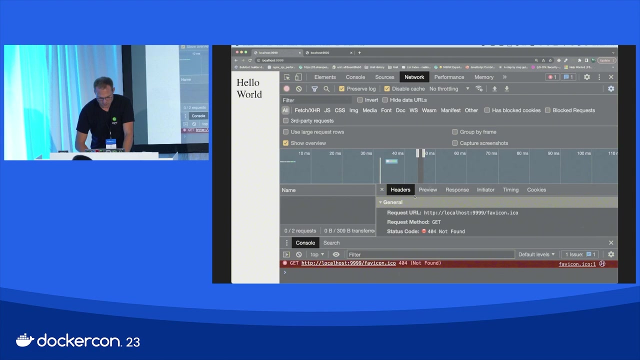 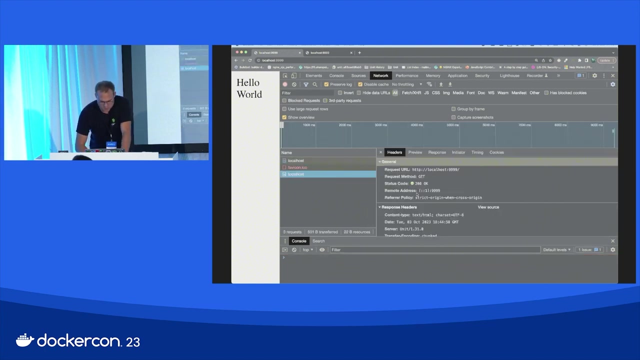 I mean that's amazing, Great. So we see Hello World, which now comes from PHP Network reload, Okay, Localhost. It's actually hard to see when it's like zoomed in like this: It says unit 131.0 and we have PHP 8.2.11.. 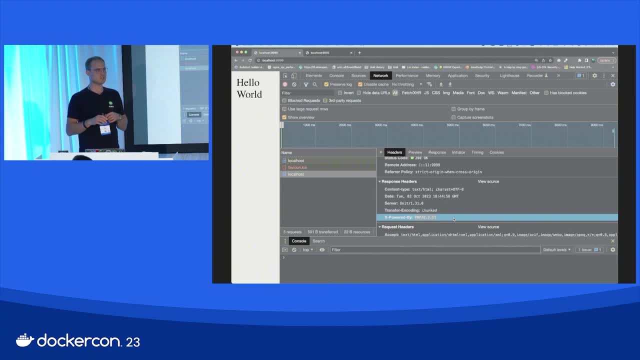 And that's all you have to do. No more PHP juggling stuff. It's unit as the base image, the JSON file and that's it right. So now we can fix this favicon thing, because that's always annoying. It says favicon is not working. 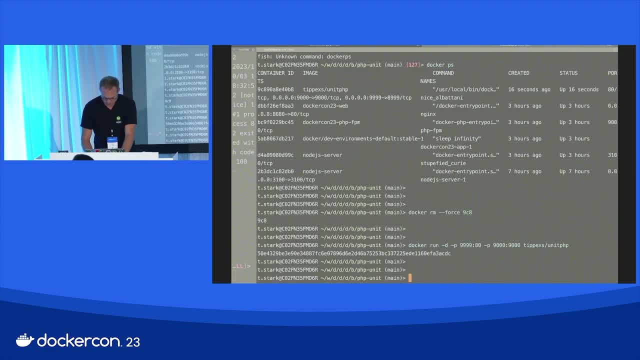 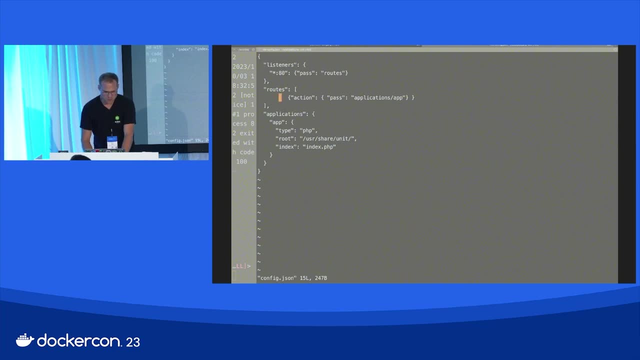 Okay, It's not working. So if we define, If we reconfigure unit on the fly and we define a config JSON in the router, let me see if I can do this on the fly. actually We do match, match, match and then we want match of URI. 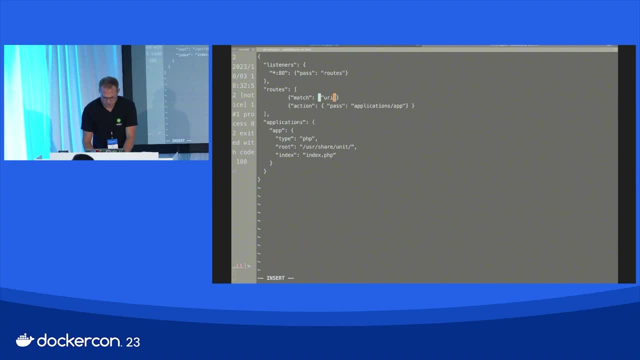 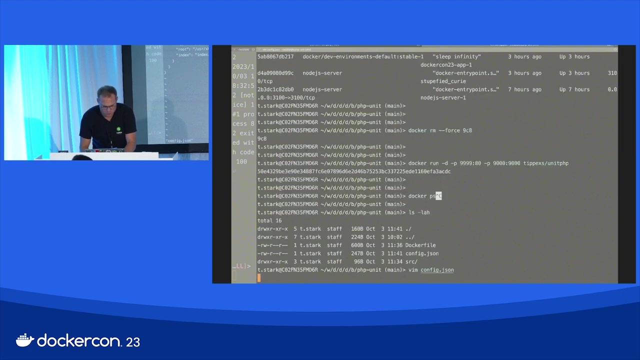 Okay, All right, All right, All right. So object is faviconico, isn't it? Yup Right, If the URI is faviconURI, then we would like to invoke an action that says return 200.. And then we do the action. 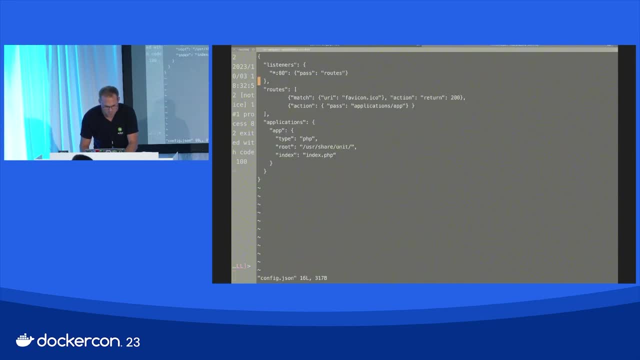 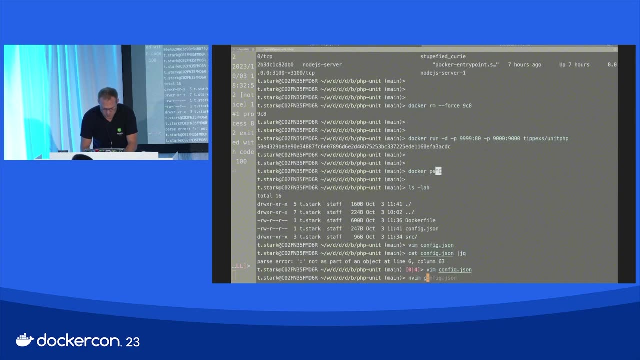 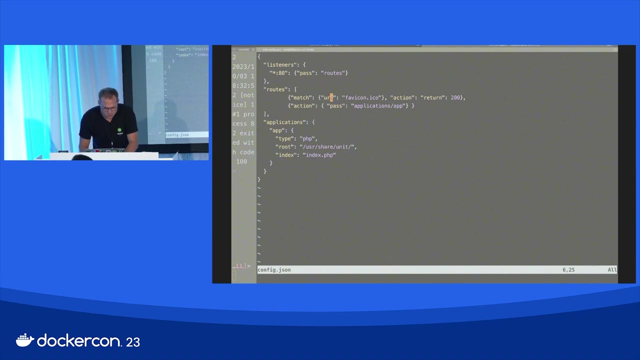 config in jq. again, we have match is URI. we use nvim, nvim config match URI, match, no, we have match and then action that should be an object and then we return. see, that's. 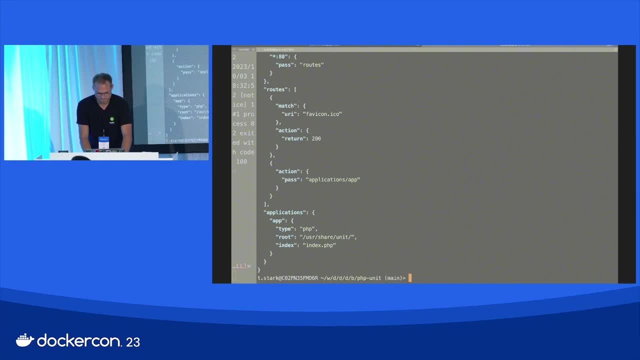 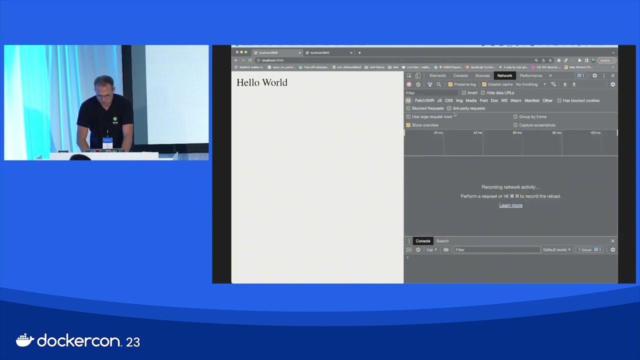 why I'm normally using the CLI, because writing serialized code is not nice. okay, so now we do the curl thing with ketting and stuff and put that in reconfiguration. done, amazing, delete it. Okay, disable cache- where is it? where is disable cache? can't even see when it's like. 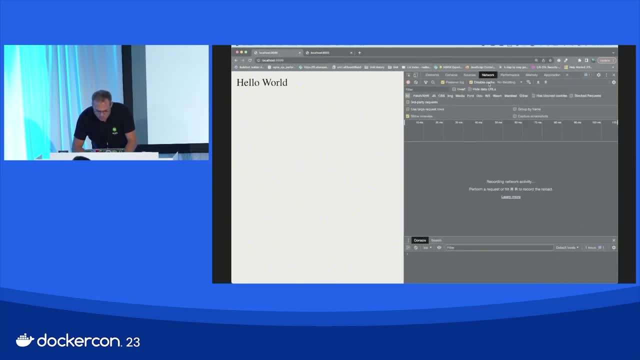 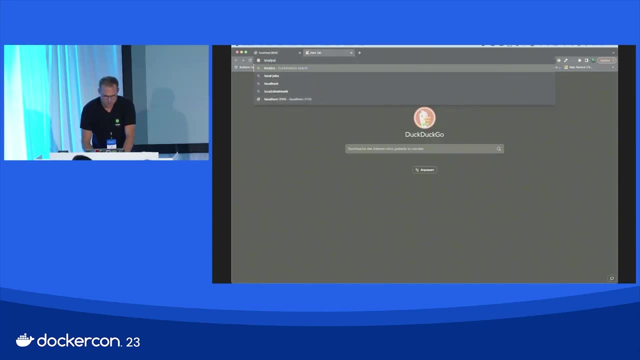 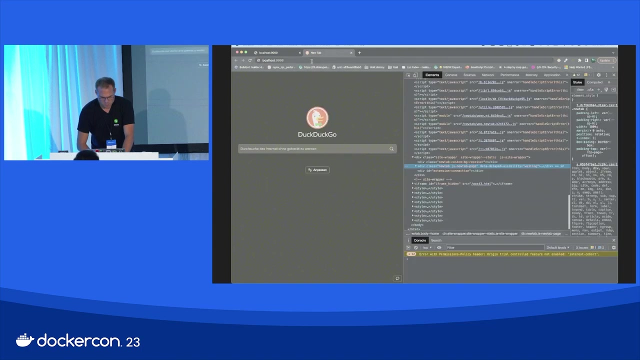 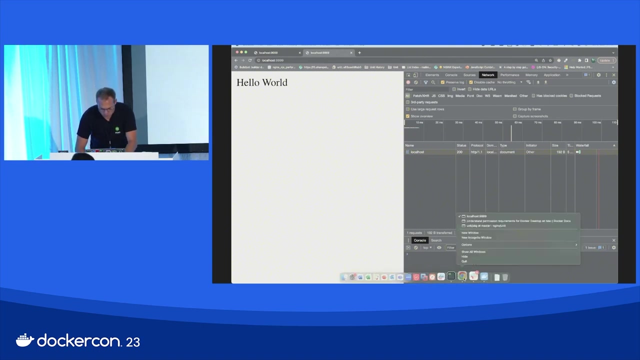 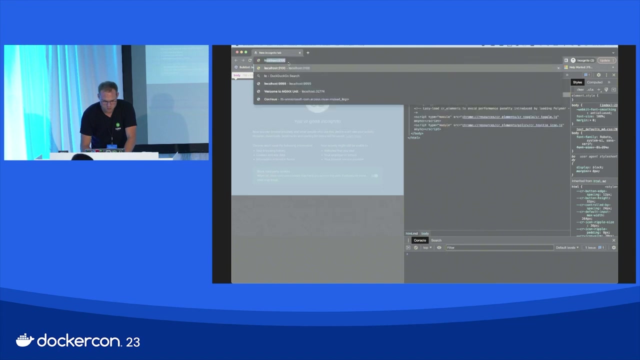 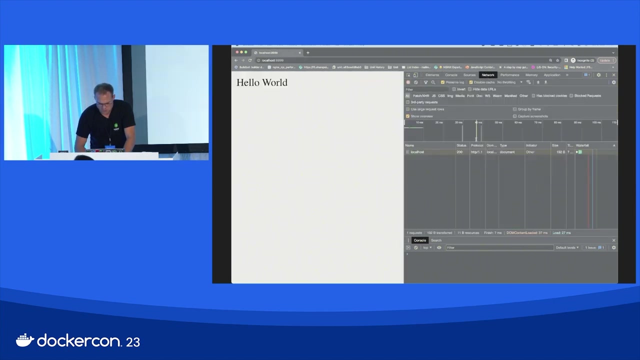 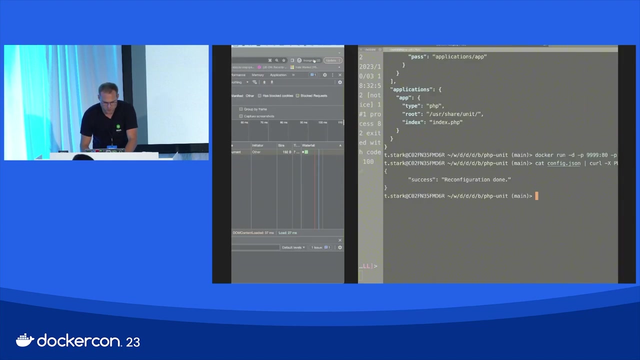 this: ah, disable cache. there you go. why is it not using favicon anymore? hello, there you go. all right in cognitive mode. if this is not working, I will use curl. curl will do it always. localhost, 999, network send it. okay, we'll use curl then, so we. 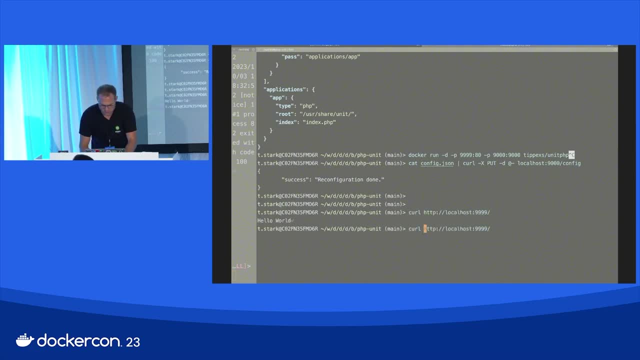 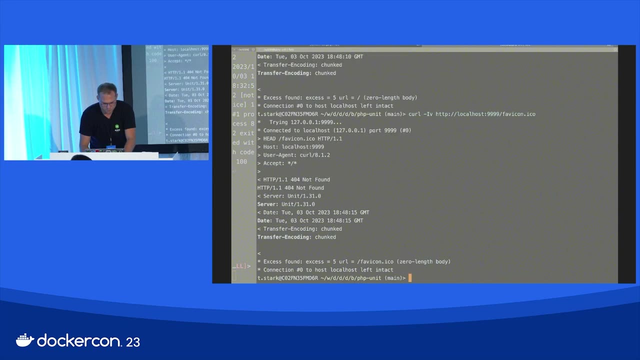 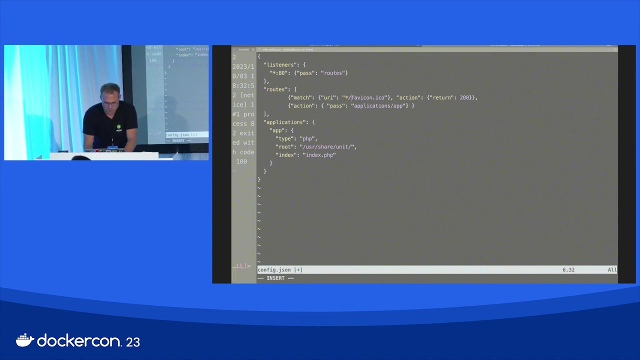 now do curl says hello world, fine, It's 200, and now when we do faviconico, still prints 404.0.0,. amazing, Okay, so that means the match here is somehow not correct, Is that right? 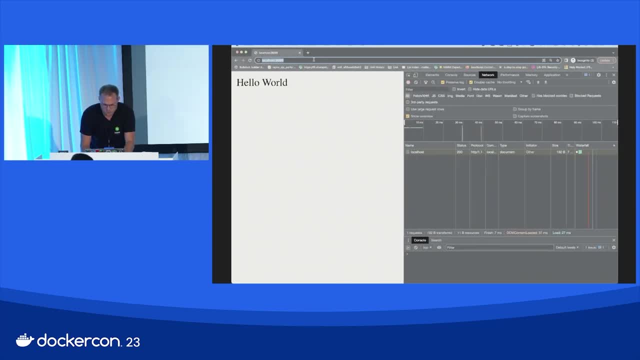 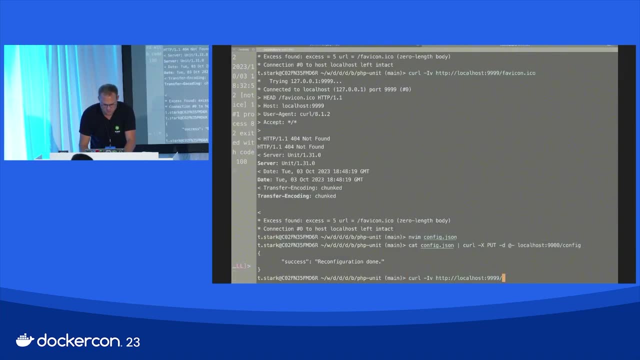 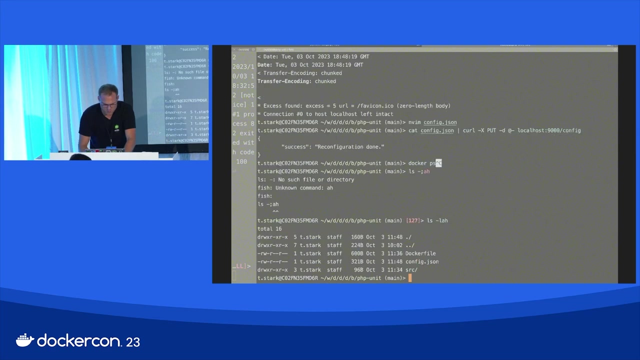 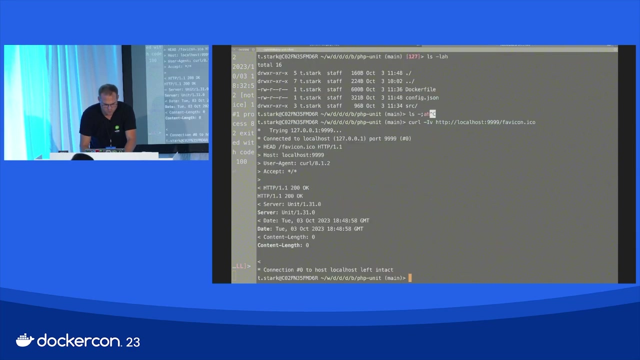 faviconico: Last test. if this is not working, then I'm not sure if it's part of the URI or if it's part of the. it's actually not an argument, I think. favicon okay, that works Good. so now it's giving 200, okay. 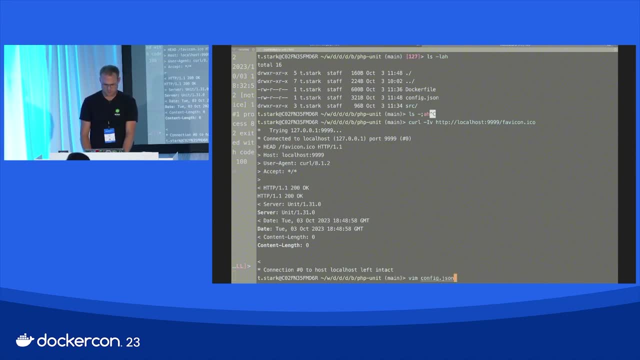 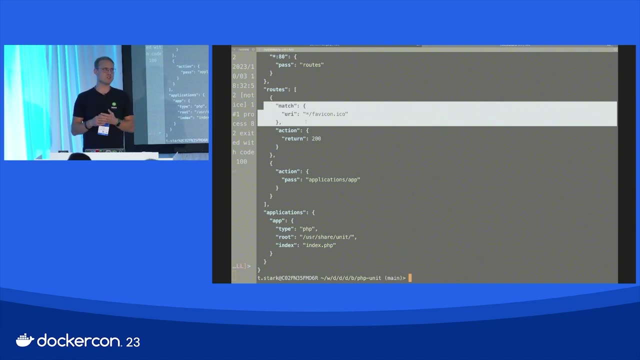 So that's the interesting stuff you can do with the yeah, With the unit router, you can simply say, okay, do it. That's why I love nginx-unit to do stuff like this, because it becomes part of your application. 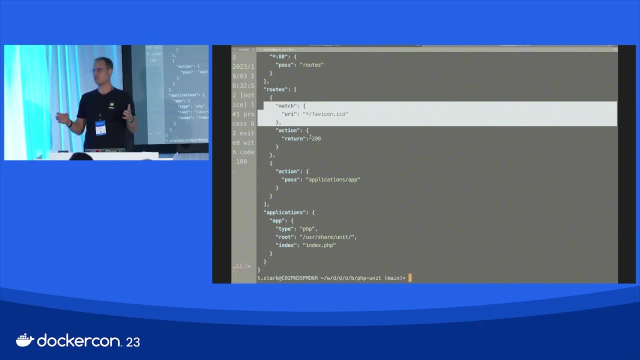 And this is pretty simple and pretty easy, but you can do the same thing for very complex things as well, And we have on the website we have documentation about using Laravel or KPHP and how to configure it. probably, and probably, that's great cool. 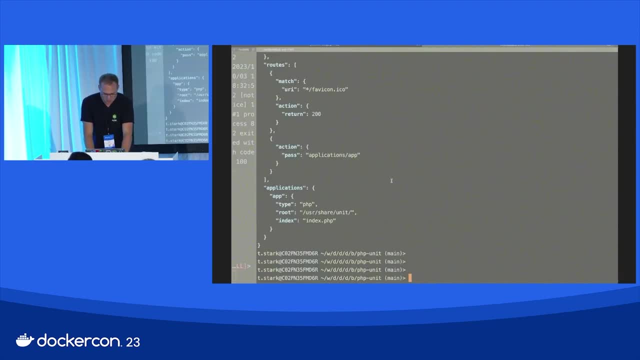 So it's like 10 minutes to go. Good, so we have now created a PHP API very simple, using nginx-unit. We have a Nodejs API which uses Express, And we have a bunch of Docker containers right now. 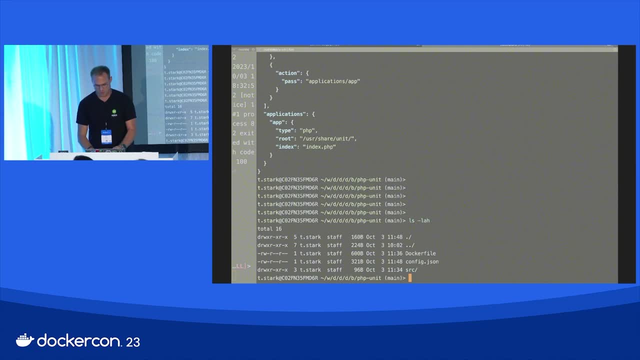 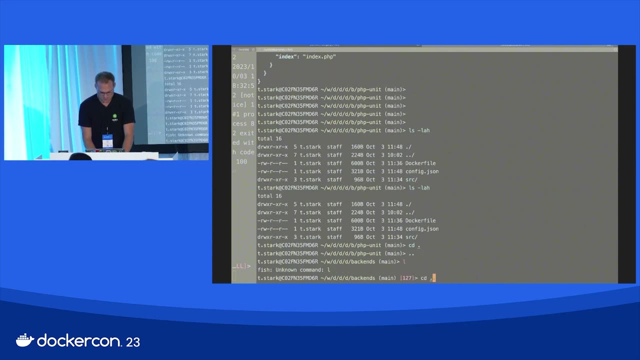 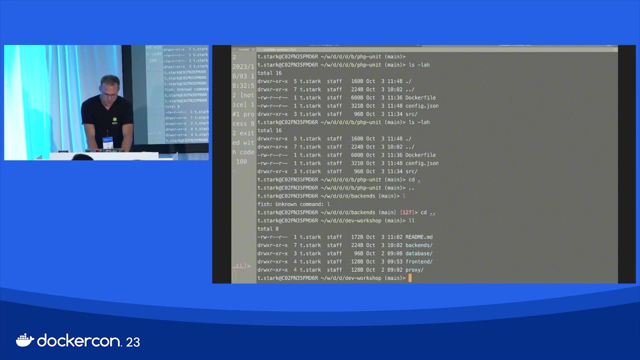 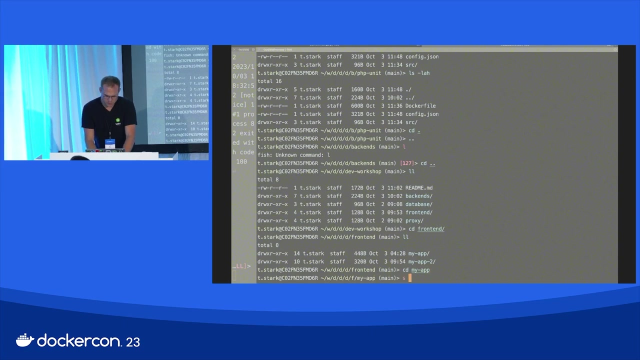 We have one for the Nodejs API, We have one for the PHP API And we have one for the PHP API. And, yes, that works, that works, that works. We have the front end. All right, so, and the front end is now something. 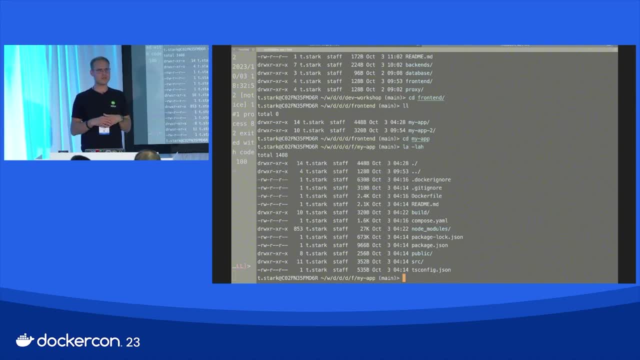 that's something usually you build as static files, right? You use HTML for that, and then you need a web server. You can run this on nginx-unit as well, if you want, or you dump it in nginx with this configuration using the try files command, right. 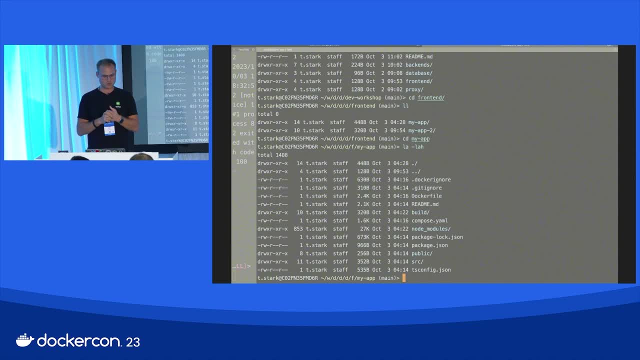 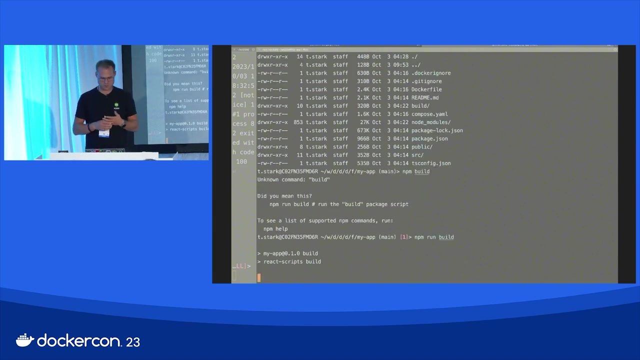 That's special for React. if you have a React router, then you have to use try files And then you can do npm build here, for example, And then it just builds your React application. Oops, that's a script, Good right, so? and then you have to build output. 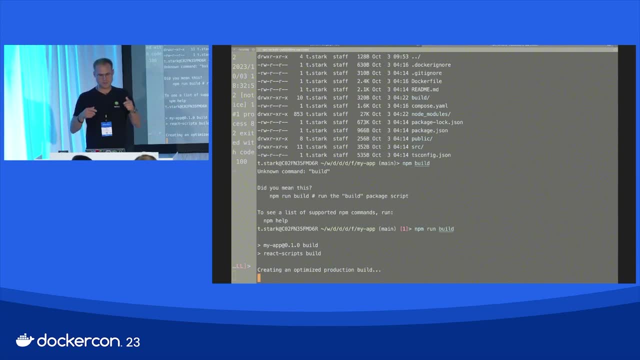 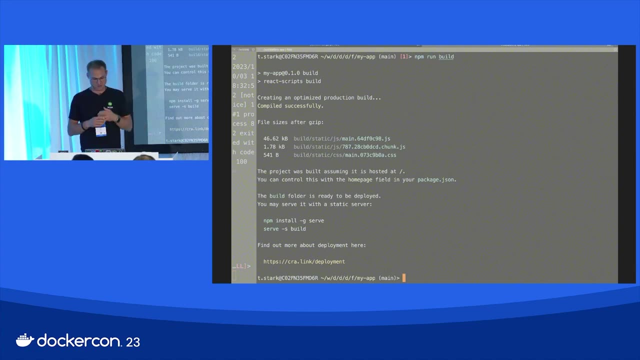 and then you will have- you can copy the build into another container. So now- and we have just 10 minutes left and I really would like to cover at least a couple of more things- We have Docker Compose Watch. I completely missed right now. 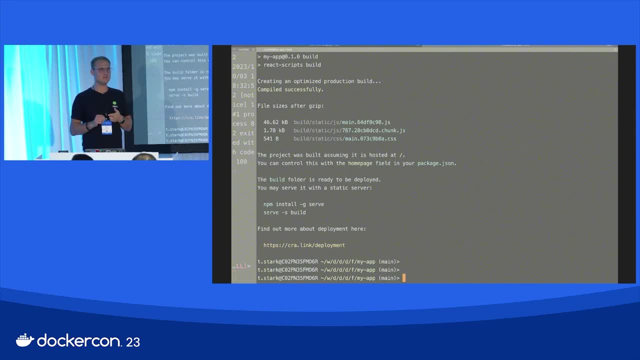 which is a bummer, and we have multi-stage build. Is there anything you're interested right now that we do the next 10 minutes? Docker stage multi-stage build or Docker Compose Watch? Docker Compose Watch is something new. 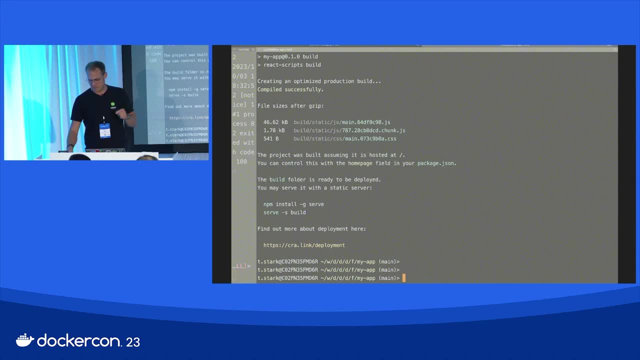 Watch, watch. okay, now let's do watch In Docker Compose Build. I make a promise in my notes I will put it in this PDF document how multi-stage build work and how you can use it to have, like a build, a local build pipeline. 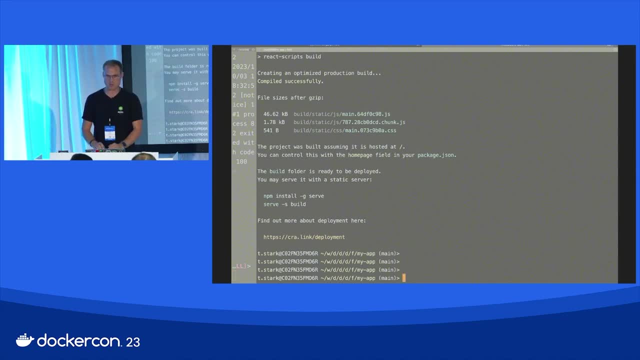 a mini pipeline on your computer, laptop, just to use it with multi-stage build promise, Because what you can do is one word. you can use node as a base image for this React application, then copy everything from the source directory in the node thing, set it in the Docker file as a build. 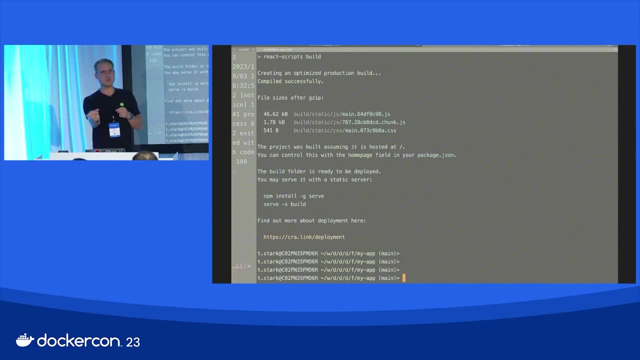 then run npm build and just copy the build output in an nginx container and then that's it. But you don't have to have node on your system to build your application. So if you pull down and type Docker, Compose, Build, it will just build your project. 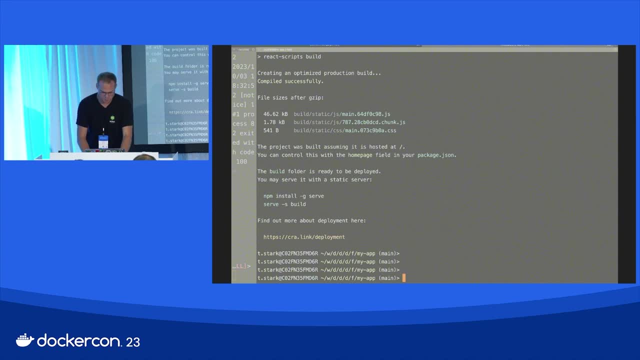 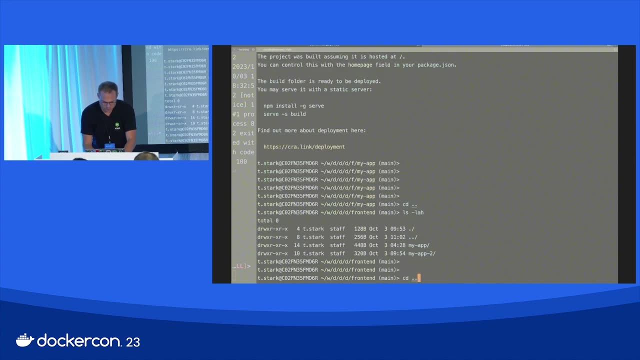 and you don't have to have node on your system. okay, That's why multi-stage builds are always super, super important. But let's do Docker Compose Watch real quick. So Docker Compose Watch, And I have actually a slide for that. 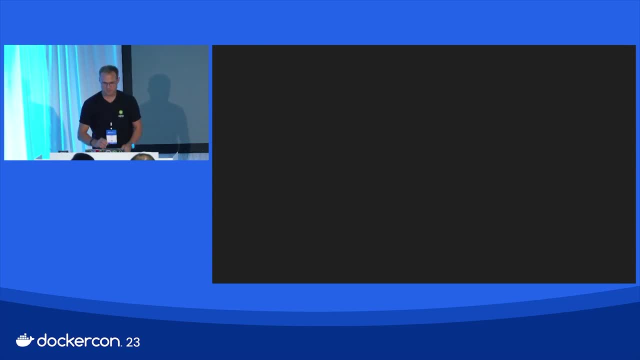 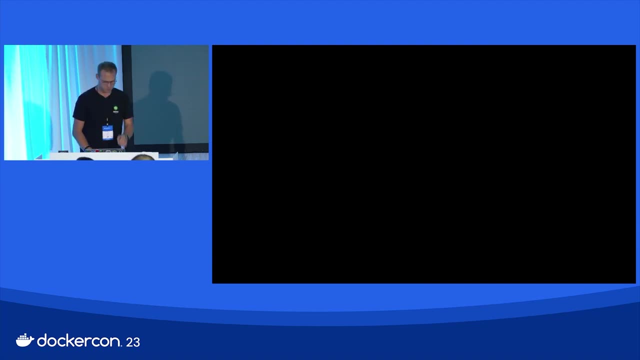 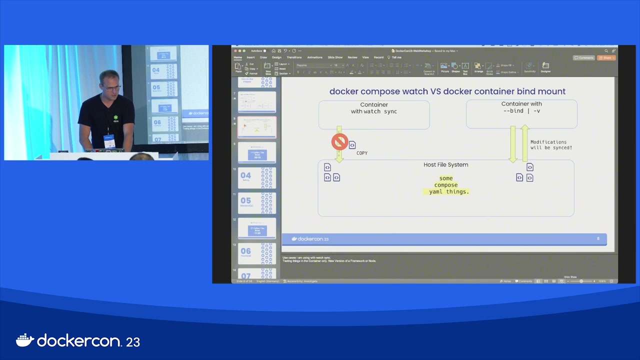 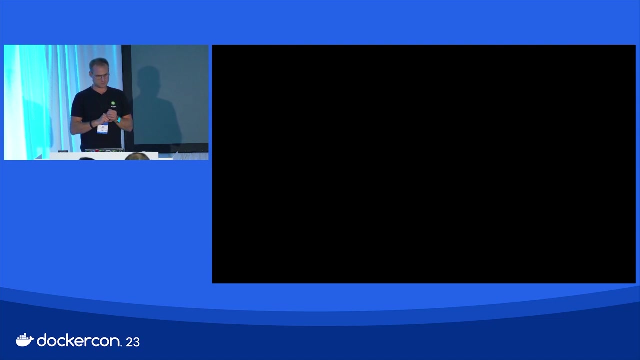 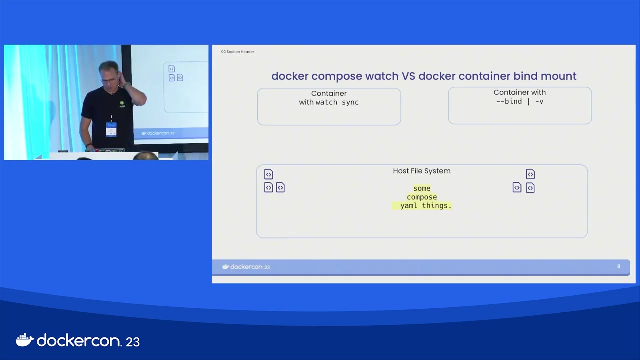 So excellent, excellent choice. So what is Docker Compose Watch versus the bind mount? we already okay, That's too fast, I have to do it slower. Okay, wait, okay again. Nope, Let's see. Yes, perfect, okay. 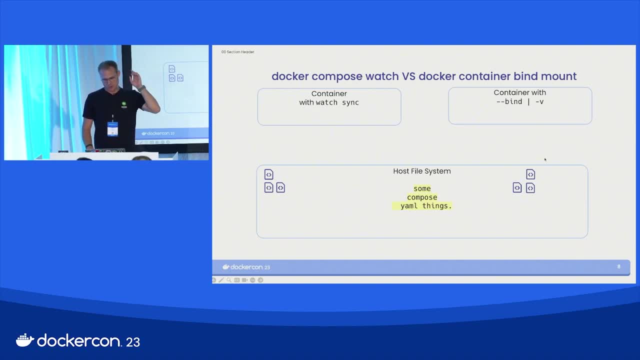 What is Docker Compose Watch? Docker Compose Watch has two different modes. One is sync and the other one is build. So what it does is basically on sync mode is it will detect local file changes from a given file. 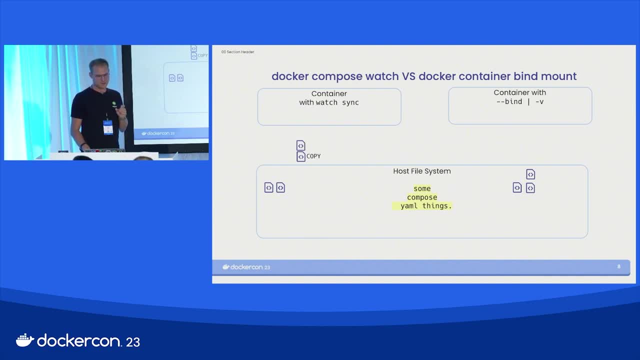 and then it will create a physical copy of that file and sends the physical copy of that file into the container. So it will not use the files you have on your system, it will copy them into the container. That is handy because if you do stuff in the container, 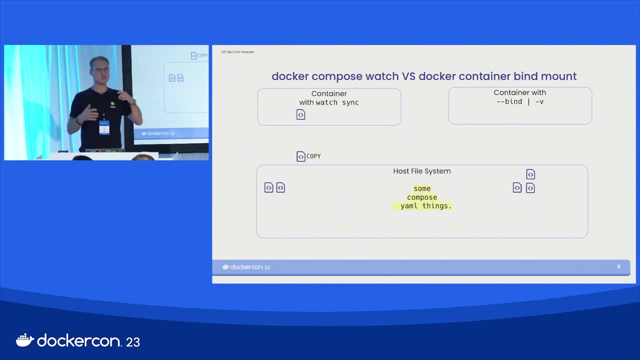 then with Docker exec, because you would like to try something different with node modules or whatever. it will not never copy stuff back to your system, Never, never, ever So, and this is the problem with the bind mounts: If you, if you mine, or bound like mount, 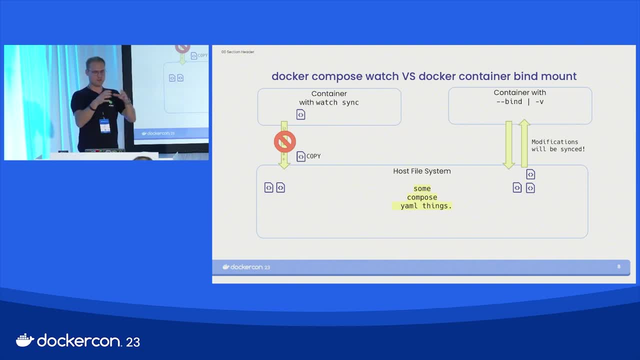 like a directory from your computer software, like laptop, whatever- into a container and you do something in the container, it will automatically sync between your client and the container And this sometimes is very, very dangerous, For example, if you have a caching folder. 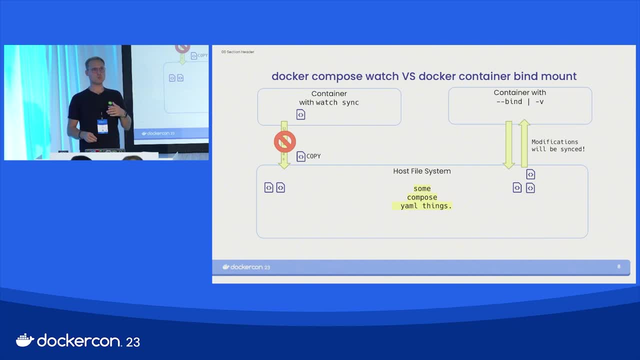 you have a node version 25.1 on your system and you're launching it with 25.3 because you would like to do some testings. and then you run npm install in your container. it will override what's ever on your node modules folder locally. 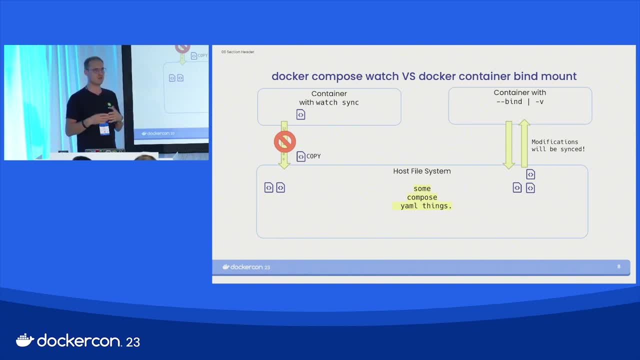 on your machine. That results in a non-working thing, maybe. So that's why Bind mount will be synced Always, Ever, Because it's not a copy. It's like a physical mount of files in your container. With Docker Compose Watch, it will create a physical copy of that file. 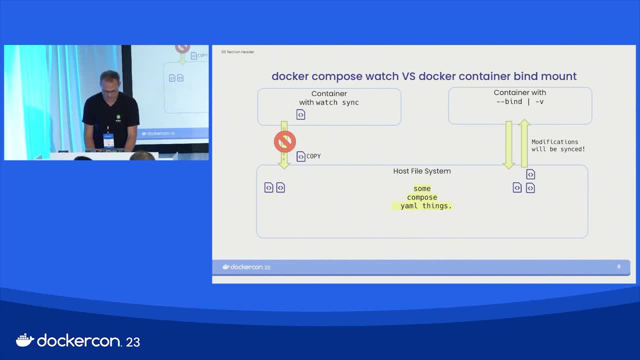 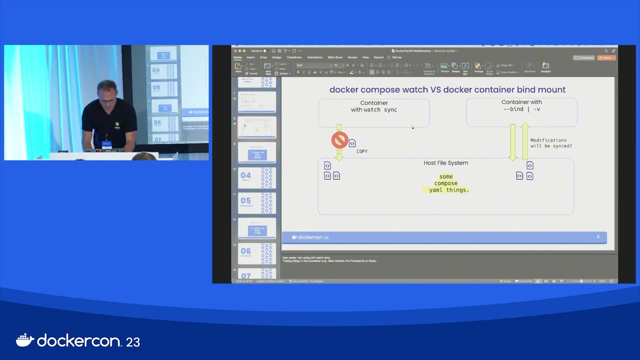 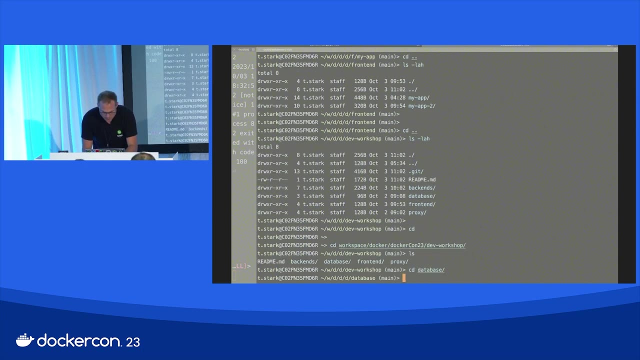 send it to the container so it will never sync back. So let's have a look how that looks like actually in production Or on the command line. Let's see. Yes, Good, Alright, So in workspace Docker web workshop in backends. 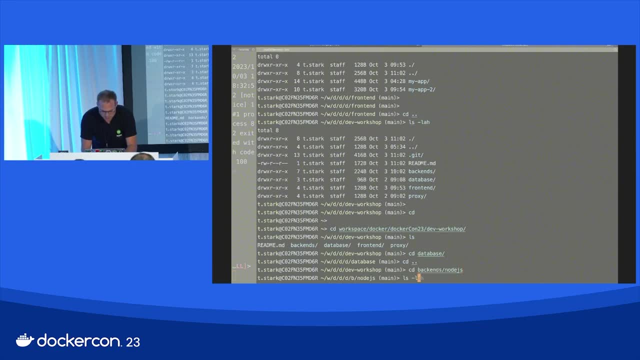 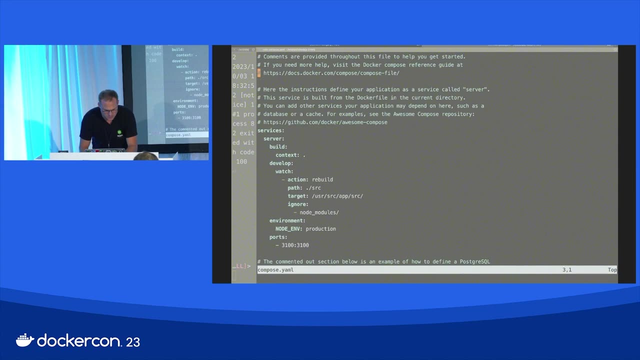 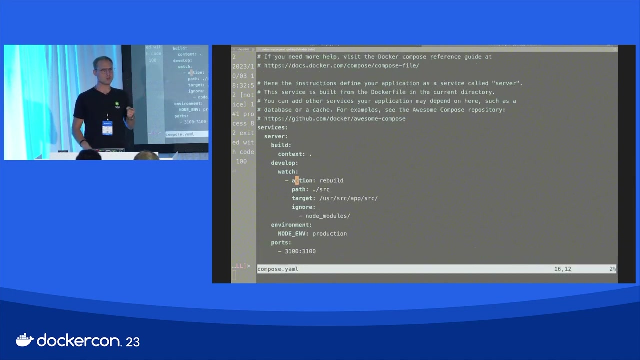 nodejs: vim docker compose, watch, Let me see. And vim compose: Yes, So you can use, develop and watch. and then we have action, And the action can either be- let me make this a little bit bigger- The action can either be rebuild or sync. 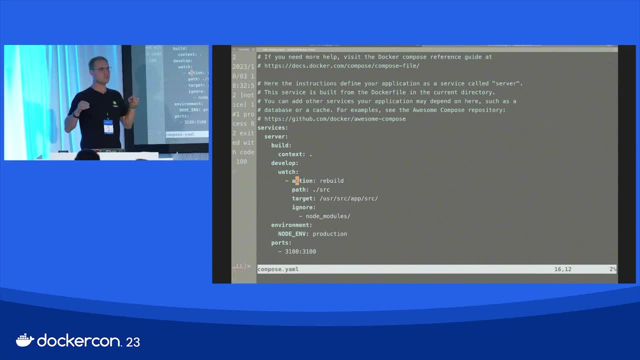 Sync will just copy the data, not rebuild the container. So if you just want to copy data for PHP, for example, you don't have to hot reload or build the image, because PHP will read the file, interpret the file, send the output- For nodejs, for example. 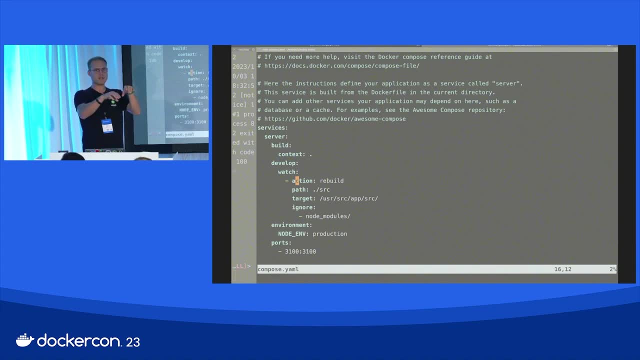 If you already started the container using node fake backend, whatever js hit enter, You cannot modify this appsjs file without reloading the node process because it will not hot reload files from that server. So in this case we define action as rebuild and anything that is in source that goes to user source, app source. 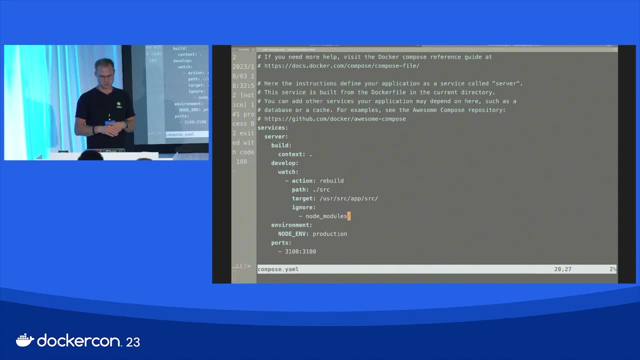 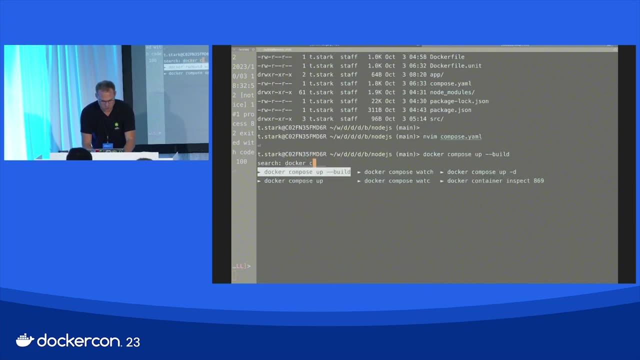 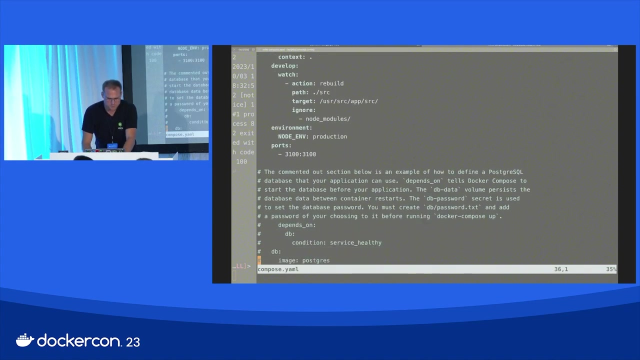 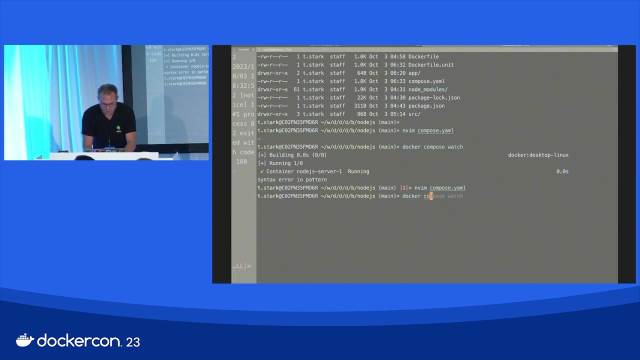 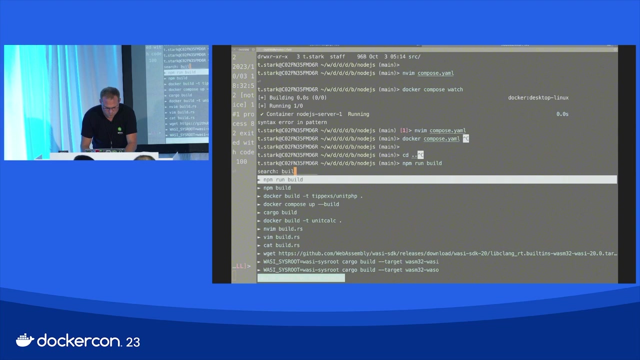 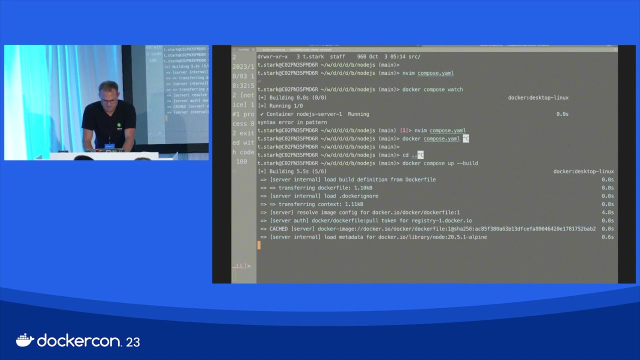 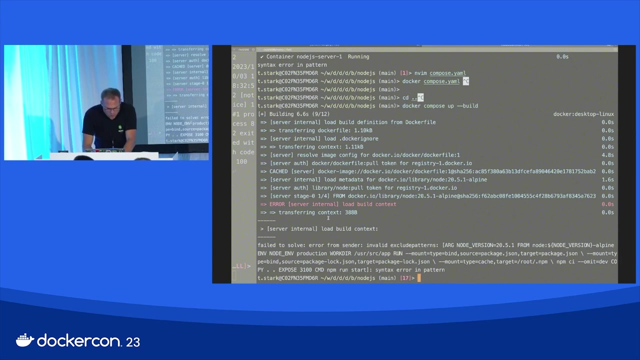 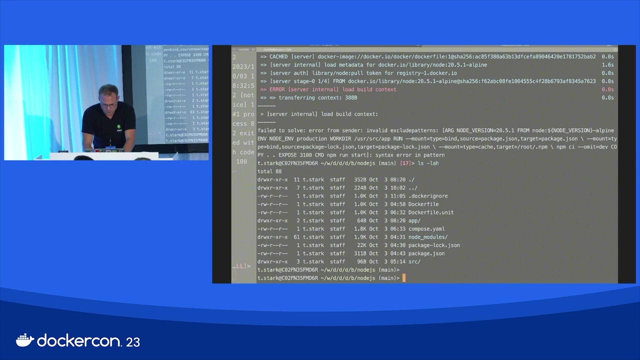 will trigger this rebuild And we will, of course, ignore node modules. So that's how you define it, And now let me show you how that looks like. Then we do docker compose. watch, Did I screw up anything? Then docker compose What is wrong? 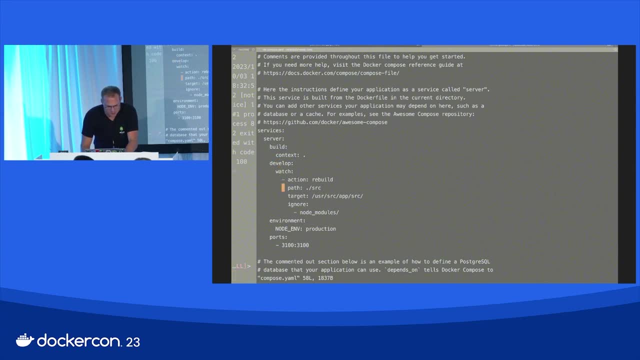 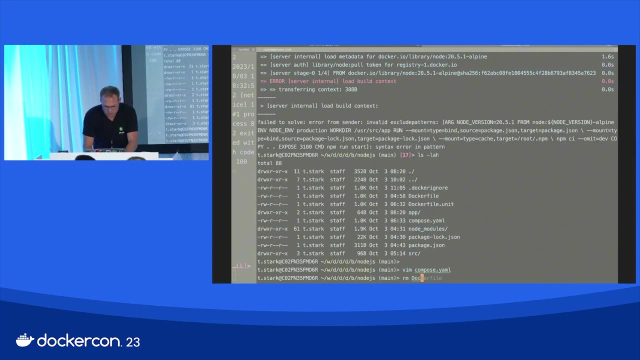 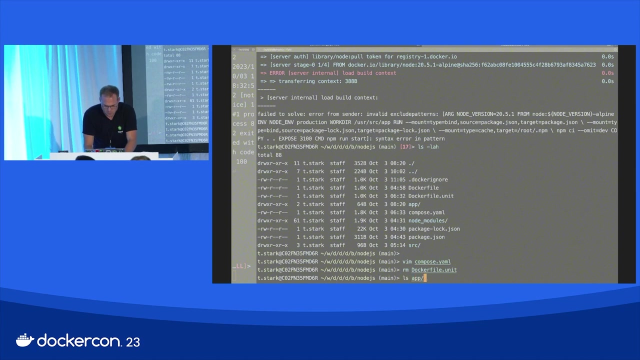 I think I've changed something and now it's not working. That is bad. We have action as rebuild Anything. that's source, it's that target And we build this. Let's remove this. What is in app? Nothing Right. 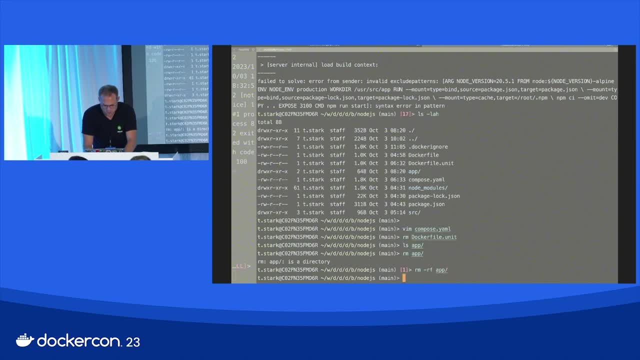 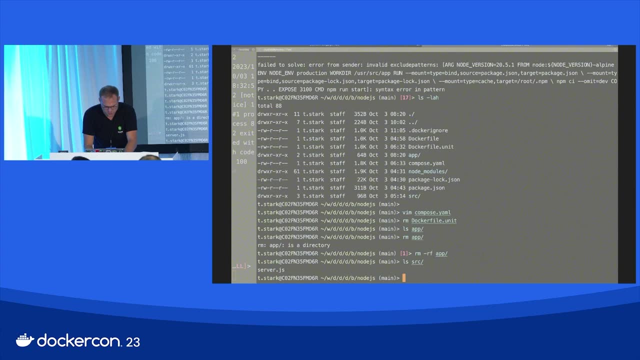 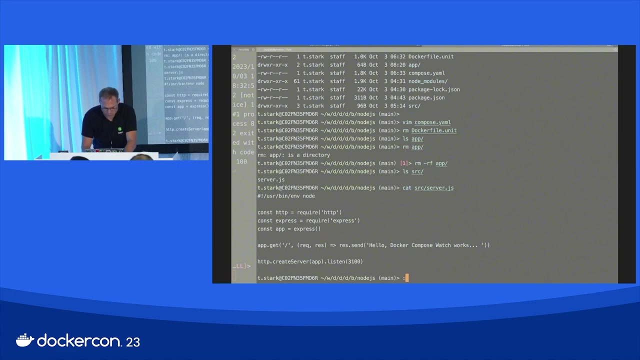 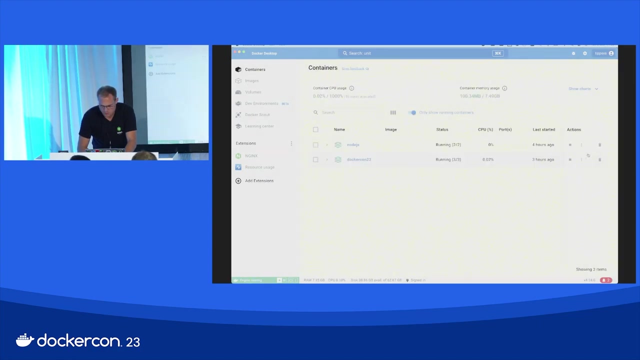 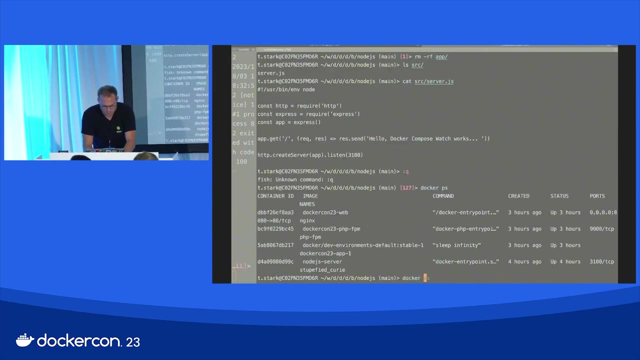 Remove it. Node modules package- docker file. What is in source? Serverjs 3100.. Let me just kill everything really quick. Go away, Nope, No, Just want to make sure we have Okay. Oh, now I can show you my favorite command. 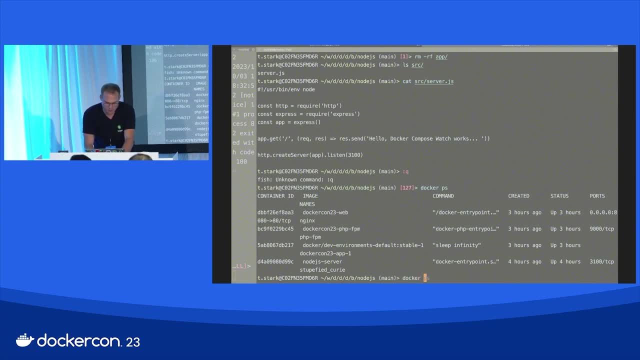 Docker. That's like weekend transaction Docker- rm dash, dash force- I'm just kidding, That's very dangerous. And then type dollar docker, ps dash, q, Enter, And it will literally take just the IDs and send it straight to rm force. 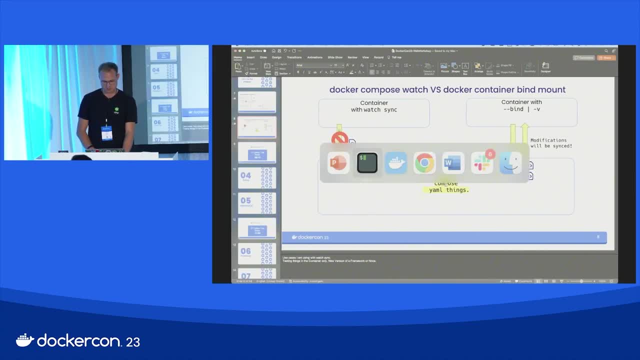 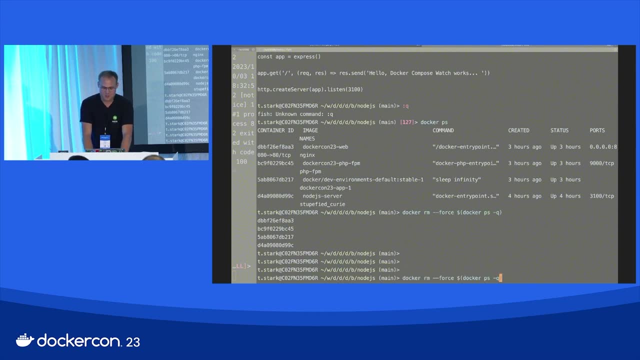 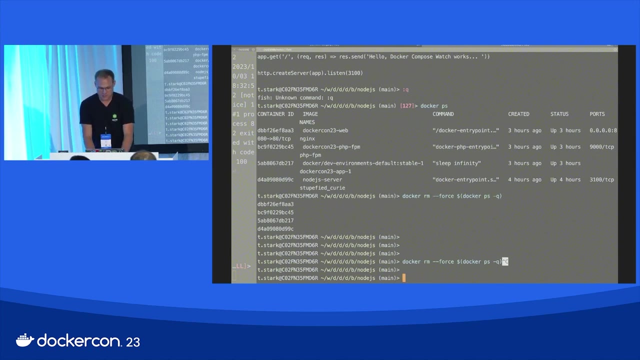 It will delete everything. So now it's clean. See, Blank. Just kidding, Don't do this in So docker. I mean you can do it with a lot of other docker commands as well, But if I'm done with some stuff and I want to clean up my system, docker rm, dash, dash. 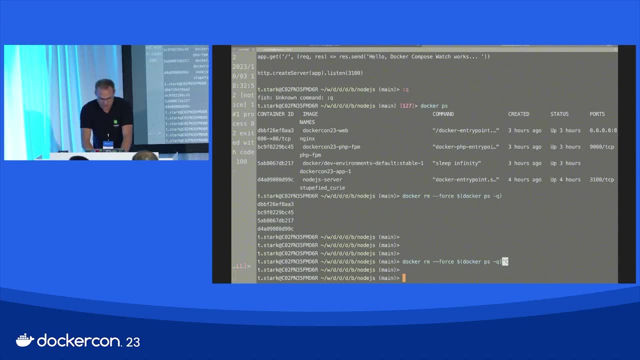 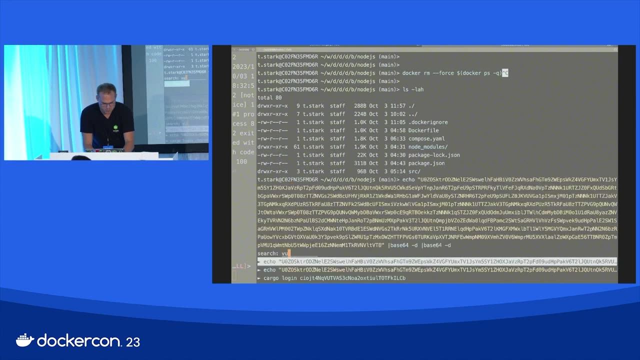 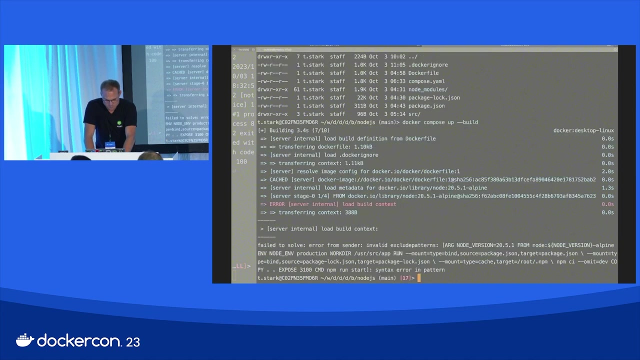 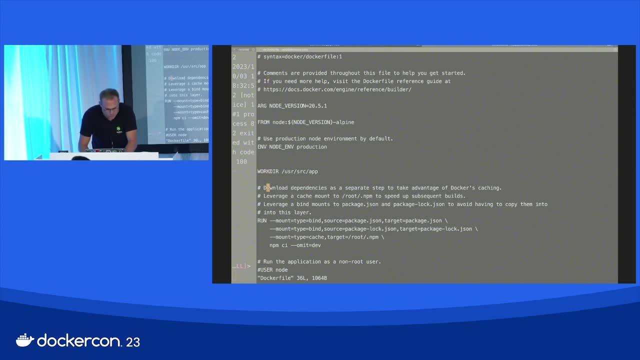 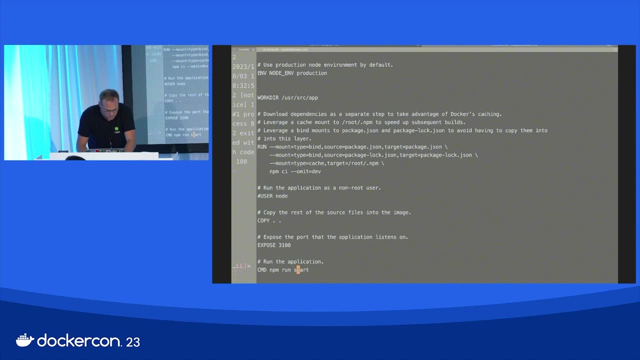 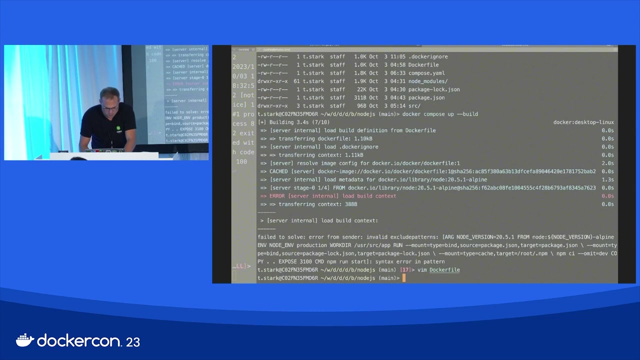 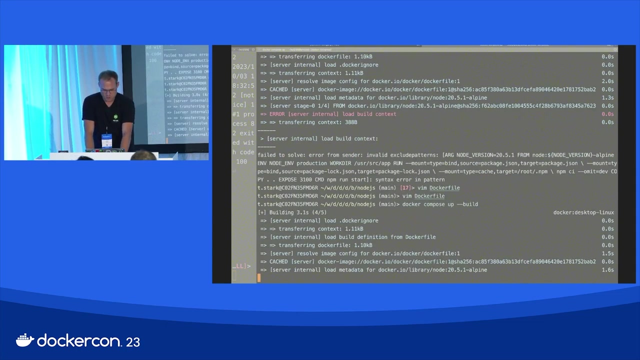 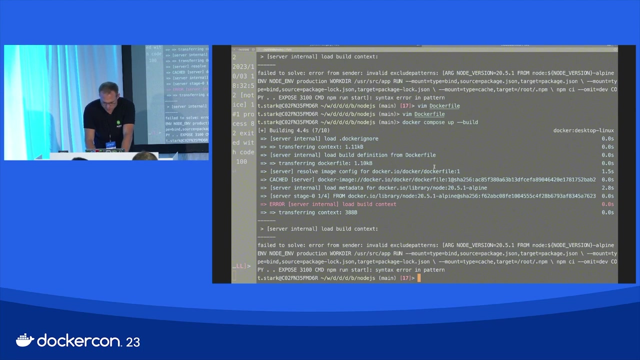 Note version: note version: production run copy: expose npm run start. When did I change this? I've tested it this morning and it worked. I just wrote it back. All right, That works. All right, Server is not internal okay. 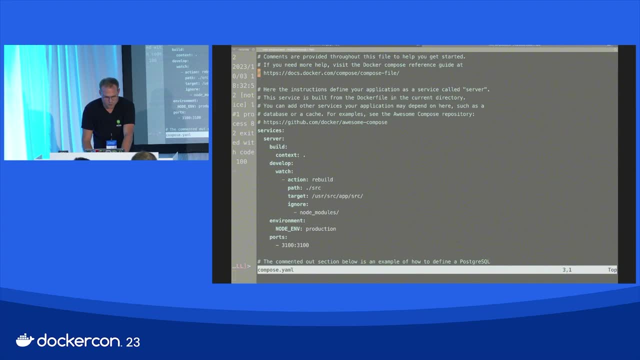 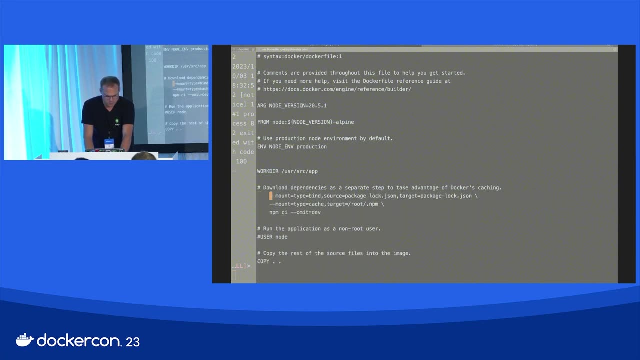 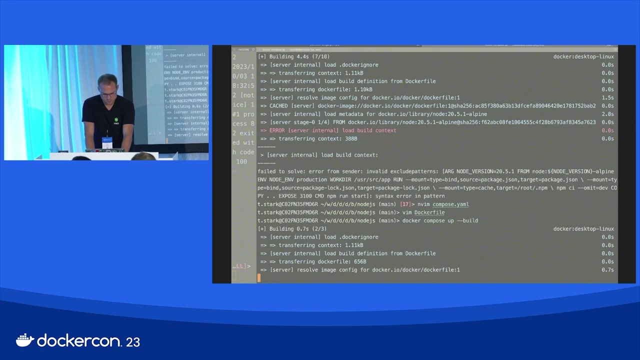 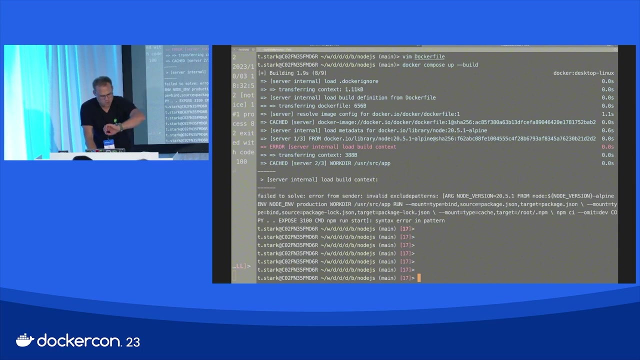 Oh, okay, Let me remove the caching real quick. I think we have screwed up something with that and we don't have enough time to fix it. It's still not working. All right, that's a bummer. That was the most important thing, by the way, almost. 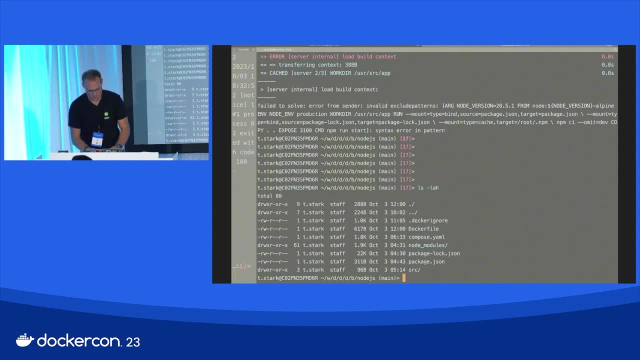 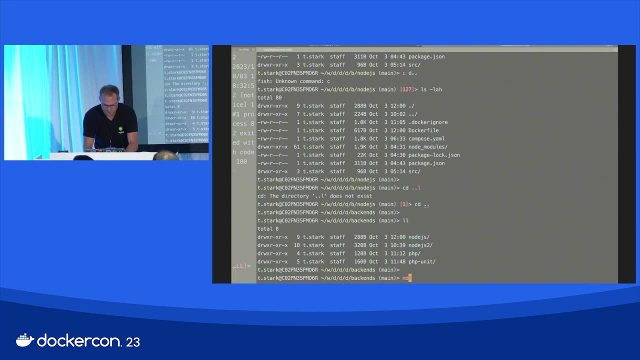 Yeah, basically it's like: then you change the file, it will trigger a rebuild. I know we are over time and then they will actually kill me if I'm running over time, but let me quickly fix that real quick. Nodejs. 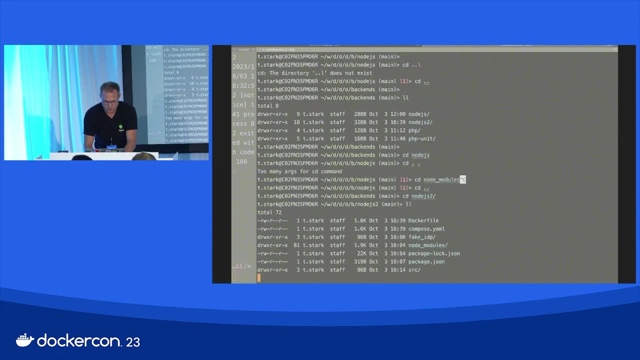 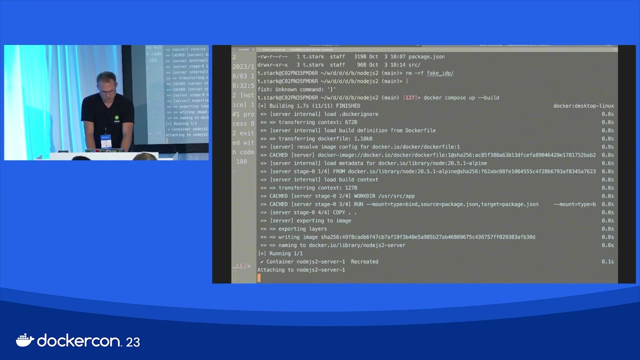 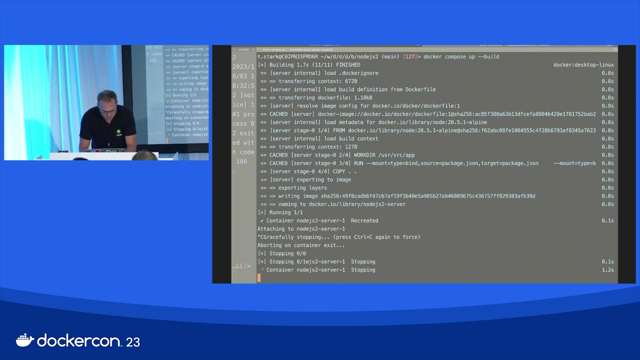 Trying to fix it real, real, real quick. Nodejs to RMRF fake backend. Was this working? by the way? I think that worked. Okay, then the docker-compose watch is working as well, So this works finally perfect. So let's do it here. 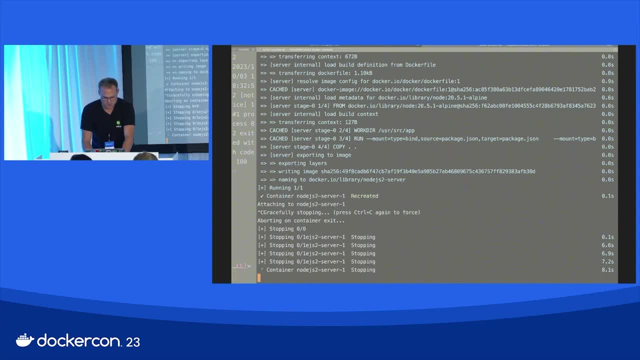 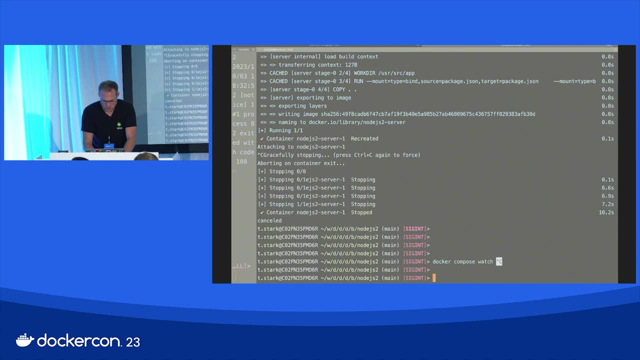 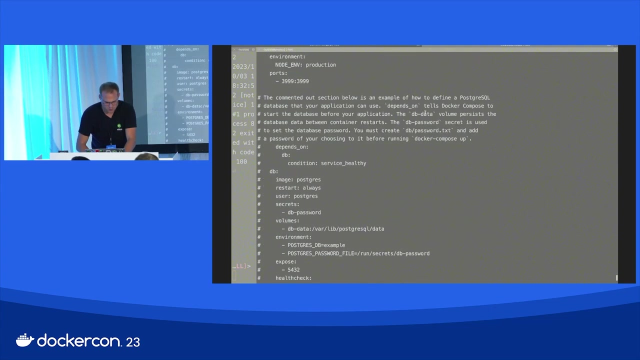 That's the other app we have created here, So let's do it. Let's do it. Okay. docker-compose- watch. It has no docker-compose things in it. Okay, fine, Nodejs compose. I'll just copy that real quick. 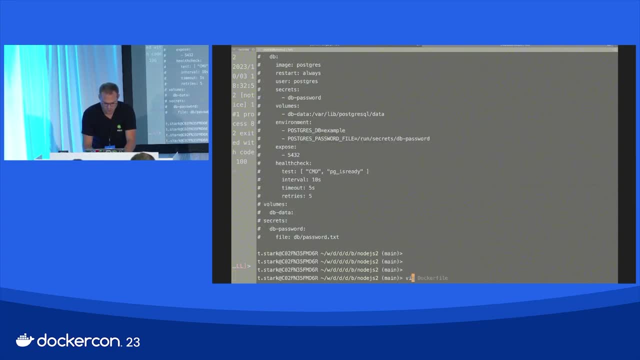 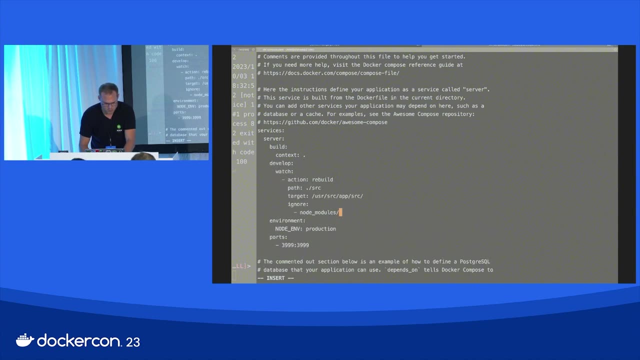 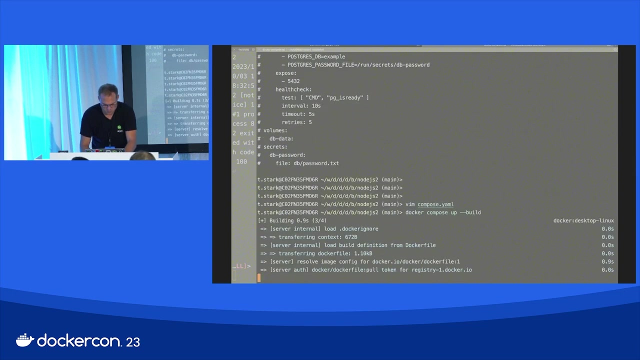 Copy. All right, It's working. And then the docker-compose watch. Now you are going to go back to your machine And you are going to go back to your machine, So let's paste that in Paste. that in. That's going to be a little lousy. 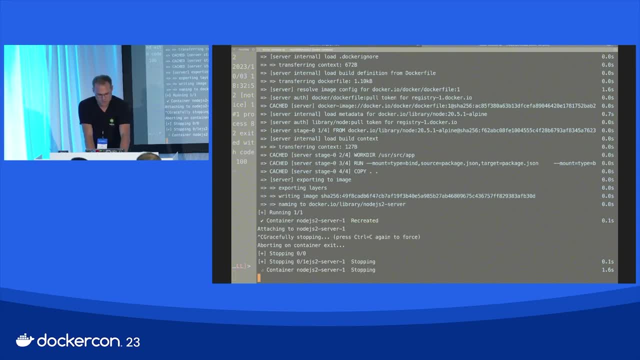 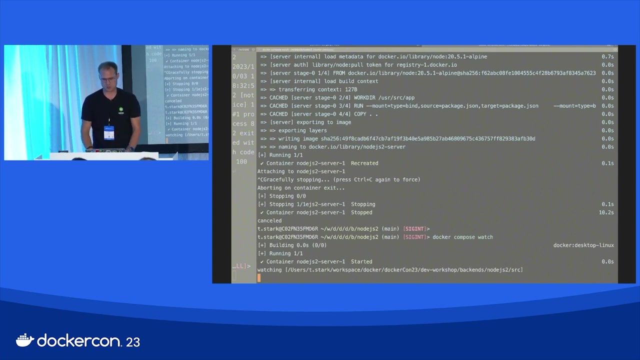 Okay, It's still working fine, All right. So now let's do the docker-compose watch thing. I don't know what's wrong with the other project, But now it should. But now it should work. docker-compose-watch- Okay, now it works. 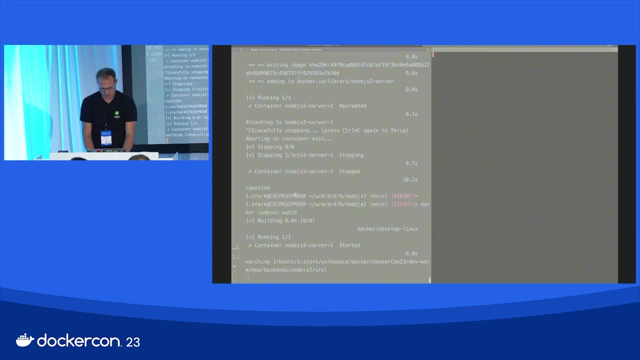 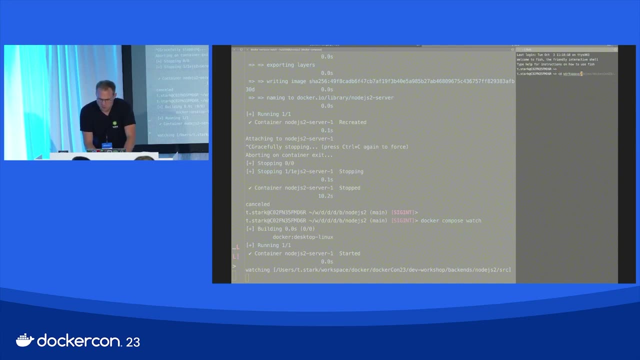 So now it says it's watching Nodejs source, and when we open up another window, I know it's small, but it's not really interesting what it says. So now I'm navigating to backends and then Nodejs 2, and in source we have indexjs. 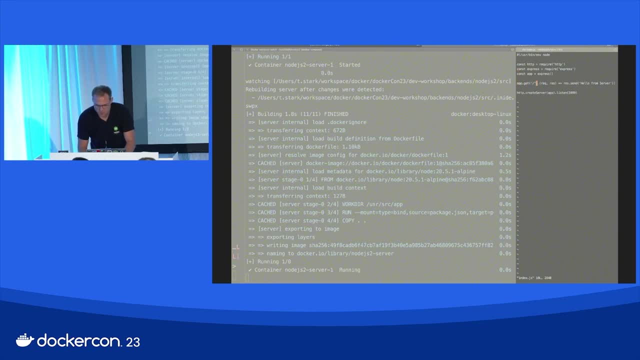 Oh, I already saw what happened. So now it's saying that is 3999.. That should print hello from server- amazing. So now we change that and say hello from compose-watch. We save it Now. look what's happening here on the left side. 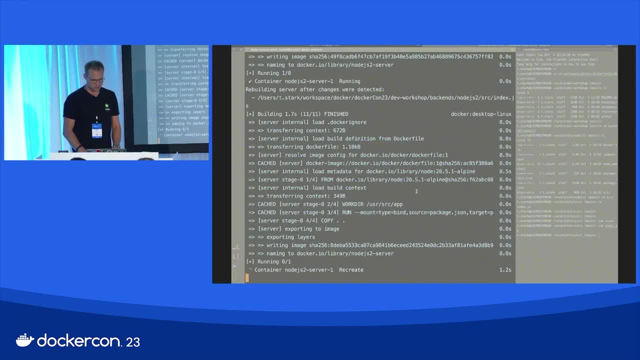 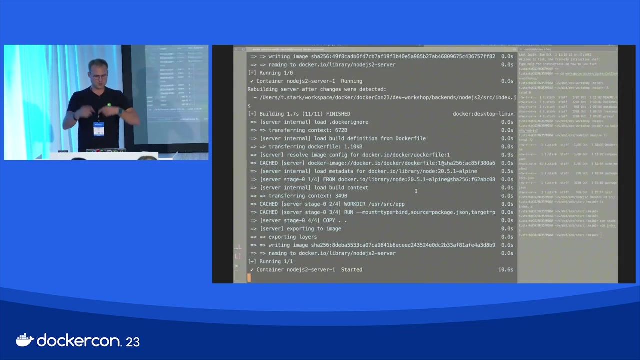 It detects that we have changed the indexjs file and now it's basically automatically regenerating and rebuilding the docker container. It will automatically boot it up and says: hello from compose-watch, So you don't have to do this step manually. then You change files and docker will automatically take changes. 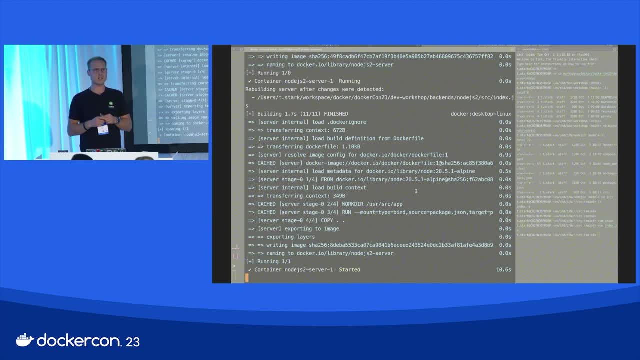 copying it into the container and kicks off the rebuild. Pretty handy, So you don't have to do that by yourself, right? So that was docker-compose-watch, and it's working. It has two intervals: One is sync and the other one is rebuild. 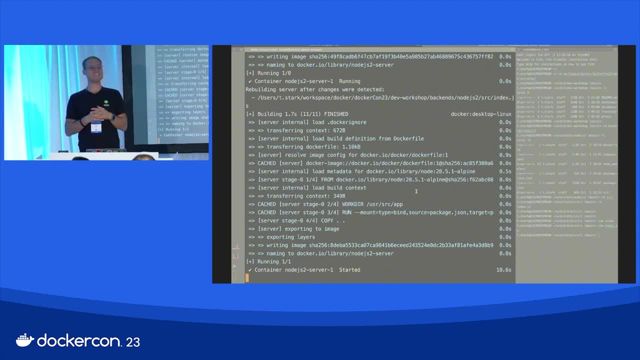 Perfect, Just four minutes- amazing. If you have now any questions, I think I will be around anyway, so we can close the official part and then I will be around for as many questions as you have. I will show you the SSL NGINX stuff. 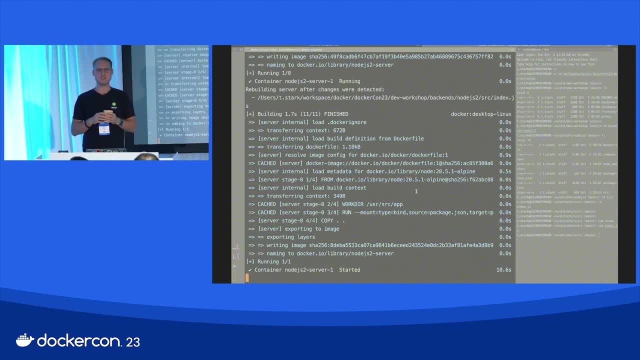 I promise Will do Right. What's the benefit of doing the docker-compose-watch instead of doing NPM watch? In this case, if you have NPM, the question was: what's the benefit of doing the docker-compose-watch instead of doing NPM watch? 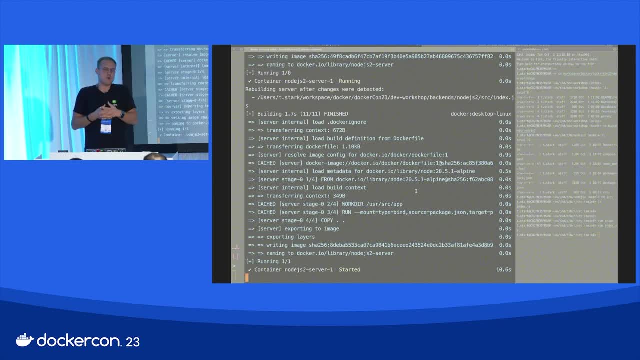 For development purpose. sometimes something like the NPM watch could be more efficient than the compose-watch, the compose-rebuild thing. As I said, it depends, Right, It depends. In my case, I'm most of the time using sync. 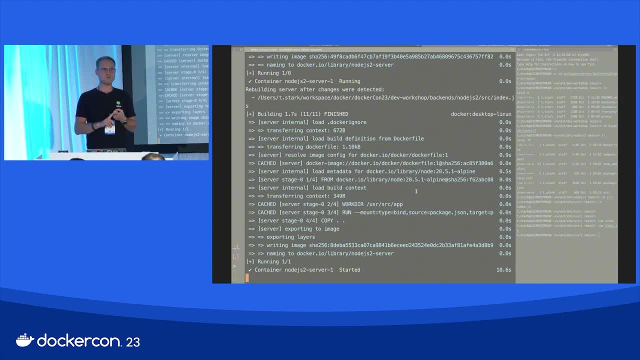 I'm using rebuild for things where node- something like watch in node- is not possible. for things like when I have a mock database, for example, and I have a SQL file and I edit the SQL file in my repository, save it. 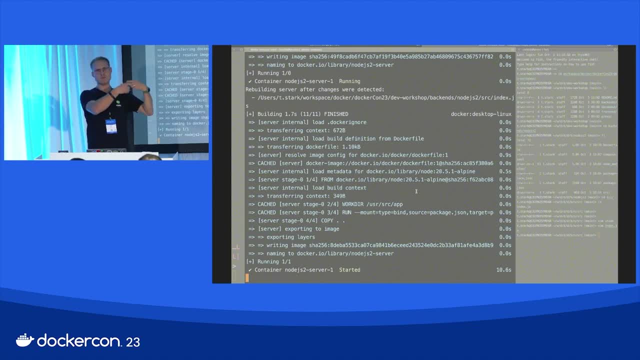 I create automatically a rebuilded version of my database with all the new SQL stuff in it. That's handy when you don't have something like NPM watch. That's what I'm saying. Maybe node is maybe here not the best example for rebuild. 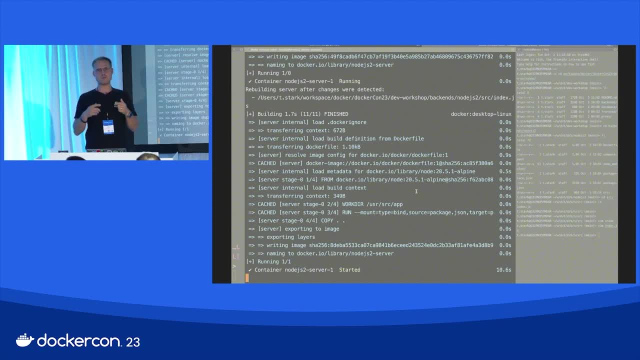 but I'm using it most of the time for database stuff. When I change things in the SQL file and I want to have a new version of the database, I don't want to have to kick this off manually. That's cool because it's under no brainer. 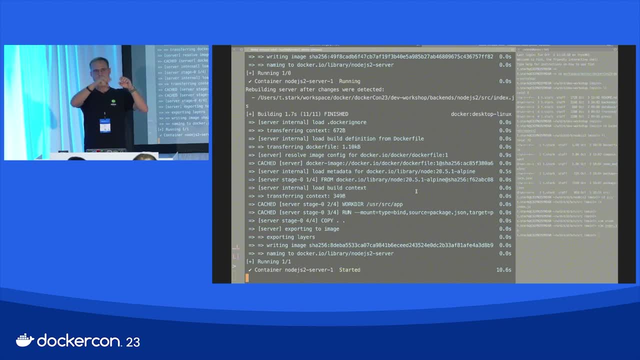 You have it in your. you have the database like dump SQL in your project directory. you need some other files. you just edit manually the SQL stuff, you save it and it will kick off the rebuild automatically somewhere in the background, without even. 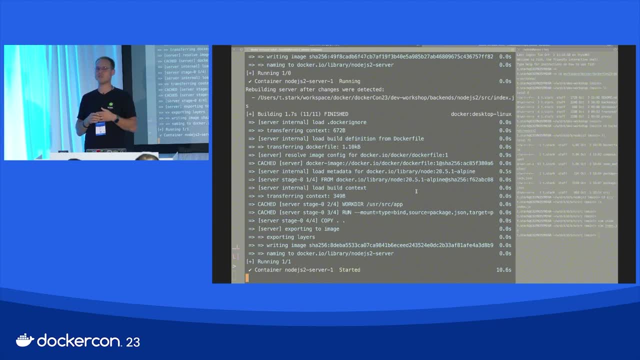 without your notice, You just have a new version of the database up and running and that is super important and super easy. Any more questions? If not, I think we can close the official thing then looking into the jury, the things Right.